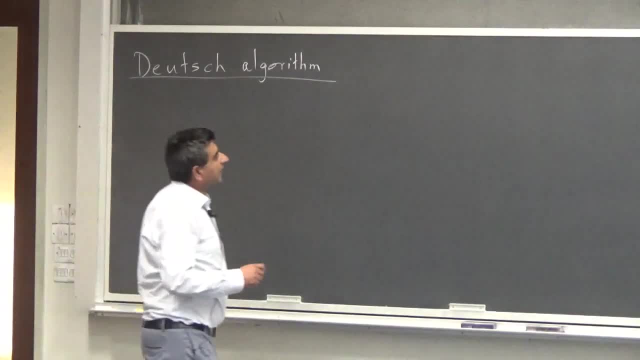 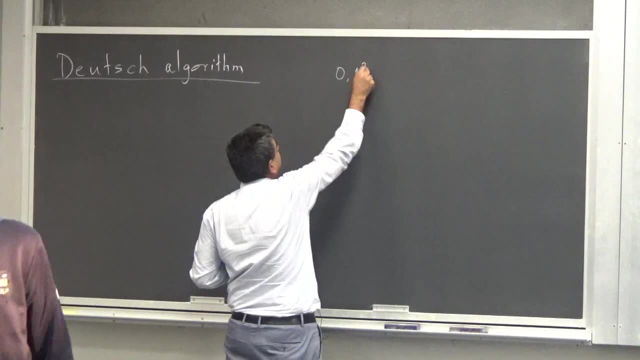 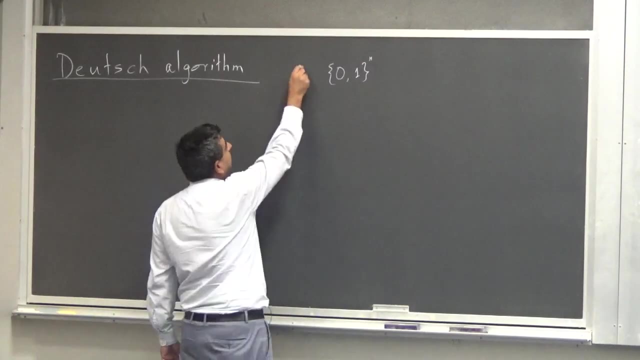 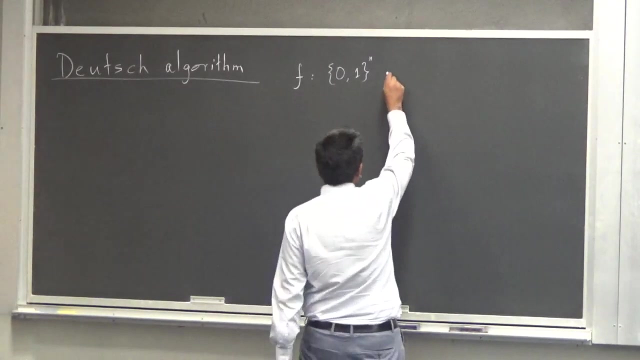 So the Deutsch Algorithm goes as follows: Suppose I have a string of bits- zeros and ones, zero and one, and I have n of them, And I define a function f that acts on this string and yields a binary number, zero or one. 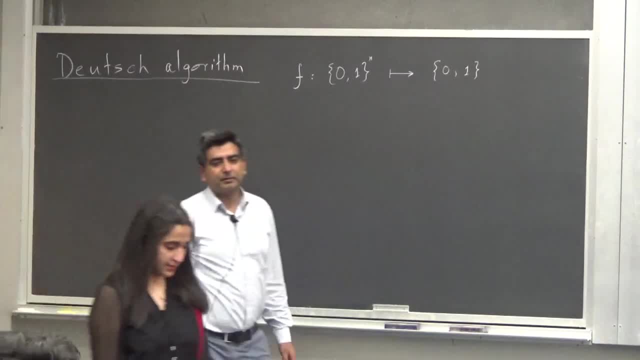 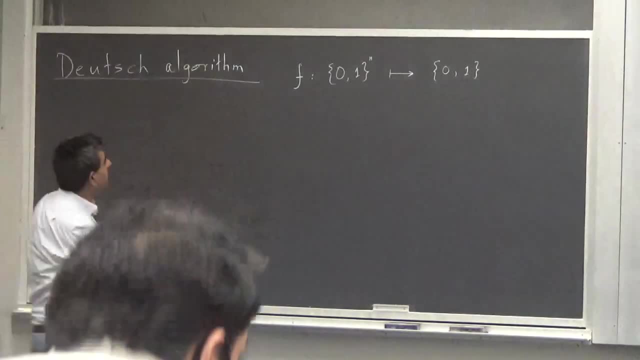 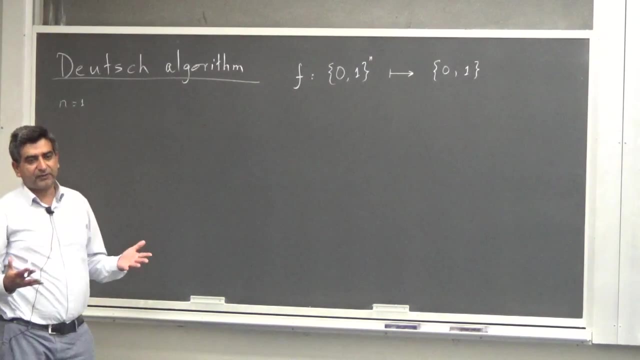 So to exemplify this, suppose my n equals one. So I'm looking at four kinds of functions. I'm looking at one function with two possible inputs, So I could have f equals zero, f of zero. This is some binary bit, zero or one. 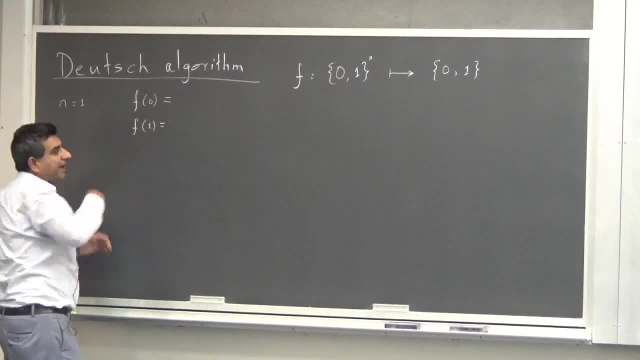 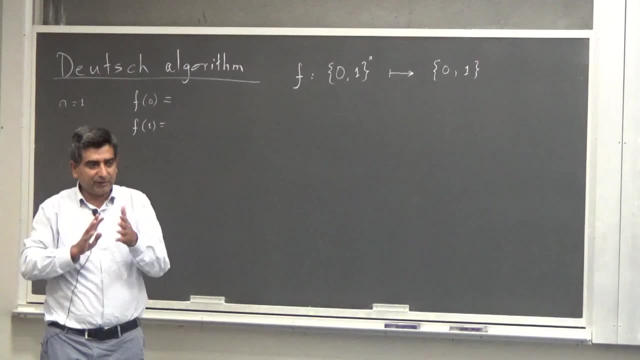 I can have f of one. The function acts on zero and one, So I'm just considering one-bit strings. The one-bit strings are zeros and ones, Just a zero and just a one. So this function can act on this string. So it's acting on this bit. 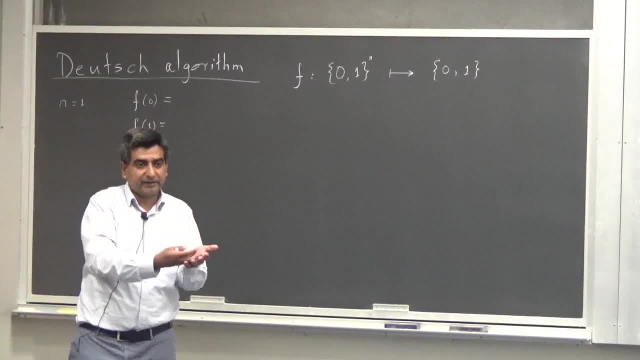 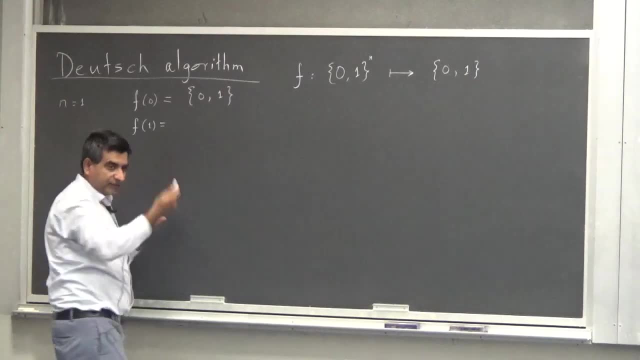 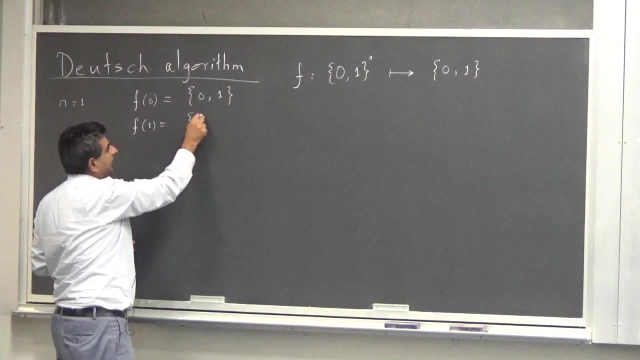 f acts on zero and yields something, The output could be zero or one. So this output could be zero or one, Either of them. And when f acts on the other kind of string, which is one, the output could be zero or one. 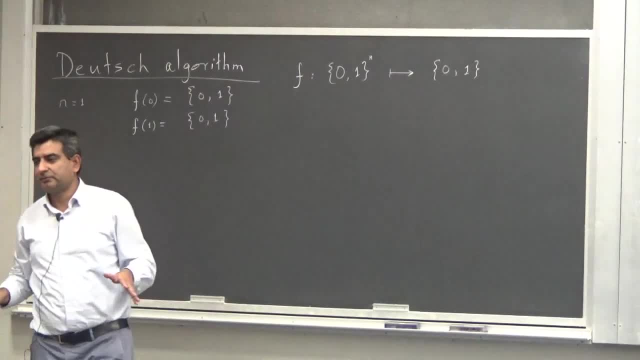 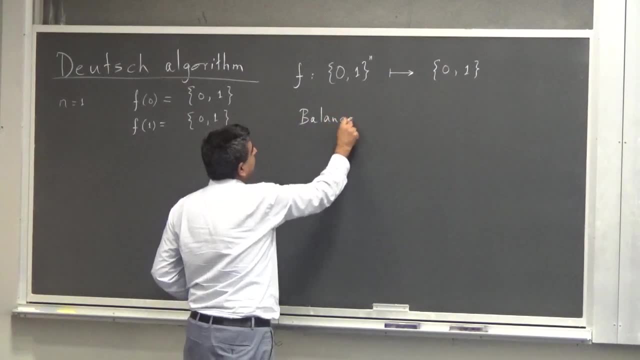 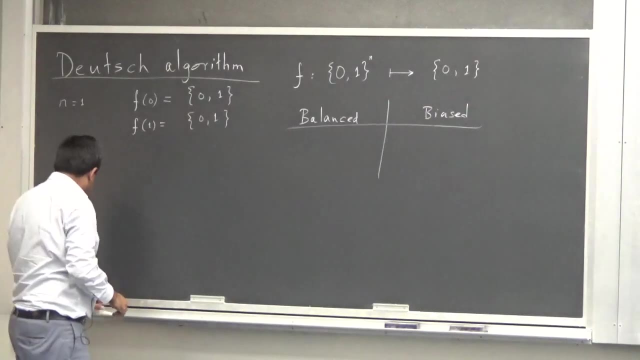 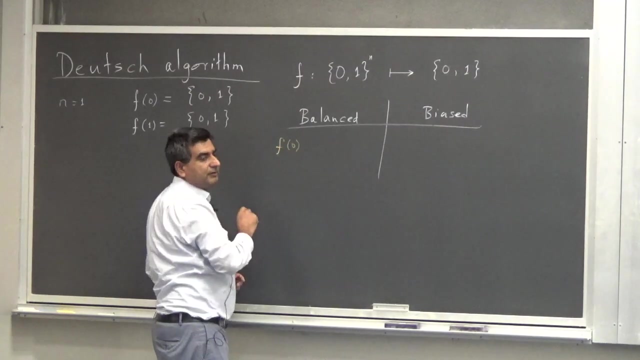 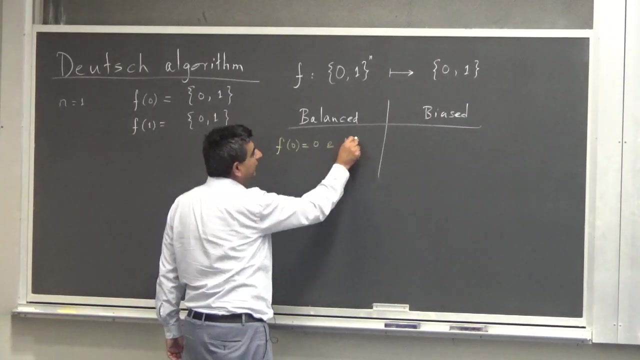 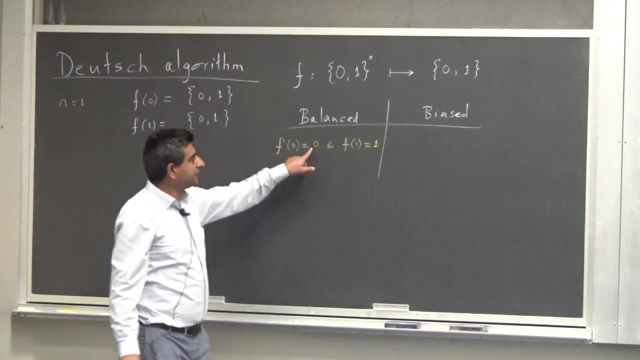 Now I distinguish between two kinds of functions: One I call a balanced function And the other I call a biased function. Now, example of a balanced function is that f acts on zero and yields me some number, say zero, And it acts on the other bit, one, and yields a number, a binary digit one, which is different from zero. 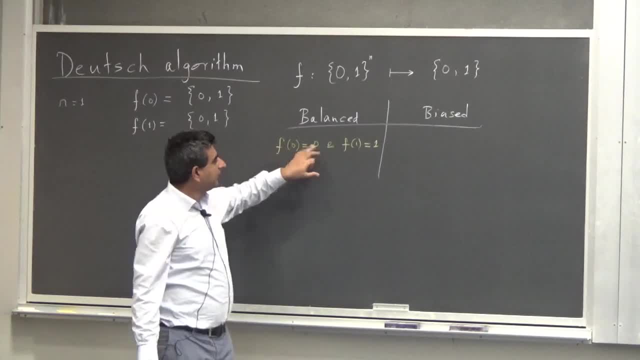 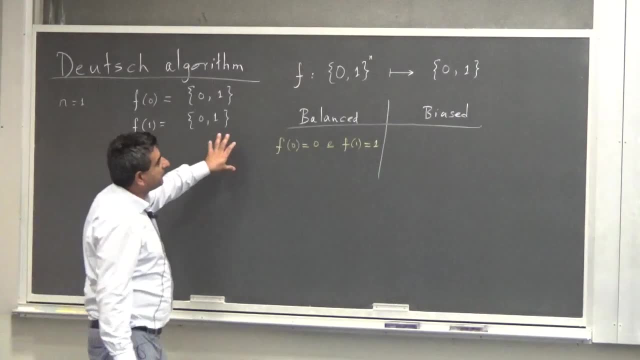 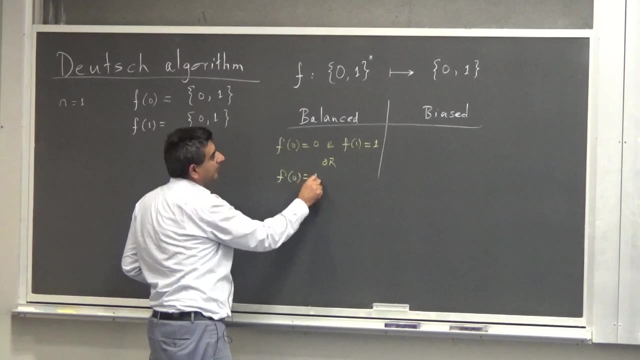 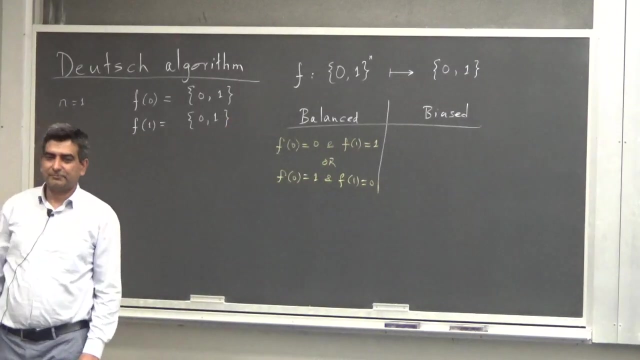 So when f acts on zero and on one, the outputs are different. So this is one example of a balanced function. The other possibility is that f acts on zero and yields one, And f acts on one and yields zero. So we have two kinds of balanced functions. 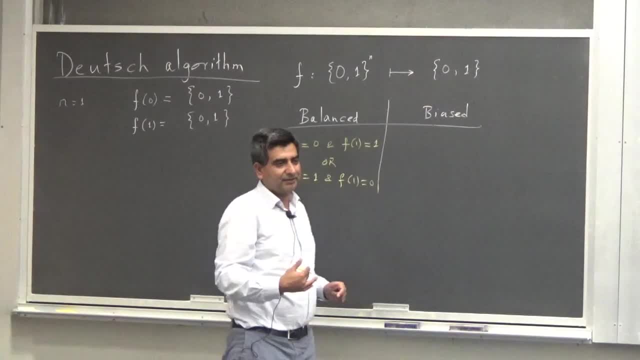 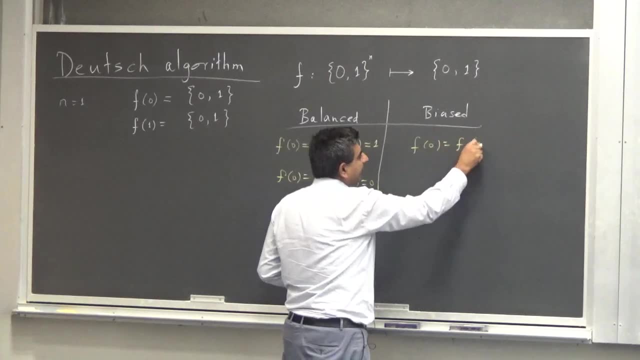 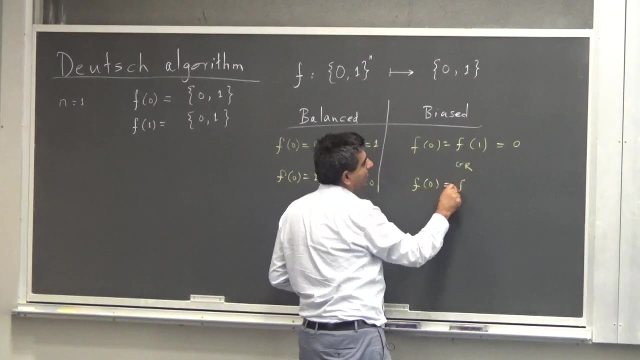 The other kind of a function is a biased function, And in a biased function, as you can imagine, that f acts on zero and the output is the same when f acts on one, And this output could be zero or it could be one. 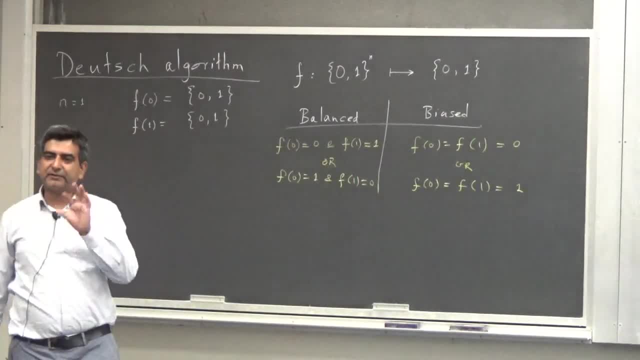 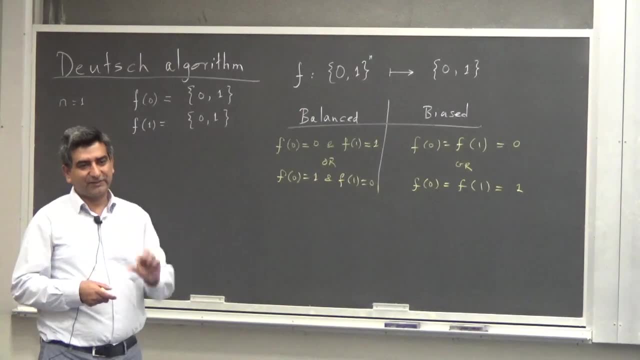 It's just like having a coin And you want to decide whether the coin is balanced or is it biased. Balanced means that there is a head on one side and a stain on the other side, And biased means that both of those sides have either heads. 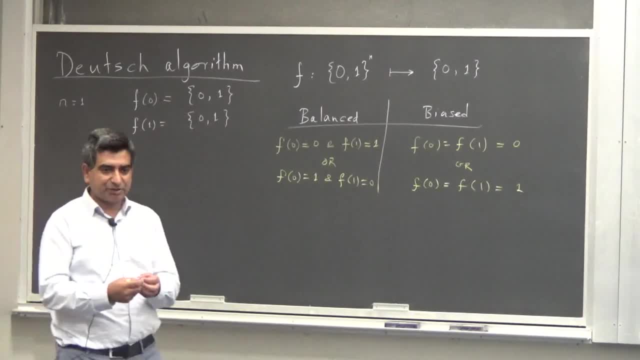 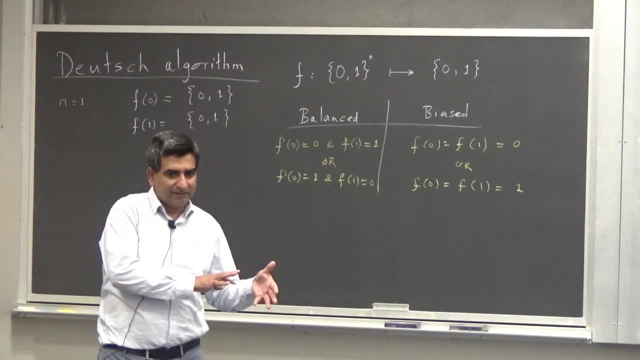 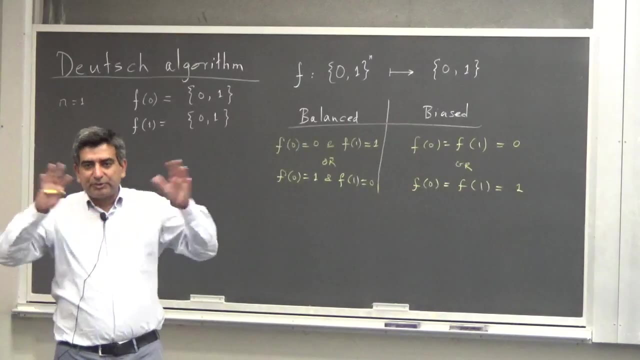 So you want to distinguish between the two scenarios, whether the coin is balanced or is it biased. So that's what the two kinds of functions are, And you would like to distinguish between these two kinds of functions. So that's the task at hand. 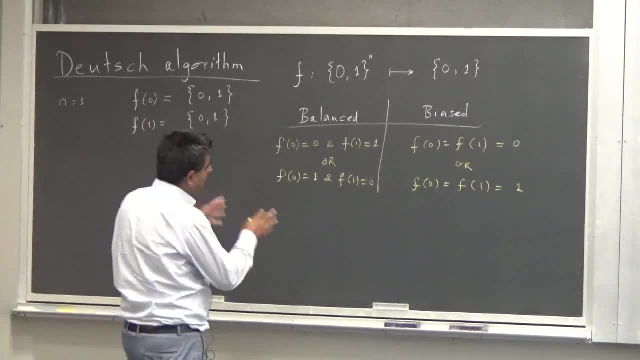 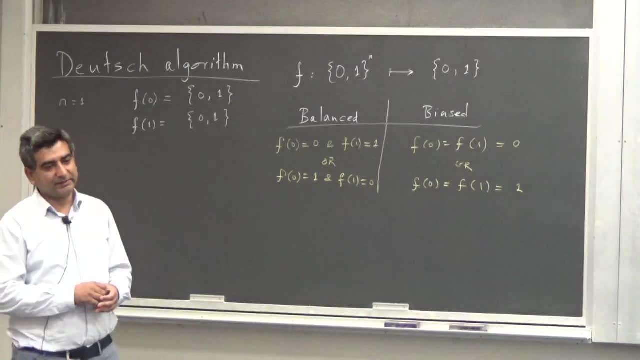 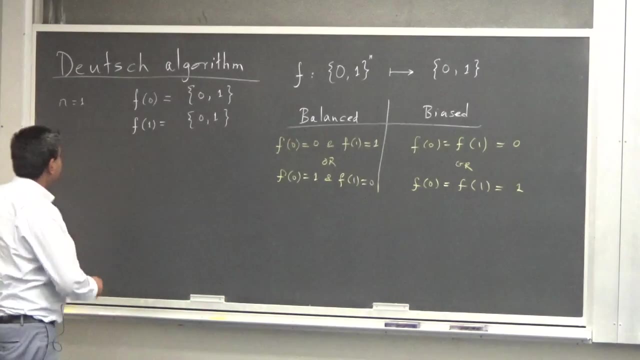 So we have a function f and we would like to tell whether it is biased- Is it biased or is it balanced? And in order to, the easiest approach to do this is: if you look at this classically, you could just have a box. 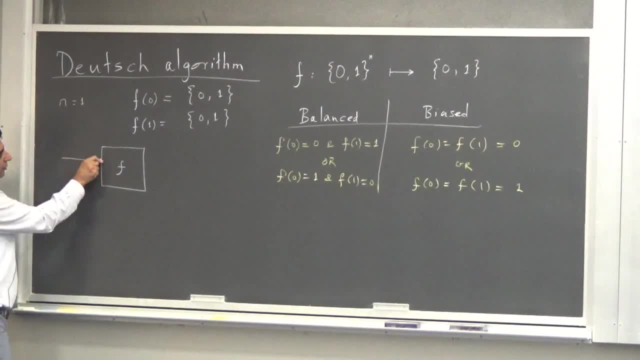 a black box that implements the function f. You input a state- zero. Now, this is a classical state coming in zero And you note what the output is. You have a detector, a classical detector, that notes what the output is, whether it is zero or one. 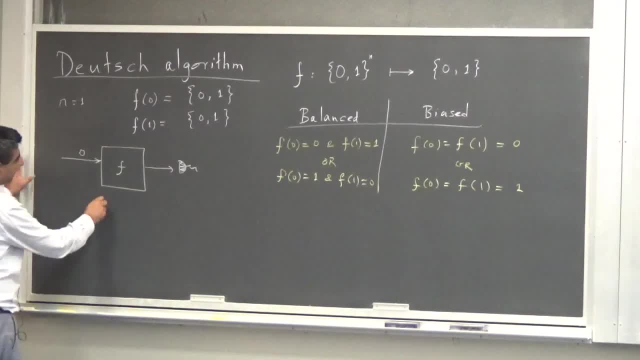 And then you repeat the experiment. So you do the experiment once in this fashion and then you repeat the experiment in another fashion and you see what the output is. So by doing these two queries, you can determine whether the function is balanced or biased. 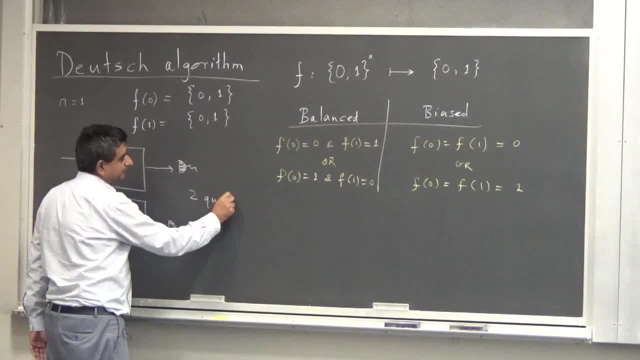 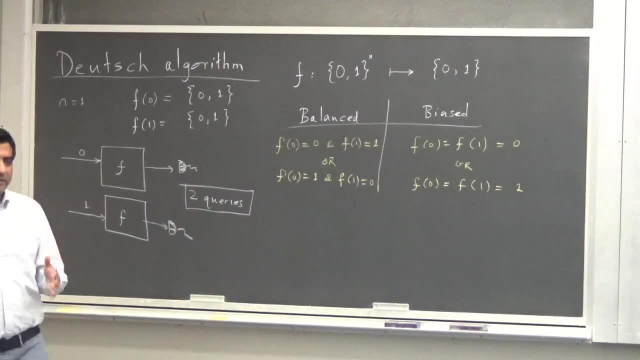 So you need two queries, classically. However, let's take advantage of the idea of superposition and initialize a quantum computer so that both of these inputs are fed into the quantum computer at the same time, And our idea and motivation is to do one-shot determination. 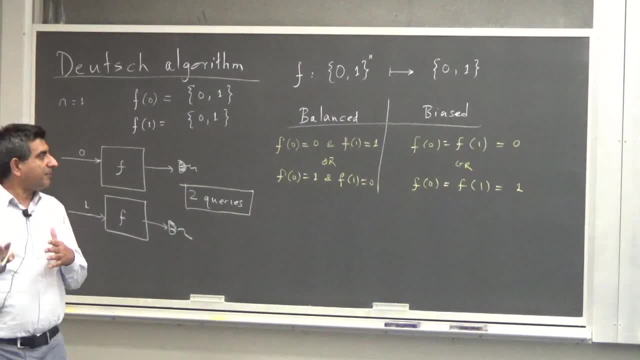 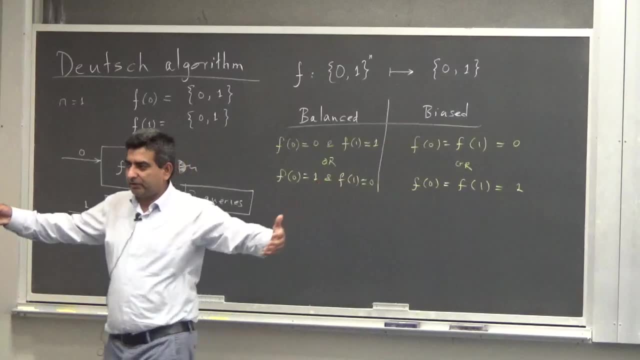 and discrimination between a balanced and a biased function. So we want to do it in one shot, And right now our n is one. You can have longer strings as well, And you want to distinguish between the different kinds of functions by just doing the experiment once. 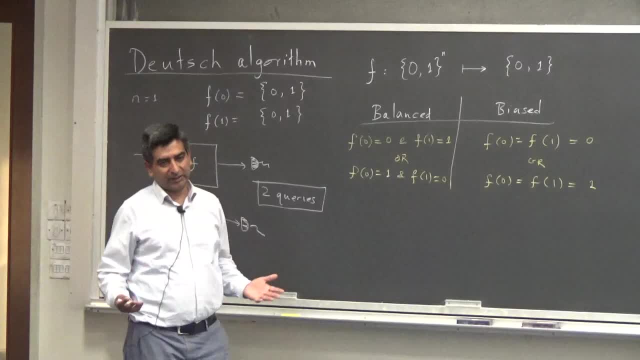 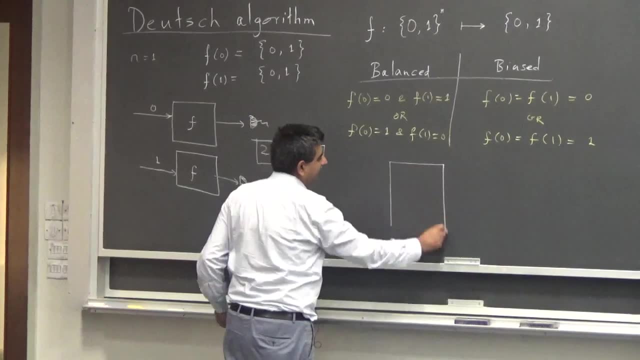 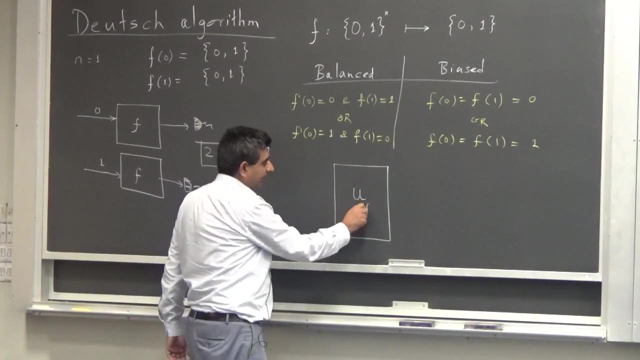 So instead of having two queries, let's see if we can reduce this number to a single query. So if I were to design a quantum computer or a quantum circuit, let's call this circuit U sub F. So this is a unitary propagator or a unitary operator. 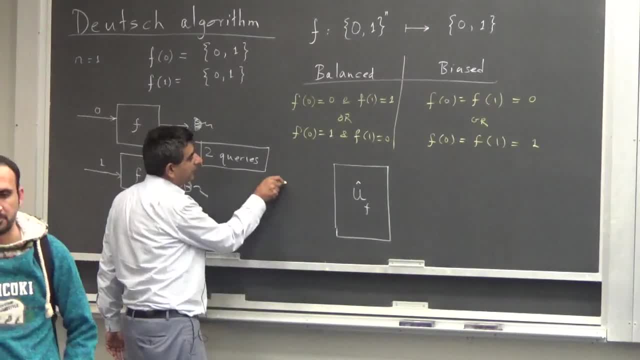 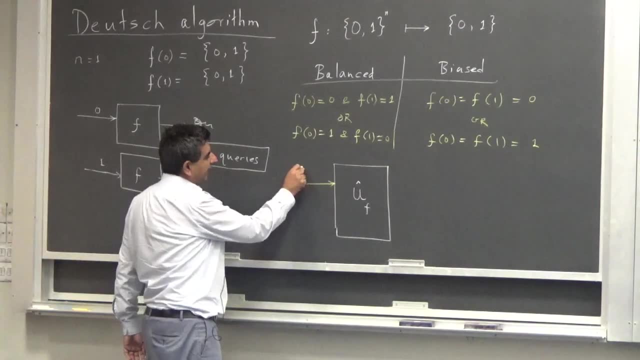 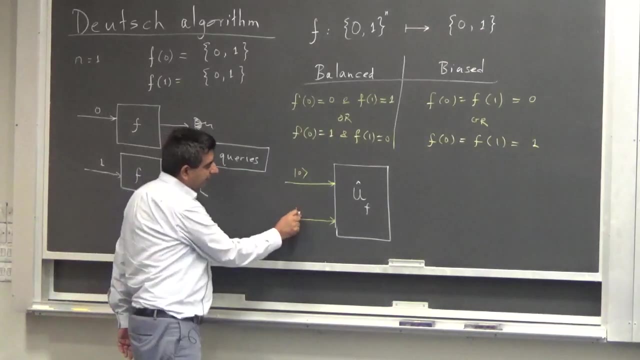 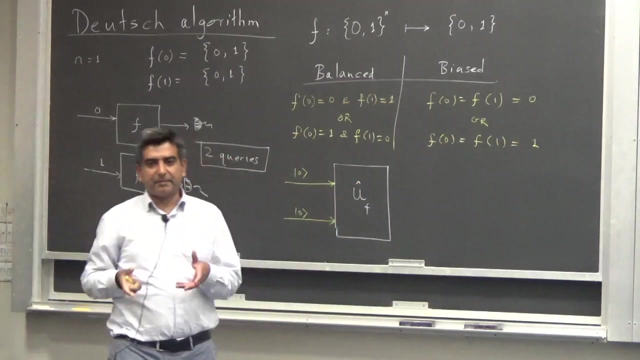 And let's suppose that I have two inputs. I encode my initial states as a quantum state, So I encode as ket 0. And then I have an auxiliary qubit. It is also in the state ket 0. And somehow this unitary function is designed in a manner. 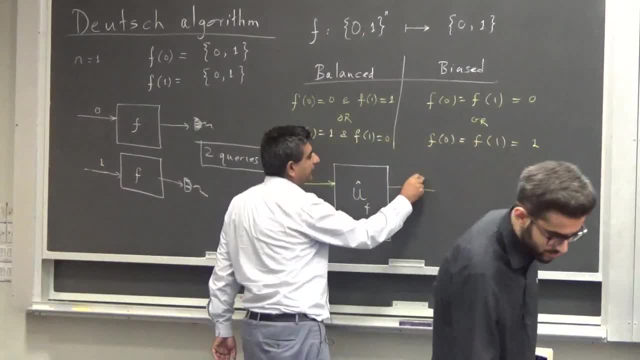 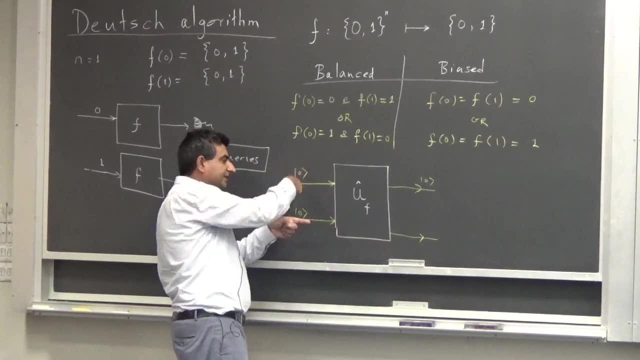 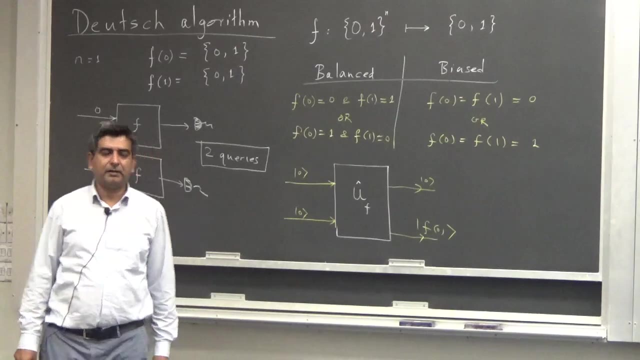 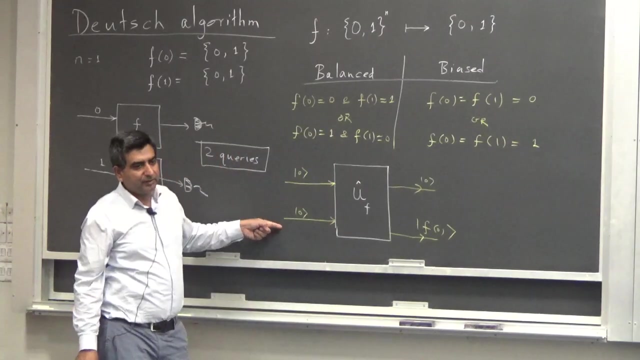 that nothing happens to the first qubit but the value of the function acting on the first qubit is encoded into the second qubit. So I am hypothesizing that we can make a quantum circuit that does this. It takes two inputs. One is on this channel we are inputting our quantum state. 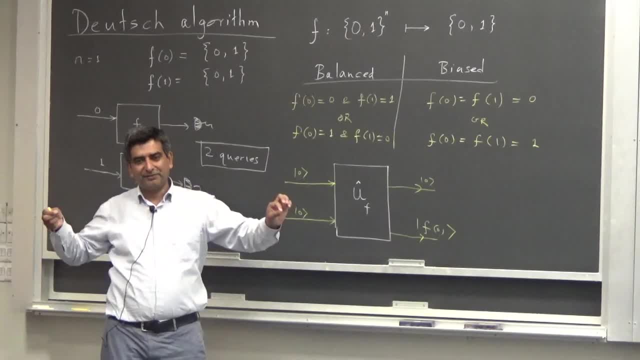 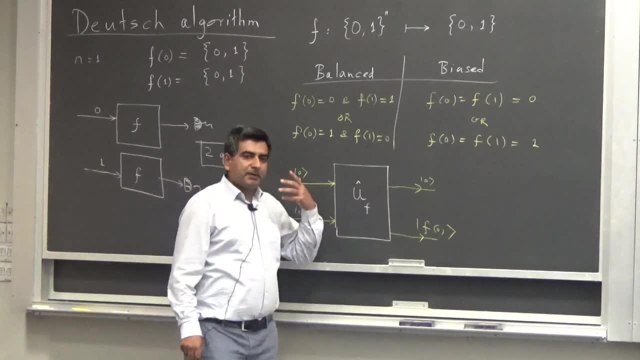 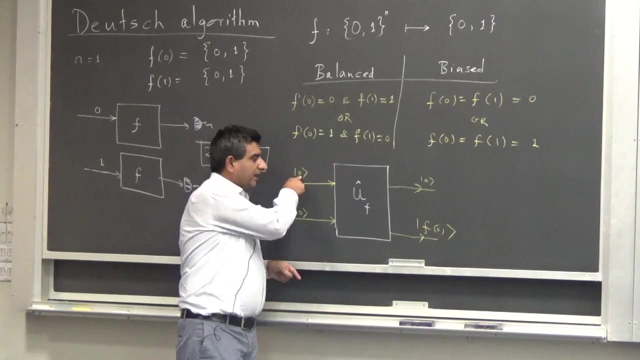 We would have to find out what is the role of the function on this quantum state. And we also put in an auxiliary qubit Or an auxiliary qubit And just design this quantum circuit so that the action of F on this logical label is reflected in the state of the second qubit. 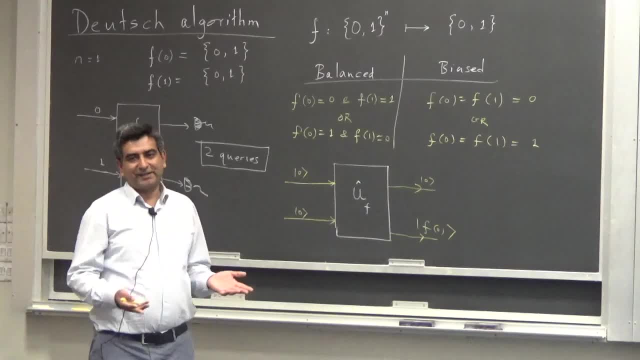 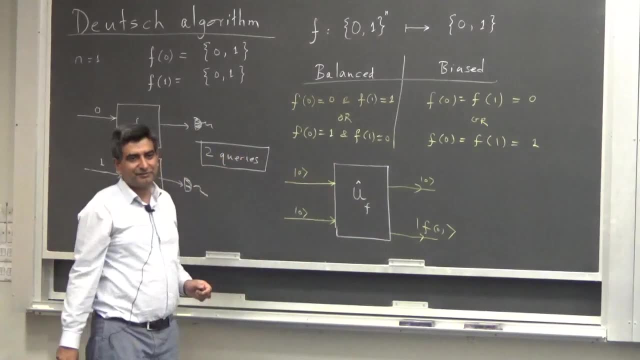 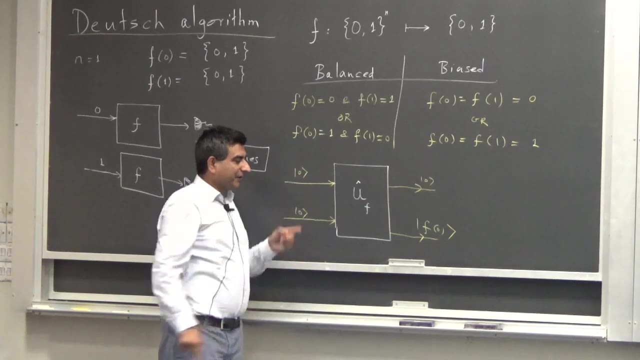 So this is one possible way of doing this task, But you would have to run this circuit once with ket 0 as the input, And then you would have to run this circuit once with ket 1 as the input. So in each case you will determine what the value of the function is. 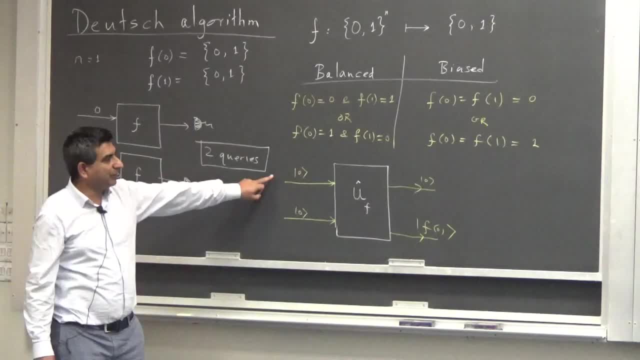 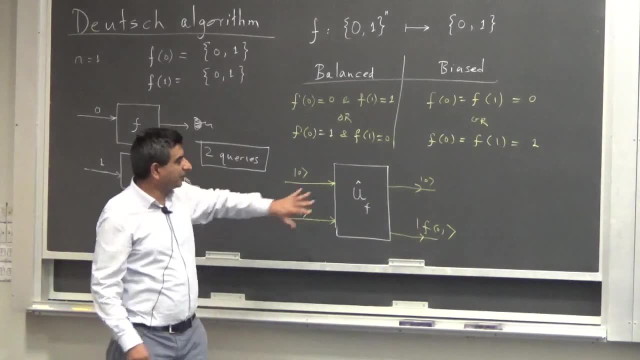 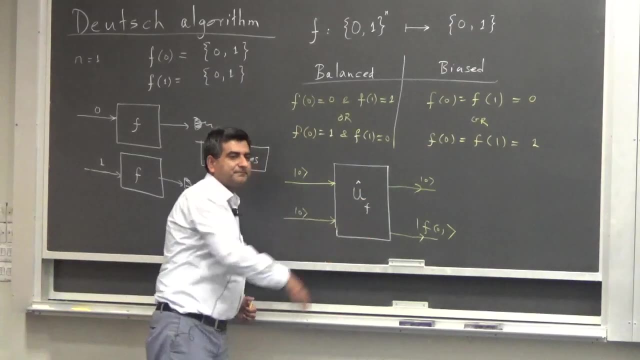 But you will have to do two queries, One with ket 0 as the input and one with ket 1 as the input. Got it Now. can you come up with a circuit? We have seen many circuits in the past. Can you come up with a circuit that does this? 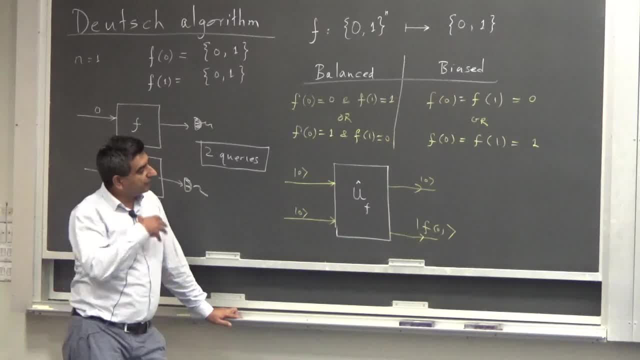 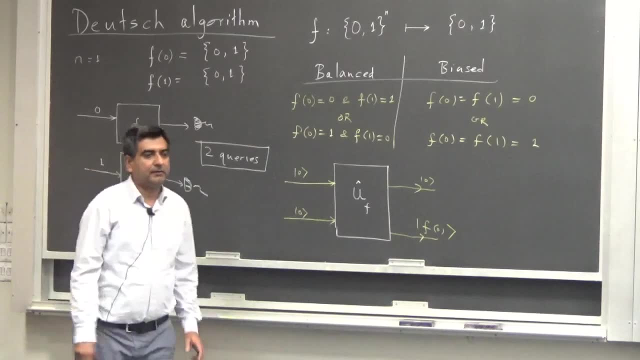 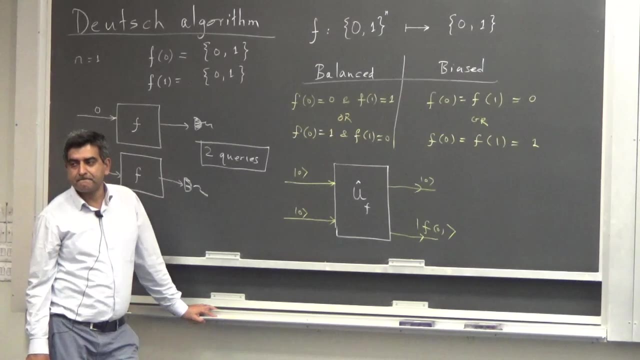 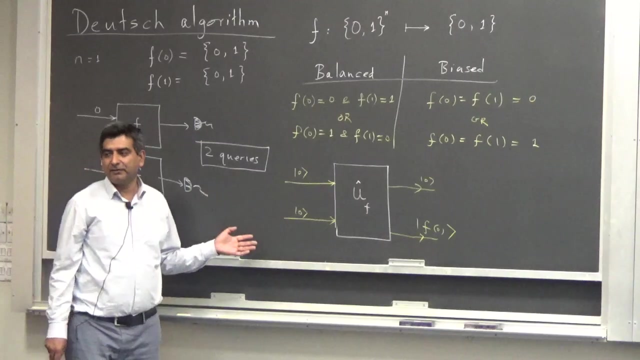 What kind of quantum circuit or logic gate needs to be applied here? Yes, How did you decide that you are going to use ket 0? So we have to initialize it in some manner. This is one possibility that this is ket 0.. 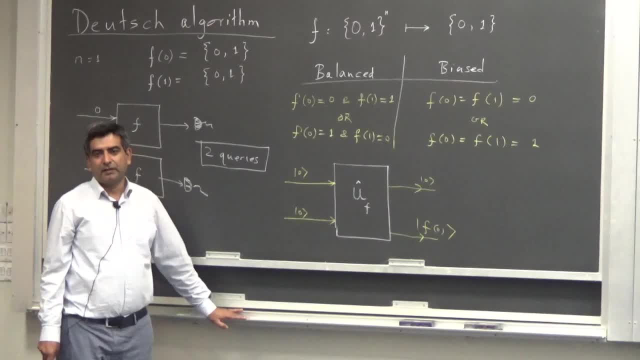 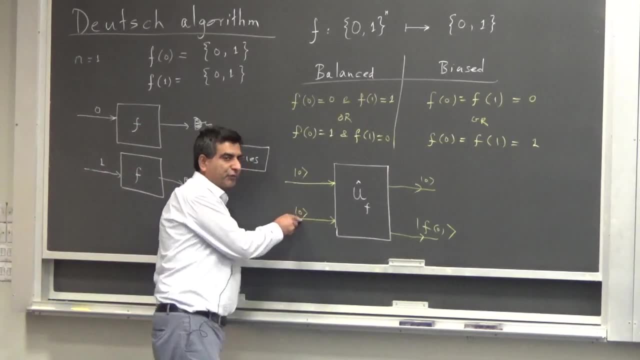 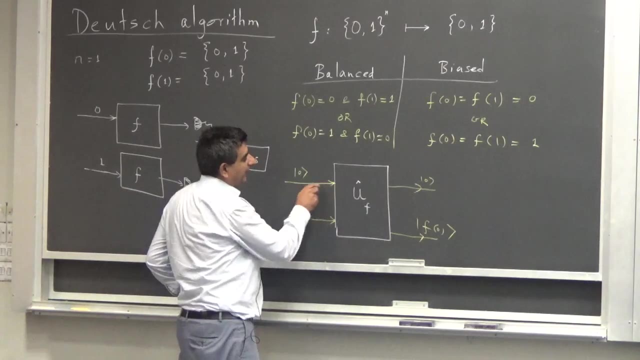 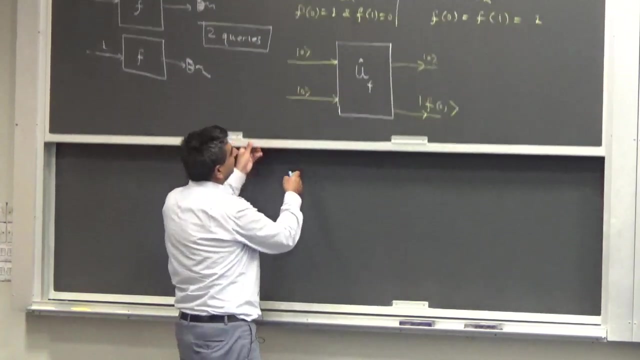 Could be anything else. Yes, Sir, control naught, Control naught, But control naught is always going to invert this. So it is similar to control naught, Suppose I do the following. So what I do is on this channel. let me redraw this. 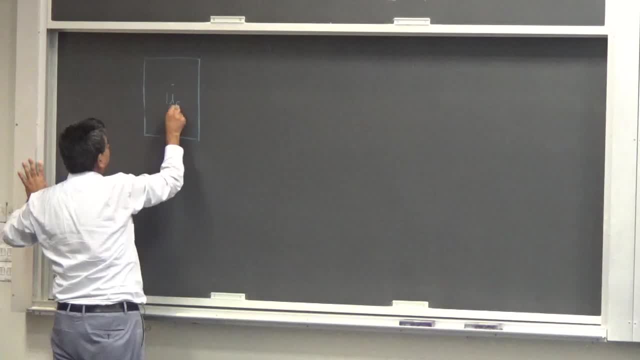 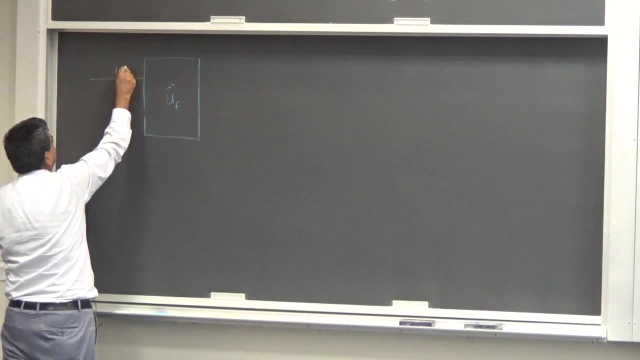 A UF that does the following will work. following will work. I have an input, ket A. A could be 0 or 1, this is ket 0, something happening here. I am building a quantum circuit that does something and this output remains. 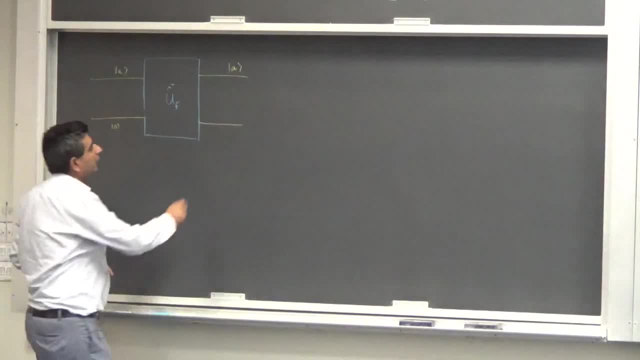 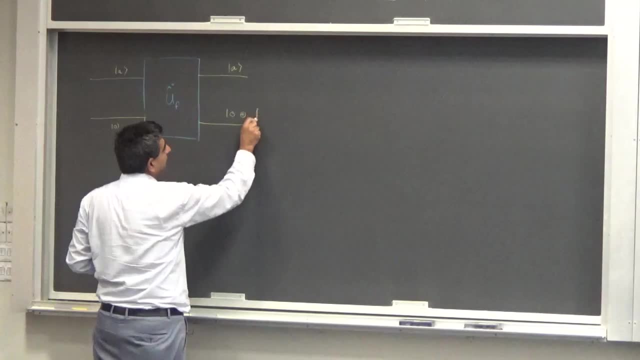 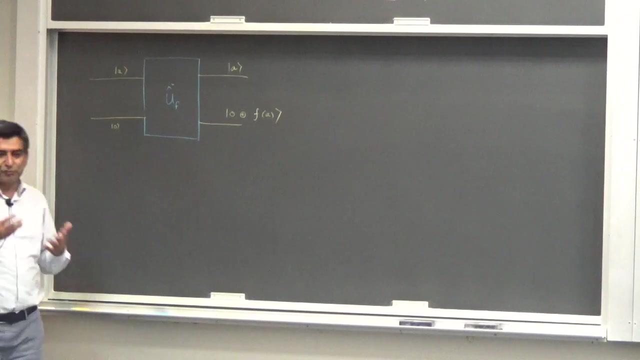 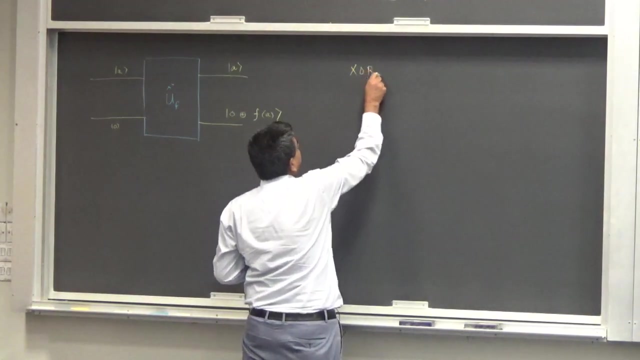 ket A, whereas this output is this state: 0 plus the exclusive OR of the function acting on this logical bit. So I need to implement a circuit that does an exclusive OR. so what is the truth table for an exclusive OR? Exclusive OR is represented by this function here an. 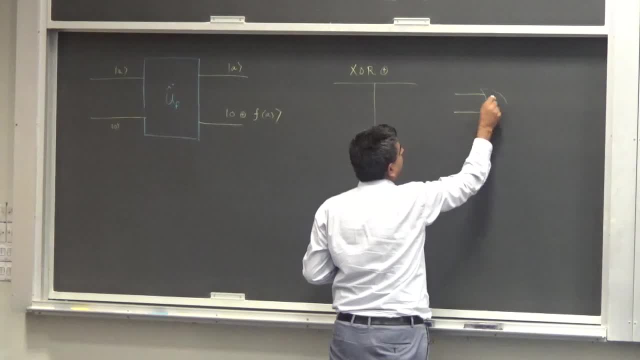 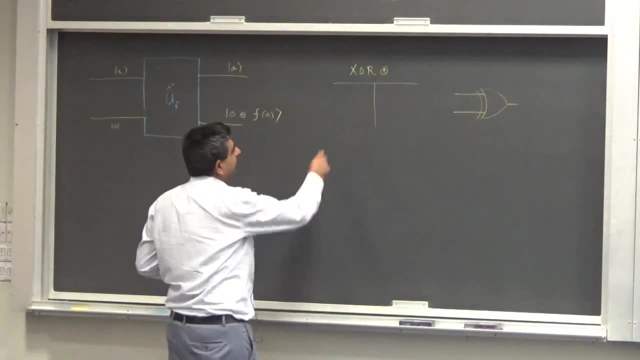 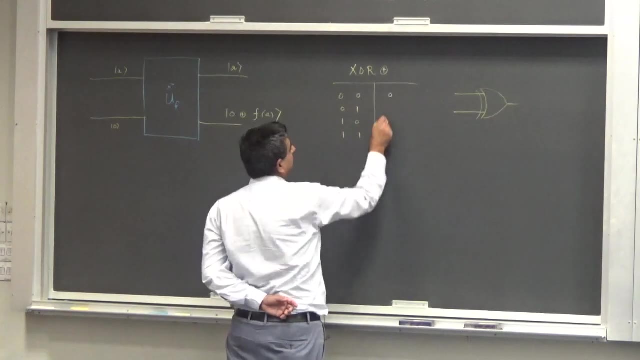 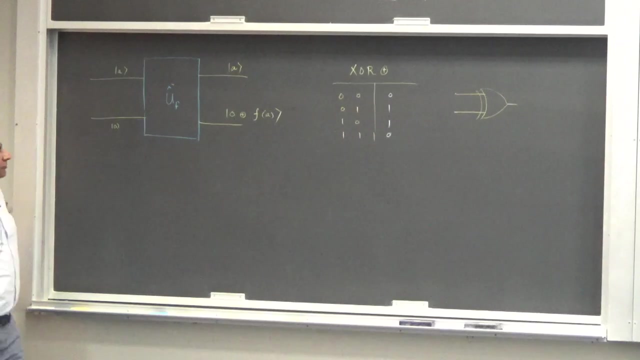 exclusive OR I, I think is represented in this fashion. So what it does is, if the inputs are the same, the output is 0,. inputs are different, the output is 1.. So you do an exclusive OR of the state of this qubit 0 with the function acting on A. So you 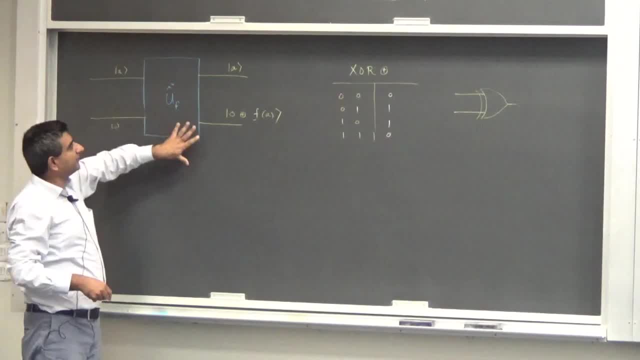 build your quantum circuit in such a way that this scheme is implemented. And why do you need two outputs? Because you have two inputs. The number of outputs needs to be the same as the number of inputs if you were to do a unitary operation. 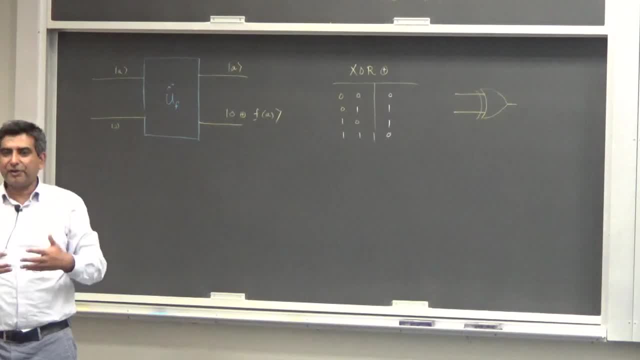 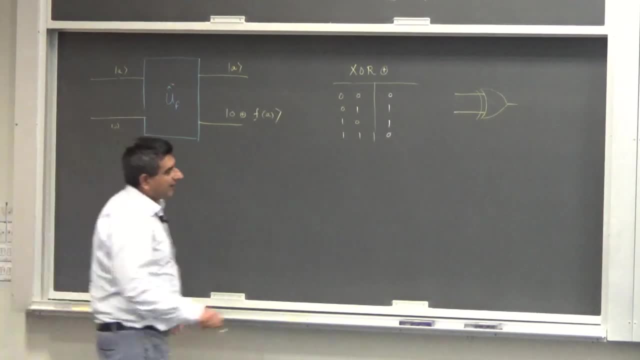 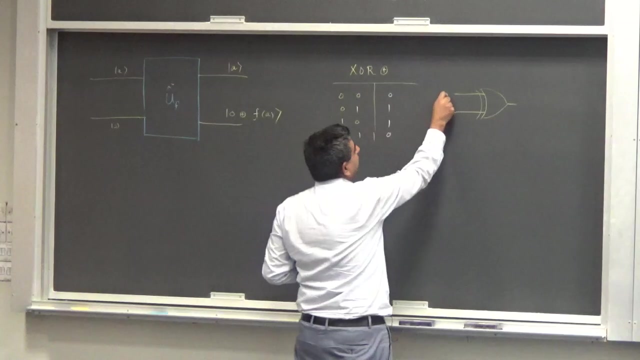 Otherwise the operation will be non-unitary, Because a unitary operation is reversible If you just so an AND gate, for example. this gate, as drawn here, is non-unitary because it takes certain inputs, gives you an output, but looking at this output you cannot tell what the 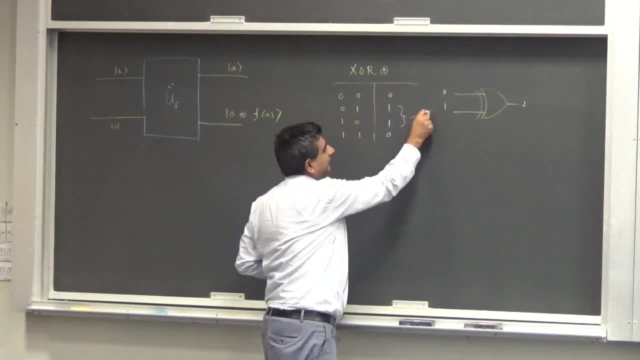 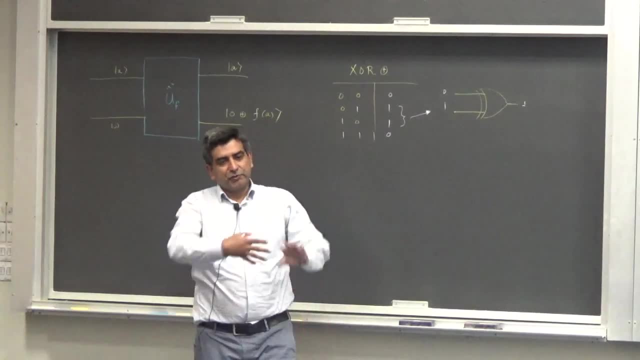 inputs are because there are two possibilities here. If the output is 1, the 0 could be on the first bit or it could be on the second bit. So you cannot reverse this gate. So if you want to do unitary operations, which most quantum computing is, you would have to. 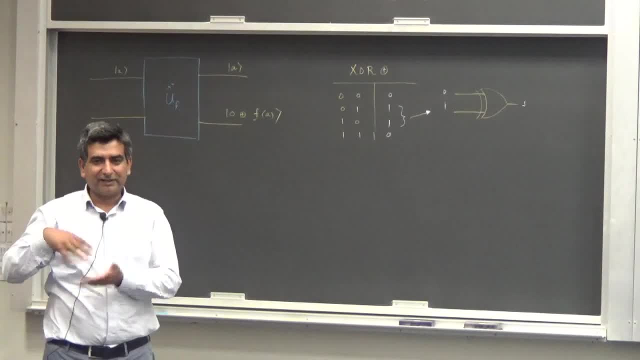 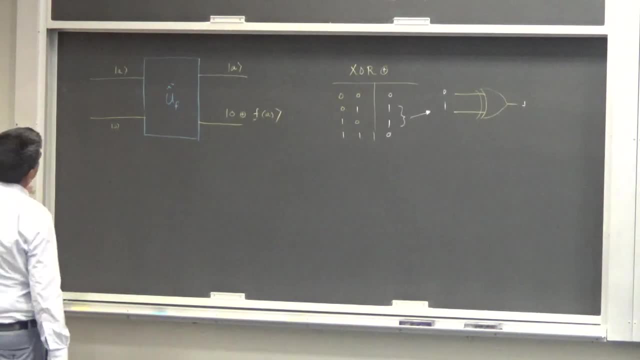 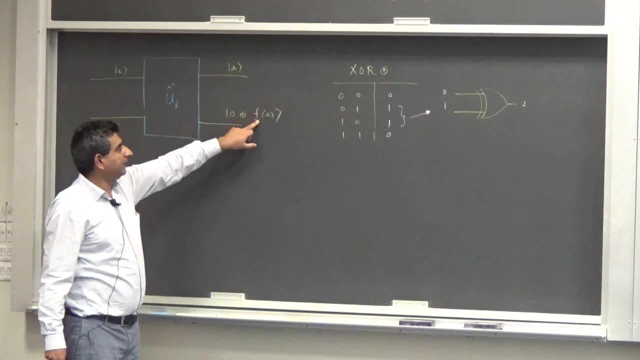 have the same number of outputs as the number of inputs. Otherwise your gates would not be reversible. So one possibility of determining this function is- and, by the way, if you take the exclusive OR of 0 with f, this is always going to turn out to be f. 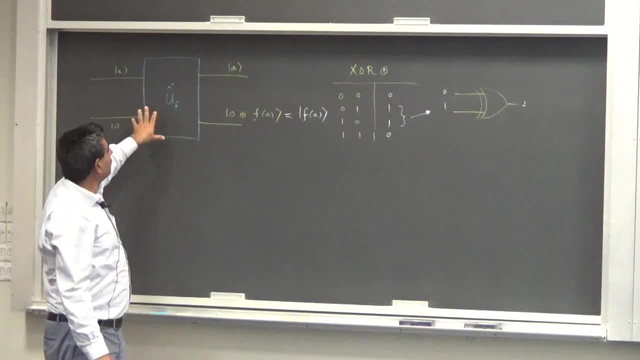 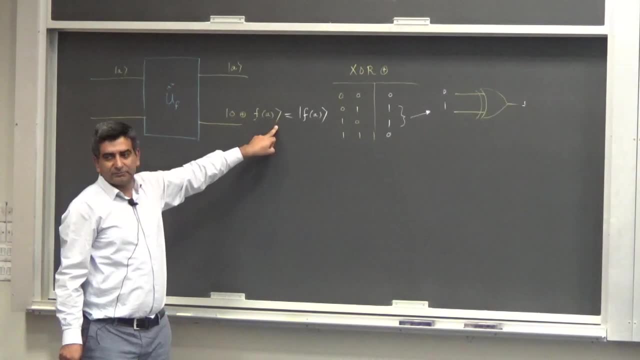 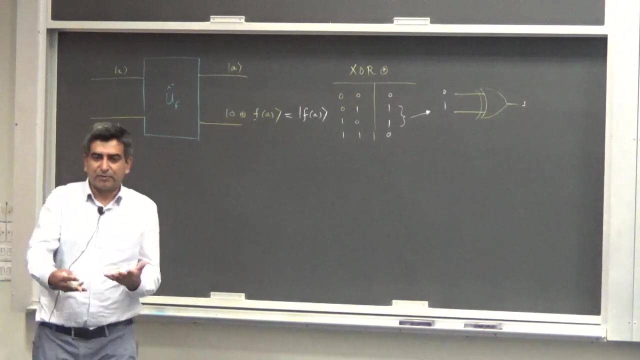 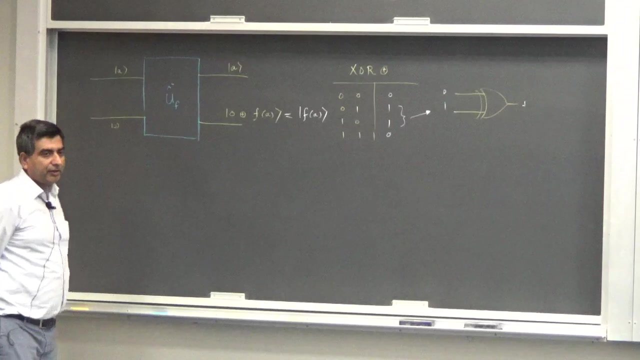 Correct. So you have encoded the output of the function acting on this state in the second qubit, in the state of the second qubit. Alright, So you need to implement this exclusive OR gate on a quantum computer. Alright, So you have to design this in a manner. it's this: so you have to build this UF so that 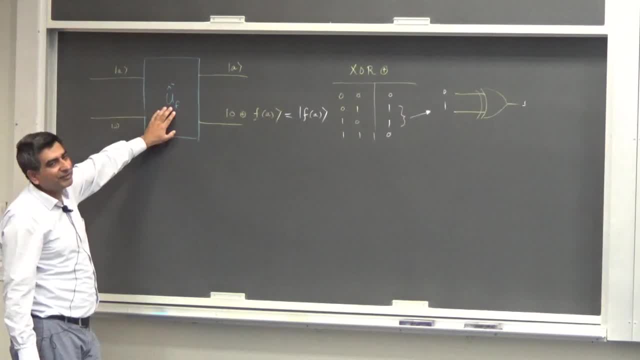 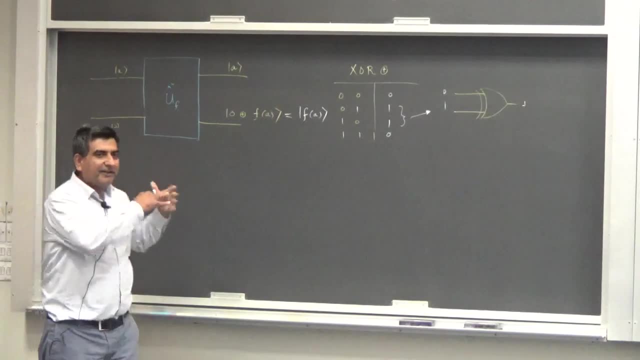 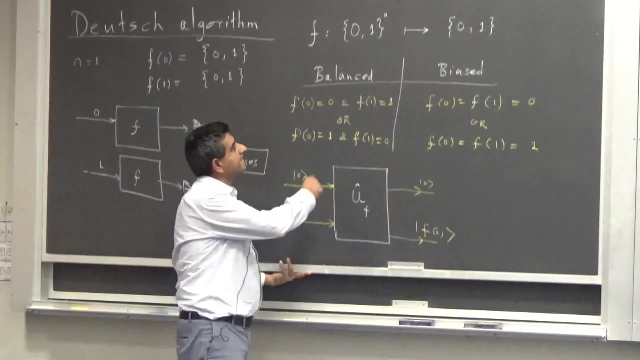 it does this function, it implements this function. it's not a straight forward, exclusive operation. you have to design this quantum circuit so that it achieves the desired task. For example, looking at these possibilities, this could be homework problem, say, our function. 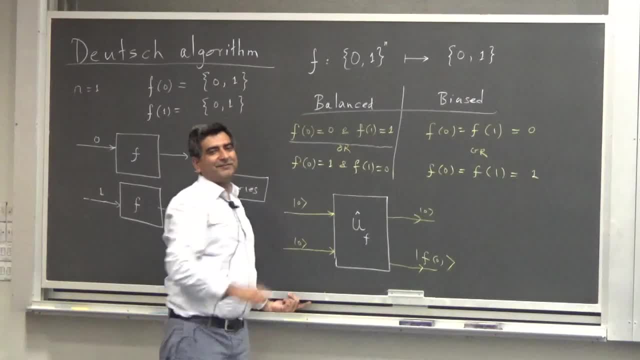 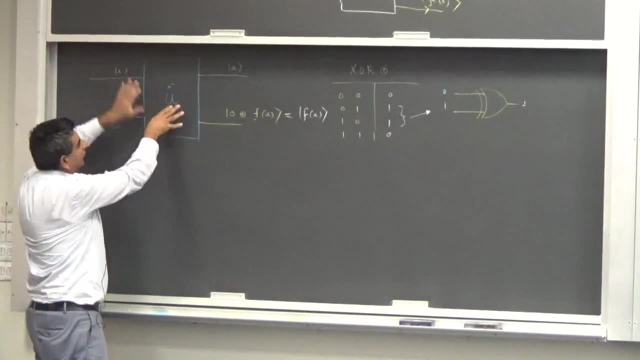 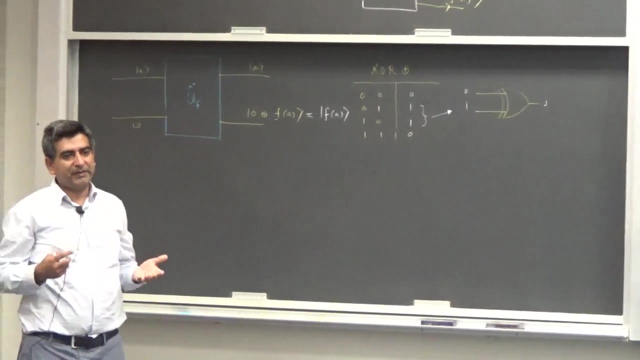 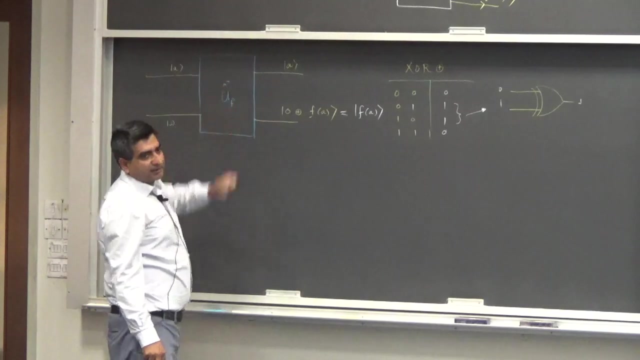 does this. can you design a UF that implements this and draw the circuit model for UF in here, in this box here? Okay, so that's what engineering the quantum computer means: you have to design out of many elementary gates something that goes inside the black box. 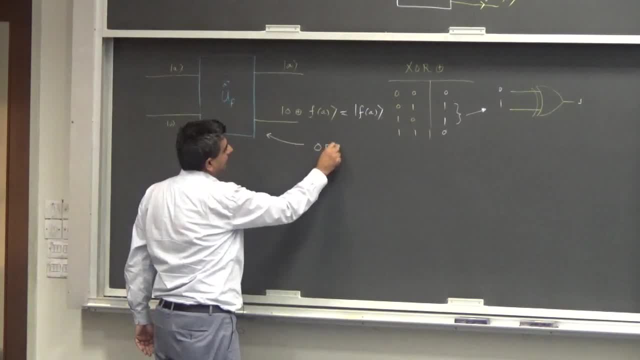 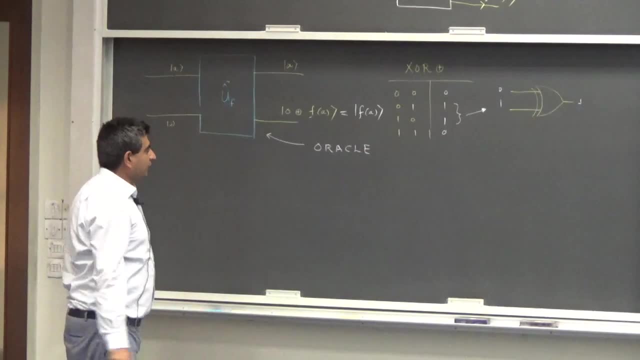 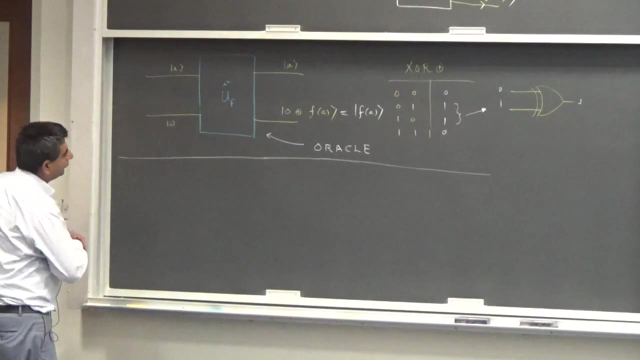 Such a black box, by the way, is called an oracle. What an oracle does is I'll explain what the oracle does. it's a quantum oracle. so let me get a bit further in this description. Suppose I do the following: I have two inputs, two qubits. 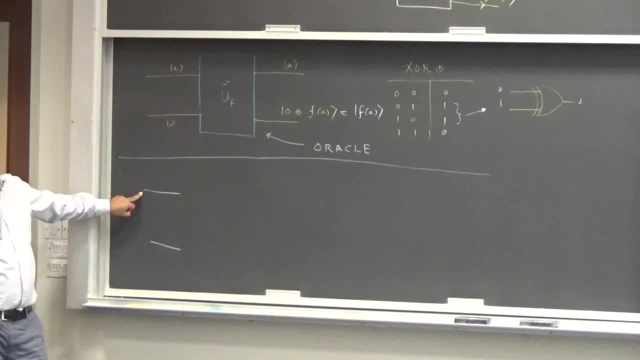 Okay, One is my working register. my bit is encoded on the first channel and I put this in a quantum state- cat 0 or cat 1- and I initialize this as cat 0 and then an ancillary qubit I also initialize as cat 0, alright. 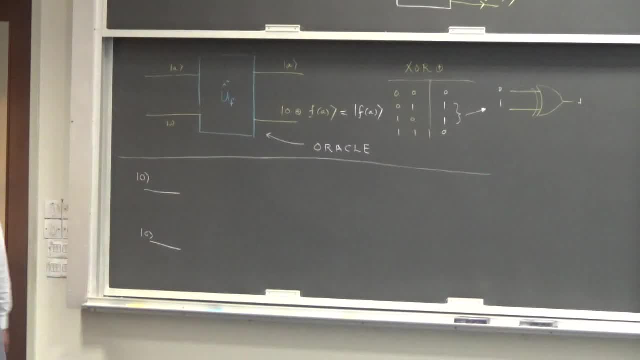 So let's see how all of this works, and then I think the ideas will be much clearer. So this is my working qubit and this is my auxiliary or ancillary qubit. I want to add this ancillary qubit because I want to encode the output, perhaps here. 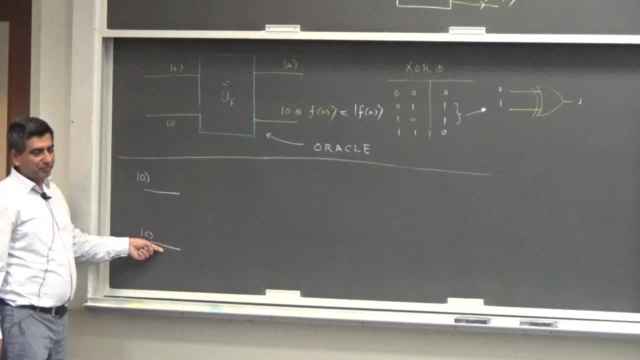 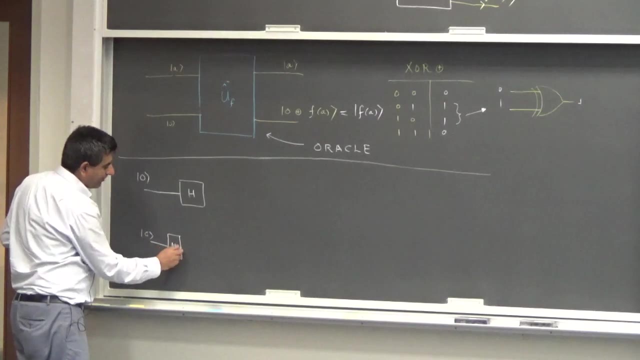 I need to have. I need to have this ancillary qubit here. So what I do now is I put a Hadamard gate here on the first qubit, and on the second qubit I put a not gate, followed by a Hadamard gate. 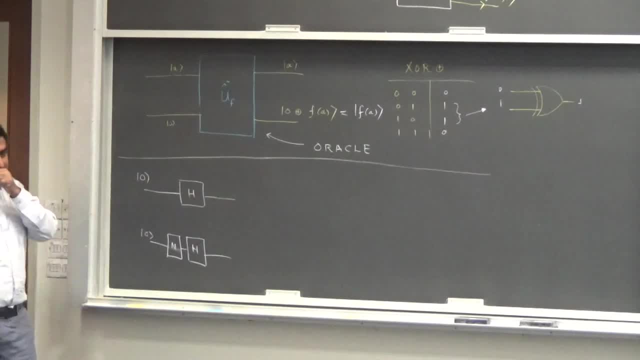 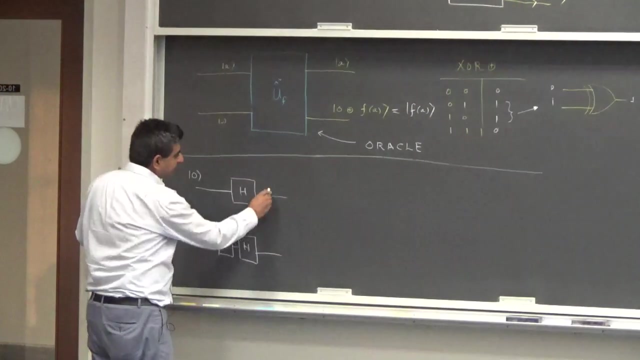 Okay, Okay, Okay. So I am going to implement the Deutsch algorithm. I am going to find out whether my function is balanced or whether it is biased, or it is biased. First of all, I need to initialize my quantum computer. So I input, with cat 0 on my working qubit and cat 0 on the ancillary qubit. 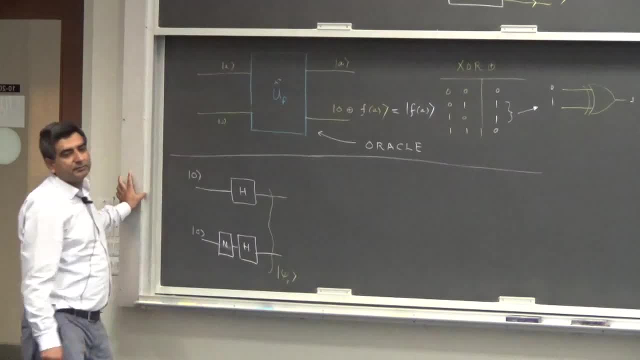 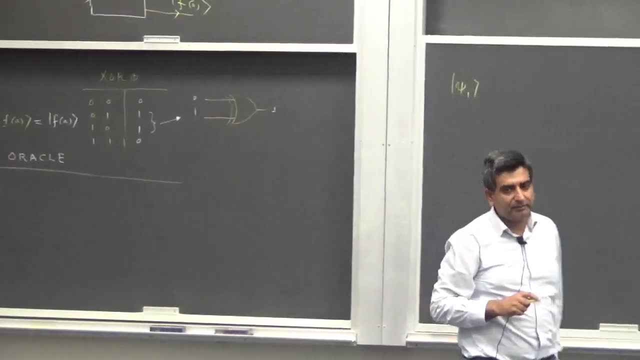 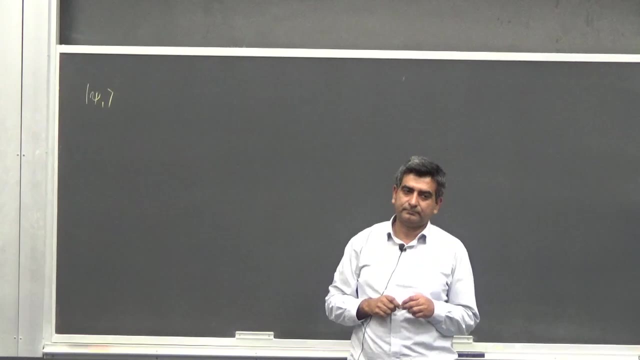 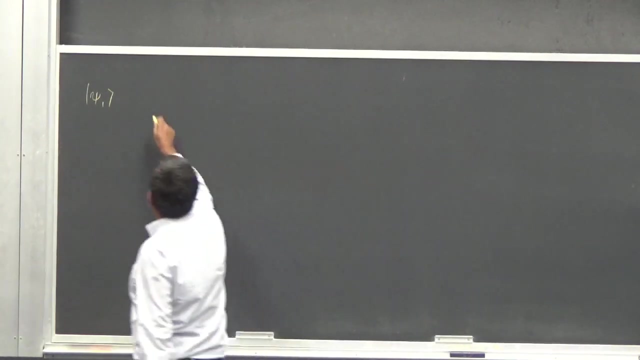 I ls denoted by psi 1.. What is this psi 1 going to look like? What is the cat representation of psi 1?? So what is the state of the first qubit after the Hadamard Right? So it is 1 over 1 over 2, cat 0 plus cat 1.. 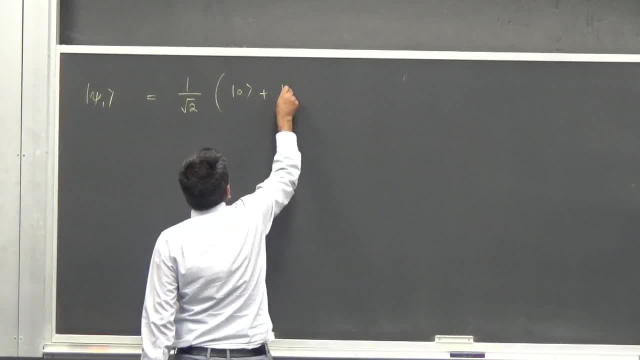 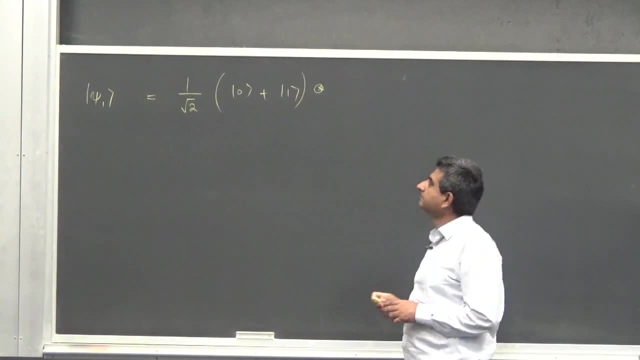 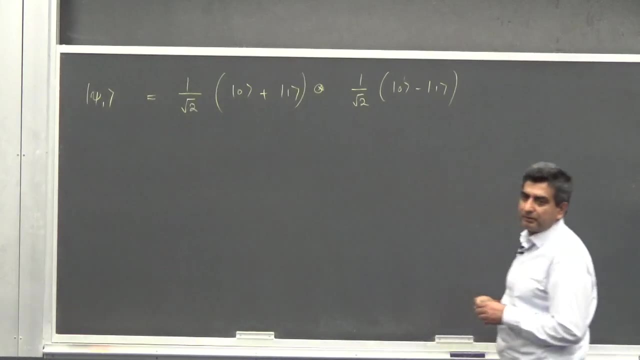 Is this the case? Yes, sir, So there is a potential. I am now adding the crates. do you see this? ket 1 and the second qubit, right 1 over under 2 ket 0 minus ket 1 right, So I can also. 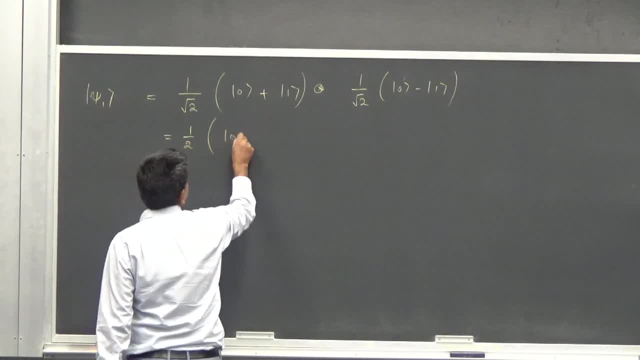 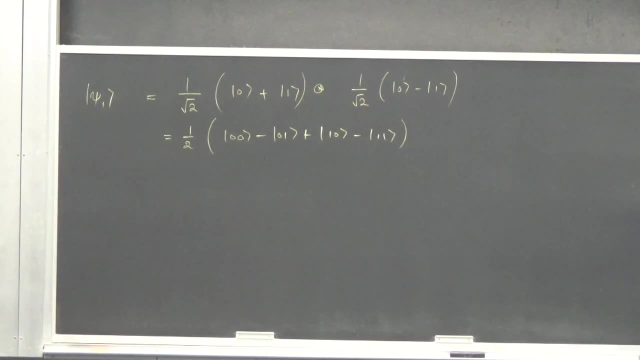 write this as: one half 0, 0 minus 0, 1 plus 1, 0 minus 1, 1.. So I created a superposition, in a sense. Now I would like to put in my oracle here. What this oracle does is that. 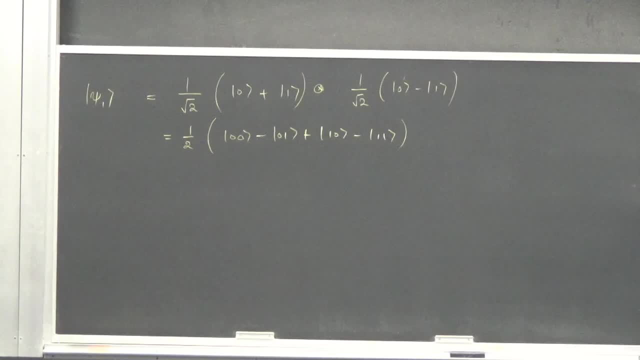 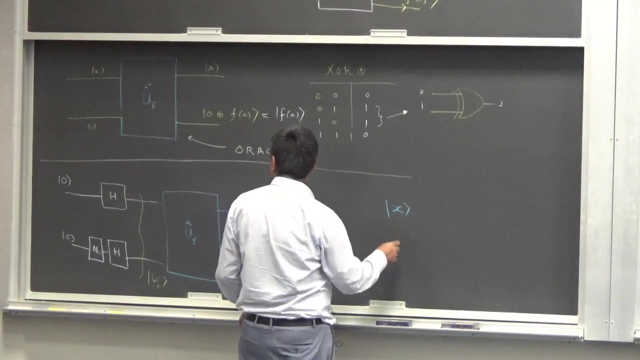 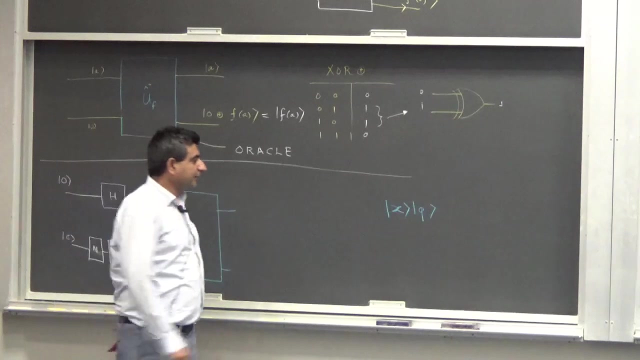 it gives the first qubit As it is. So let me describe what the oracle does. So my first qubit is in a state x, x could be 0,, 1.. The second qubit is in some state: q, q could be 0,, 1, and it is a unitary. 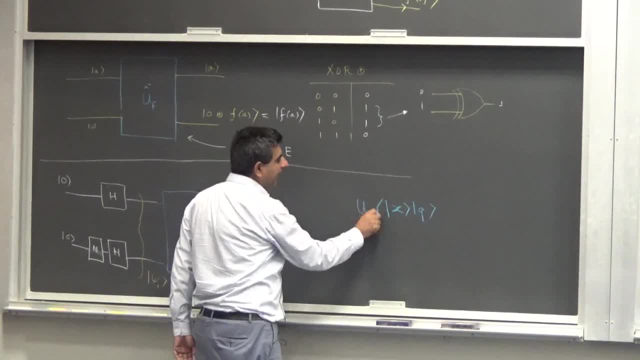 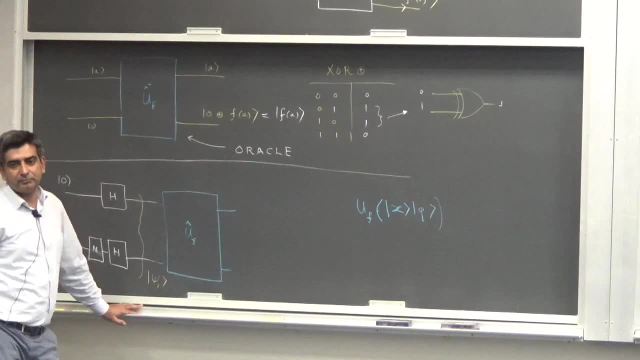 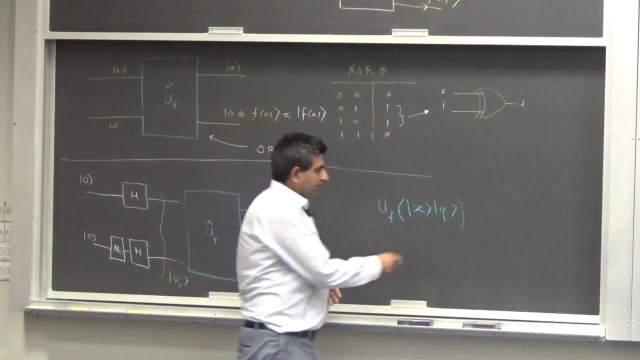 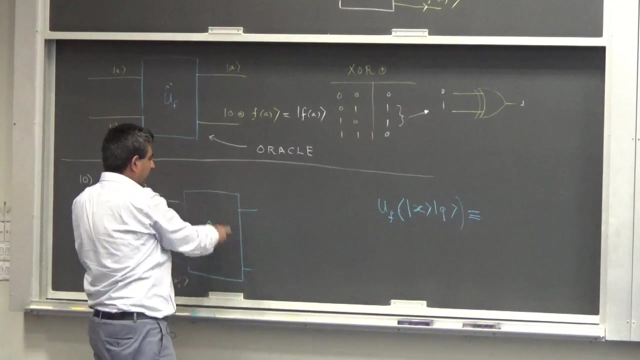 operation u f that acts on this input state. So I am defining. what does this black box do? So this is my definition. So I am putting three signs here. I have built my black box, which is called a quantum oracle, and I am 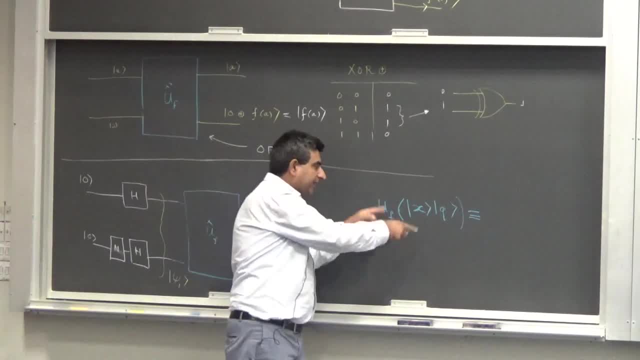 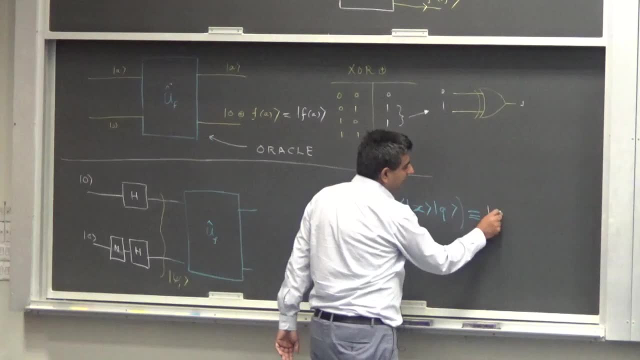 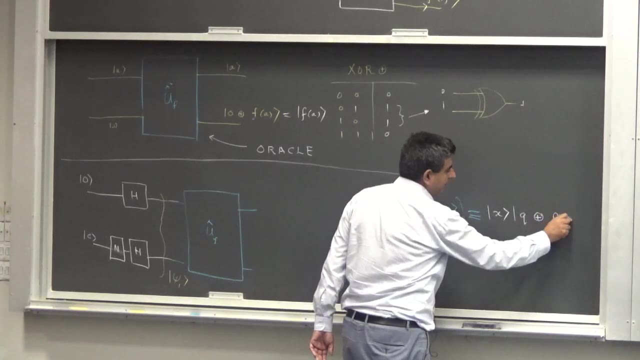 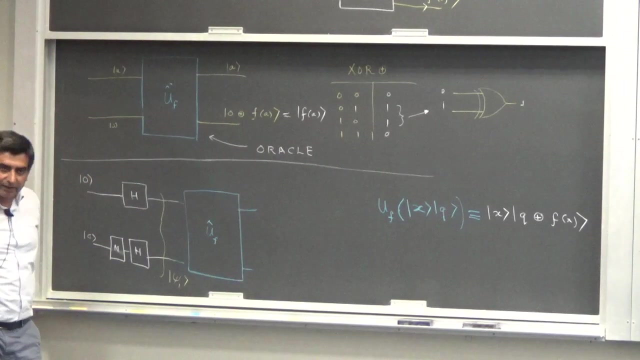 going to describe why it is called a quantum oracle, So that the action of this black box on any input state that comes in is as follows: Nothing happens to the first qubit And the second qubit acquires this form. Now I have built my unitary operator. I want to achieve this unitary operation, This 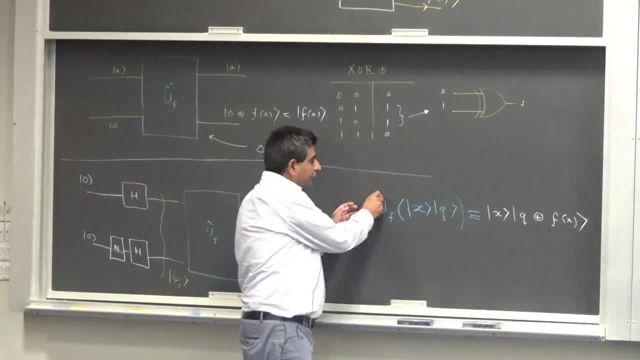 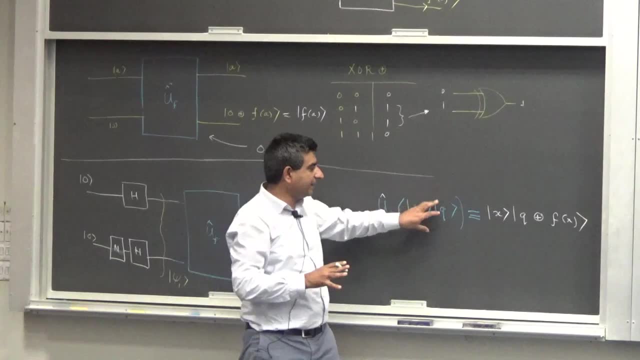 I take an input and get this. I can feed in different inputs: 0, 0, 0,, 1 1, 0. what is the general… update? So the제를pete, we have to understand that a quantum oracle. 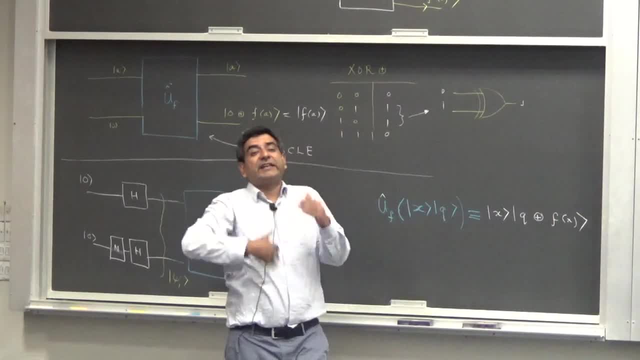 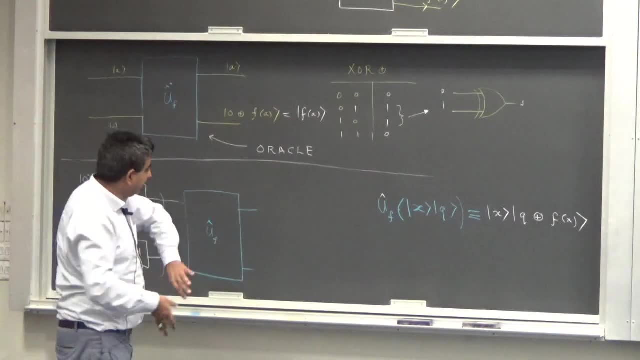 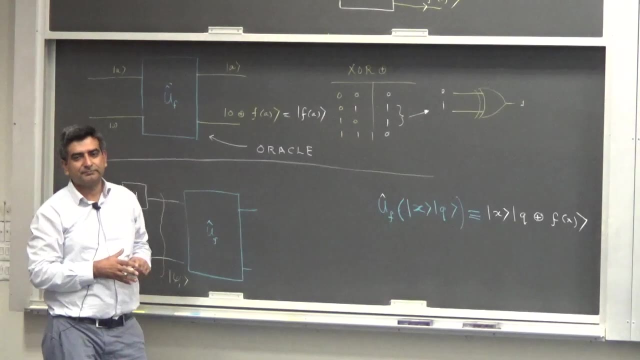 1, 1, 0 and find out what the outputs are going to be for a given F and for that given F. the task of a quantum computing engineer is to design a network of logic gates so that this task is achieved right now. why is this called a quantum oracle? a quantum oracle is a tool. 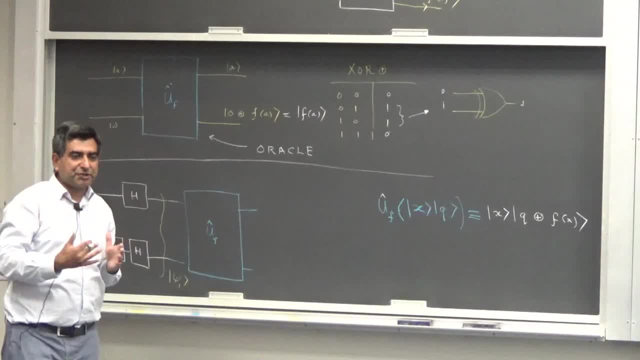 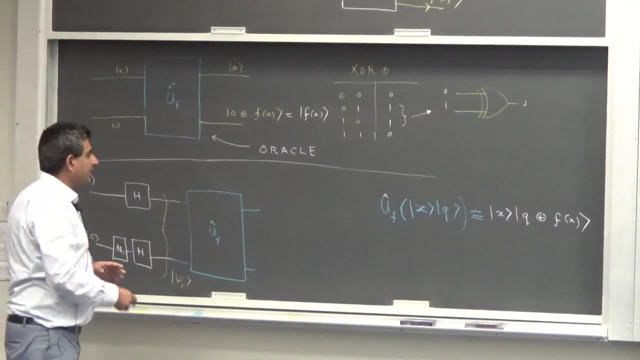 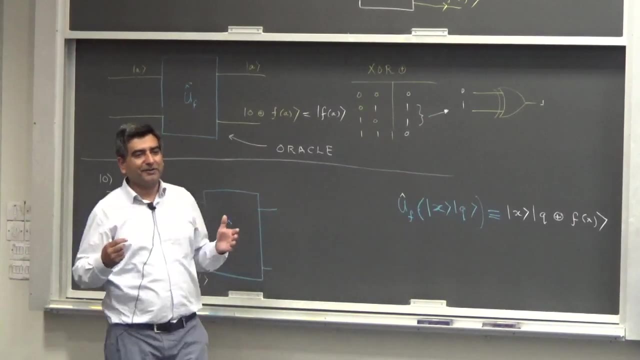 that helps you distinguish one solution from many possibilities. so, if so, it can tell you what the function is, so you and it can light up when you get a desired result. suppose you're searching something and you're searching for a particular string. if the Oracle can tell you that, 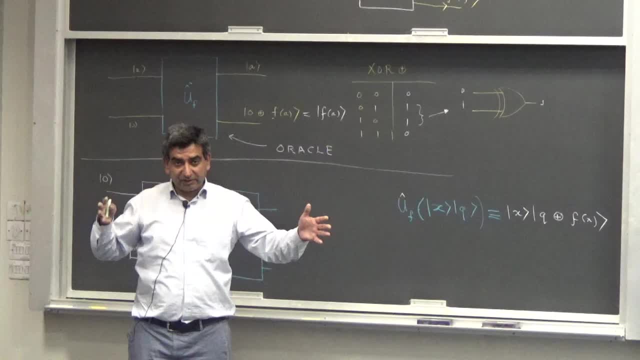 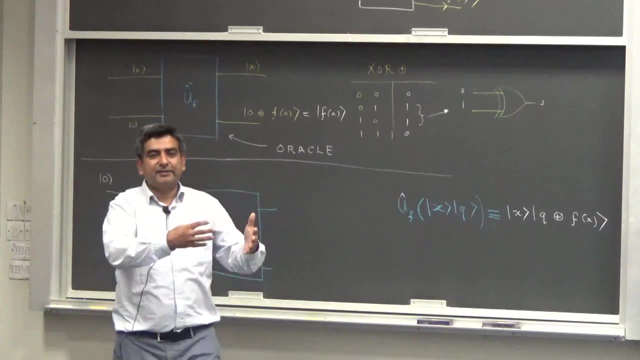 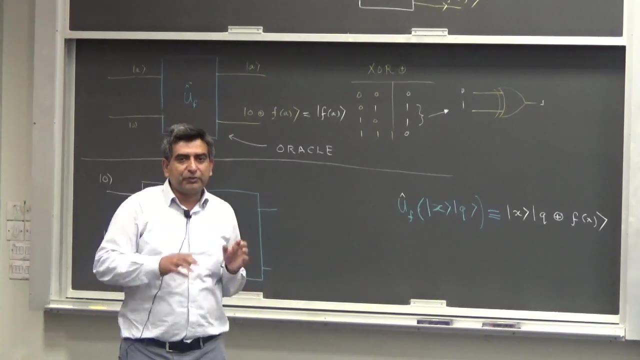 it gives you a certain output and if the search string is input, it is available to the input it. it gives you a signal that, oh yes, we found our search. so it's a. it's a tool or a machinery that helps you discern your solution from other possibilities. so if it were, if the 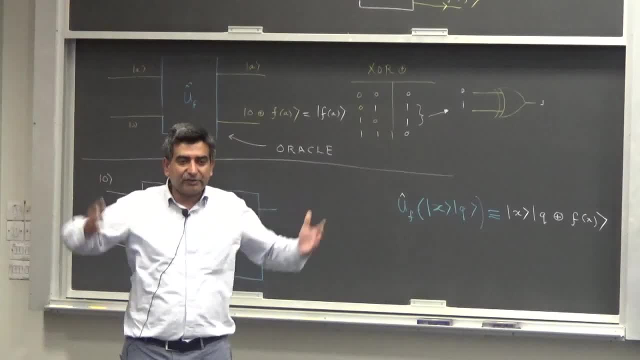 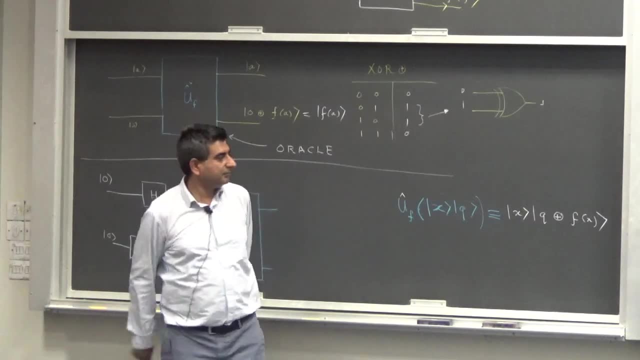 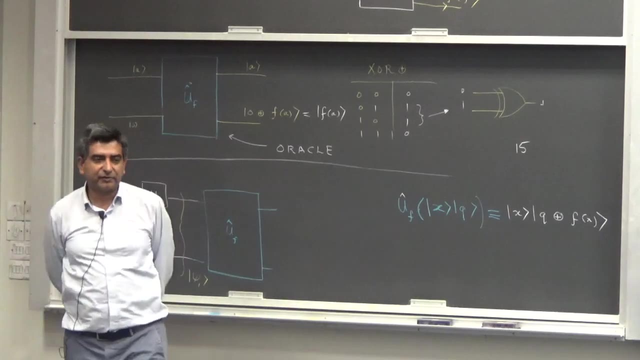 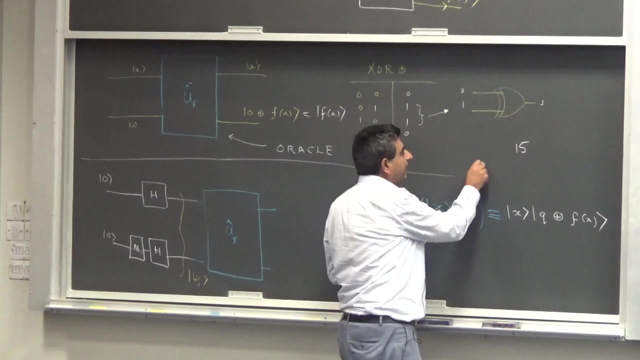 solution is found, it goes bingo. yeah, I found the solution. just imagine if you you were to factorize the number 15, so you have a number 15. one possibility is to design an algorithm that finds out the prime factors of 15. but suppose you are given it hits upon 5 and 3 in. 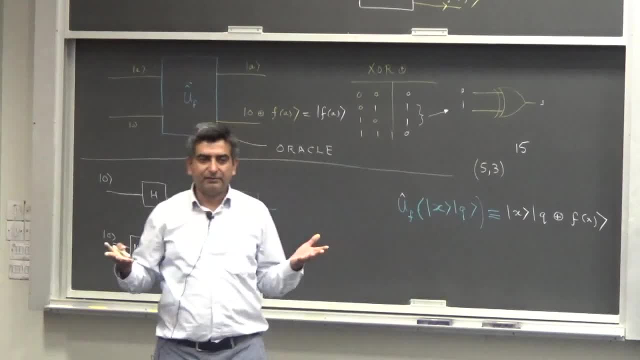 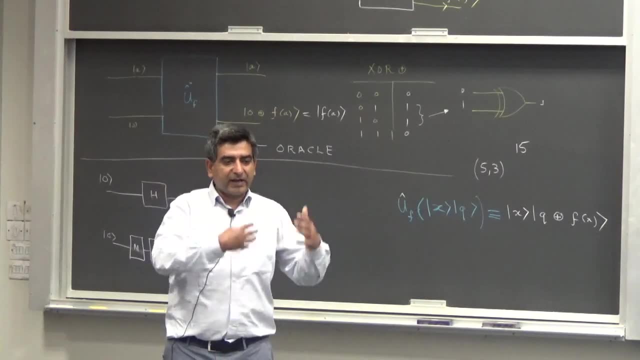 its, in its input space, it, the Oracle, can tell: yes, 5 and 3 have been found, they work as prime factor pair and they work as prime factor pair, and they work as prime factor pair and they work as prime factor pair of 15. so the Oracle tells you that five and three is the solution. if you find 4 and 4 and 4 and 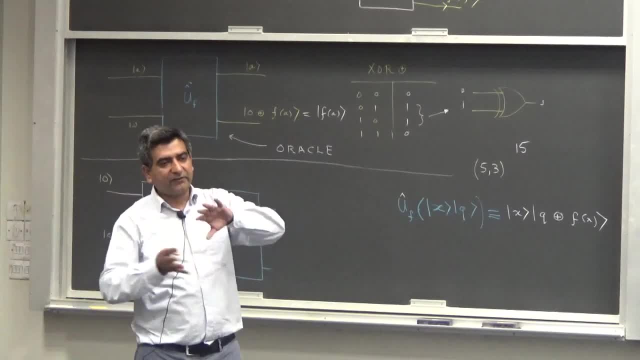 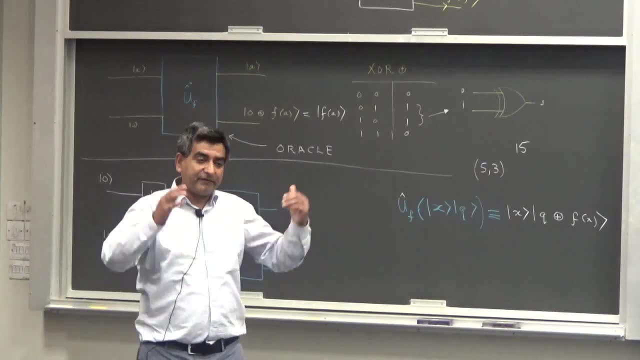 4, it's not a solution. so if the Oracle is fed with four and four, it can tell you: no, this is not the solution. but if it is fed in in five and three, it can declare that, yes, I found the solution. that's what the quantum protocol does. but it has to be pre-designed. so the Oracle is three design. so 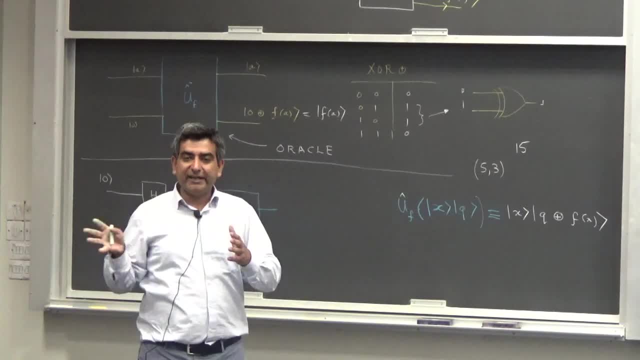 that it can look for the prime time, if it can test whether the input function is allowed to be perfect, and all that you can do is you can attempt, because the questions, that is the one- claw modules, principles and drop in the complex matter which is the code on how the output question. 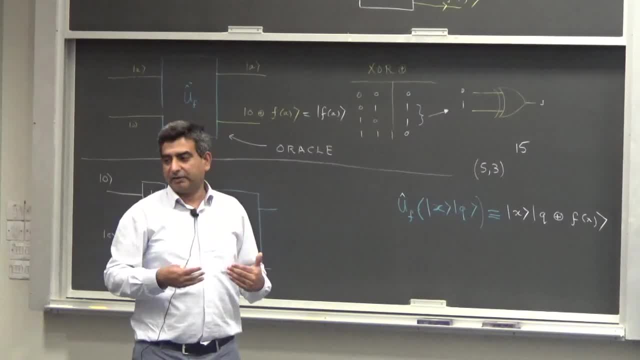 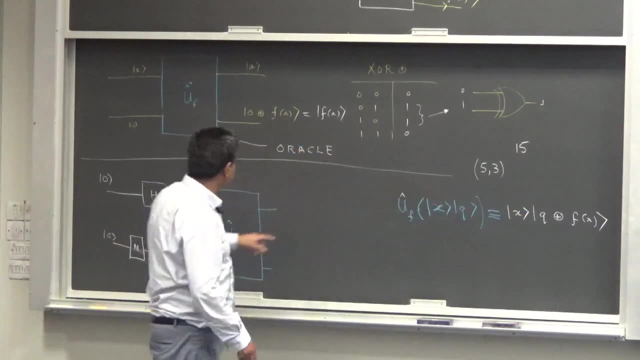 is observed. create, stop and write right and put the any type of question- that is what I do in my- are prime factors of the number 15. That's what the oracle does. So now we have this unitary operation. This unitary operation has to be built into this uf. Now you can. 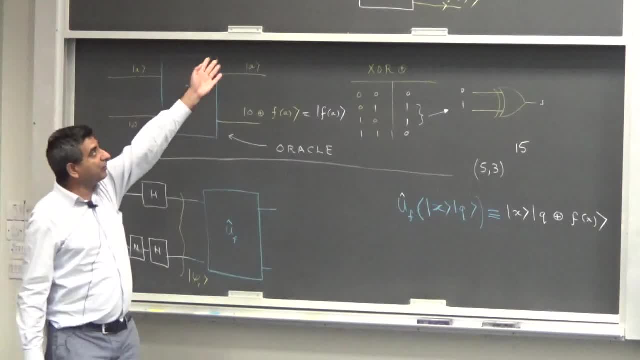 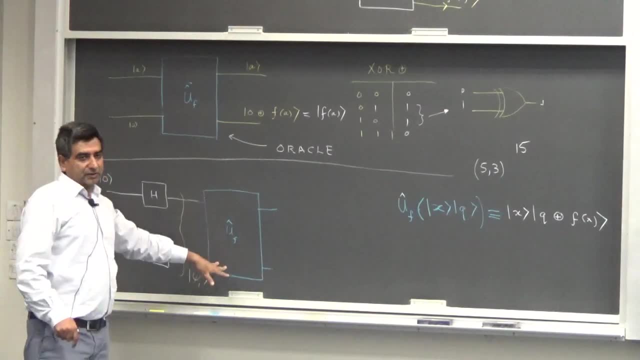 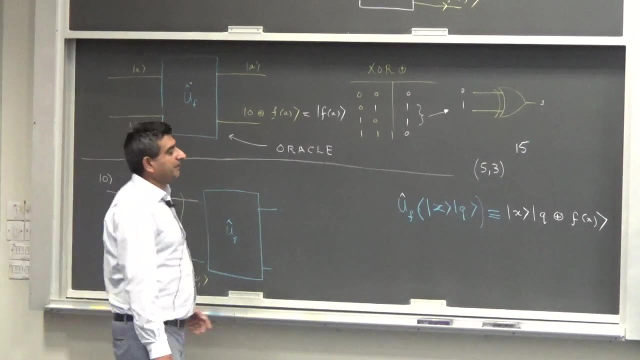 do this as a homework- that if I have any one of the four possible function sequences, what kind of quantum logic gates do I need to build this oracle? Yes, Sir, what does f of x mean? f of x means f of 0 or f of 1.. 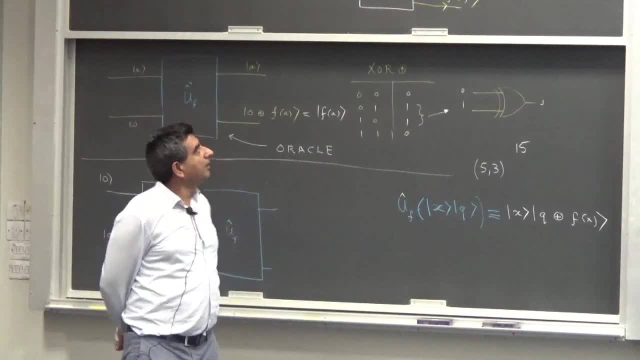 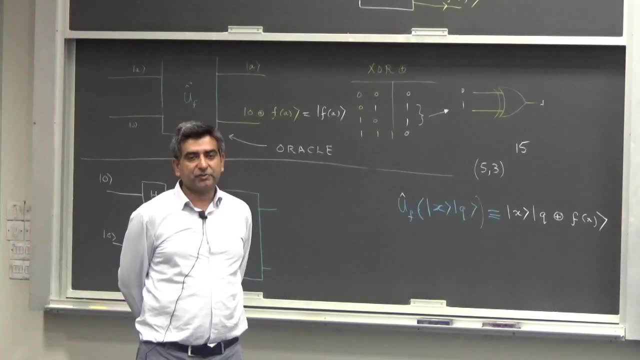 So do we know the form that f of x has? So we do not know the form, but we would like to distinguish and tell whether f is balanced or biased. So there is some f and it is either balanced or biased. So this: 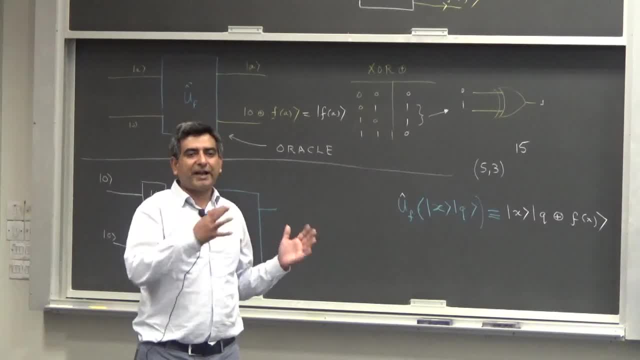 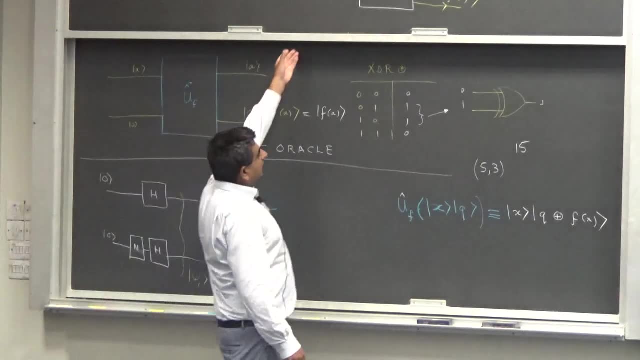 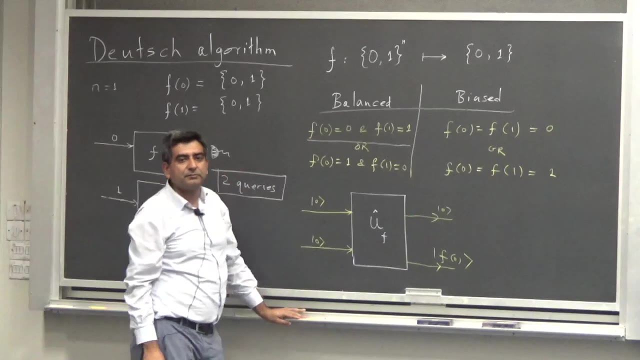 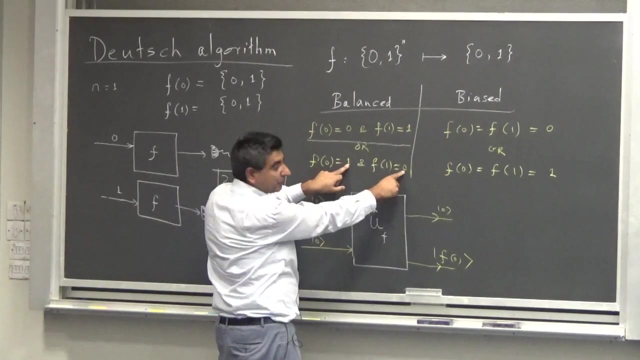 algorithm discerns which kind of function it is. Sir, that function is biased or not. So, screen, So balanced function is that gives me two different outputs for two different inputs: 0 and 1, 2 distinct outputs for 2 distinct inputs: 1 and 0,. 0 and 1 for 2 distinct. 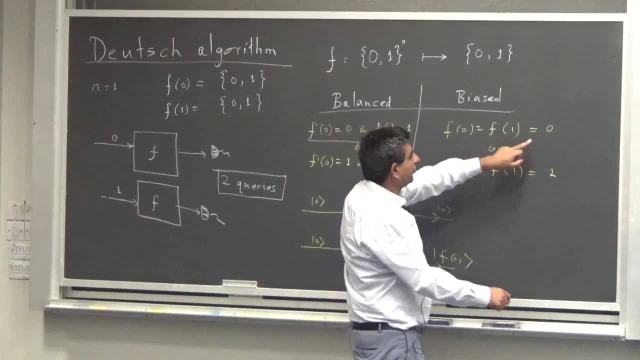 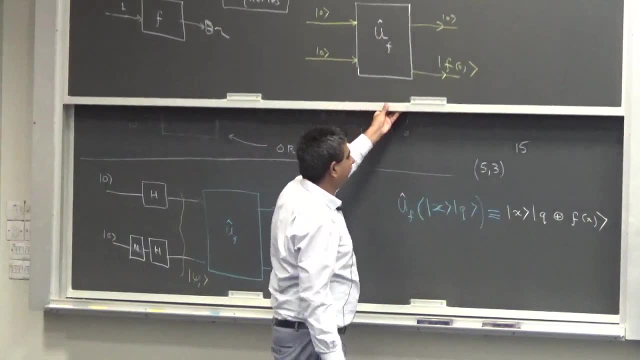 inputs. However, a biased or unbalanced actuallly gives the same output, no matter what the input is. Alright, So this unitary operator is to be build into a little captures respect. some of these parameters are not temperature in decision. Okay. So all right, I'll see you in the next class. 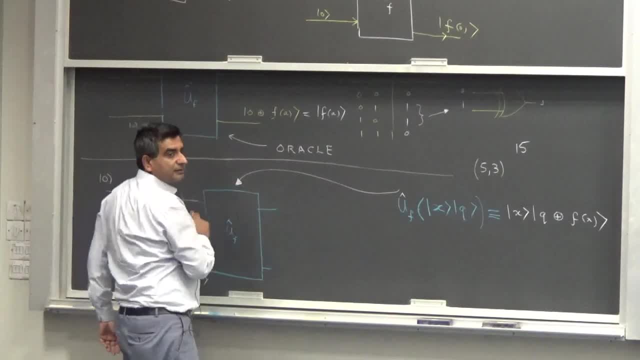 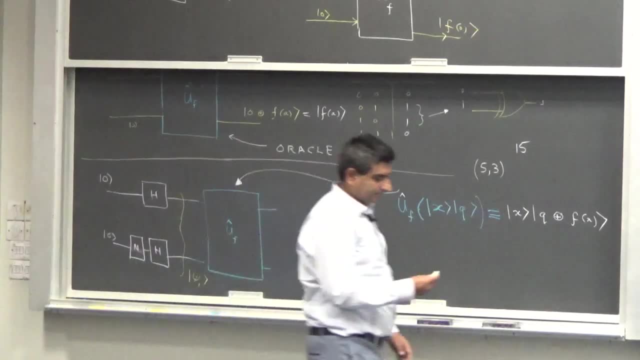 is to be built into this oracle. So what is going to happen to the output here? So this is my psi 1, what is my psi 2 going to be, Which is the oracle acting on psi 1.. So 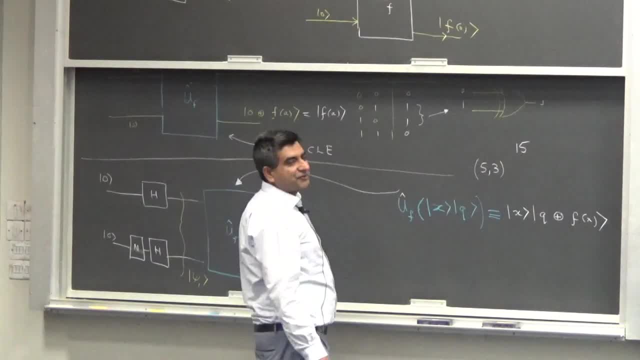 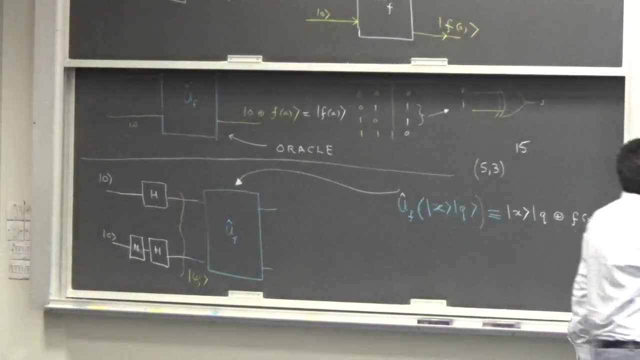 you can use this argument here. So let us try to do this. Do you understand what is meant by oracle? Let us complete the argument and let us revisit the idea of an oracle. So what this does is one half put a big bracket, So nothing happens to the first qubit and 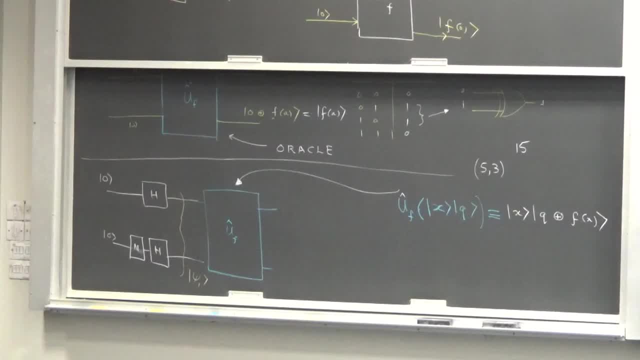 I take the exclusive OR of the second qubit with the action of f on the first qubit, So 0 plus exclusive OR of 0, right, This is what the unitary operator does. Yes, Yes, This is what the oracle does. So I am just translating this into here with specific inputs. 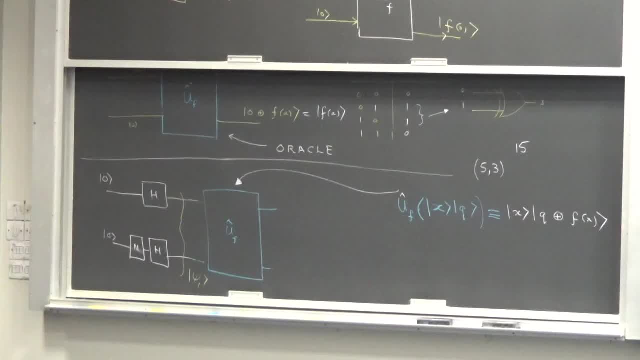 So if x is 0 and q is 0, I get x here and q exclusive, OR with f acting on this qubit. Yes, sir, So x is going to become first qubit or second qubit. First qubit. 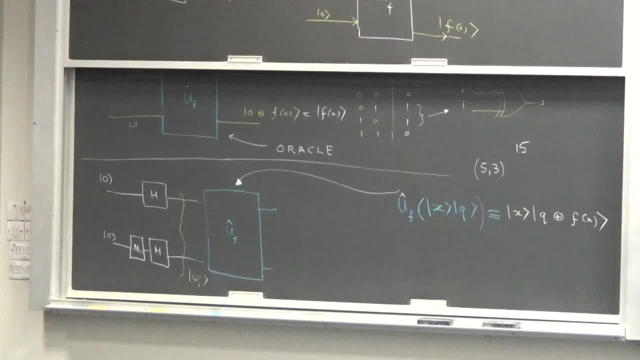 So on the first qubit or the second qubit. So I am just mapping this. So unitary function act. this is my first qubit, this is my second qubit. The first qubit remains unchanged and the second qubit you take the exclusive OR. 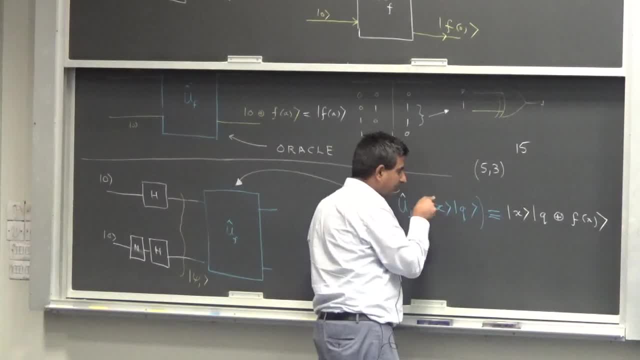 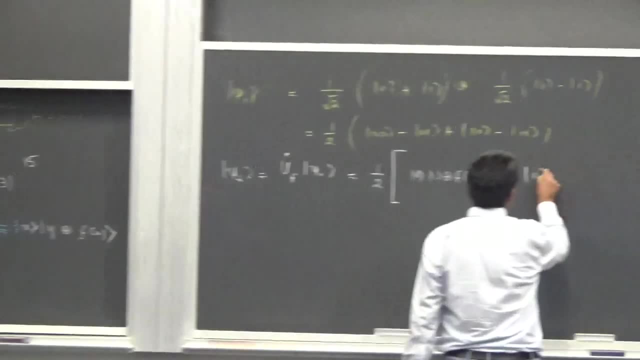 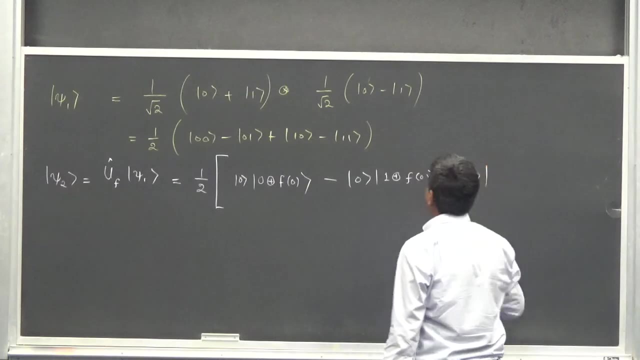 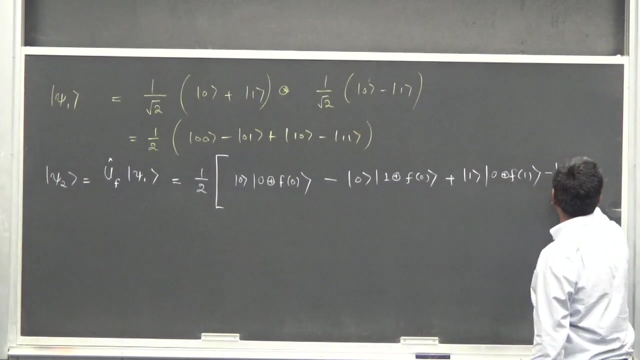 of the state of the second qubit with function acting on this label here: Minus 0, one exclusive, OR with f acting on 0. Plus 1. 0 plus exclusive, OR f acting on 1, minus 1, correct. 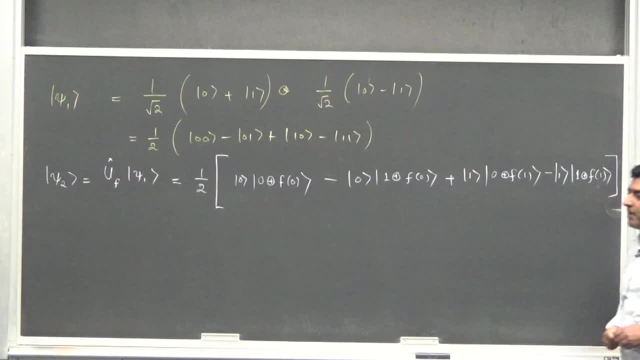 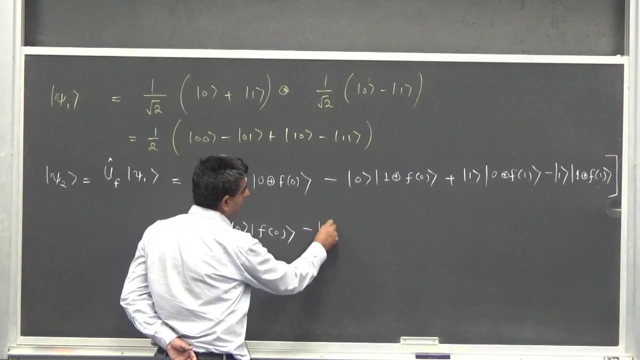 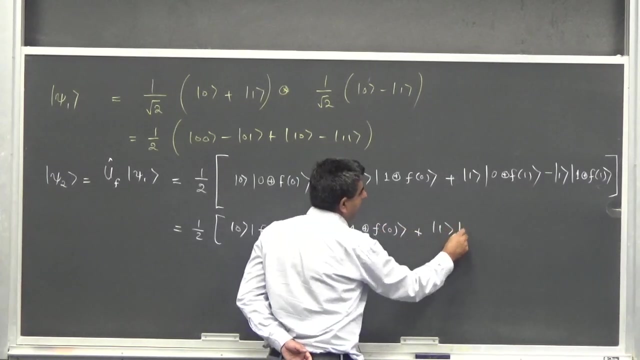 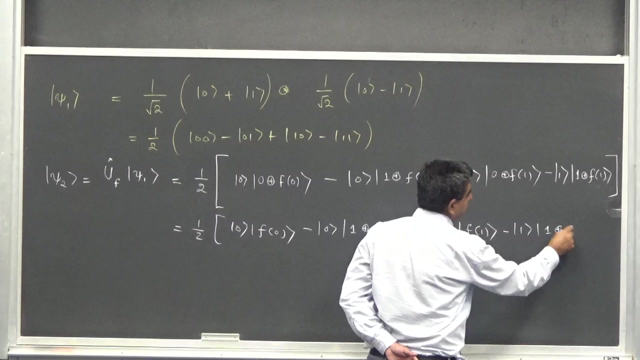 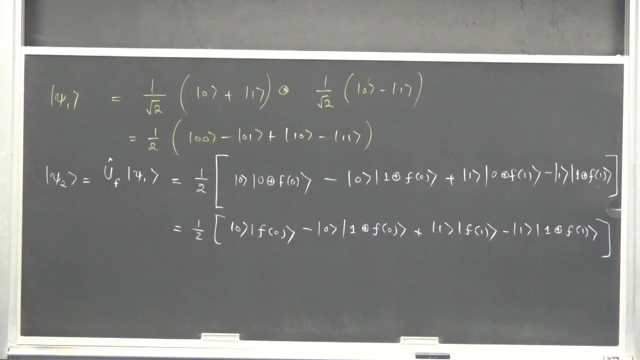 So I just simplify this Exclusive OR of 0 with anything is just the second thing, right? Minus, Minus, Minus, Minus. So this is a state that we achieved over here. Yes, Right, so I still don't know what is F0 and F1, the four possibilities for F0 and F1. 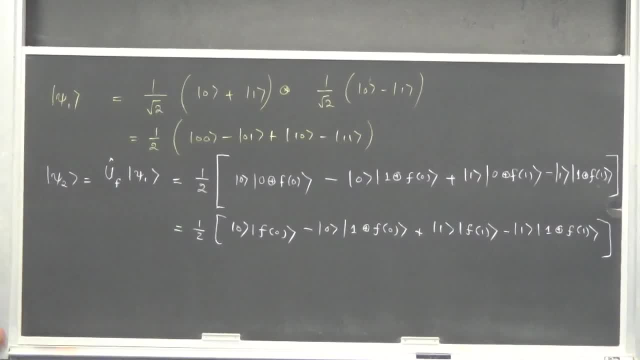 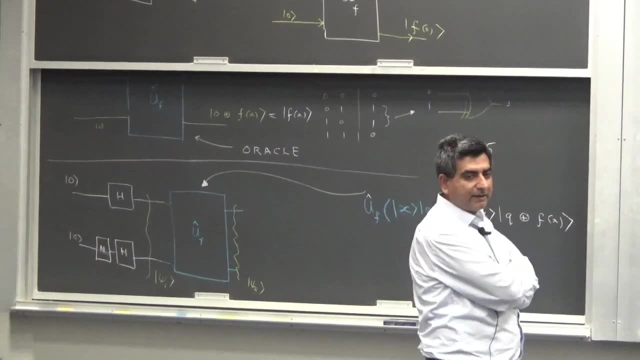 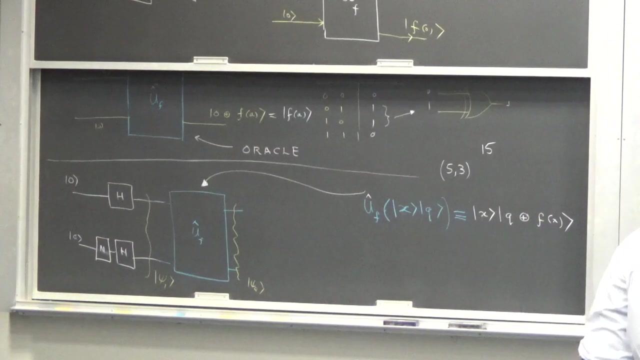 So what should the next step be? No, no, I don't want to assume anything at the moment. So what I would now like to do is… Okay, Okay At 0, F of 0 minus 1 F of 0 plus F1.. 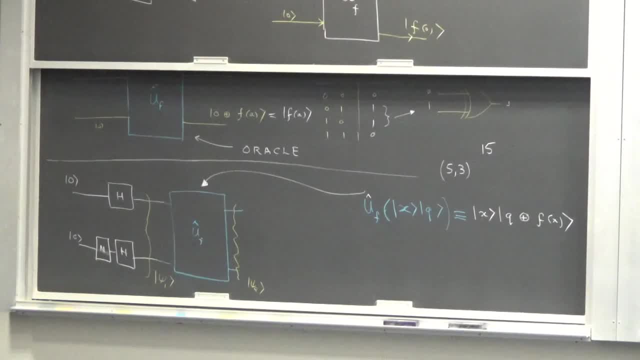 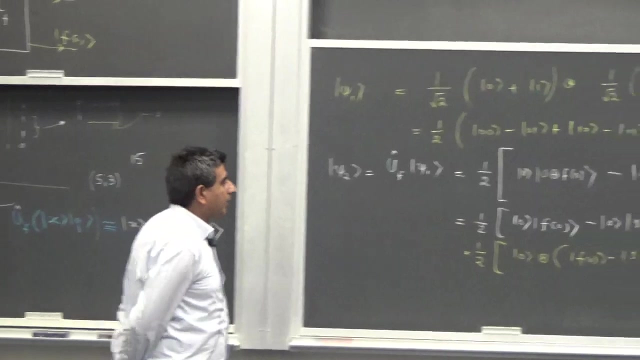 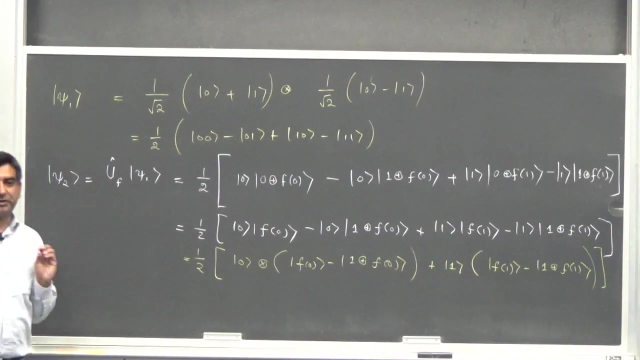 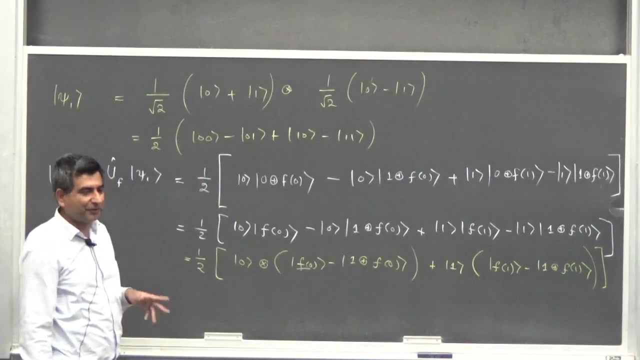 All right. So now things are getting a bit clearer. Can you tell what… What's going to happen if the function is balanced? If the function is balanced, this output F of 0,. if this is 0, suppose this were 0. 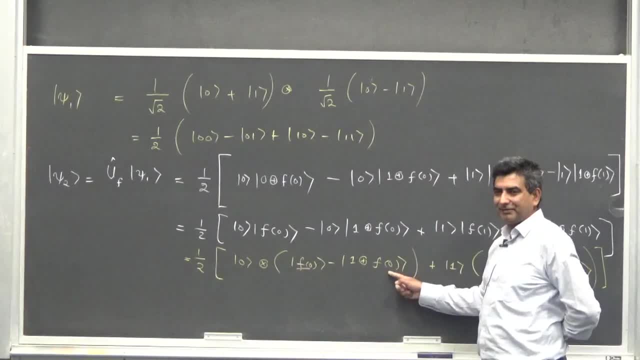 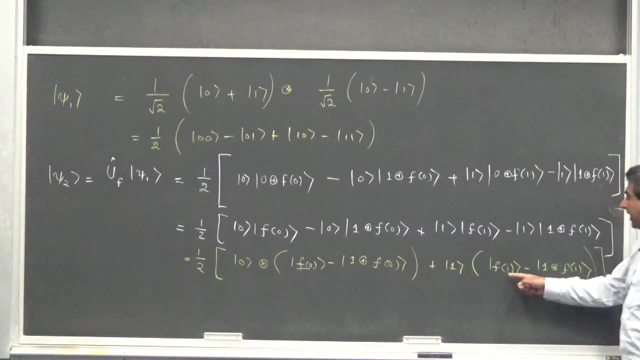 If this were 0, this would be 1.. Right And 1 exclusive odd with 1 is 0.. Okay, So here if I have. If this were F of 0… Sorry, if this were balanced then this would be 1.. 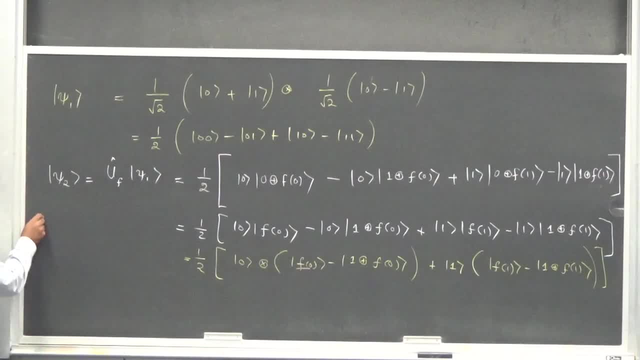 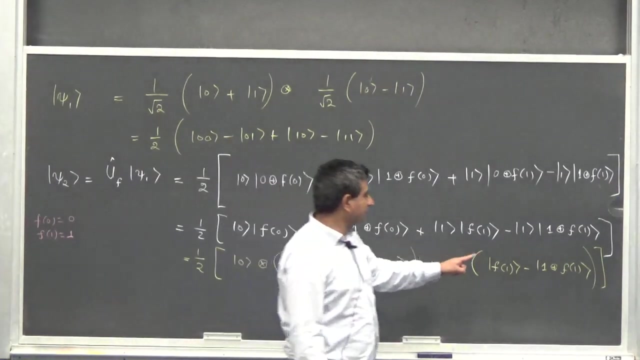 1.. So possibilities is: F of 0 is 0.. F of 1 is 1.. All right, All right, All right, Okay, Any other questions? All right, So this will be 0,, this would be 1, then this would be 1 and this would be 0. 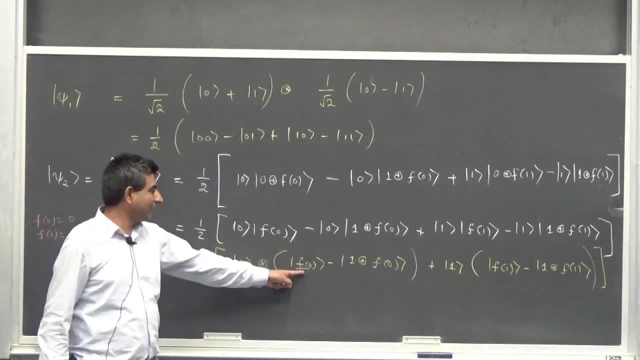 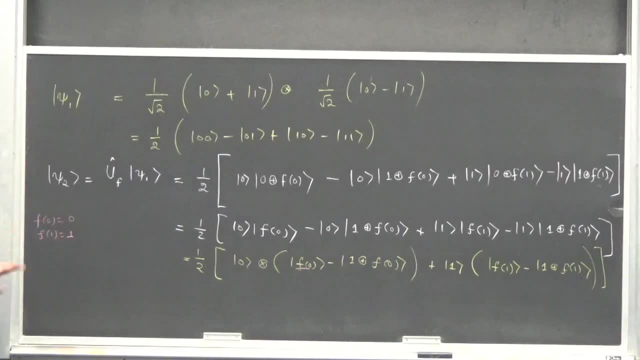 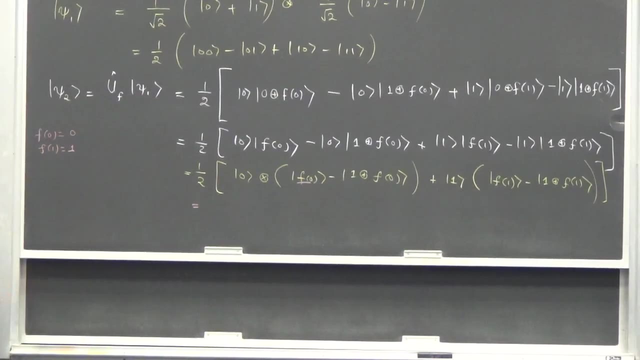 The other possibility is that this is 1,. if this is 1,, this is 1, this would be 0. So can you determine a form which is consistent by determining whether the function is balanced or biased? So if I put one half here, this is ket 0, if f is so, what is this thing equal to? 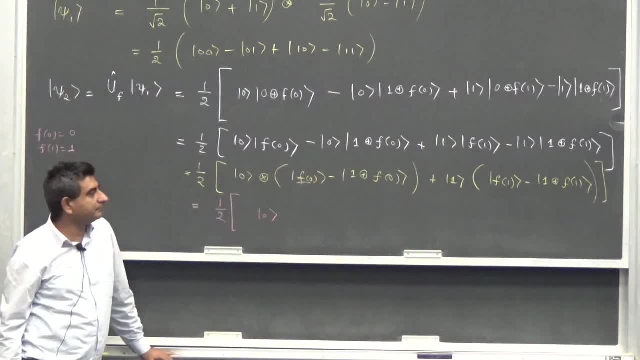 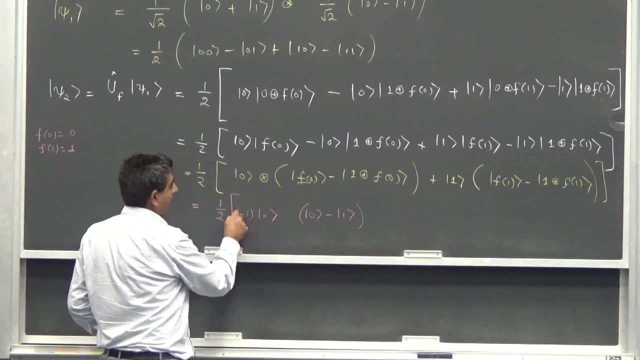 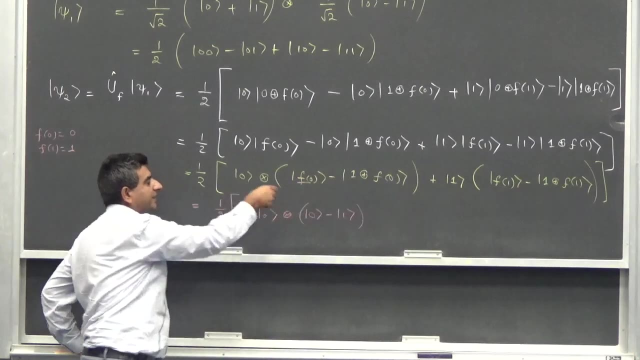 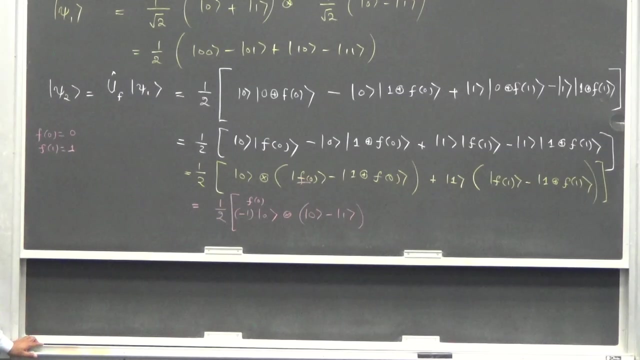 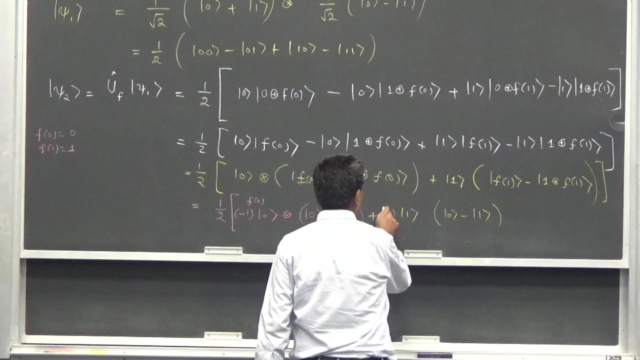 Can I come up with a general formula? Can I come up with a general formula for this? Can I write this two qubit state in this form: Right plus ket 1, this will be minus 1 raised to the power f acting on 1.. 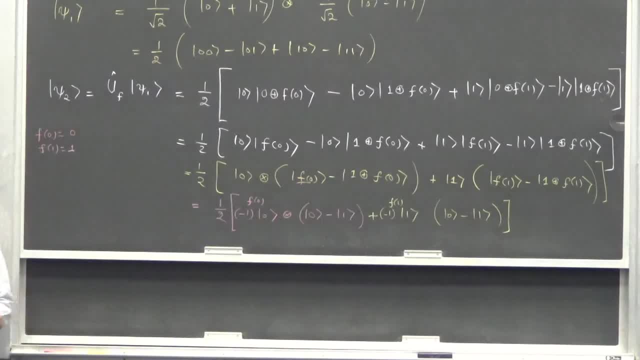 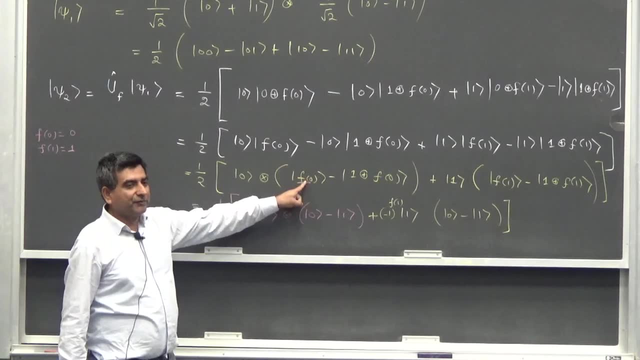 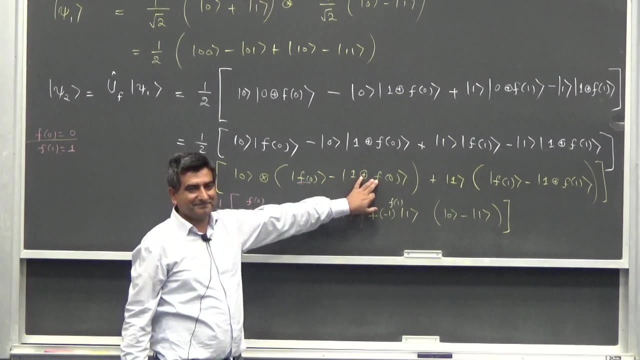 So what is happening here? This function could be 0. If suppose f of 0 is 0, this thing Right. So this is f of 0 here. this is ket 0 minus ket 1.. Ket 0 minus ket 1, with a plus sign, that is minus 1, raised to the power f of 0. 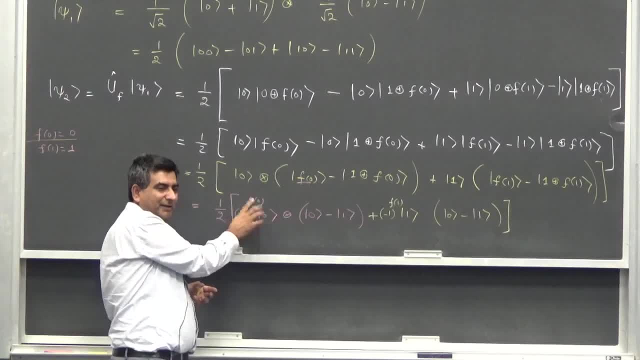 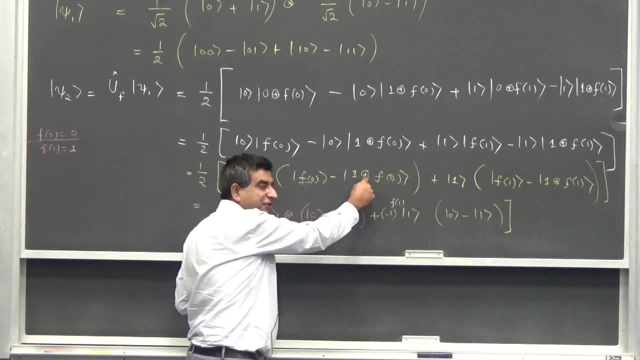 f of 0 is 0, minus 1. raised to the power, 0 is 1.. However, if f of 0 is 1, then you get a 1 here and 1 exclusive. all with 1 is addition. modulo 2, gives you a 0 here. 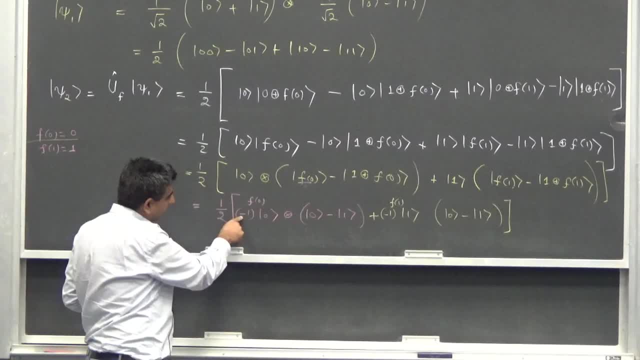 So it is the same thing with the negative sign. That is why I put minus 1 raised to the power f of 0 here. If f of 0 is 1, that is minus 1 raised to the power f of 0.. 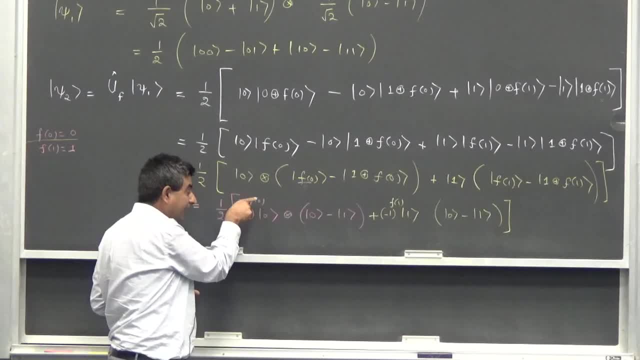 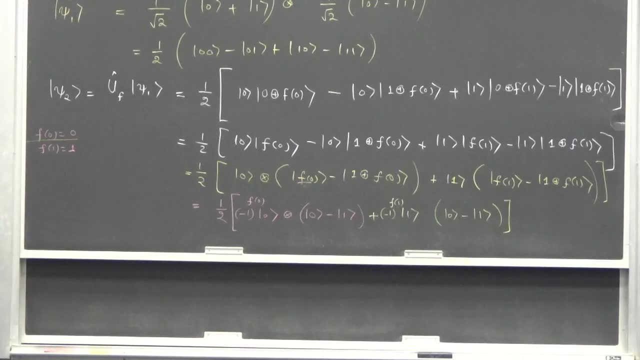 So I put minus 1, raised to the power f of 0. here, 0 is minus, it is minus is 1. this would be minus 1 is for one, which gives a negative sign. so everything is working here. yes, which which? so right now there is no great balance or biased, it's just so. what what I'm? 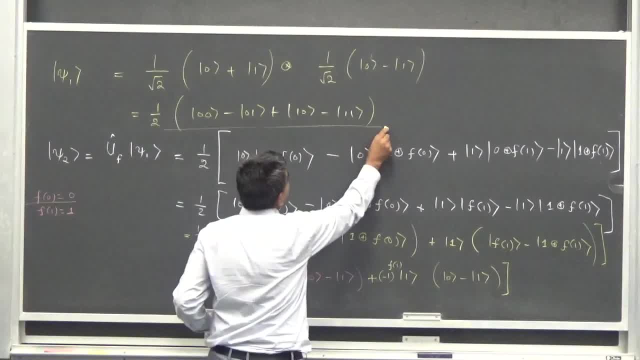 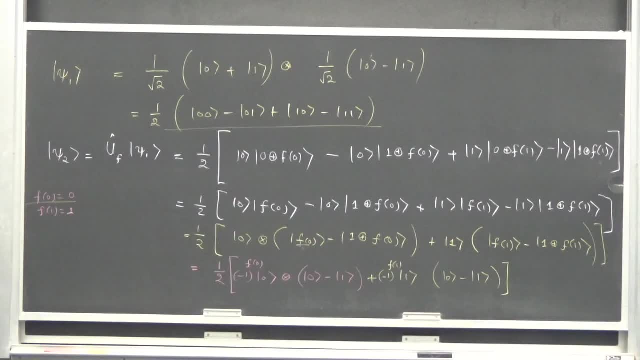 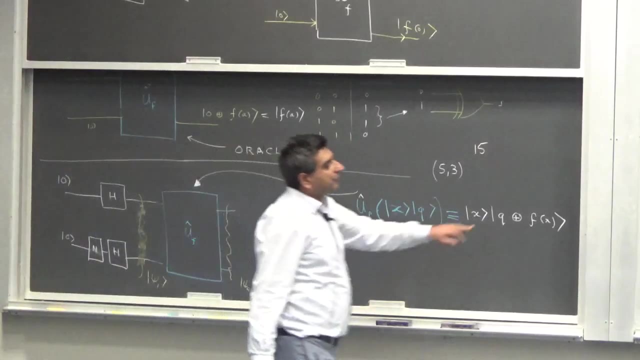 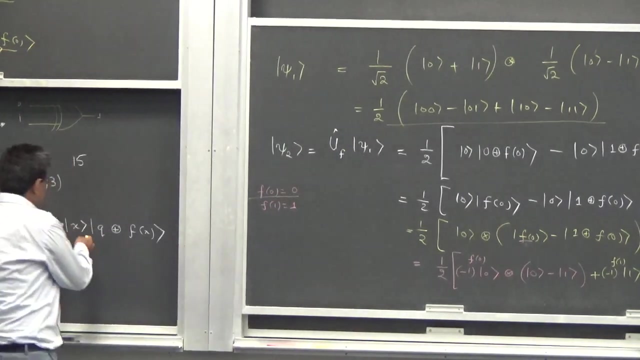 doing here. this is my input state. this is a state that we have achieved at this point in time. now we apply this function, this Oracle, this Oracle is applied to this input state and I get an output state. now I would like to determine what the output state is after the Oracle. so I'm just taking this recipe and plugging. 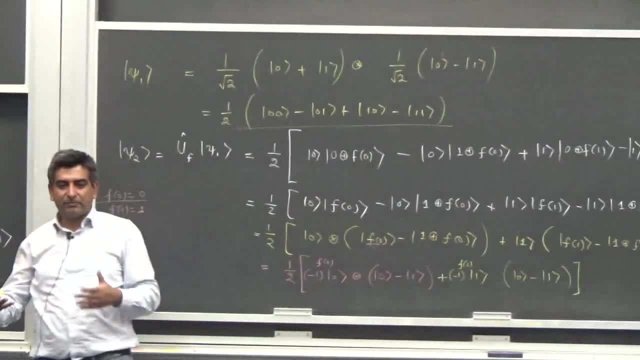 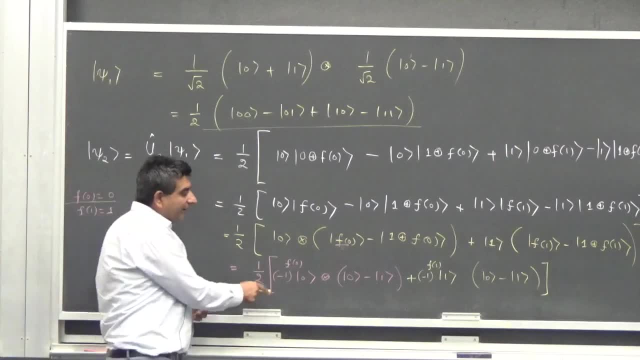 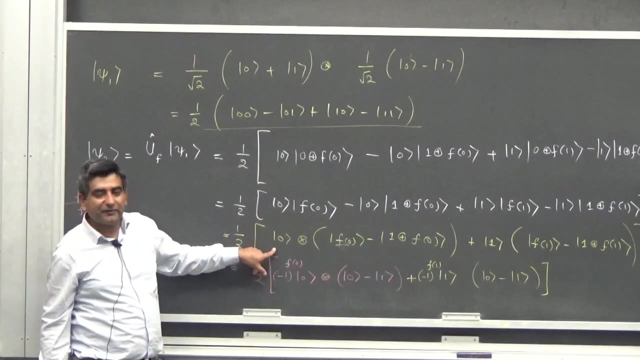 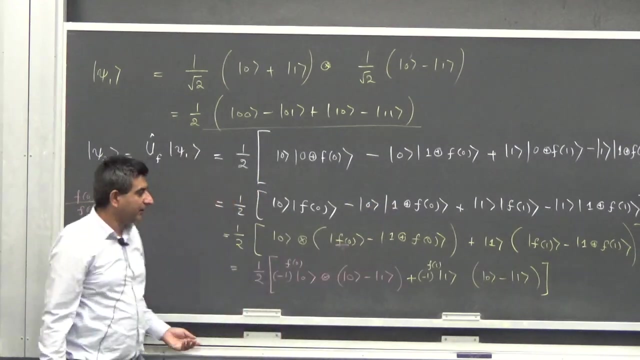 it in here. so there's no, no, no concept of balanced and constant as yet. now what I would like to do. so do you understand this final step? no, so do you understand this step? so I have just factorized out the first qubit, cat 0, here, and written these two qubits, the second qubit, together. now the possibilities. 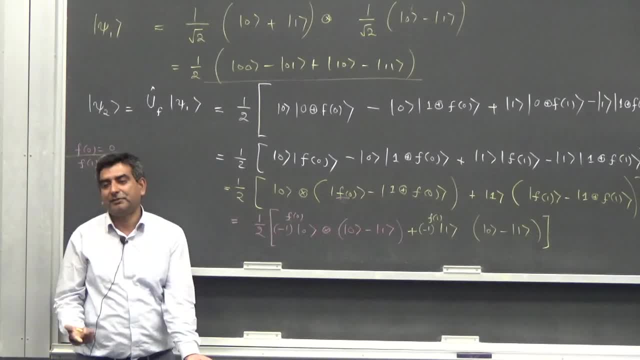 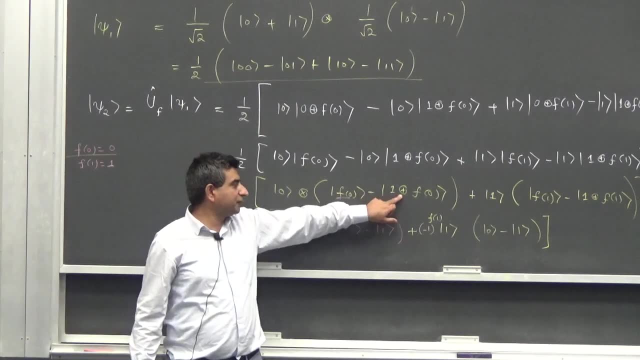 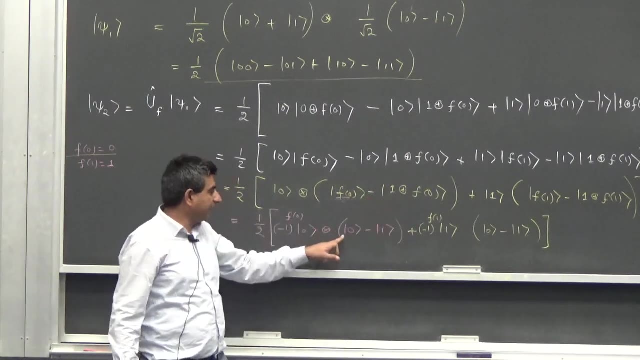 this function of 0 could be 0 or it could be 1. if it were 0, then this would be cat 0. what would this be? 1 exclusive or with 0, which is 1, so 0 minus 1 cat 0 minus cat 1 cat 0. 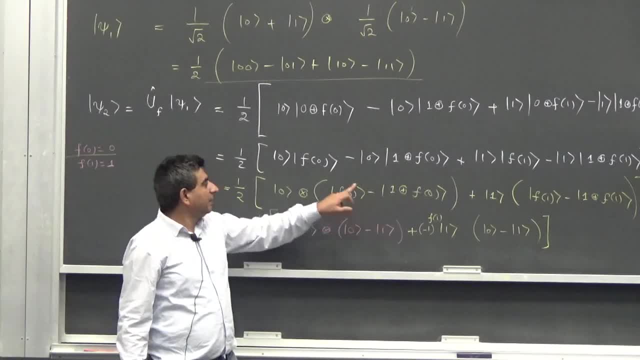 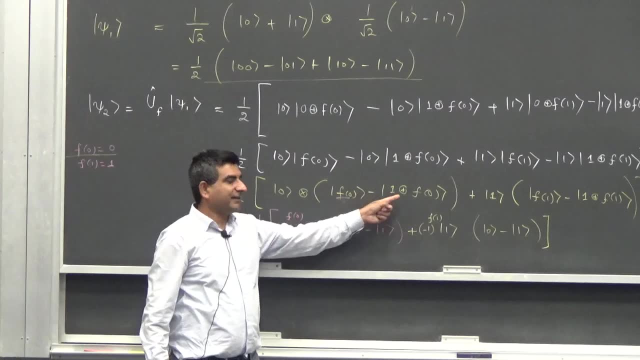 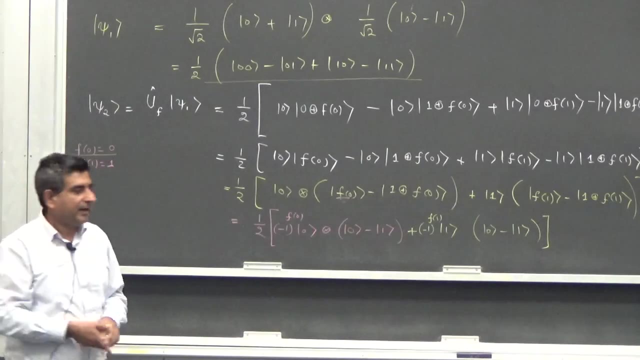 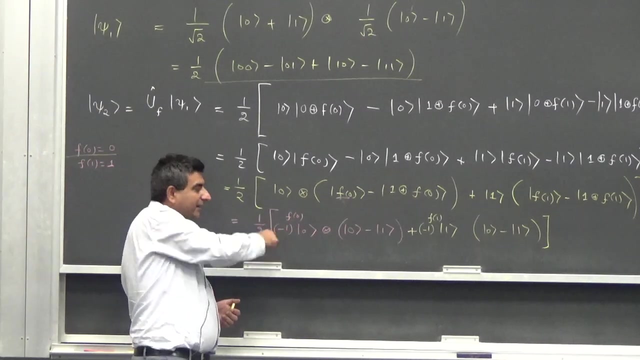 minus cat 1. right, if this were 1, then this would be cat 1 minus cat 0, which is cat 1 minus cat 1. this is just the inverse of this. now, how do I take into account this inversion? I just put in a minus sign where needed. now that minus sign where needed is incorporated. 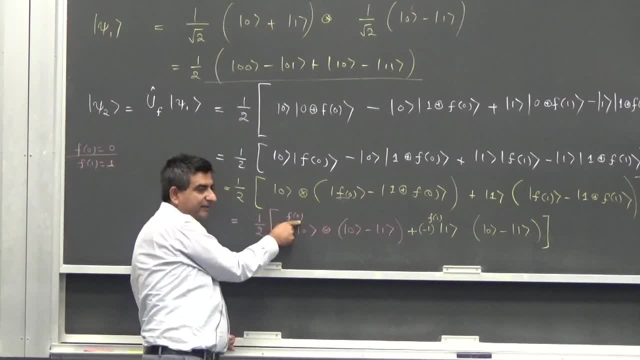 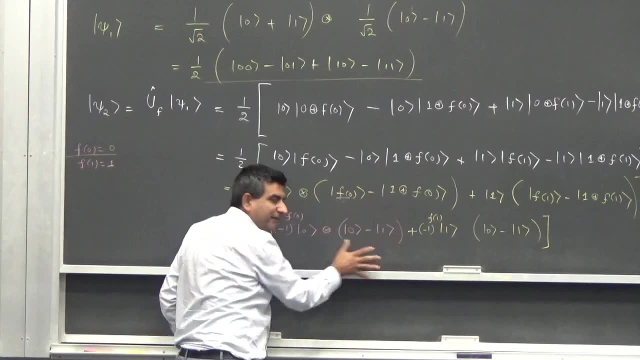 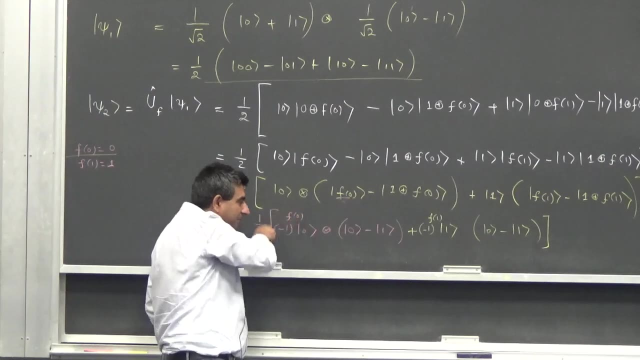 by this minus 1 raise to power f of 0. if this factor is 0, then minus 1 is for 0, just gives me 1, so I am left with this being positive. however, if this takes the form minus form, 1.. This is minus 1 is for 1, so it imparts a negative sign to this. so all of this is inverted. so 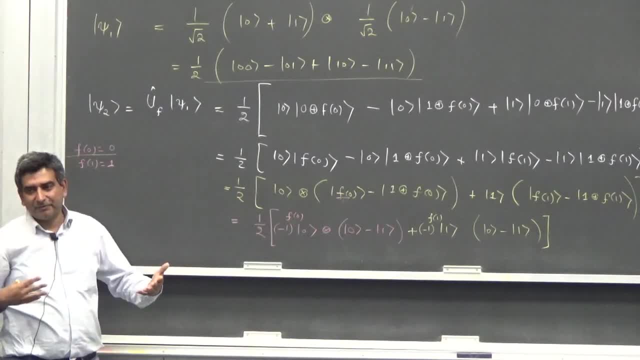 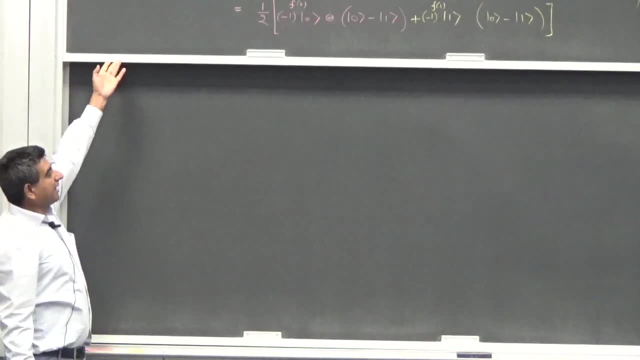 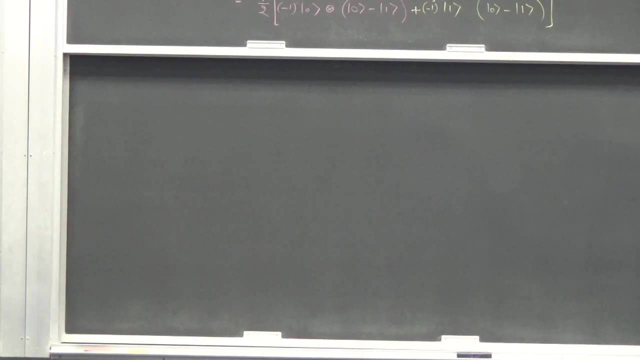 this is the proper way of writing this state cycle. now, what is your guess? how would I like to do a measurement? how would I like to tell whether my output is balanced or is it constant, biased? any guesses? so what I could do. what if I put a Hadamard gate here? 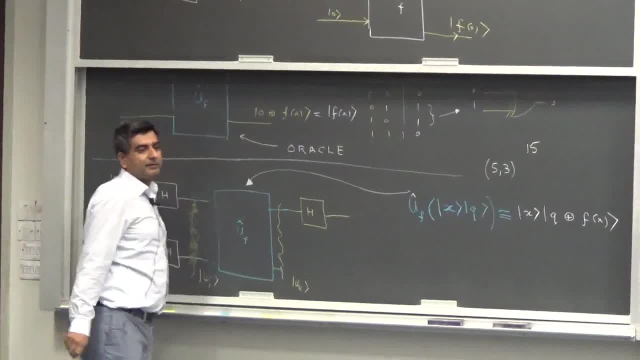 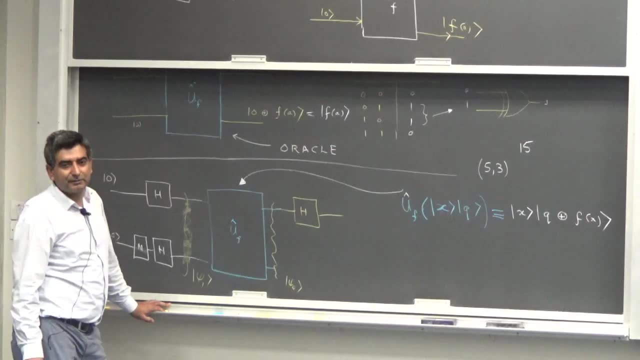 let us see what will happen. so if I want to put a Hadamard gate on the first qubit, now that is the first qubit and this is going to be the second qubit, this is going to be the third qubit, this is going to be the fourth qubit. so since I put four qubits, I am putting 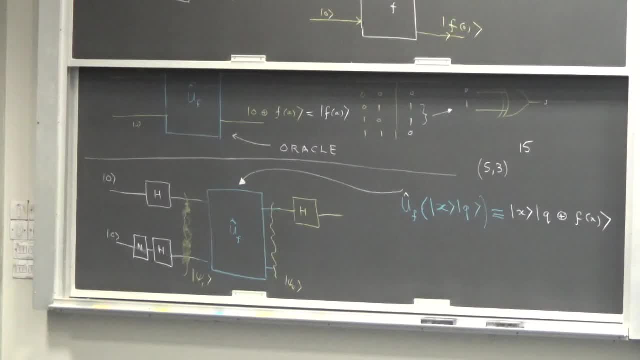 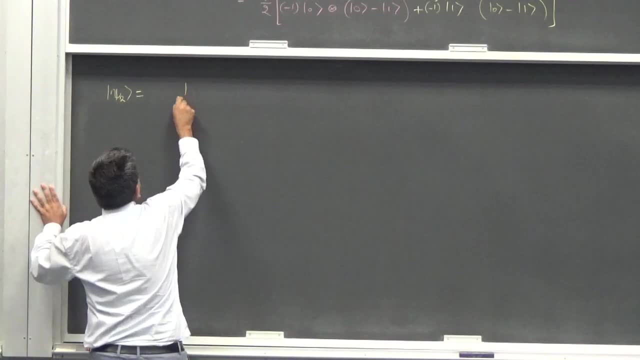 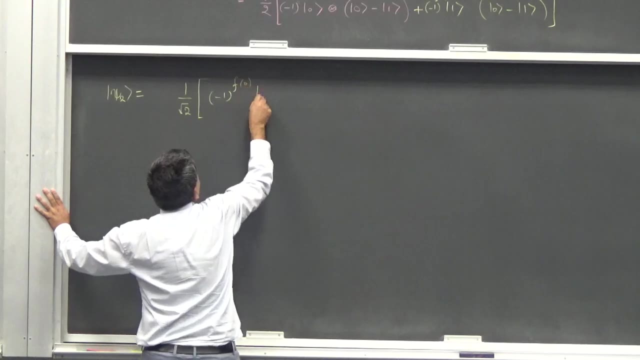 a Hadamard gate here. so I am just going to see the top qubit. so we are going to put 4, So I can also write the state psi 2 in the following form: 1 over n root, 2 minus 1 ket. 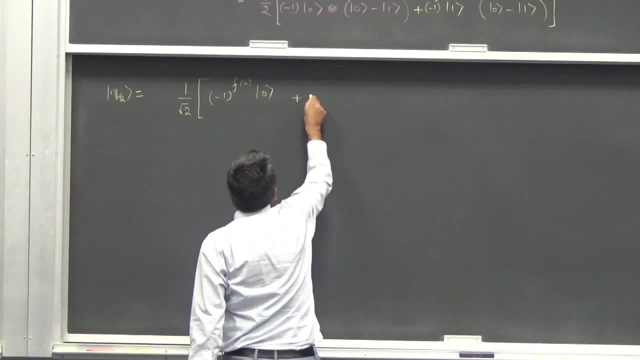 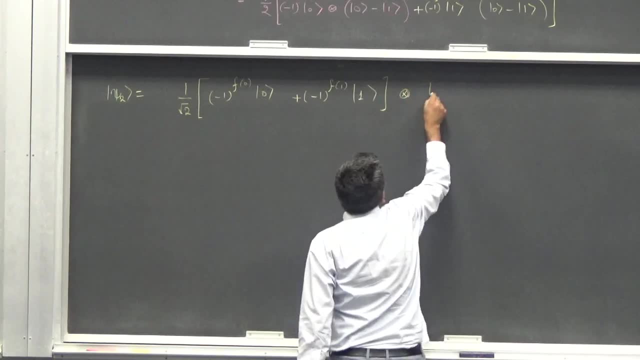 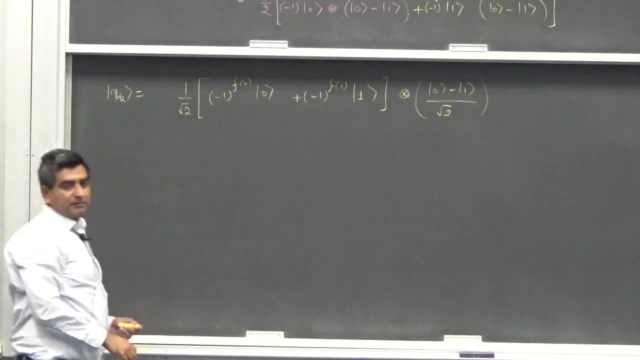 0 plus minus 1 ket 1.. So now I would like to do a Hadamard gate. So on this psi 2, I apply Hadamard operation just on the first qubit, and if I want I can apply Hadamard gate. 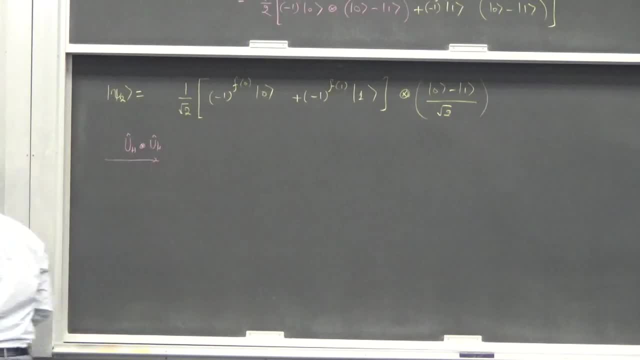 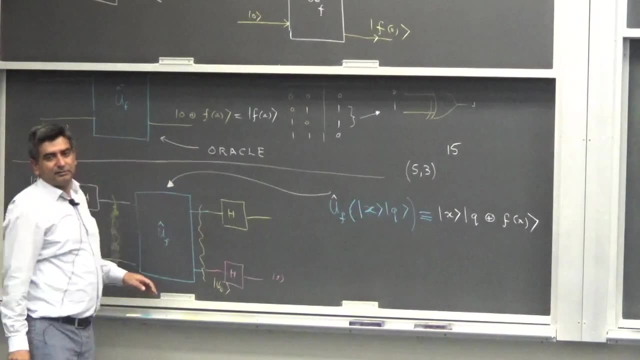 on the second qubit as well, But it does not really matter. what this Hadamard gate here would do is that it will bring this state back to ket 1. right, but that is not really needed. but let us, for the sake of 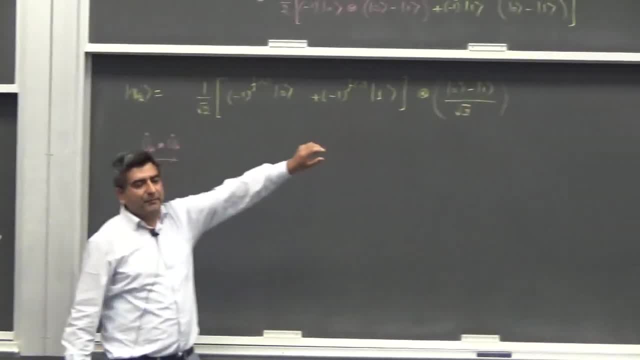 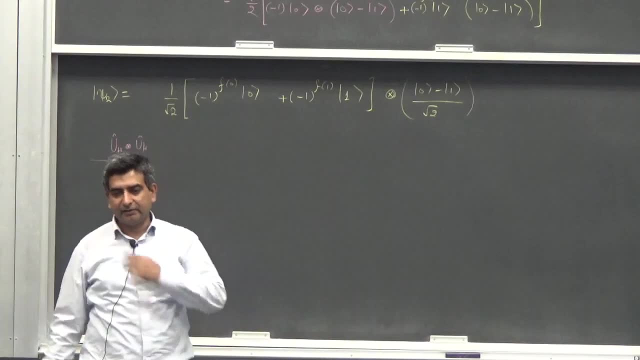 completion. do this because now we have a separable state. by the way, we can write down the state of the first qubit and the state of the second qubit. there is no entangling as yet and there will be no entanglement in this in this algorithm. So what is going to happen when the Hadamard 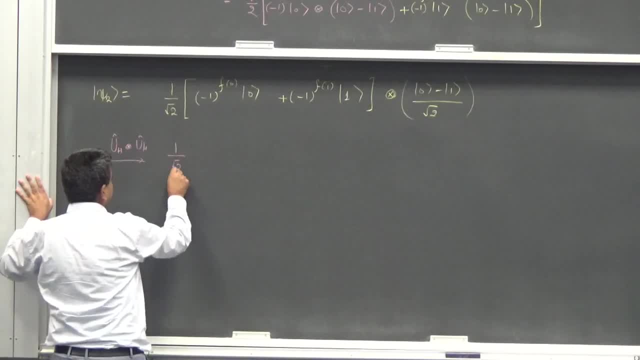 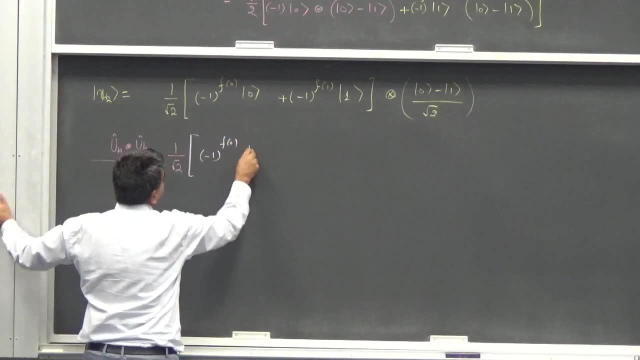 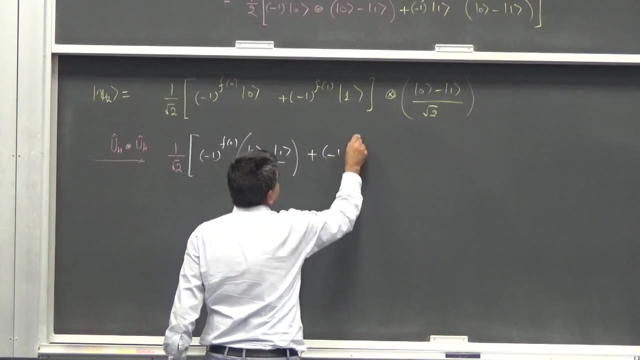 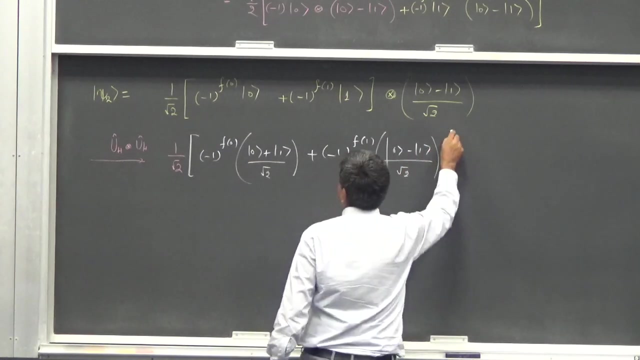 gate acts on the first qubit. you already know what the recipe for this is: 1 over n root 2 minus 1 is for f of 0. this will become 0 plus 1 and root 2- big parenthesis, minus 1. f 0 minus 1 over n root 2 big parenthesis. and this is just gone back to ket 1.. So this: 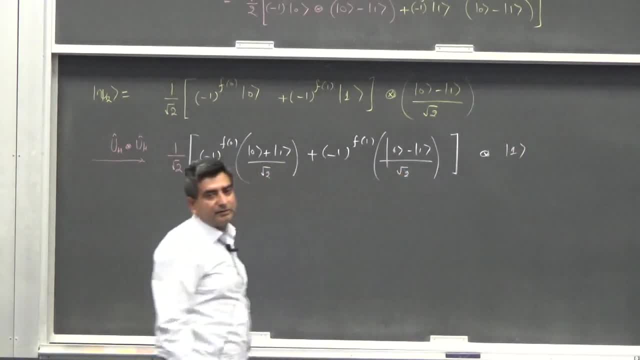 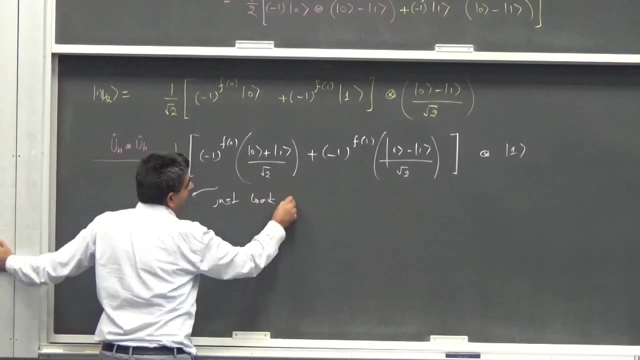 is the first qubit. Thank you, Thank you, Thank you, Because the Hadamard gate acts on the second qubit and just converts it back to ket 1.. Now let us try to just. let us just look at the first qubit. I am not concerned with the 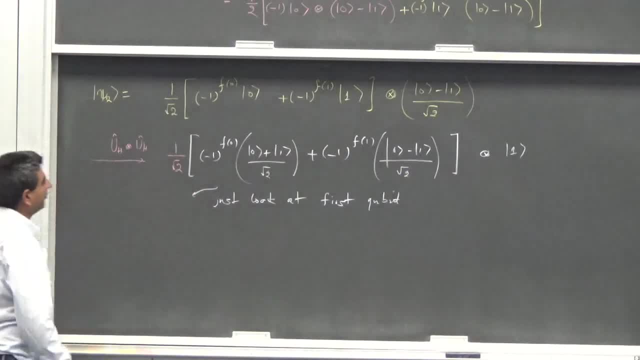 second qubit: right, we already know what this is, so the first qubit will go as follows: 1 over n root 2, 1 over n root 2 minus 1 plus 4 over n root 2 plus 1 over n root 2 plus. 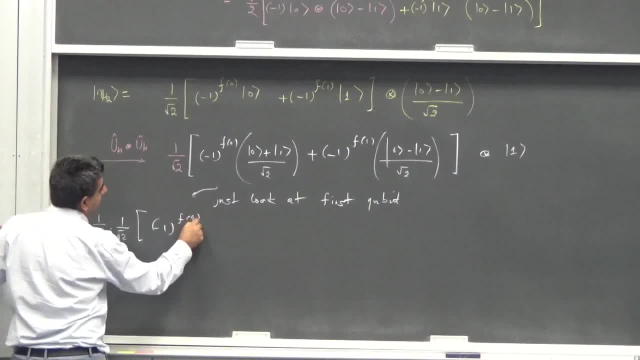 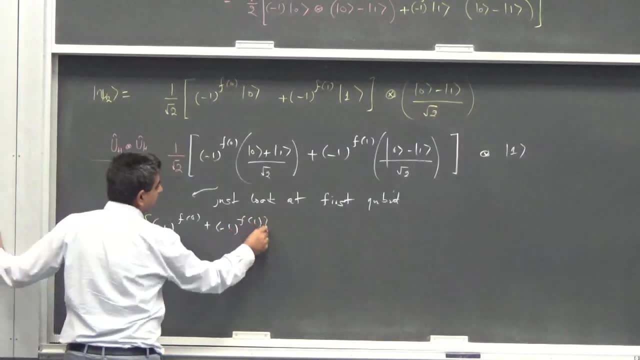 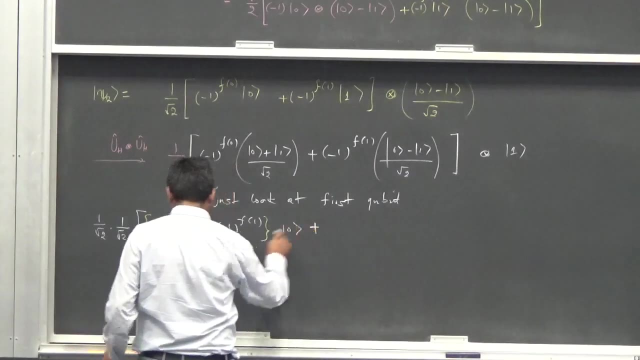 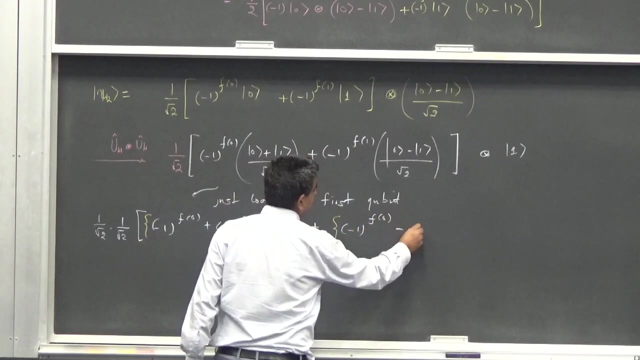 1 over n root, 2 minus 1.. F of 0 plus minus 1, F of 1, ket of 0, plus minus 1, F of 0, minus minus 1, F of 1, ket. 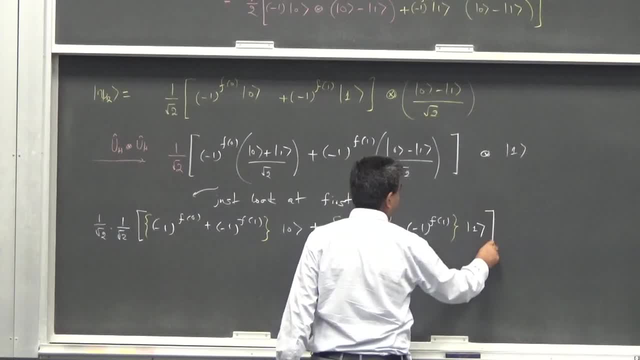 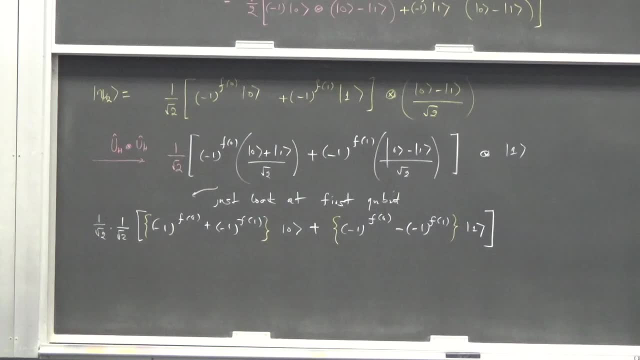 of 1.. Now is it possible to distinguish between balanced and constant or biased functions, Isn't it So? if F 0 and F 1 are constant, then it is possible to distinguish between balanced and constant or biased functions If F 0 and F 1 are different, which means that if the function is balanced, which means 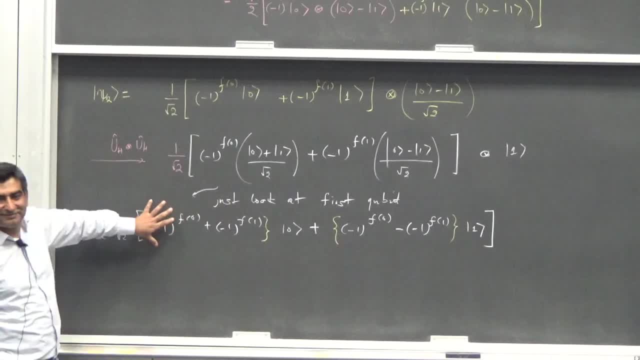 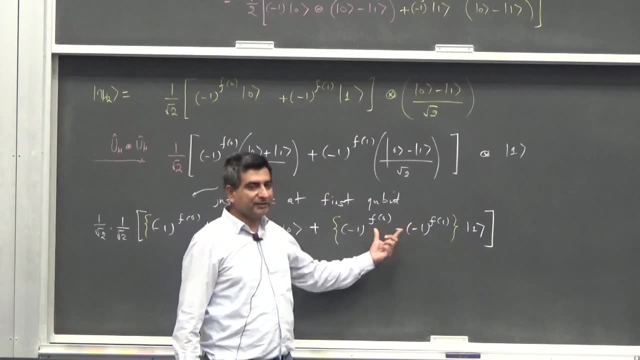 1 is 0,, 1 is 1, then this term disappears, But this term survives fully. So this becomes a 1, this becomes a 1, this becomes 2.. There are two cancels of this. you left with ket. 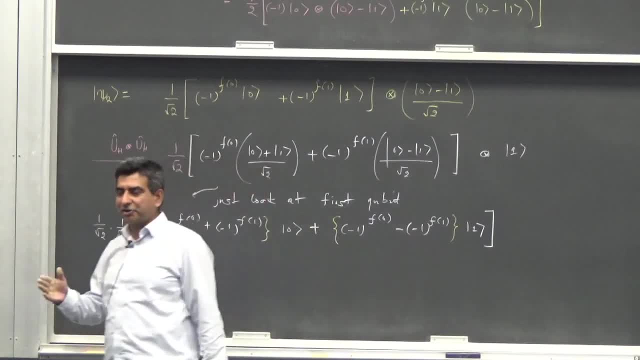 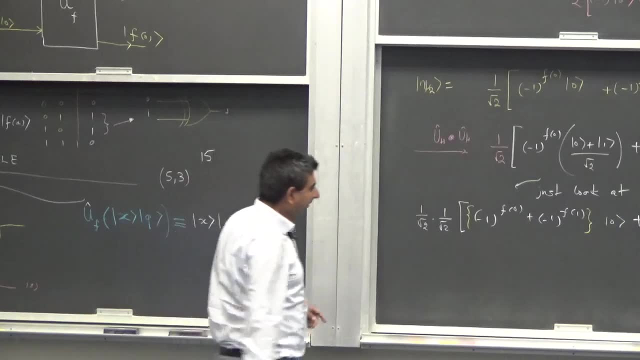 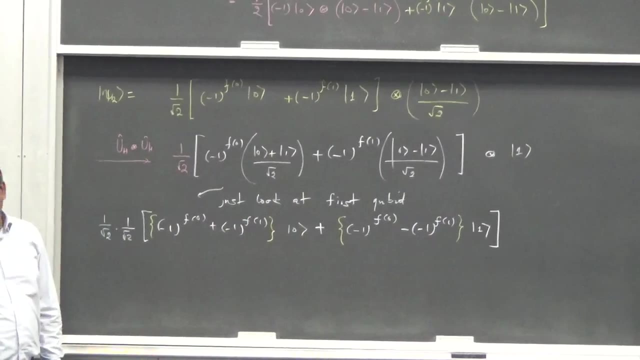 1. If the function is biased, which means both of the functions are balanced, then this terms give you the same output. then these terms will survive. this term is going to cancel out and you are going to left off with ket 0 only. So now I put a detector over. 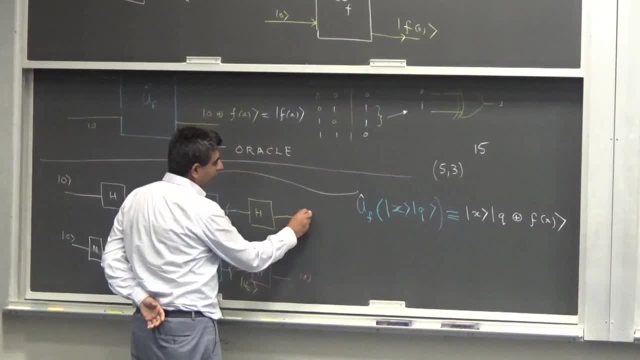 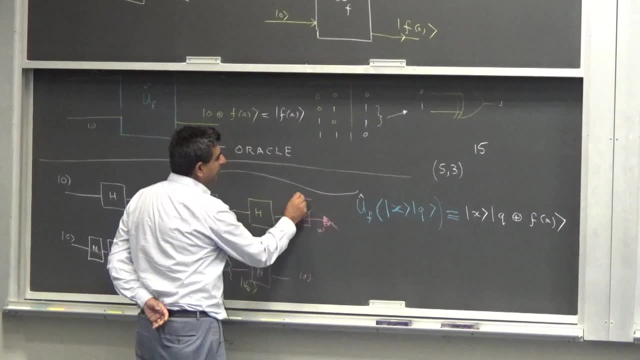 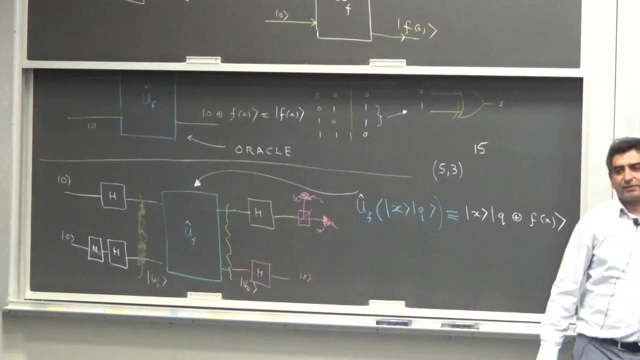 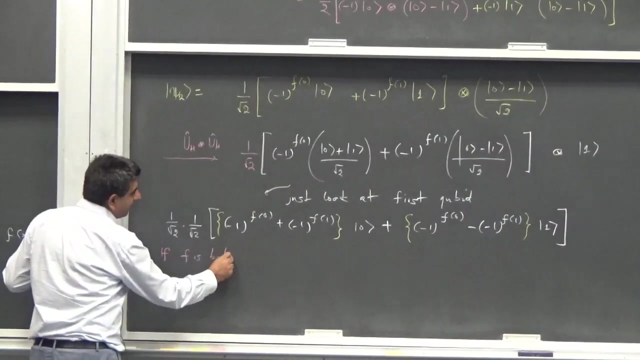 here, of course preceded by a beam spinner that can produce two output channels, and I put two detectors here, and by seeing which detector clicks I can tell in one go whether the function is constant or is it balanced. So if F is balanced, then this term just withers away, because this will be minus 1. 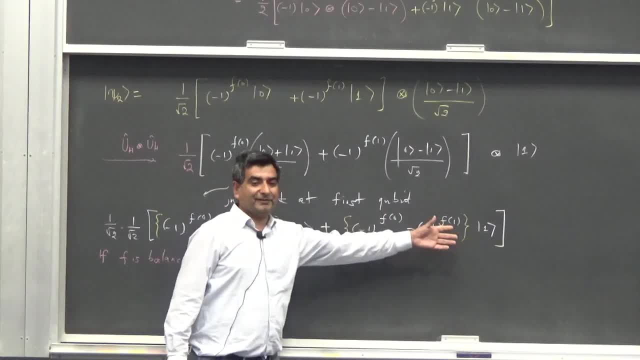 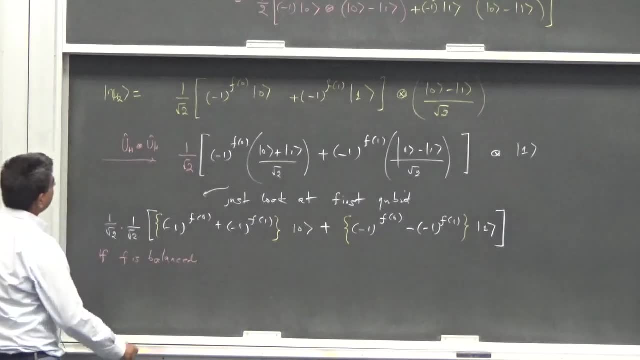 as per something minus minus 1 as per the same thing. So this will be the difference of two like numbers. that will be 0.. So the output- let's call this output, say psi 3, psi 3 will be 0. 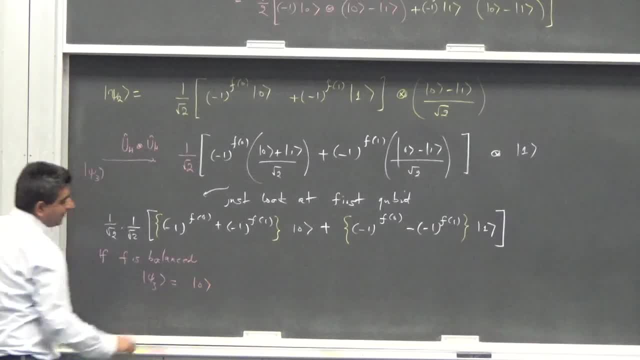 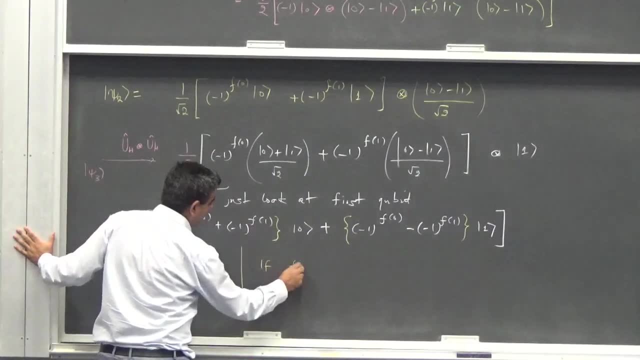 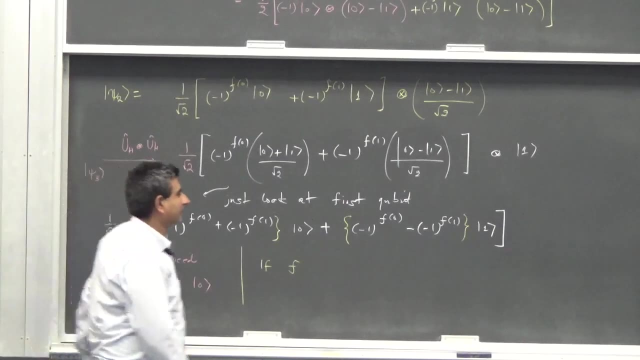 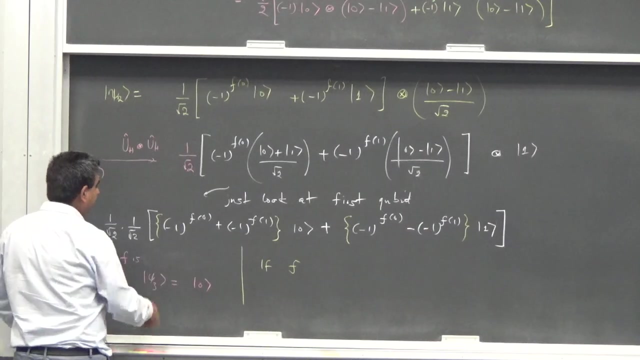 So the output will be simply ket 0,. this term is going to survive. On the other hand, if F is sorry, sorry, sorry, I am sorry. this is what is going to happen. if F is, yeah, balanced, correct, isn't it? Balanced means the Fs are different. 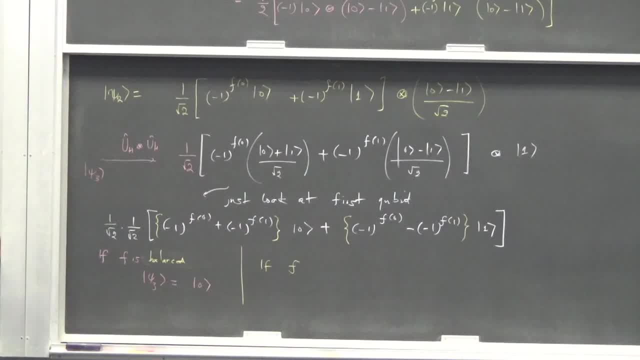 If Fs are different. suppose this is 0,, this is 1,. all right, just a minute. If F is balanced, which means that these two things are opposites, So this will be negative, So we will be left with: let's 1.. And if F is biased, bias means it's constant for both. 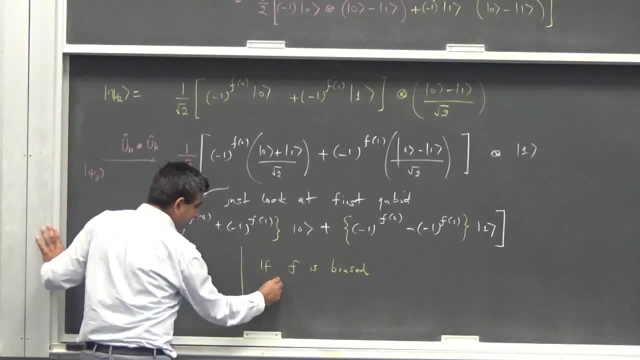 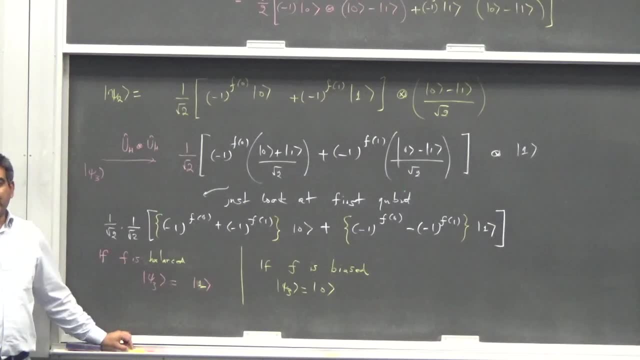 of them, then we will be left with get zero correct. So in one go we have determined whether the function is constant or it is balanced. We do a measurement over here on this qubit. Now let me recap a few things here. This is the Deutsch algorithm: a simple. 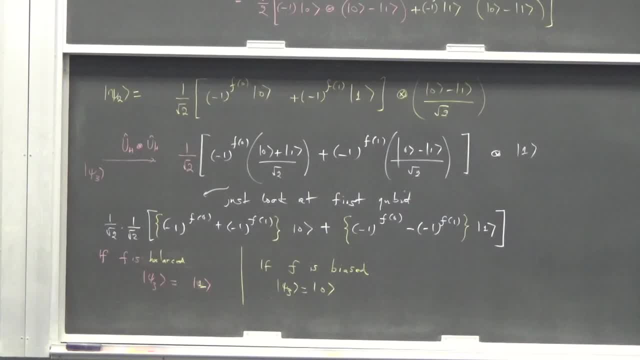 example of a quantum algorithm, one of the earliest ones. It solves a certain problem. The problem is, you have a function f that acts on a binary string, and there are two kinds of functions: constant or balanced. biased or balanced. Constant means the same. 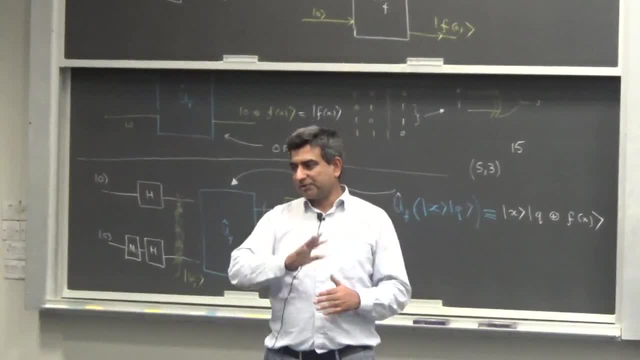 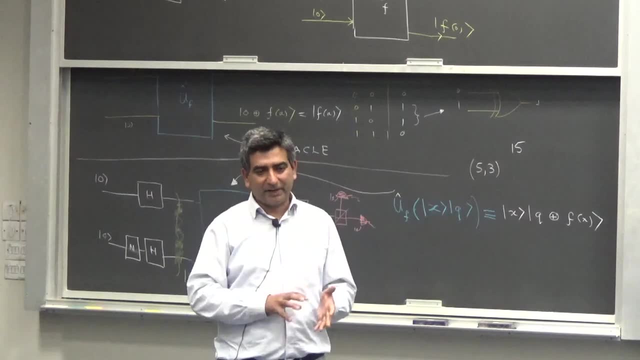 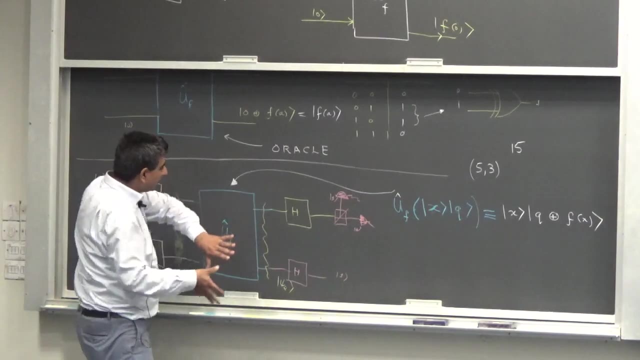 output for everything, which means biased, So constant or balanced, and you have to determine whether the function is balanced or balanced. Now the function is already there, right, because it has been encoded into this oracle. What the oracle does is you already built a function and you would like to tell whether? 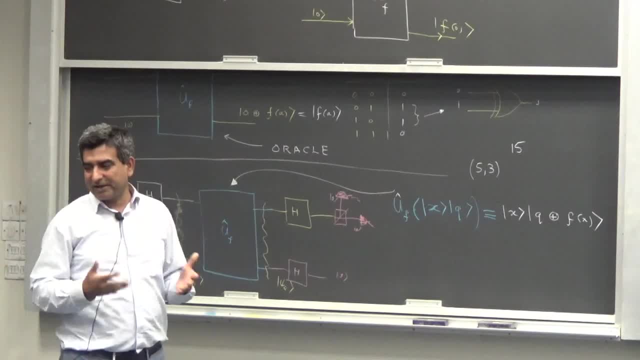 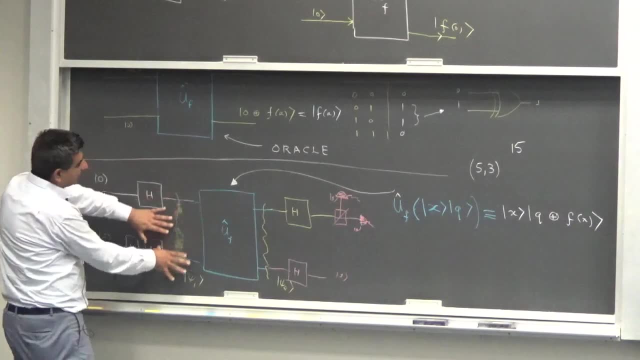 that function is constant or balanced. So you would like to investigate a property of that function. You could do this in one go by initializing a quantum computer in a superposition state. So what we are doing here is that we are creating a superposition state. So 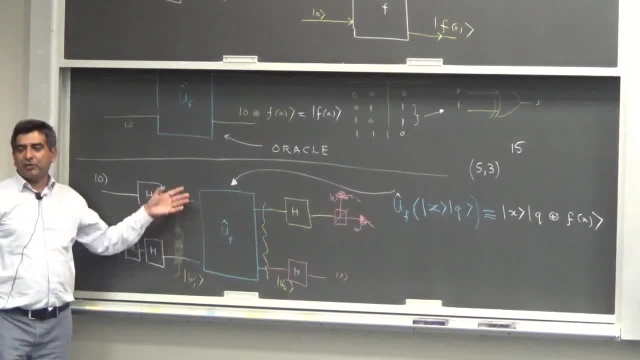 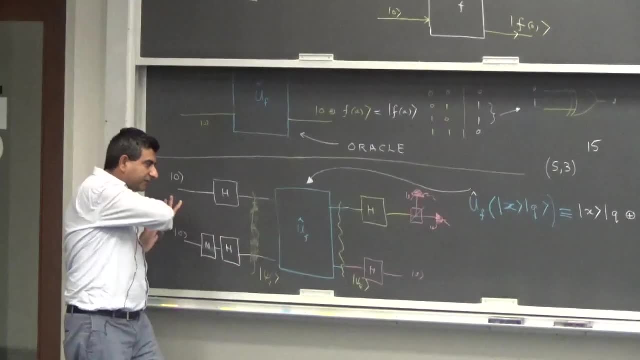 we are creating a superposition here, and that's a general scheme of many quantum algorithms. You take some inputs in the Zeeman basis or computational basis, and create a superposition and you just feed in that superposition into an oracle. Now the oracle has implemented. 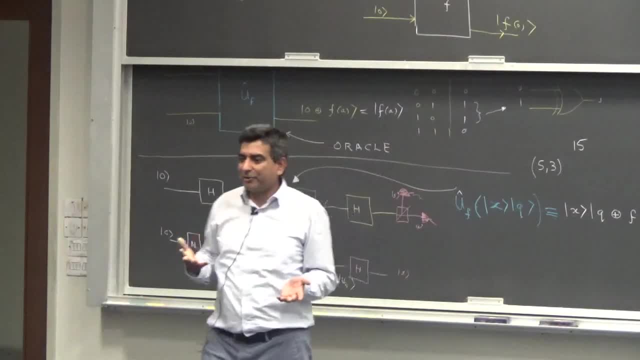 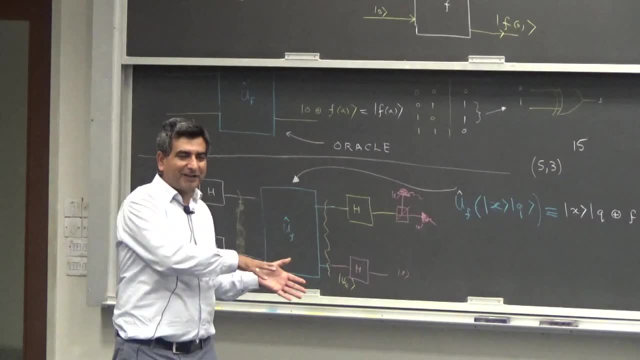 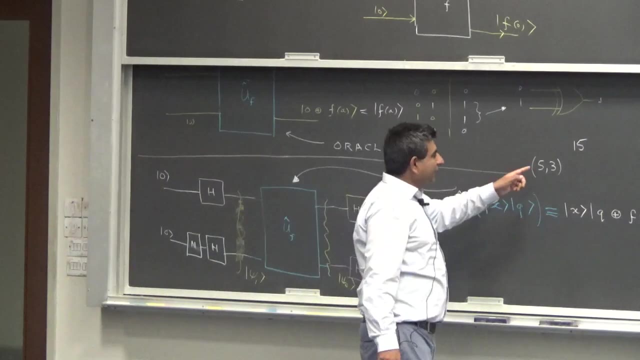 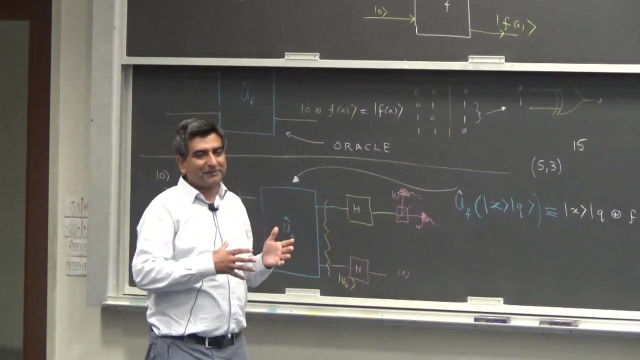 the function already. This seems kind of paradoxical that when you were building this quantum computer you knew what the function is and you had built it already. But this is just like a question of determining whether the function is constant or it is balanced by looking at 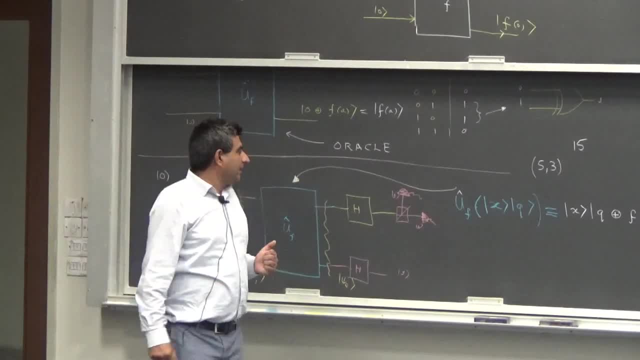 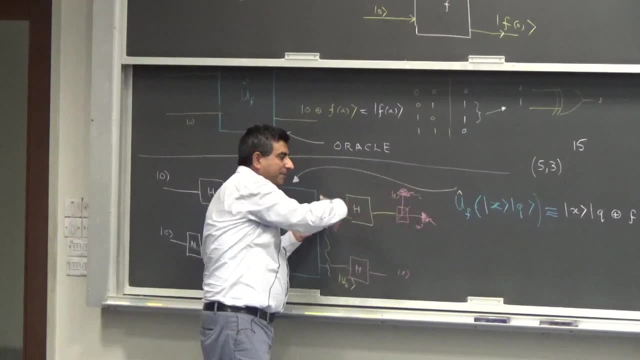 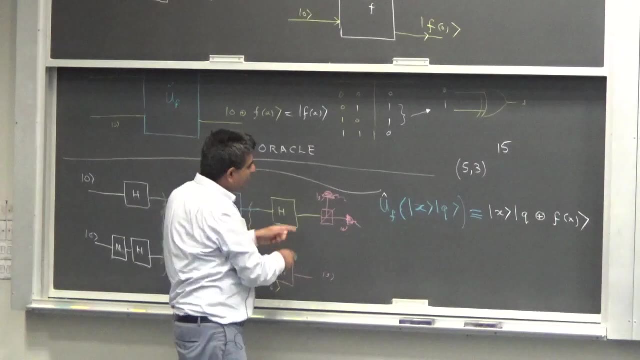 what the outputs are in one go. Now you have a certain output and then you project back the superposition into a measurable state. So you are measuring back in ket 0 or ket 1.. And the answer to your question has been ingrained into what you are doing here. So 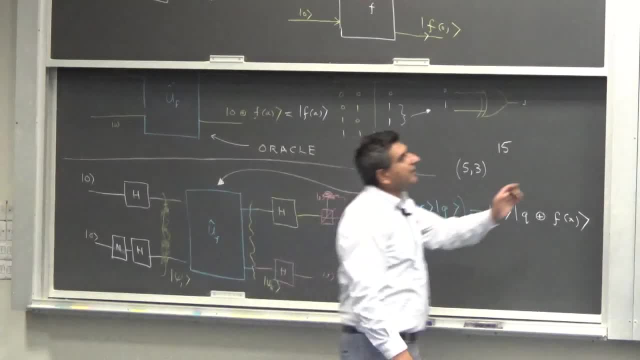 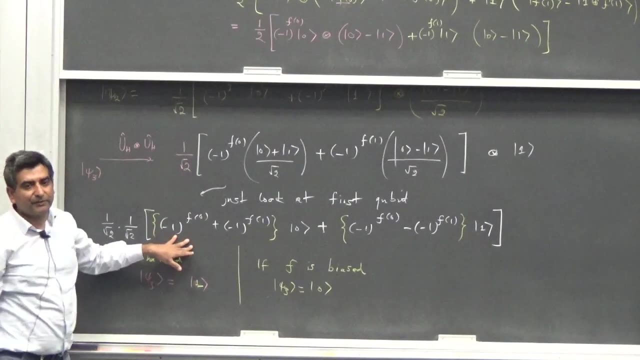 what output you are measuring here. So here we started off by creating a relative phase between components of the superposition state, And that relative phase has an impact on final probability outcomes. So even though we cannot directly measure the relative phase, that 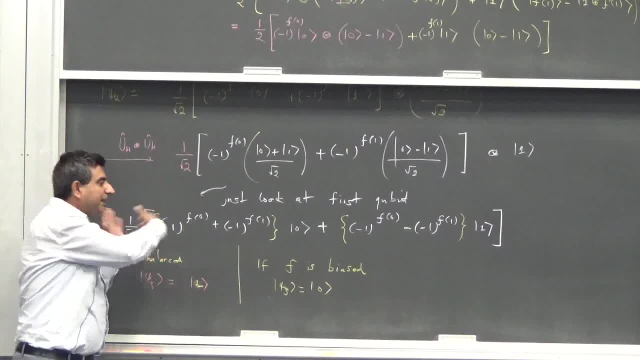 relative phase has somehow got to bleed through to the probability amplitude of the final state. So what we are doing here is that we are taking the probabilities, which are modulus squares of these probability amplitudes tell you what the function is. So, even though measurement 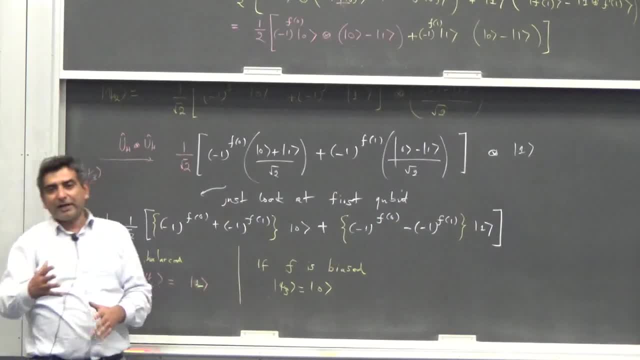 is now collapsing the state into ket 0 and ket 1, by looking at the kind of collapse- what is this state collapsing into- you can tell what function. it is All right any questions about this. Yes, Are those inputs arbitrary? I mean, can they be in a superposition? 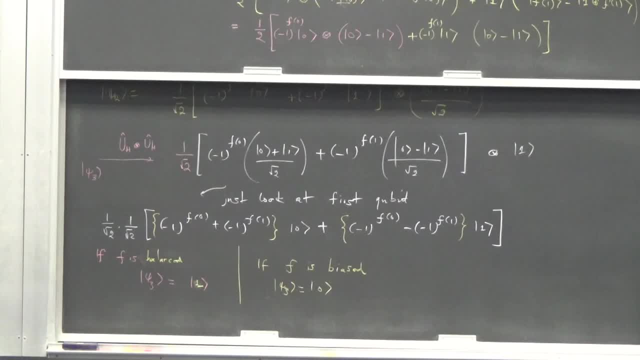 Yes, So you would not need these Hadamard gates. So these Hadamard gates are just meant to create a superposition, So that superposition is fed into the quantum computer. Otherwise you will have a scenario just like this. So, but then you will not get any complexity. 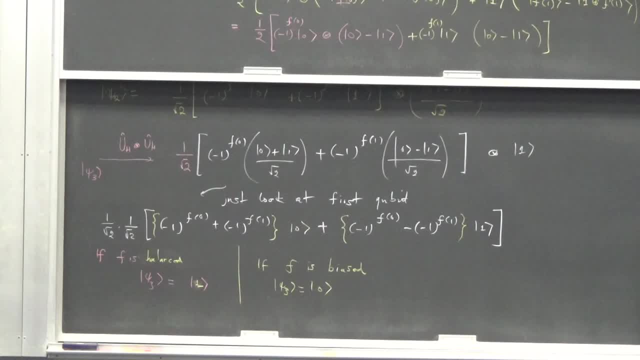 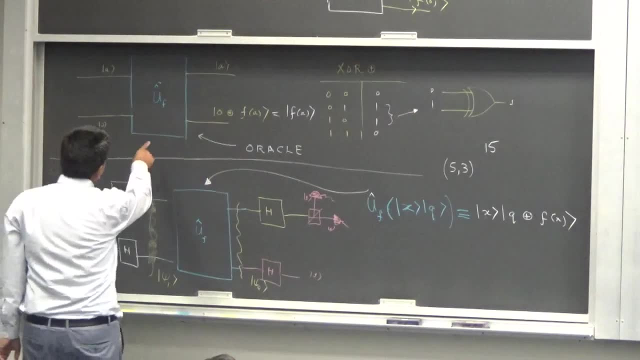 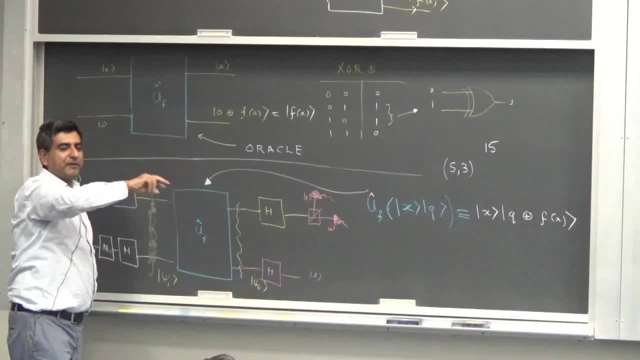 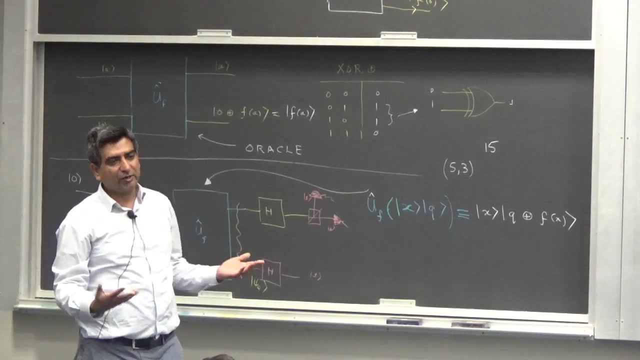 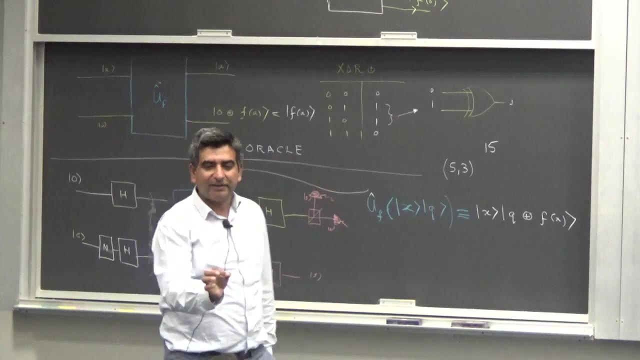 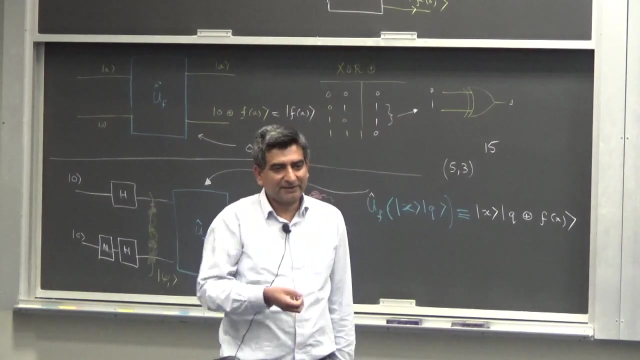 you need 2.. So you need 2.. So you need 1.. So you need 1.. So you need that. I see I am able to potatoes the I know you can see here disrupt ığını. 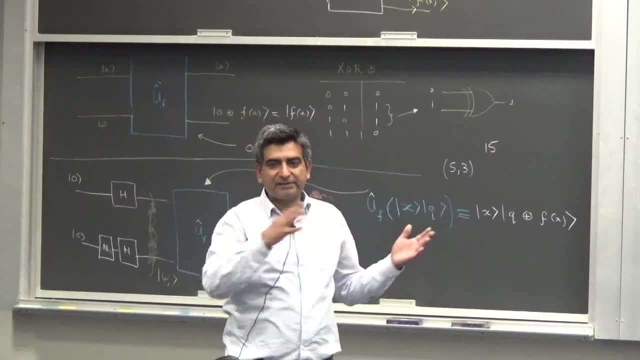 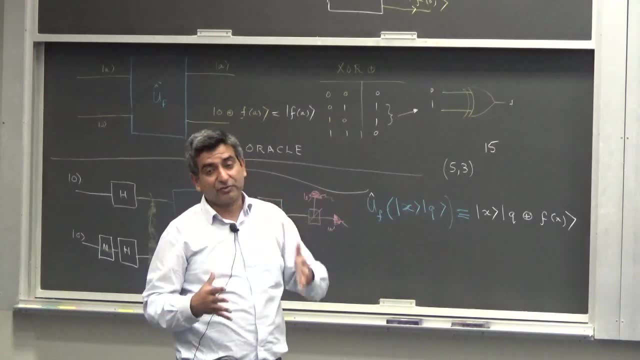 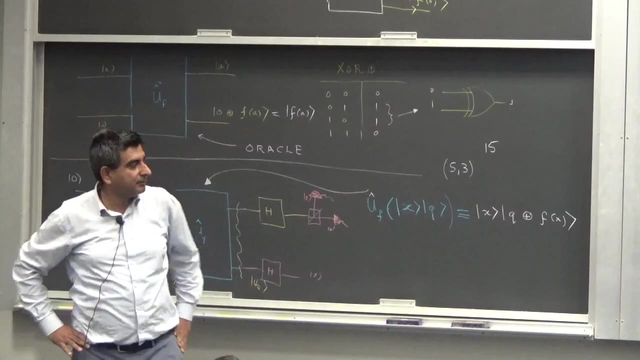 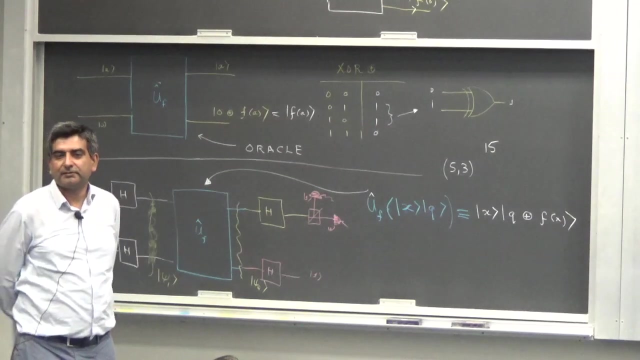 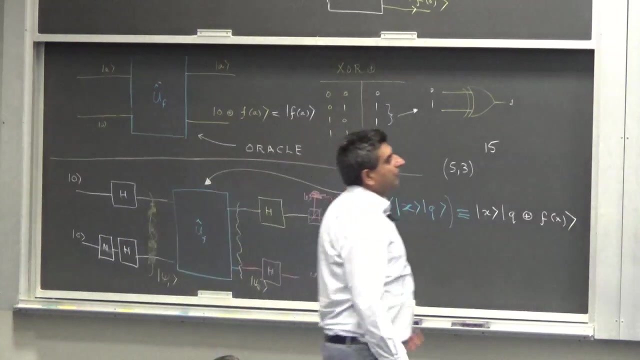 or fair. But now the query: complexity that is achieved quantum mechanically is just one. So in one shot you can tell whether the function is constant or balanced. Yes, So what is happening here? there are different ways to look at this. Initially, look at those. 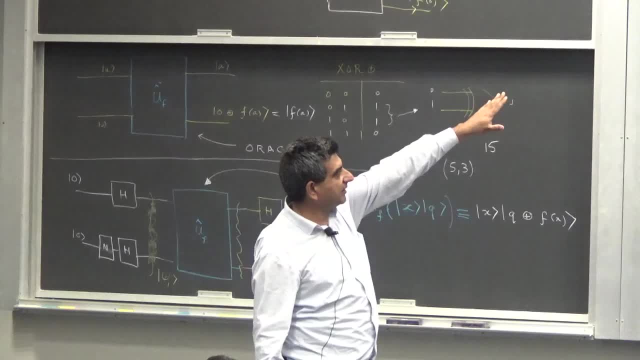 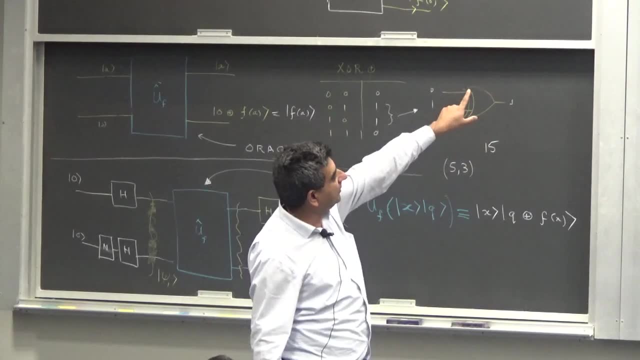 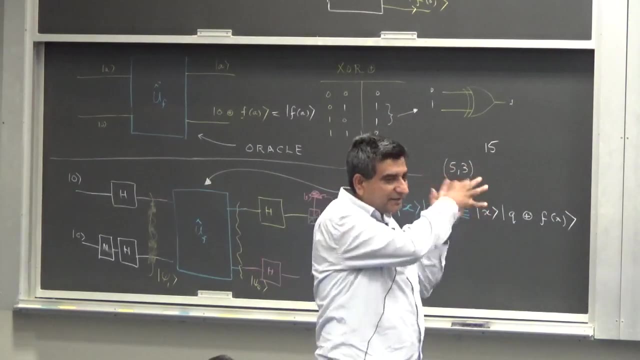 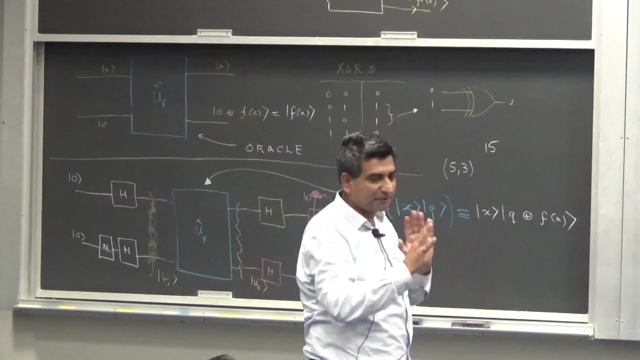 two qubits. So what you are doing is imagine that there are four paths. Each path comes with a sign. Now there are certain paths that are destructively interfering, certain histories that are just withering away there opposing one another, and you are just left with two possible paths. 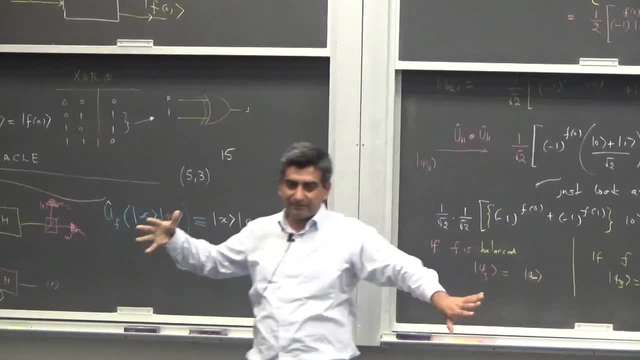 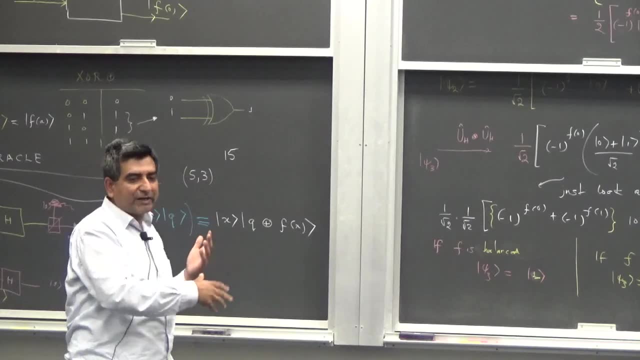 0 and 1.. So there is some destructive interference taking place and you have designed this. Yes, So you have designed your algorithm in such a fashion and your quantum circuits are built in such a fashion that, even though you are getting collapsed measurements, still your 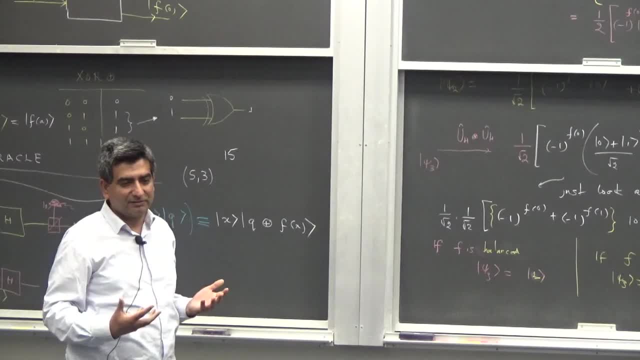 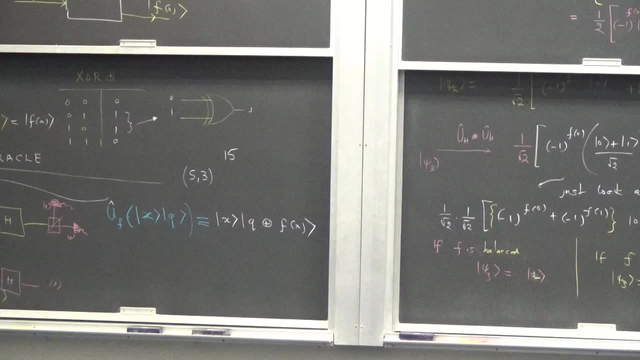 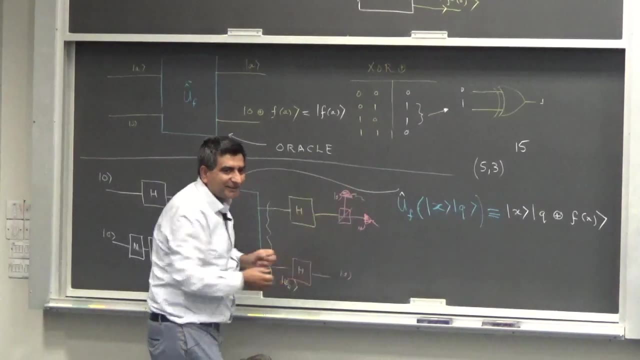 measurement is telling you something about the function. So, and how do you achieve that? This is the general scheme. You input, your initialize your quantum computer by some input states, you create a superposition, let it go through an oracle and then bring it back. 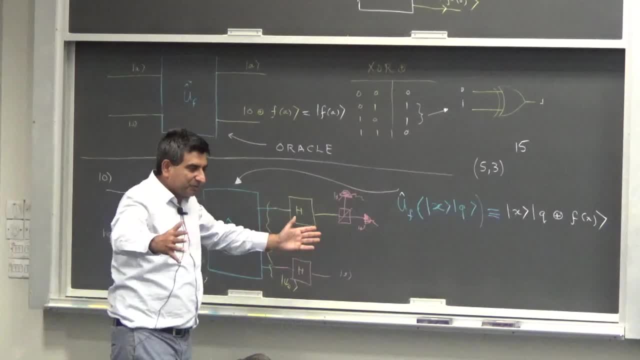 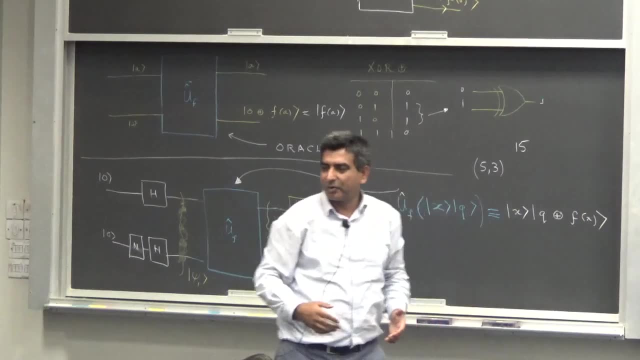 Just like two waves: you create the waves, create a superposition and then you create a superposition, Let them interfere and then bring them back and make a measurement. Remember the mass-generated interferometer. You create an input state, create two paths for the photon. 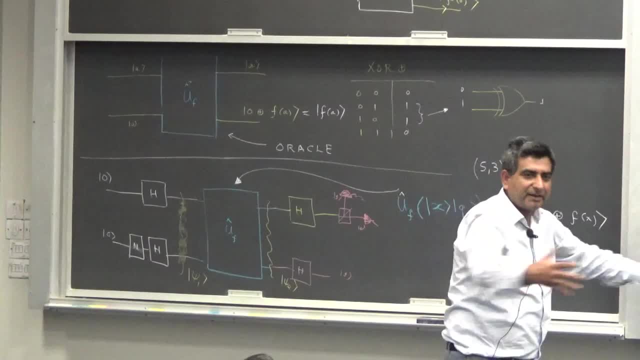 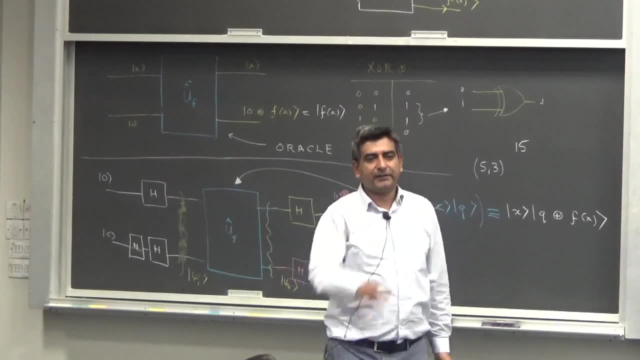 and then bring them back to the final beam filter. Exactly the same idea is at work here. You had a question. Yes, A query means a query means how many times does this, this, this, this, this, this, this? 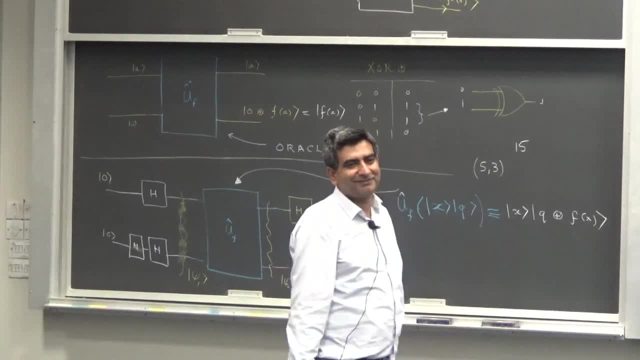 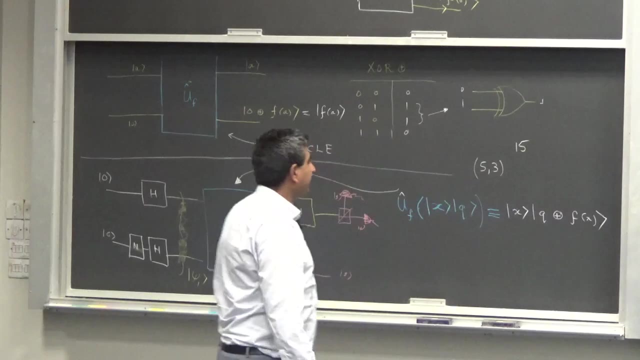 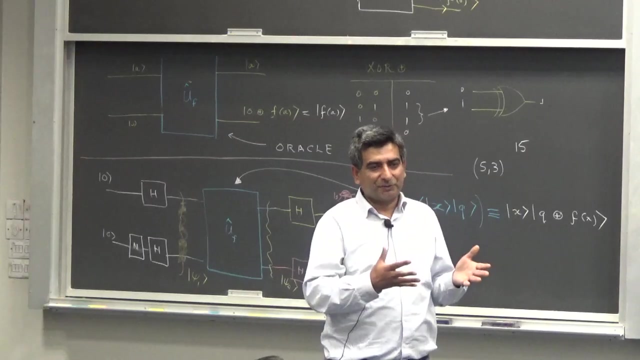 many times does this algorithm run? Measurement is something else, yes, but those two. so, having a system that has two inputs, you are doubling the number of resources, So the resources can be traded off by the number of inputs or the number of time the experiment runs. 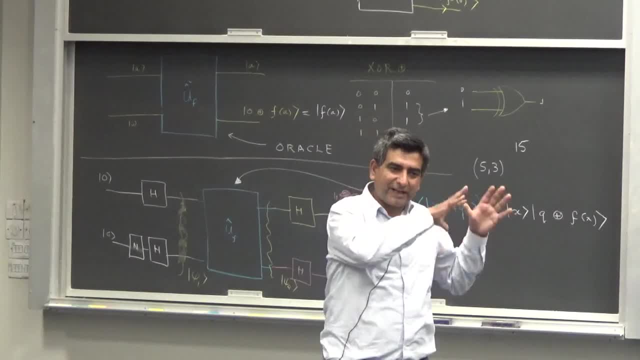 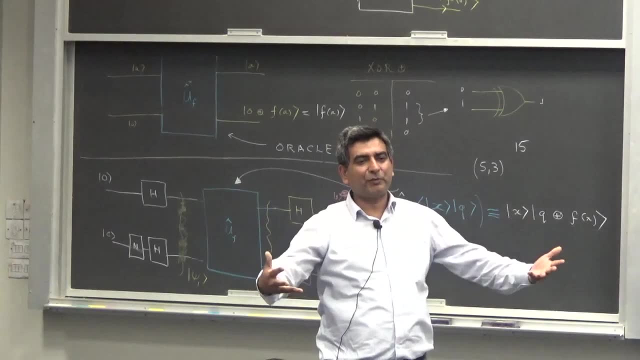 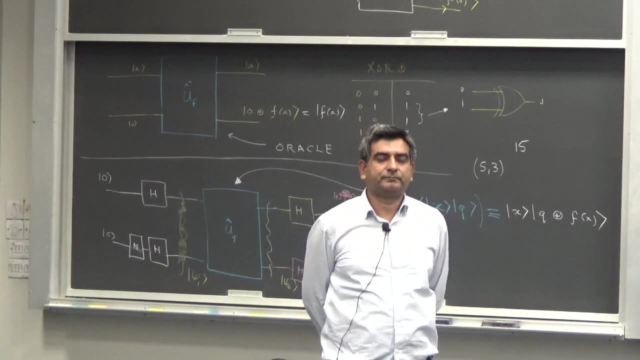 so right. so it is the same thing. number of resources input that are input into the system versus the number of time the experiment runs is just the same. both of them add to the query complexity. yes, Sir, you have designed here that the mark is not. here is all of our Doge algorithm. 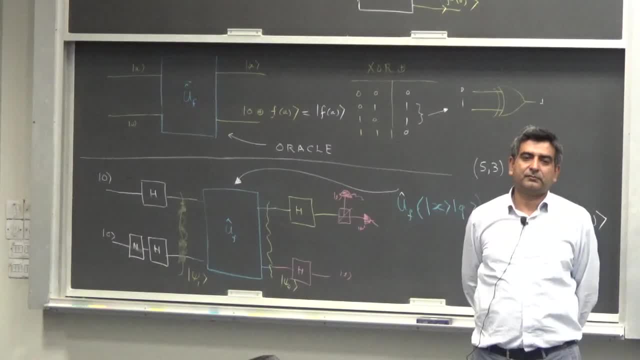 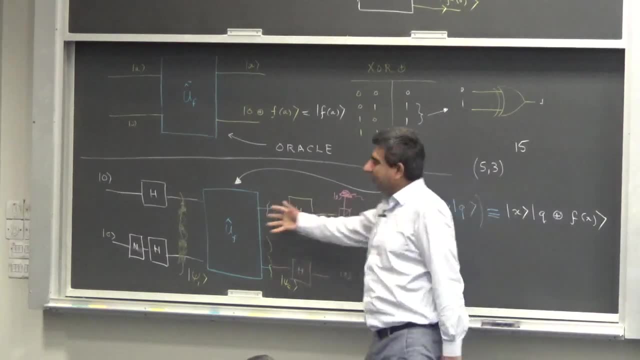 right, Right. so this is the Doge algorithm. So, basically, the purpose is to find out whether the auditor function is correct or not. Yes, And, by the way, the function has already been inbuilt into this right, so let me give. 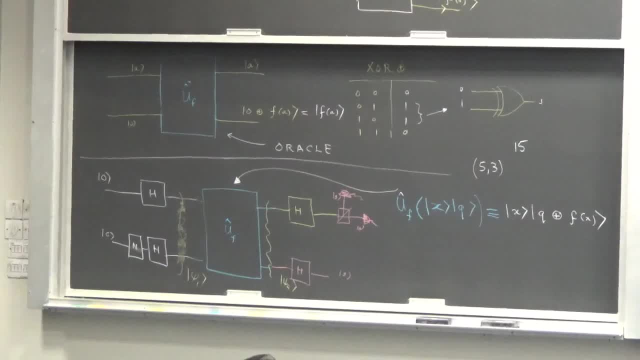 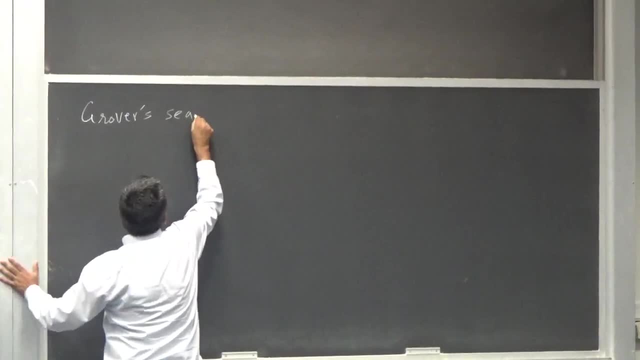 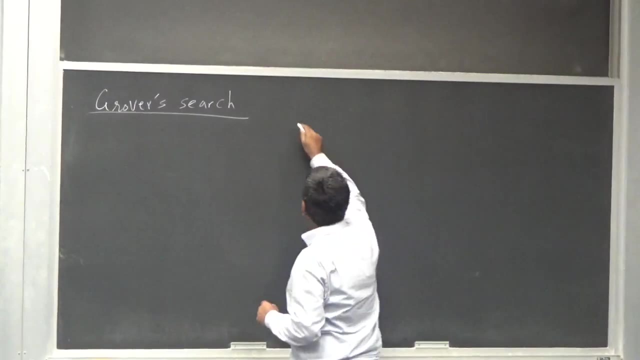 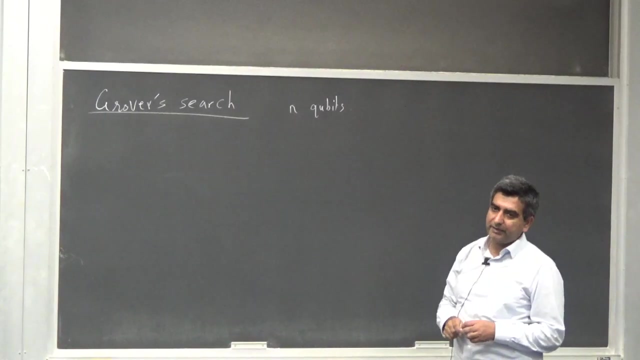 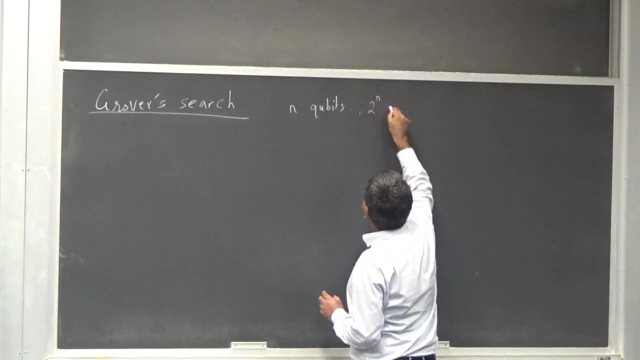 you another example, a more sophisticated example, and that is for Grover's search. Now suppose you have n qubits. Yes, Right, n qubits. so with n qubits you can create a superposition of n is power 8 states. 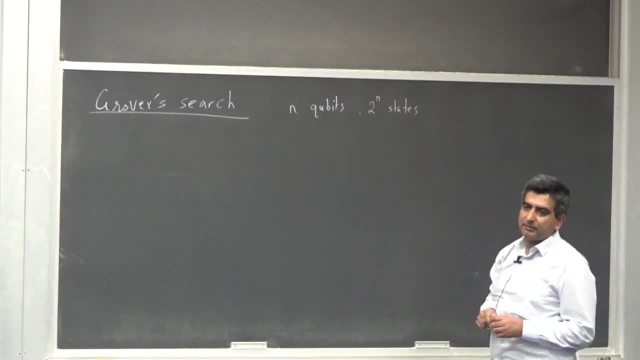 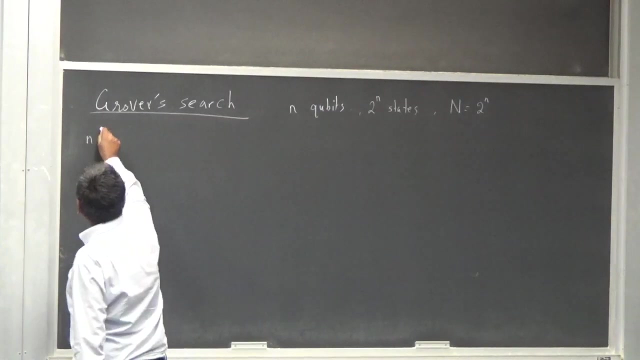 right. So let us call capital N as 2. raise power n- this is the number of states, and we have n qubits. Yes, Yes, Yes, Yes. So you can create a superposition of N bit binary string, right. so example: 0, 0,, 0, 1,. 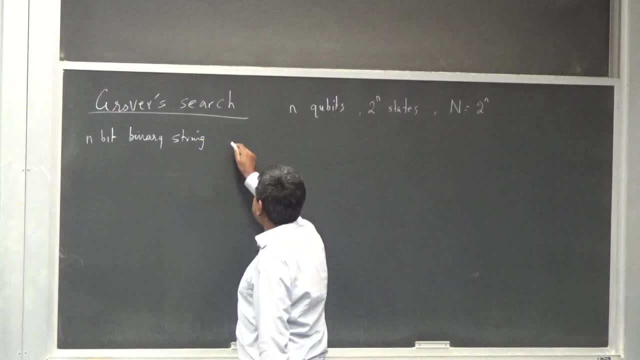 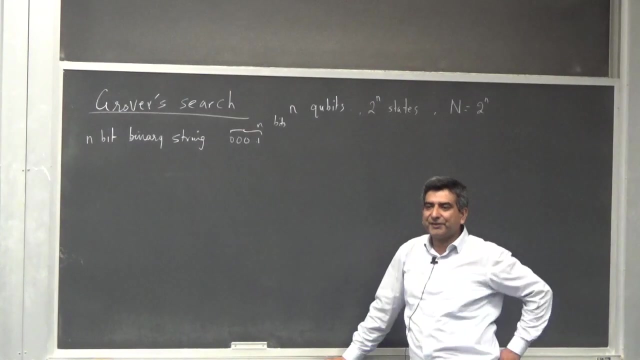 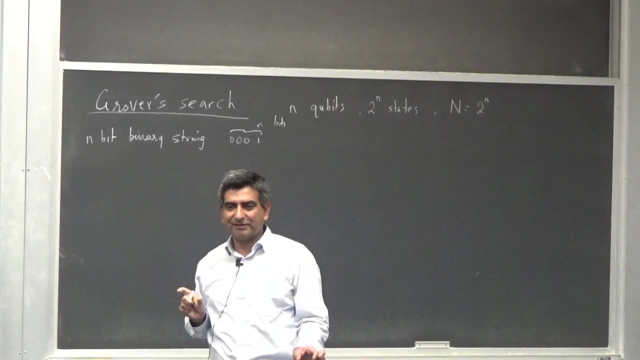 this n of these bits. so with these n bits you will have 10 is power, n possible strings and you would like to find out one particular string. you want to search for one particular search for one particular string. it's just like a phone directory. you have a. 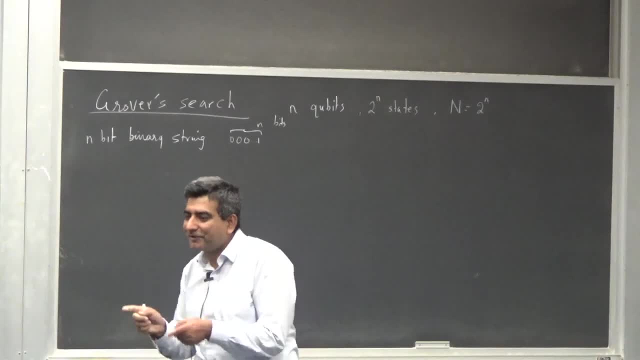 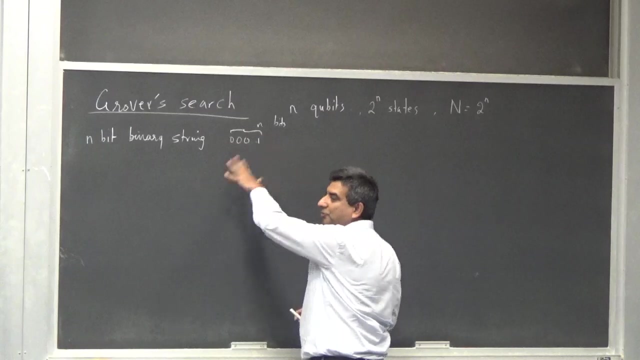 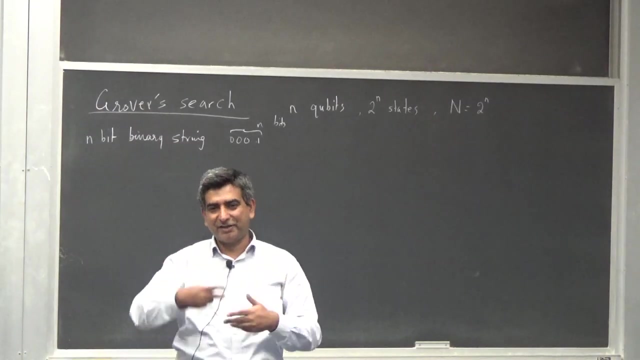 directory of numbers, large directory of numbers. you want to find out for one particular number, my phone number, from a phone directory to do the search and you have n bits and each, which means that each number is n bits long and since each number can have two values, zeros and ones, it's a binary directory there. 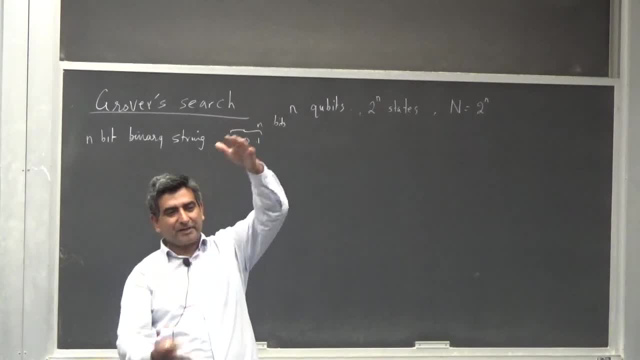 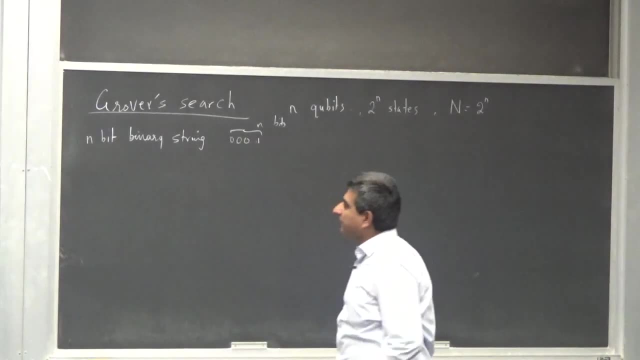 will be ten to refer, and, and small n or capital and possible numbers, and you want to find out one of them. okay, so now what we would like to do is we would like to design an Oracle for this algorithm, for this, and you want to search out our desired string from a large database of strings. suppose my 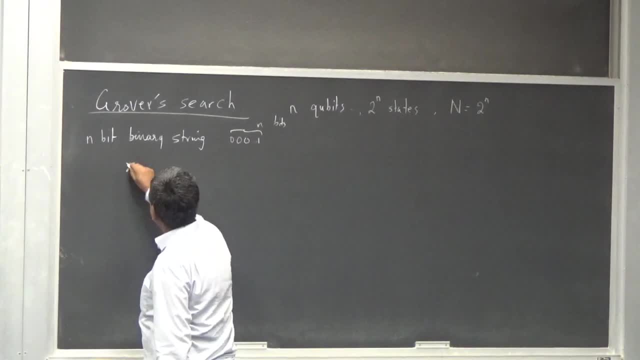 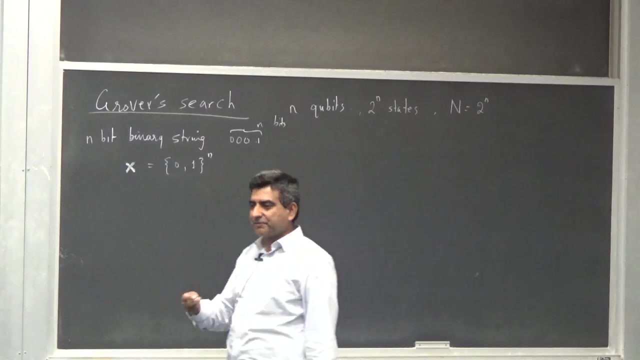 input database by any big strings are represented by this number: X. now I'm ready. this X in both side bold. so this is a sequence of n bits, some sequence of n bits, and the number that you would like to search for is, let's denote this by X star. 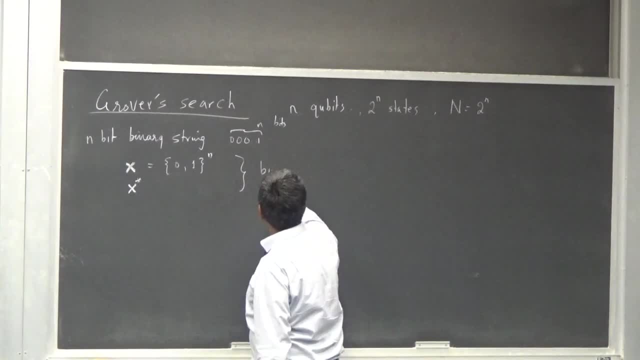 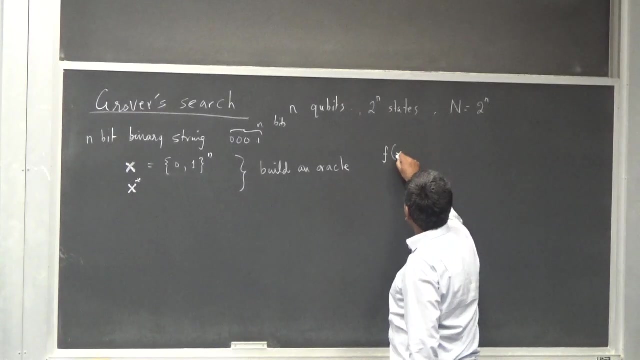 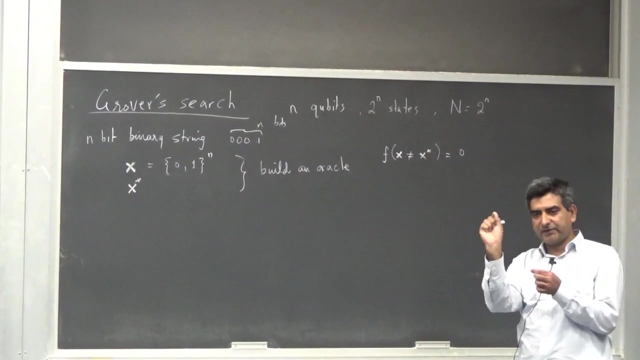 now I would like to build an Oracle, right, what the Oracle does is implement a function. the function of the function, of the function of this function is that goes as follows. so what I would like to do is, when F acts on X which is not equal to my desired number, I will get 0. my output is a single bit, 0, and if my F 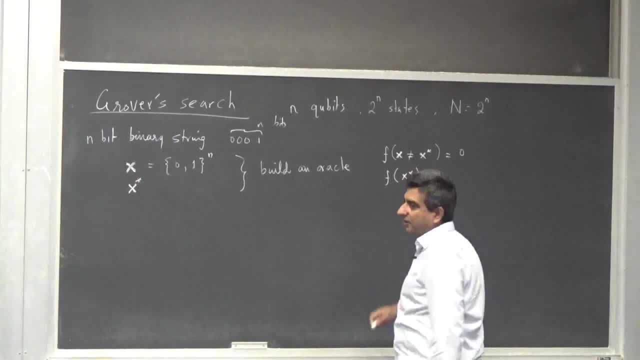 finds as argument X star, the string that I am searching for. my output is 1, so this is the logical function that I would like to build quantum mechanically into the order correct: yes, X, X, all possible, right, so this is a function that I would like to build. so, and now have defined a function similar to the: 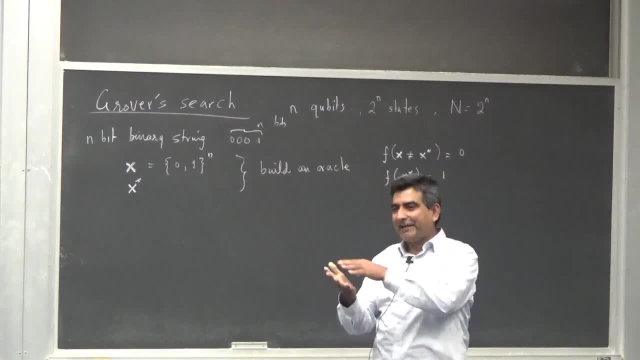 constant balance function. I have a different function F that takes in arguments and gives me a single bit as an output- 0- when my input does not match what I'm looking for, and it gives me lights up to the one where my input string is the one. 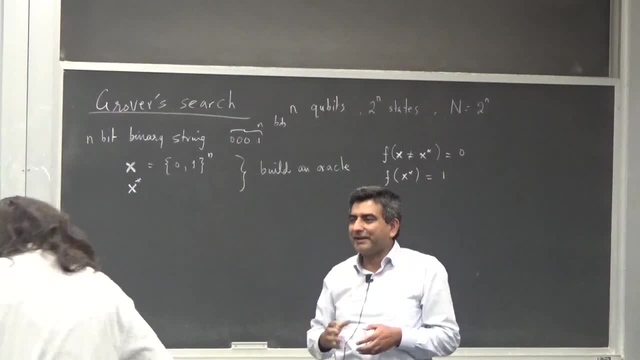 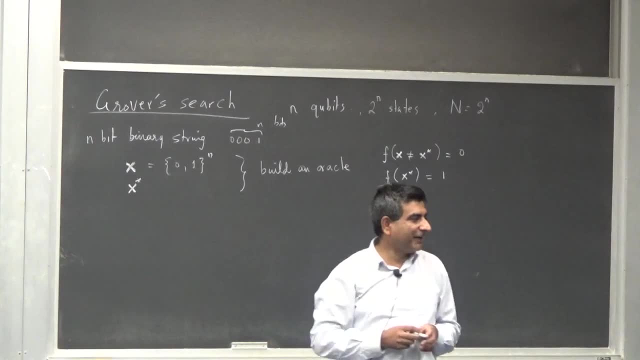 that I'm looking for now. if I want to do quantum mechanics, I would have to build this into a unitary operator and design my Oracle around it. so, exactly the same fashion: I would like to design, build a, an Oracle or a unitary op that implements 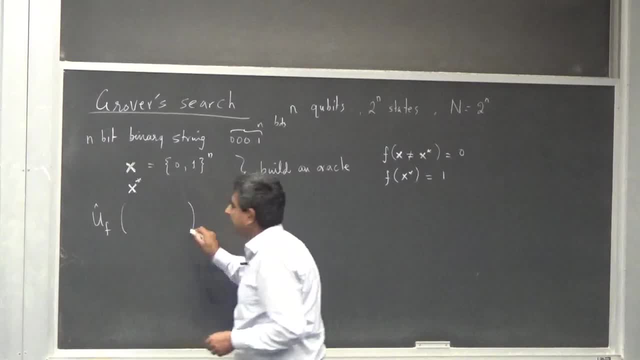 a unitary operator that implements a unitary operator that implements a unitary operator, and what this unitary operator does is the following one. so this string of inputs, any qubit string right, which is represented by this. but this is not a single qubit, this is n qubits, it's a vector, it's a big multi qubit, vector X. so 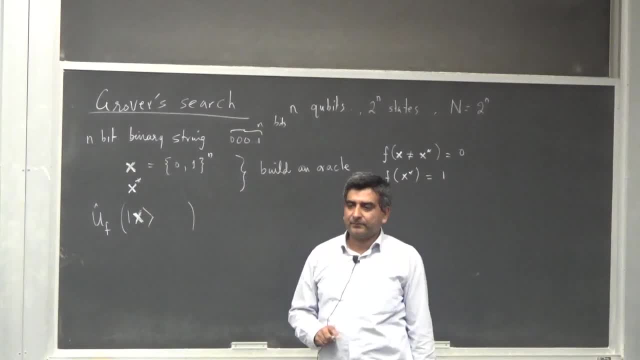 that's why I put this in bold right and I have an answer. the qubit, and this is a single state cube, and what this Oracle does is very simple: it leaves the first register, which is a sequence of n qubits in the same state, and does an exclusive. 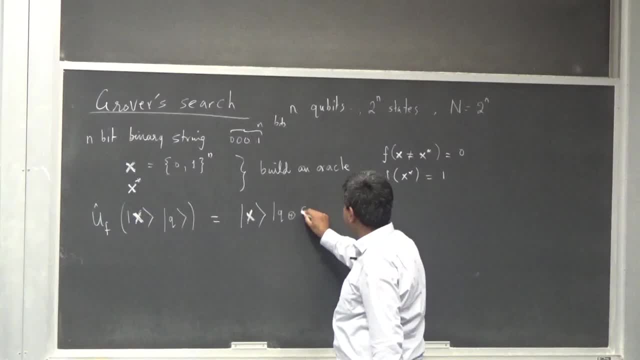 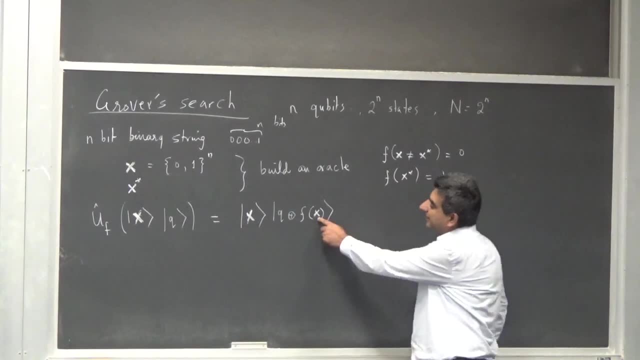 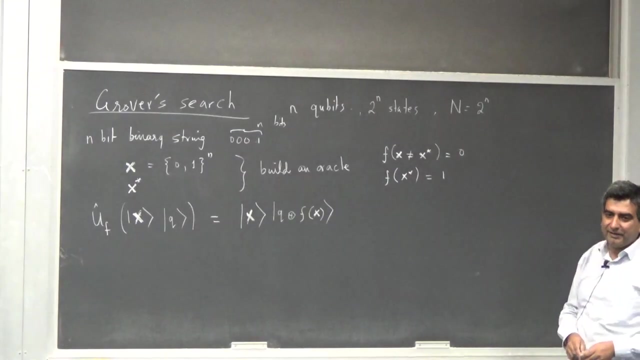 or of the ancillary qubit with the function on. if this were my desired string that I'm looking for, this will become a 1, and if this is my undesired string, this will become a 0. so now I would like to build. so this is my Oracle, this is my search Oracle, and I would like to make this a. 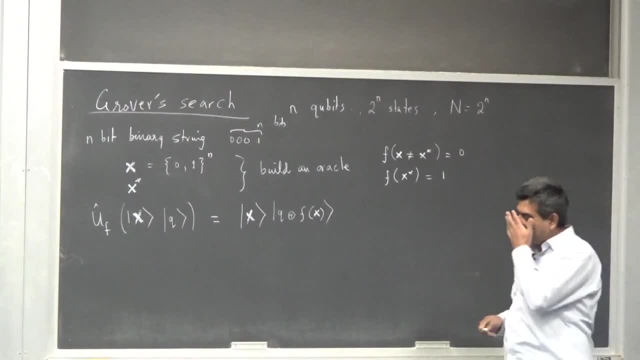 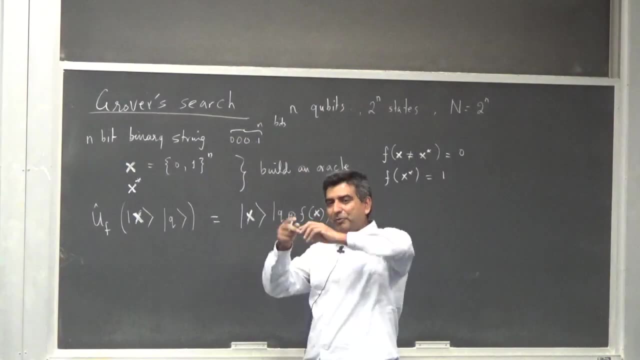 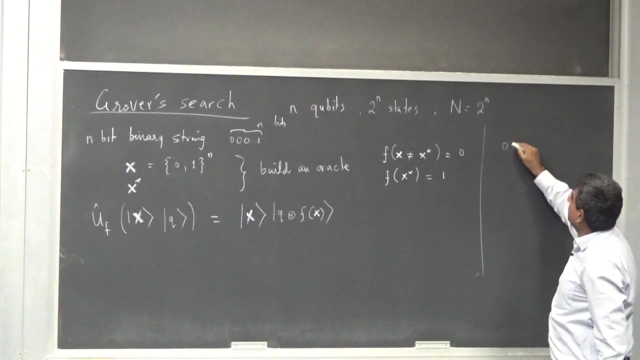 part of an algorithm called the Grover algorithm. so now what I would like to do. suppose I keep my task simple. my X, this number is 2. so I'm look, I'm looking for 2 bits strings and searching amongst two bit strings. so what two bits strings? the possible possibilities are 0, 0, 0, 1, 1, 0, 1, 1, right, so? 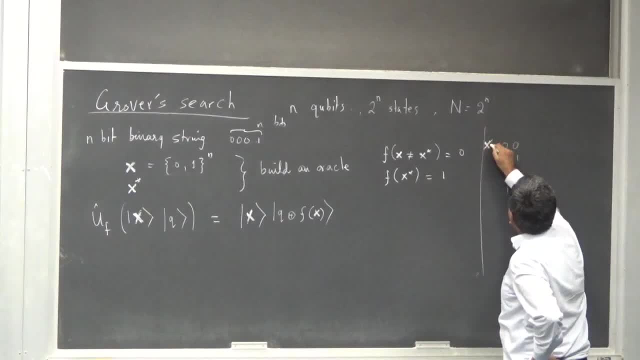 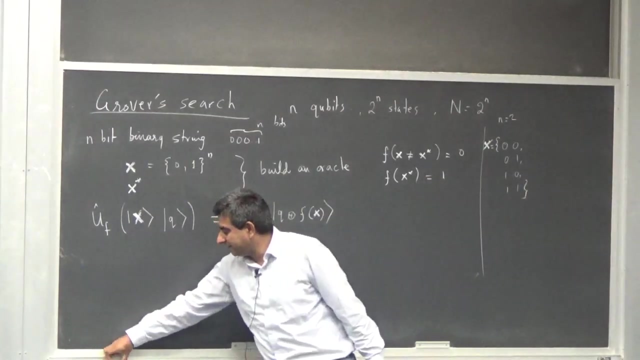 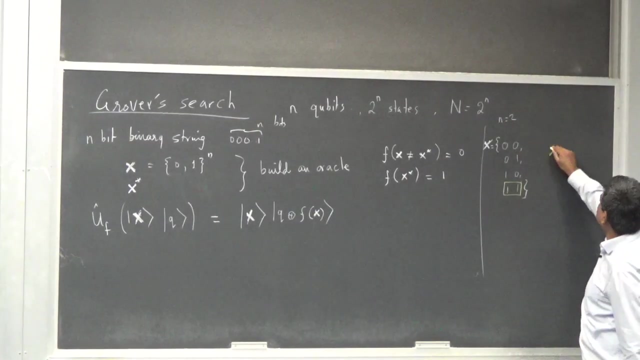 this is my entire set of possible strings. therefore, possibilities: my n equal to N is 1 string with five strings 2, capital N equals 4.. So I will need two qubits to encode these four states correct And suppose that my desired string is this one. So what I am looking for is 1, 1.. This 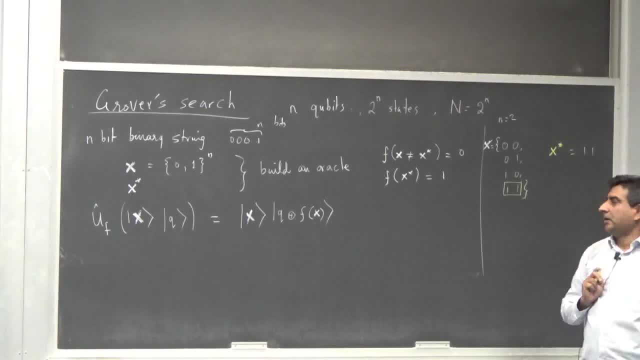 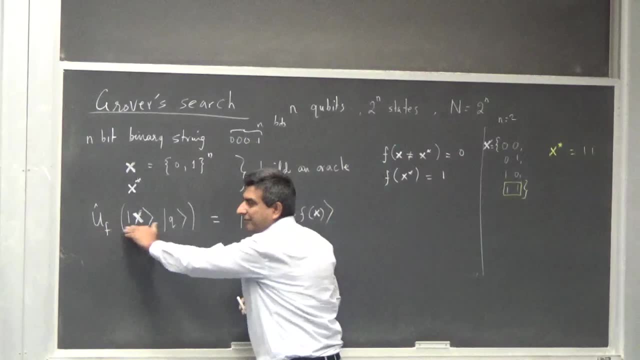 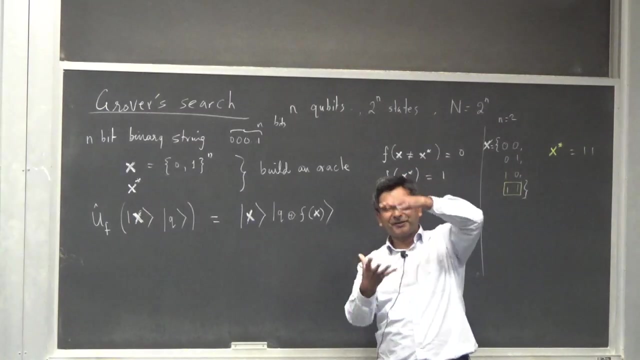 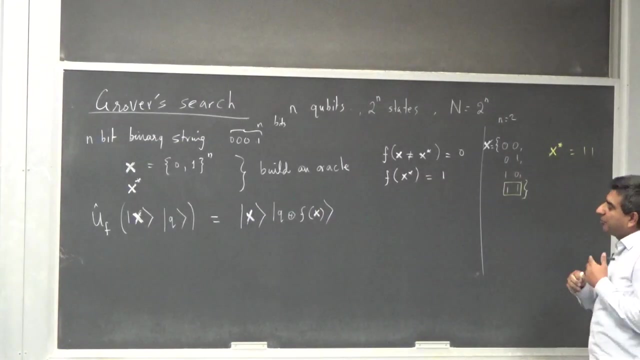 is my desired string. Now what I would like to do? so with this information, I would like to build this unitary operator That would be an oracle. So I have already built my quantum circuit that implements this oracle. Now, can you, for example, how many qubits? 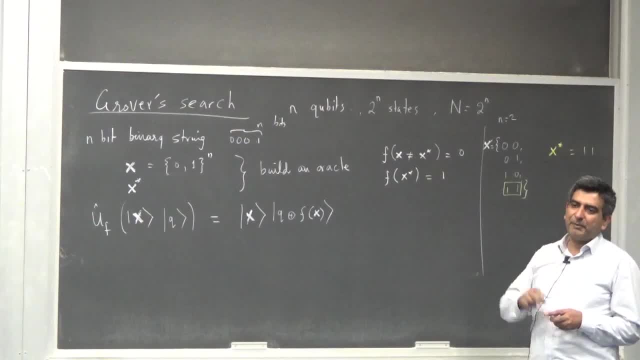 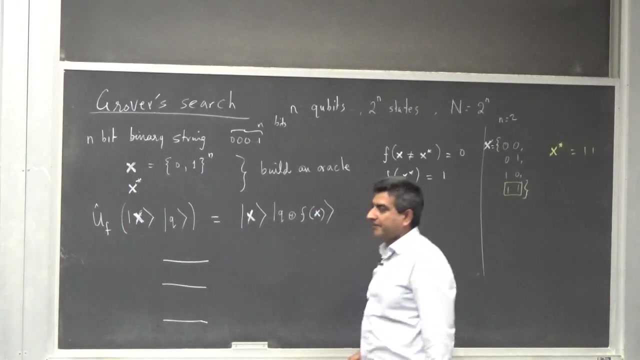 are now in this quantum computer? How many working qubits? How many working qubits do I have Two and one ancillary qubit. So I have three qubits. So I am now attempting to build a quantum circuit. This is my x right. So these two. 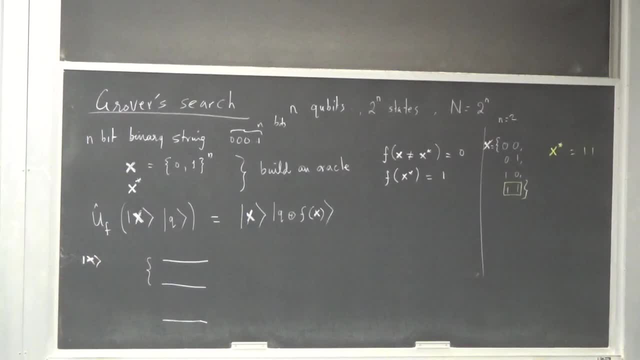 qubits represent my capital, my bold x. This represents my ancillary qubit, So I have three qubits. Now, if I were to, for example, build what kind of so? if you just look at this problem from a classical perspective, what should I do? I would like to have some. 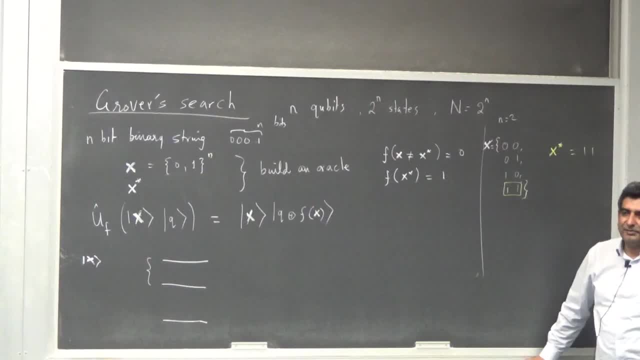 qubit that lights up, that gives me a signal that the two qubits that I am looking for, each of them, are equal to 1. What kind of logic gate would that be? So I would like to have an AND gate, But an AND gate has two inputs and one output, So I need two inputs. 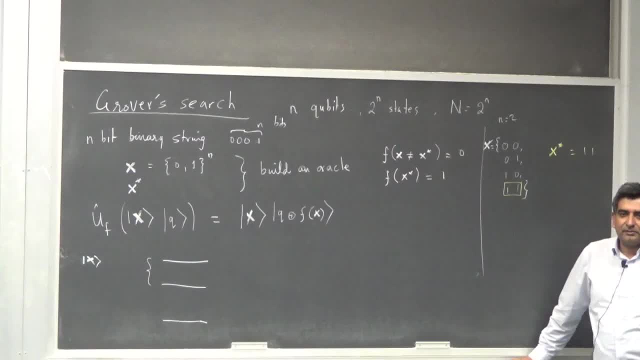 or two outputs, or three inputs and three outputs. So if I were to build a Toffoli gate, what the Toffoli gate does is that, if it has both of these inputs are ket 1,, ket 2, ket 3, ket. 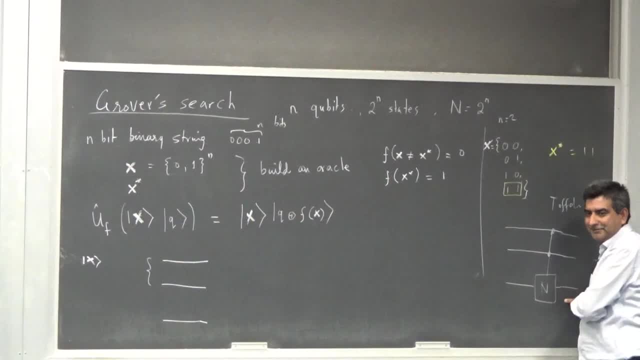 1 and ket 3, ket 3, ket 4.. That means that if that is, by the way, a appears similar, then this input will be inverted right. So it's a doubly controlled, NOT gate. So if this is cat 1,, this is cat 1,. 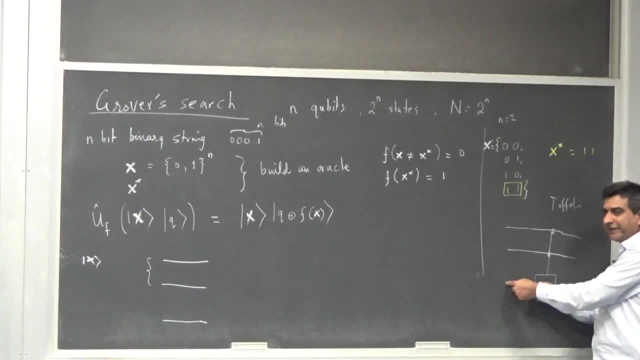 this third qubit will be inverted. So if I start this off in cat 0, this will turn to 1. If both of these inputs are 1. And by looking at this qubit I can tell that I have found my search. 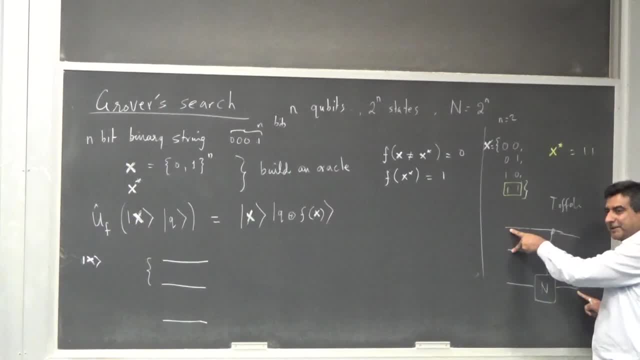 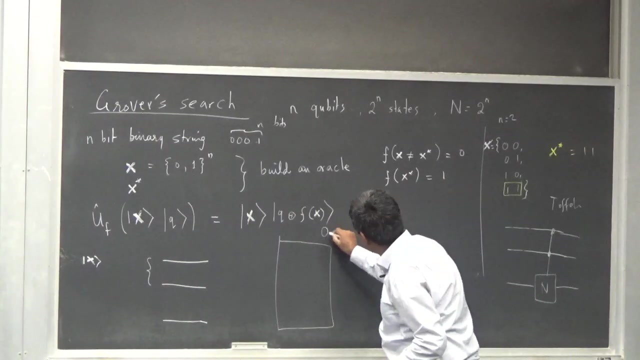 My search has been successful and the two qubits are in the state cat 1.. Right, So I would like to build a doubly gate. So my oracle. let's denote that oracle by o with sub f, because it's implementing this function f here, this one. 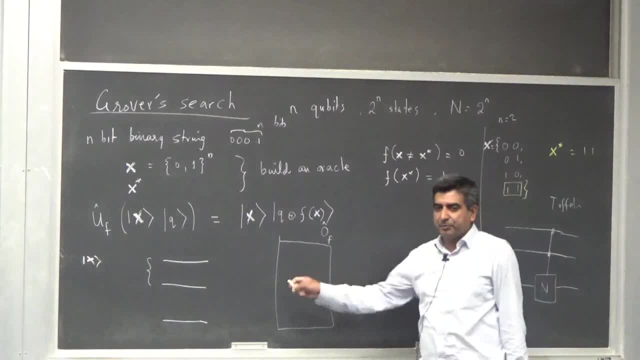 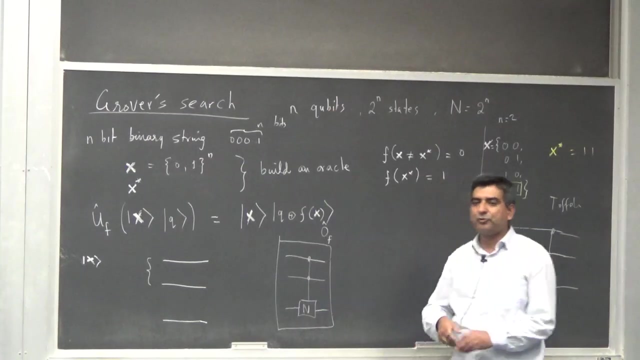 This quantum oracle is taking three inputs, Three inputs And it's really, it's really a doubly gate. So now I have one specific example of how to build an oracle. If I'm looking for 1,, 1,, this is what the oracle will look like. 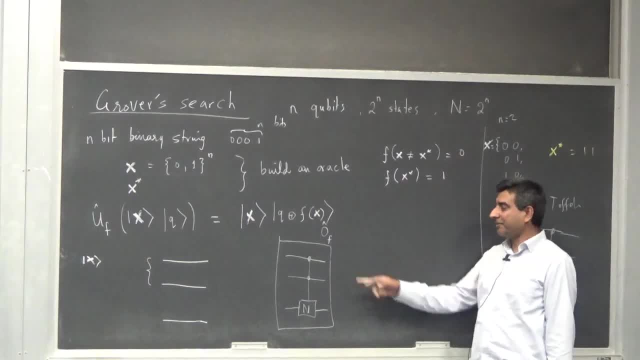 And if this bit is 1, it will flash that my two input states are cat 1 and I have found the solution. That's what an oracle means: It can determine, it can tell you, it can discern, it can discriminate. when you have reached the solution, 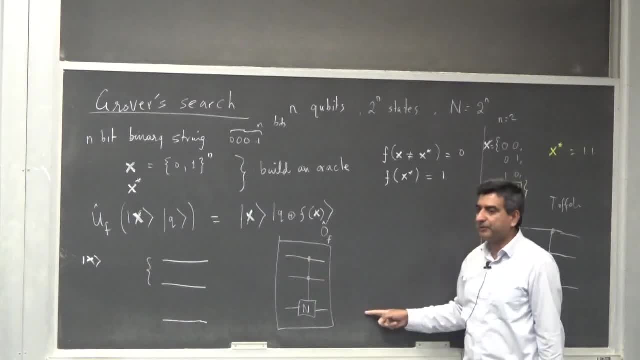 from other possibilities. When you do not have 1, 1 here, this bit will remain 0.. So the state of this qubit is going to tell you that you found the solution or not. So it can distinguish between. 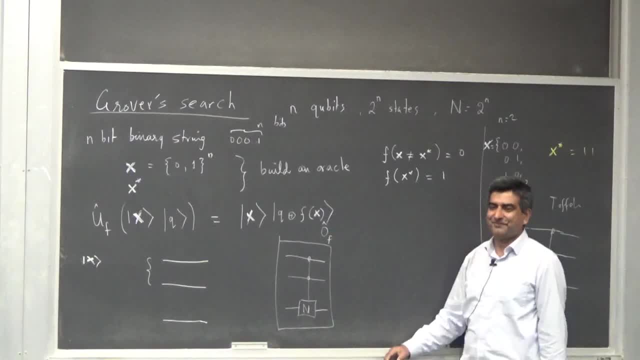 this circuit can distinguish between the solution and no solution. That's what an oracle means. Yes, 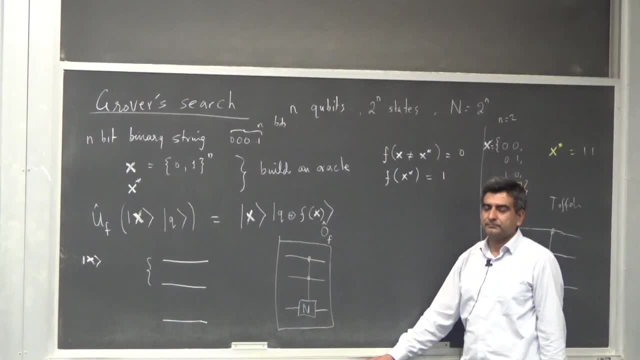 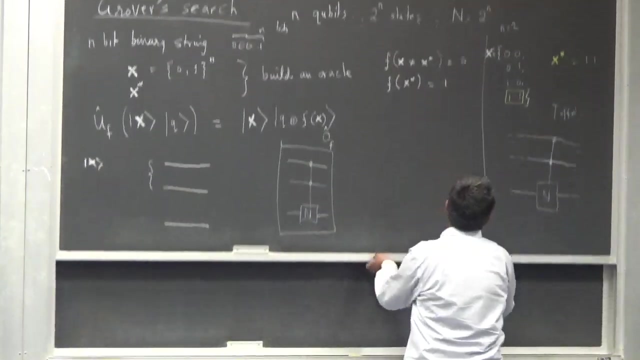 The both of them have to be: 1. Right, No. So if you look at the unitary gate for the Toffoli, the matrix for the Toffoli gate, U Toffoli gate. 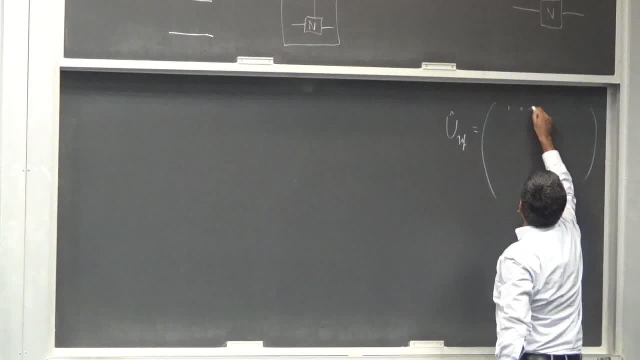 it's an 3, 8 by 8, matrix 1, 1, 1, 1, 1, 2, 2, 2, 3, 2, 3, 2, 1,. 1, 1, 1, 2, 2, 2, 2, 2, 2, 1, 1, 1, 2, 2, 2, 1, 2,. 2, 2, 2, 1, 1, 2, 2, 1, 2, 2, 2, 1, 2, 1, 2, 2, 1,. 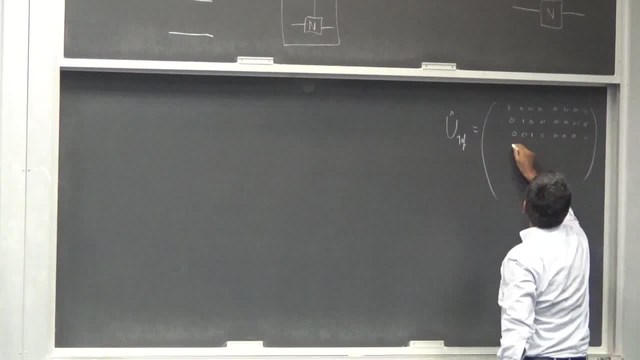 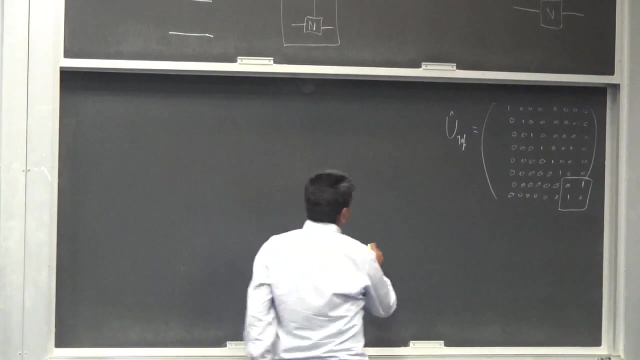 2, 2,, 2,, 2, 2,, 1, 2, 1,. This is what the Toffoli gate looks like. So in this block here, in other words, if you'd like to write the out-of-product formulation of this, 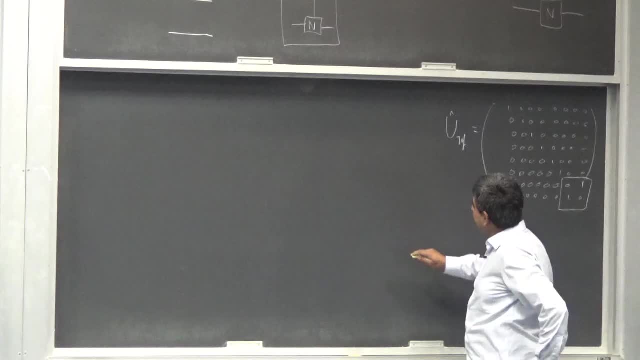 this is if this is what the Toffoli gate looks like. If the first and the second qubit are in state 1, each one of them is in state 1, you apply, not gate, to the third qubit, and if it's anything else, 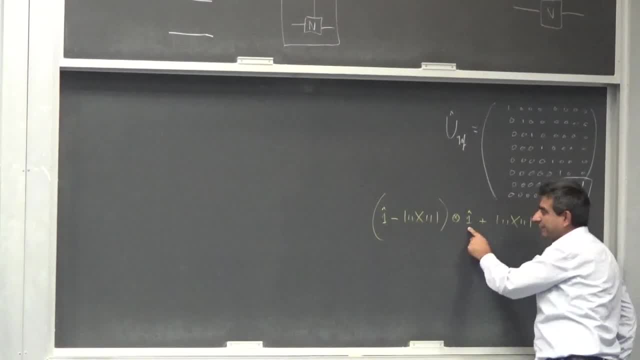 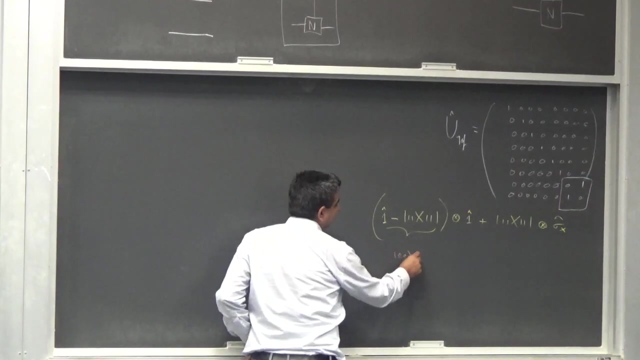 anything else, then you apply nothing to the third qubit. the third qubit just remains as it is. So this is just a shorthand for writing 0000 plus. so this really means this is just a shorthand for this out-of-product computation. 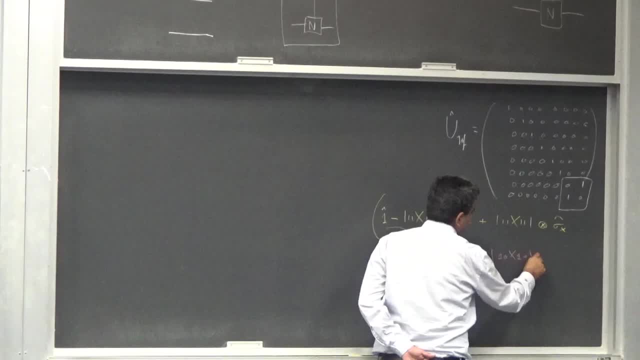 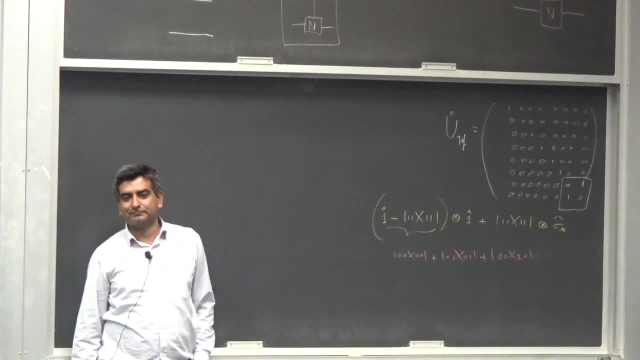 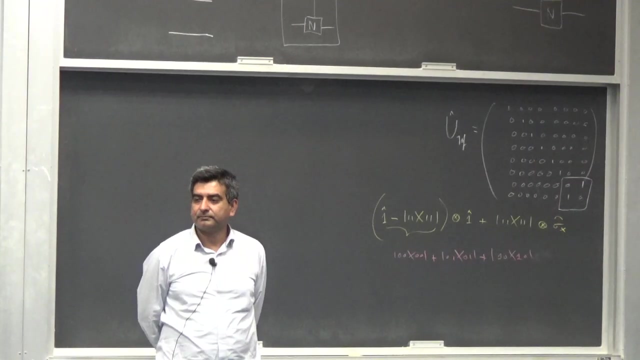 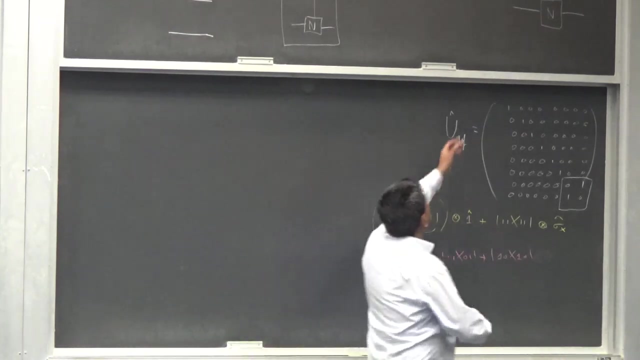 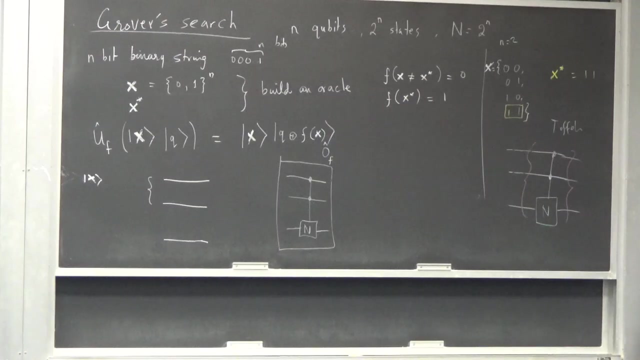 is a three input gate, three output gate. So this is a three input gate. this is a three input gate. It has one. I mean I do not understand your question. So there are three inputs here, three outputs. This is just a control channel. this is a control line. 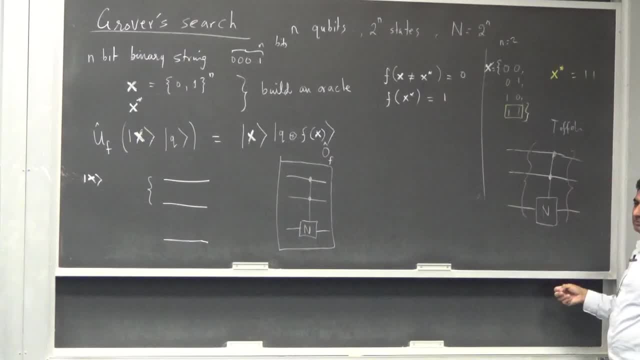 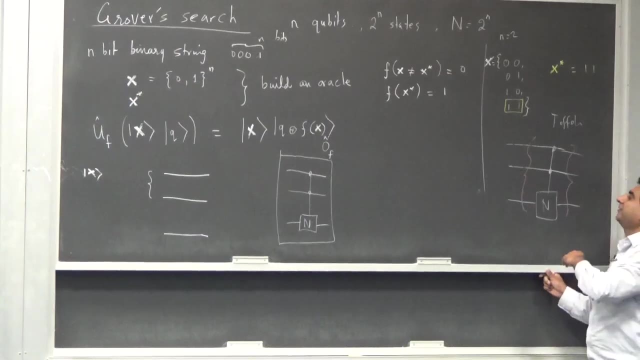 this is not an input. This is not an input. this is a control line. This is a control line, it is not an input. Look at the dimensionality of this. this is an 8 by 8 matrix: three inputs, three outputs. 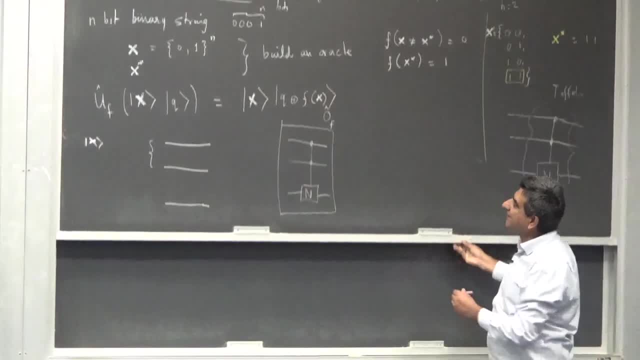 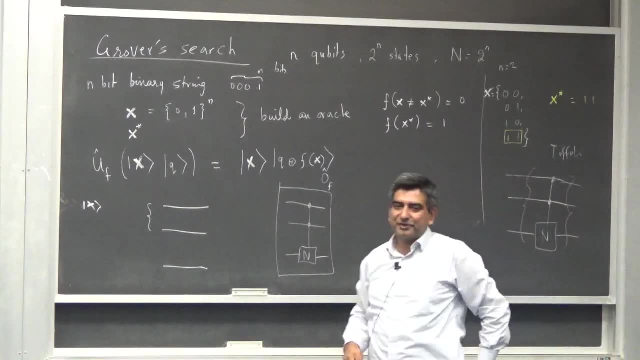 Anyway, I have to move on. So this is my implementation of the power clip. Now, what do I do? Just as in the Deutsch algorithm, I have to move on. So this is my implementation of the Deutsch algorithm. I would like to put a Hadamard here, a Hadamard here, and not. 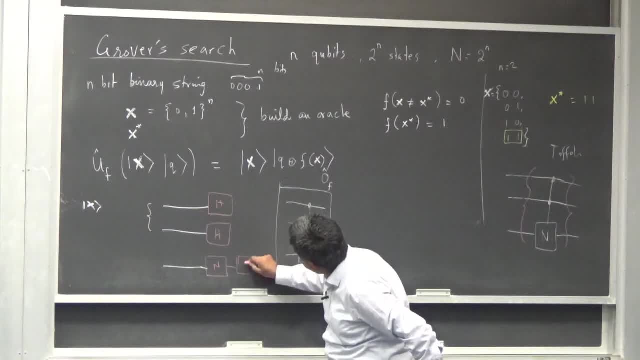 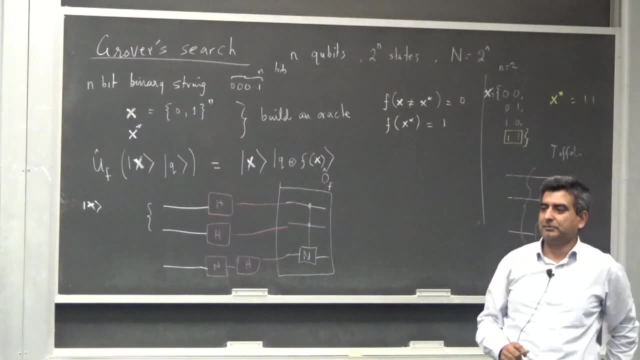 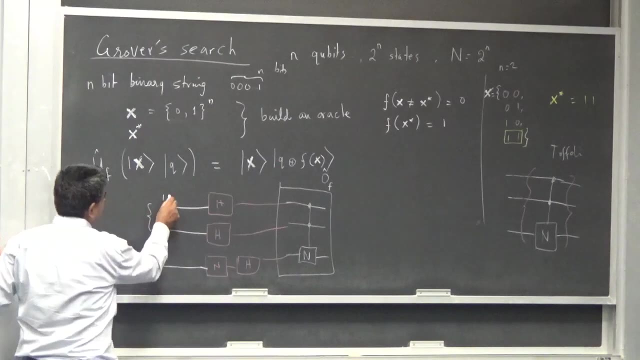 gate followed by a Hadamard here, And then feed this into the. This is general scheme of many quantum algorithms. You input in the computational basis get 0,, get 0,, get 0, zero. the ancillary qubit is inverted at one and then you have a Hadamard gates. 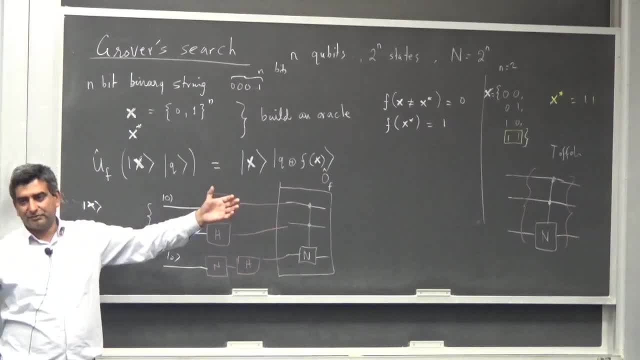 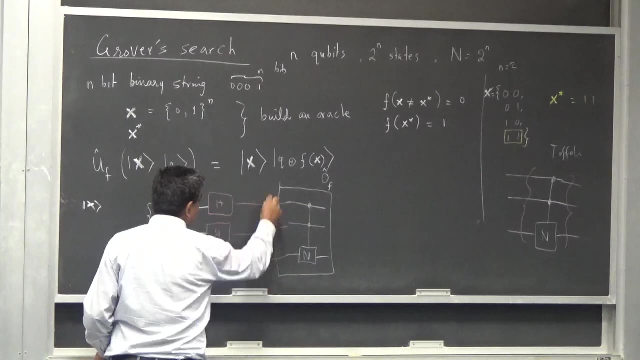 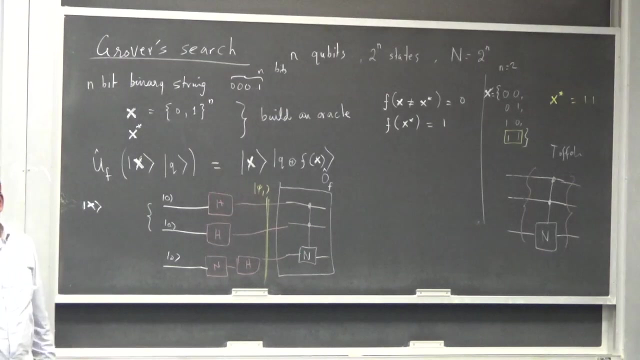 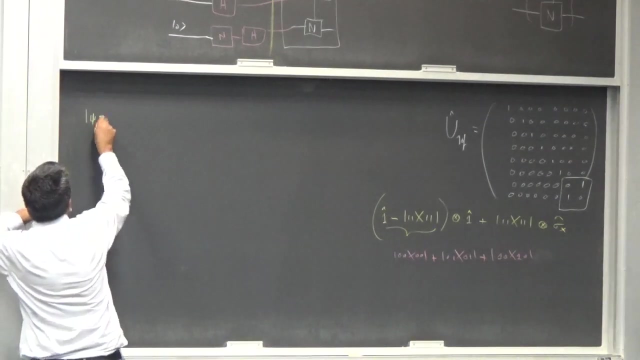 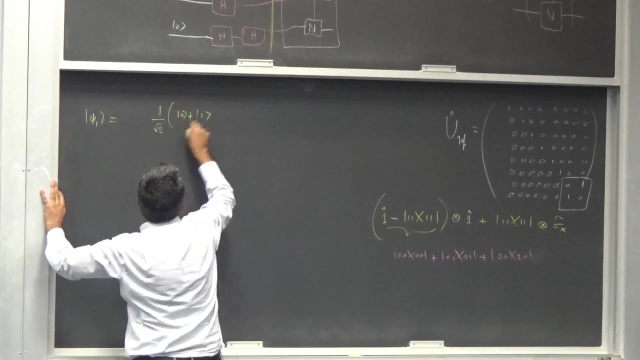 on each of the three channels and you create a big superposition and then you feed this into the Oracle right. so if you look at the state that is achieved over here, Doppler, yes, you want Good thing- is relaxable that limit over time. it's simply a super position of fund of the program and with the superposition, 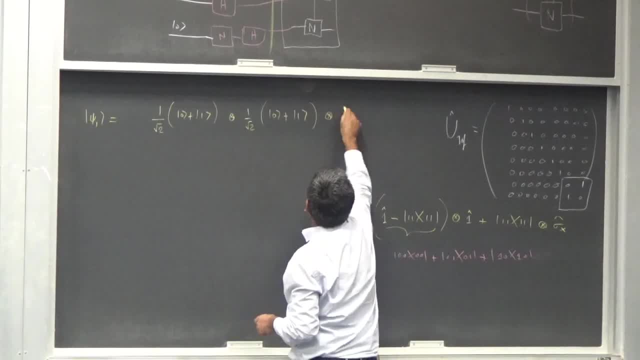 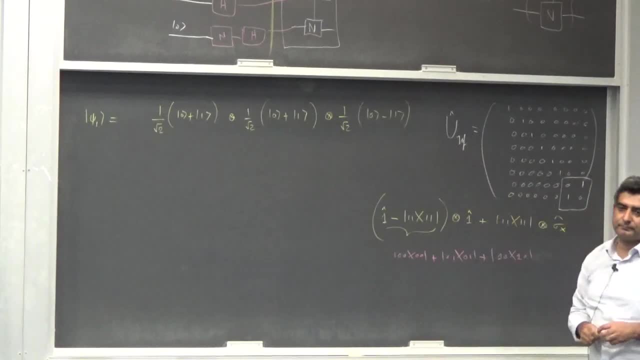 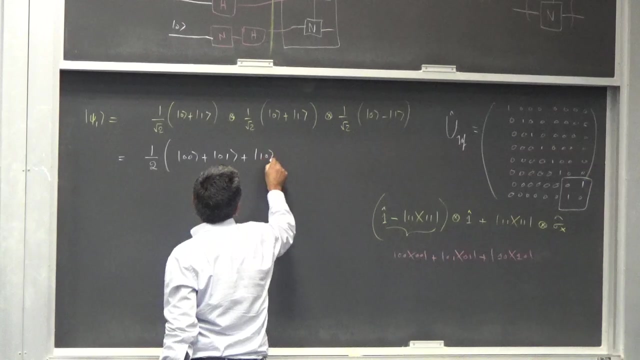 of the first but the first guide, that is这里 Europuhal Eugene. then, to touch on on the second qubit, tensed with the superposition on the third qubit, minus 1, correct, And if I were to combine the two first two qubits I will get 0, 0 plus 0, 1 plus 1, 0 plus 1,. 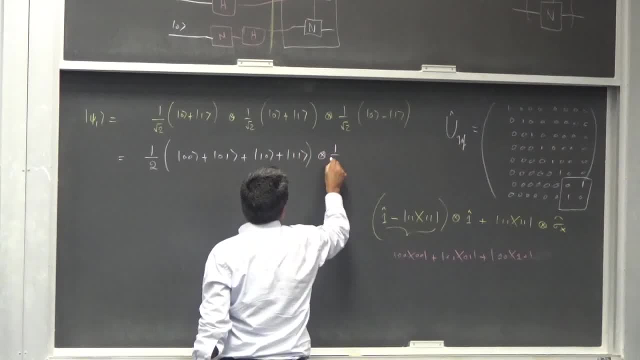 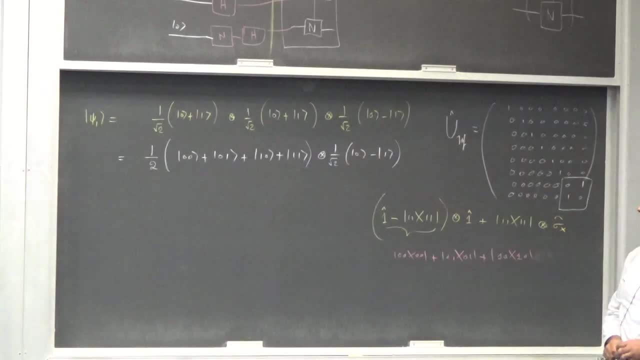 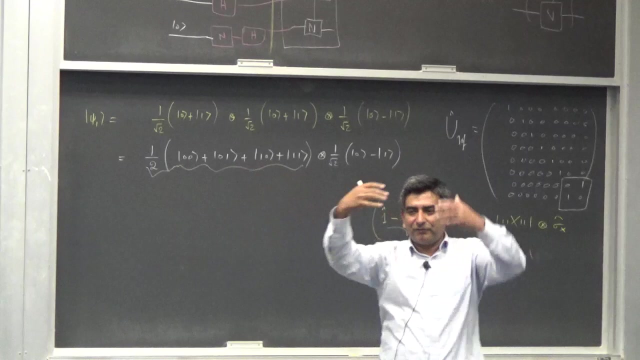 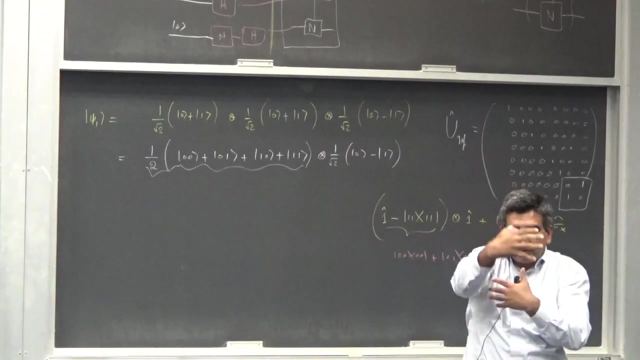 1, 4.. Now imagine this is an equal superposition. if you have two qubits, this is an equal superposition of all the four possible basis states, isn't it? Yes, An equal superposition of all four possible basis states. Just imagine the two qubits. 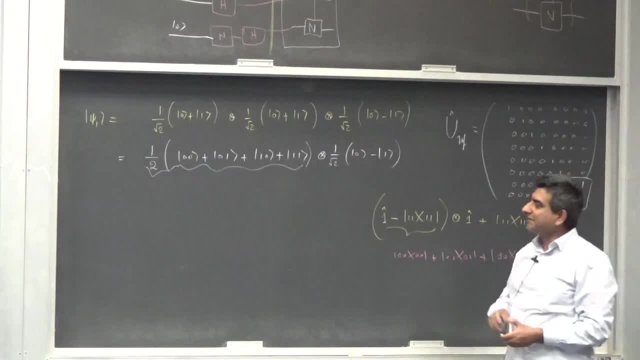 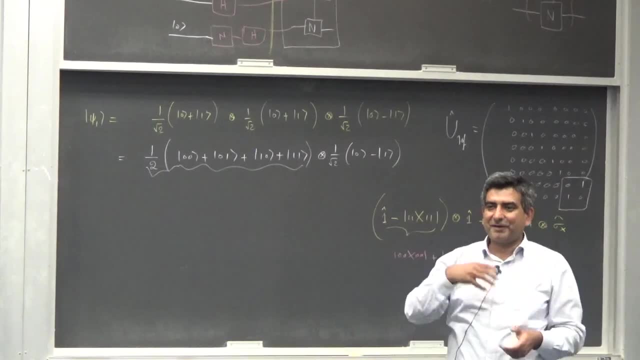 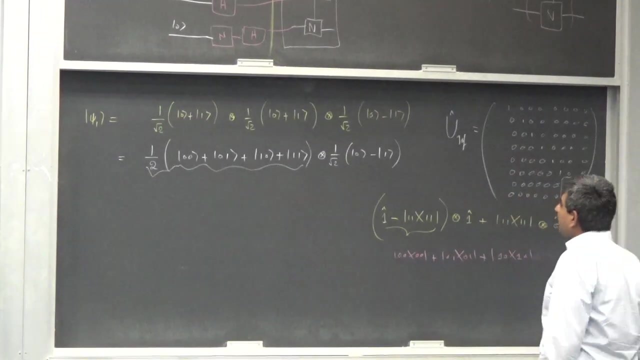 And it's separable from the third qubit. Now just imagine how the third qubit is acting very cleverly here. It's, in a sense, becoming a symptom and it's also becoming it's helping you in shifting the phases here and there. So now, what we would like to do is we would 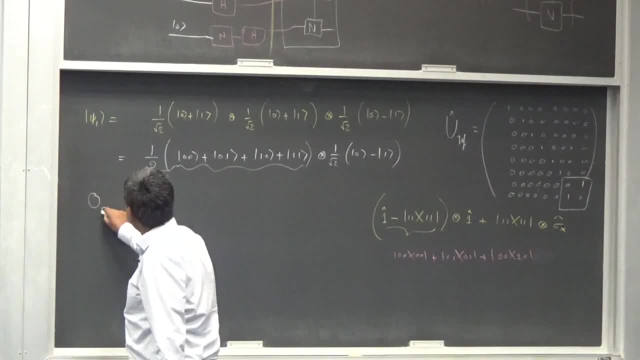 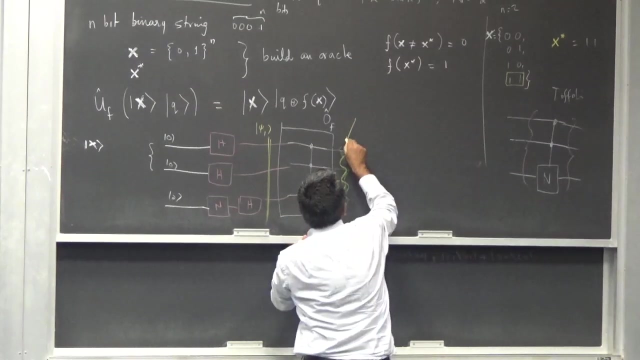 like to feed this into the oracle. Okay, So when it is fed into the oracle and I generate a new state, Psi 2,, let's call this state over here. Psi 2, comes out here. right, This is my state, Psi 2.. Now I would like to implement. 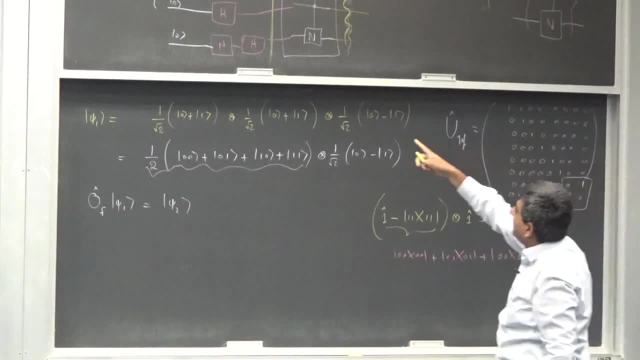 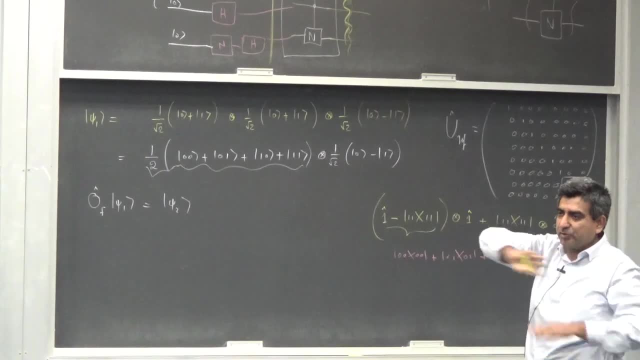 my function, which is over here. The oracle implements the function in that fashion. It's all. it remains reversible: The same number of input, the same number of inputs, and I of input, the same number of outputs. it does the logic gate, which in our case is the Toffoli. 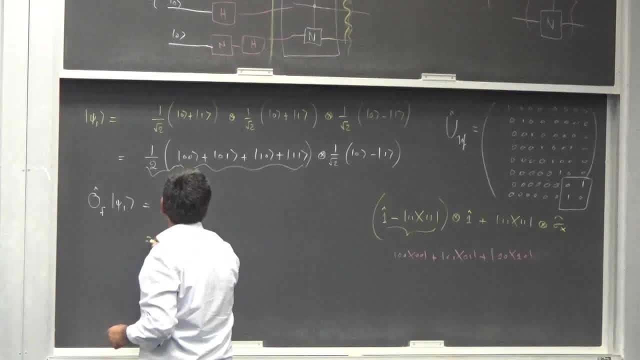 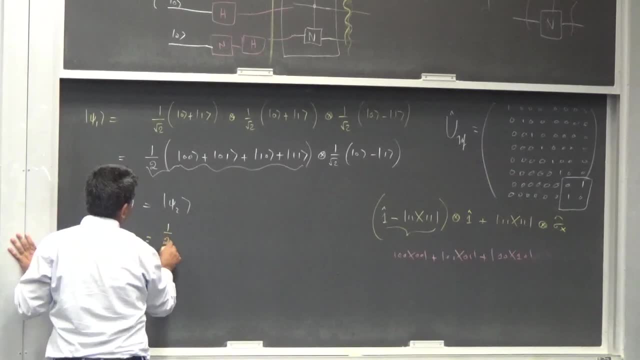 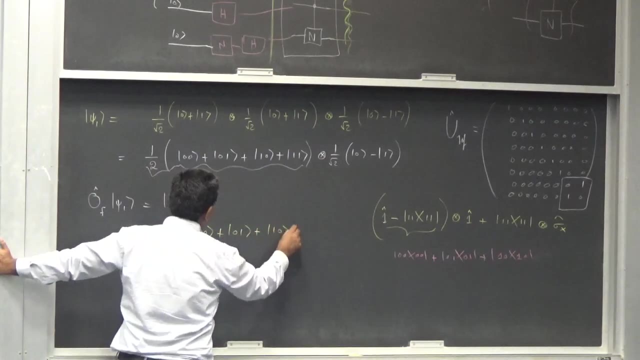 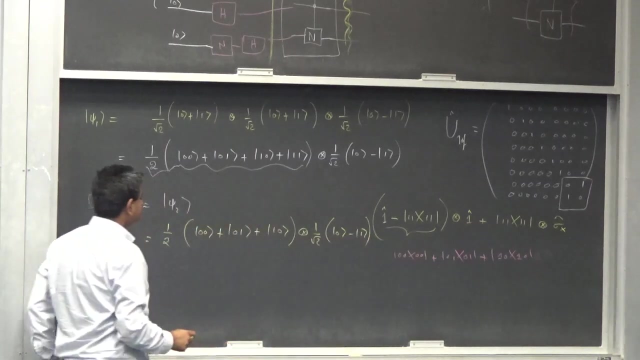 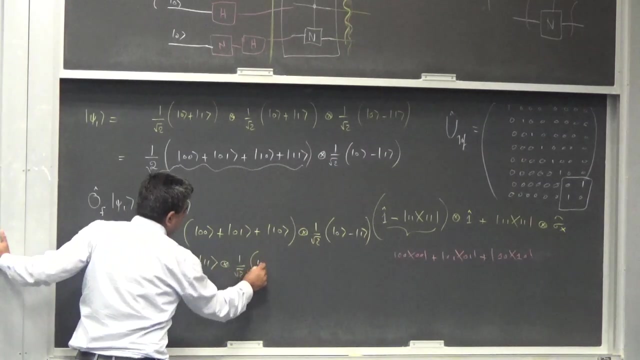 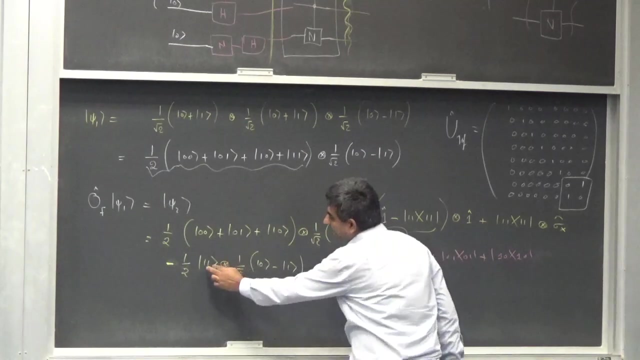 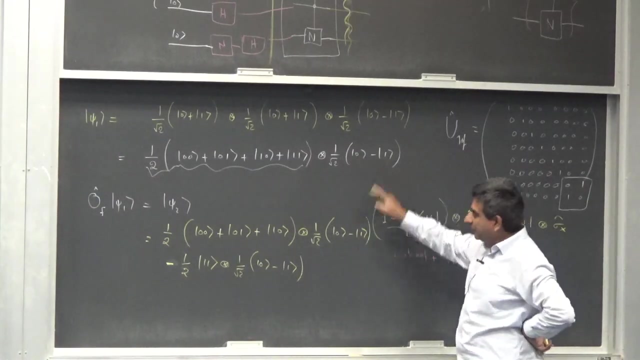 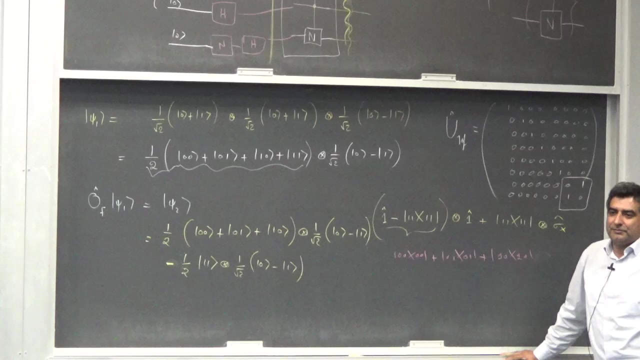 gate and you just apply the Toffoli gate over here, our output is going to look like the following: one half. So when the first two qubits are in the state ket 1,, this changes to ket 1,. this changes to ket 0, so this is inverted. so I put a minus sign over here, got it? 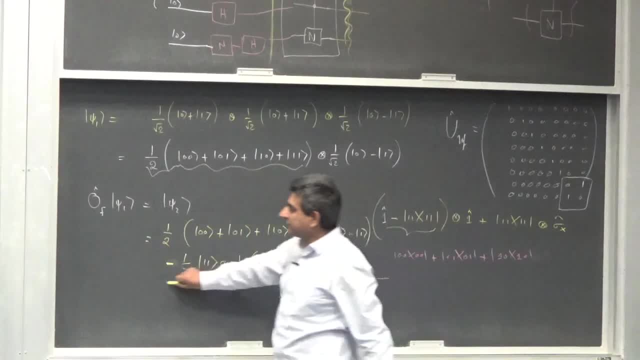 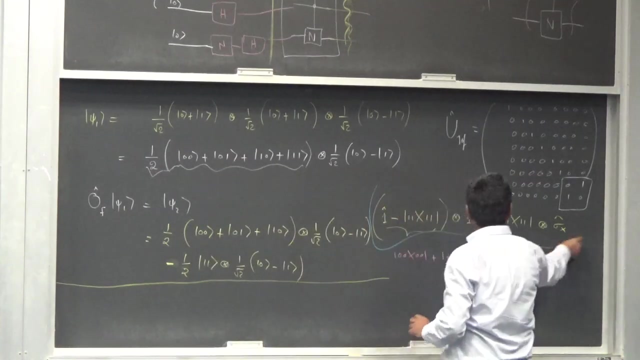 So I gave you one or two minutes to think about this, whether you understood this step or not, So, So, So, why do I have a minus sign here? So remember that this is a different thing, right? This is a different piece of information. 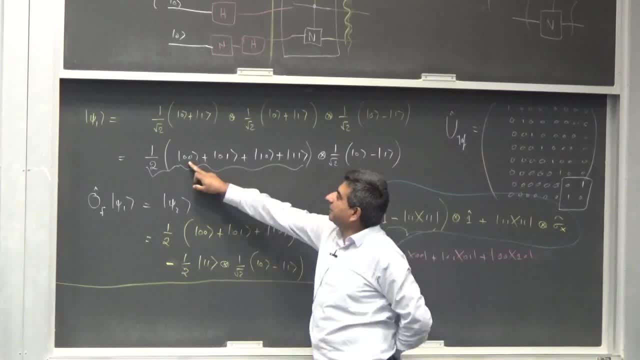 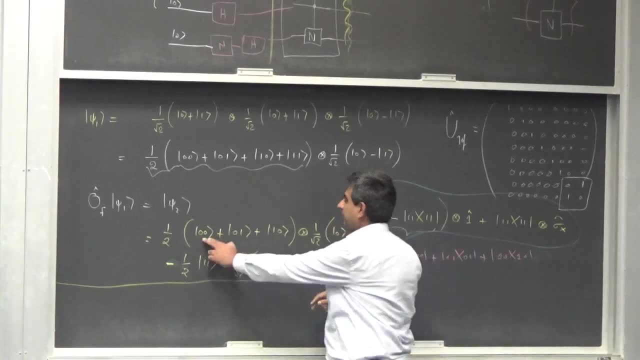 So if I expand this, if this is these are my two qubits- 0, 0, nothing happens to this. the third qubit: So this is 0, 0, 0, minus 1,. if this is my first two qubits, nothing happens to this. 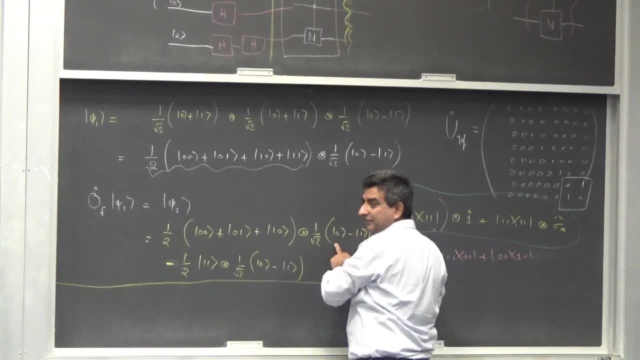 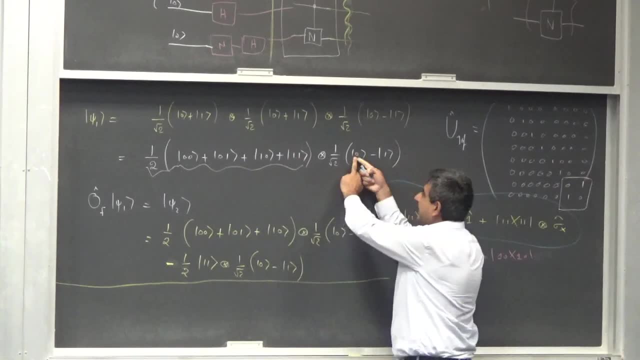 qubit. If this is my state, nothing happens to this qubit. but if my first two qubits, each one of them is in the state 1, this ket 0 becomes ket 1,. this ket 1 becomes ket 0, so ket 1 minus. 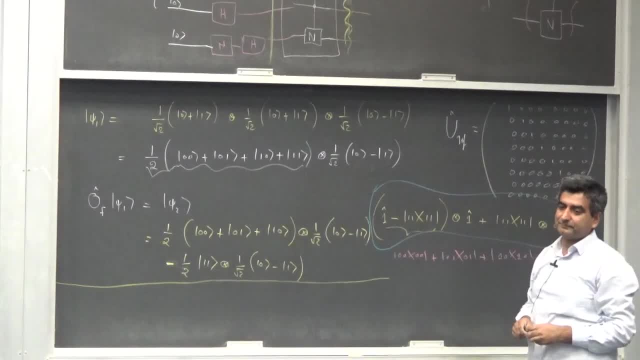 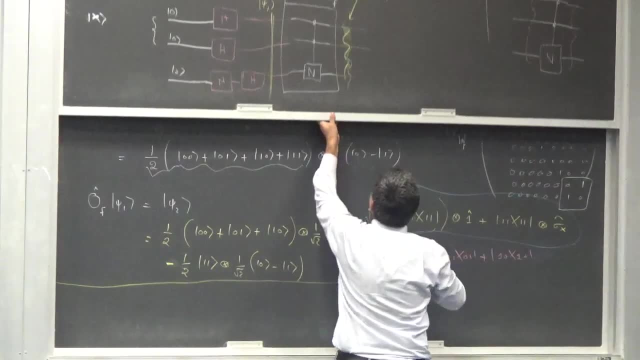 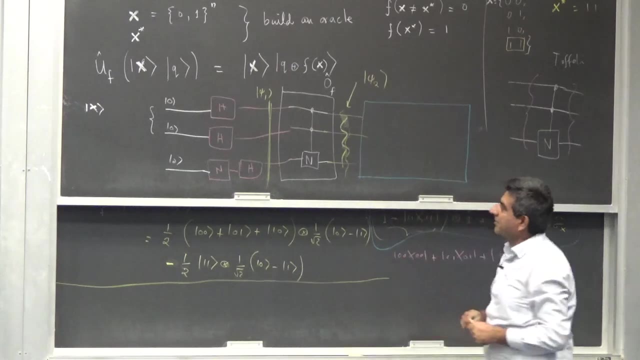 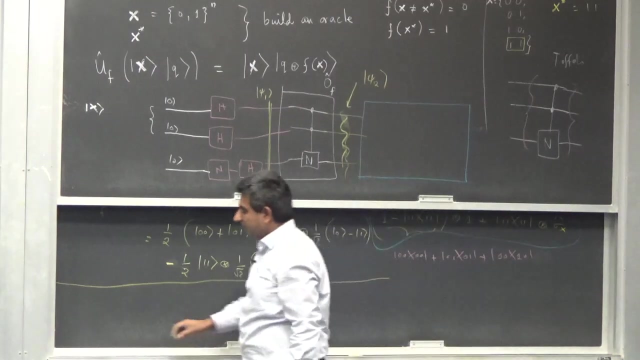 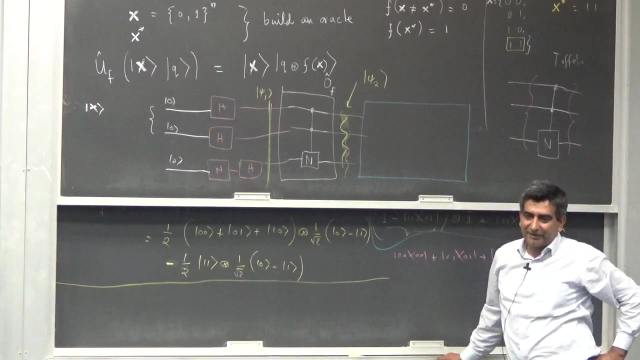 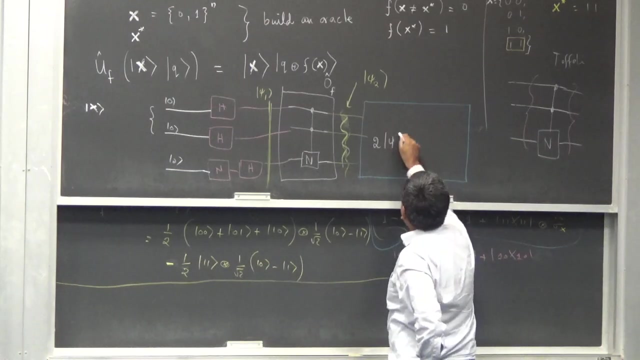 so I just put in a minus sign over here. Now what I would like to do? I would like to do something more advanced here. I would like to implement a function here, an operator here. That operator is given by two times ket, psi, bra, psi, minus identity. 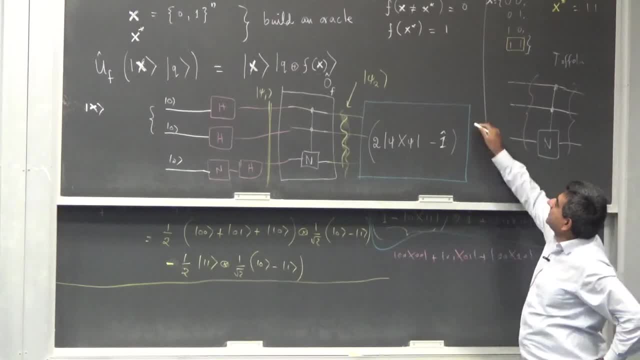 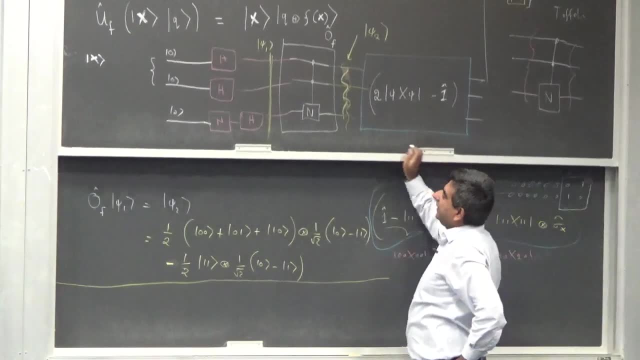 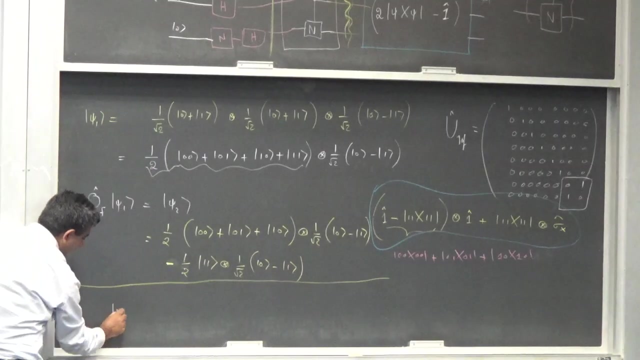 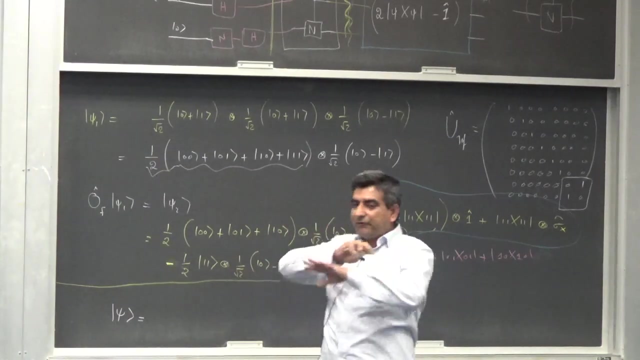 So let's figure out later how do we implement this and what is psi? my psi is is an equal superposition of all the basis states. Now forget about the Ancillary qubit. I forget about the Ancillary qubit. 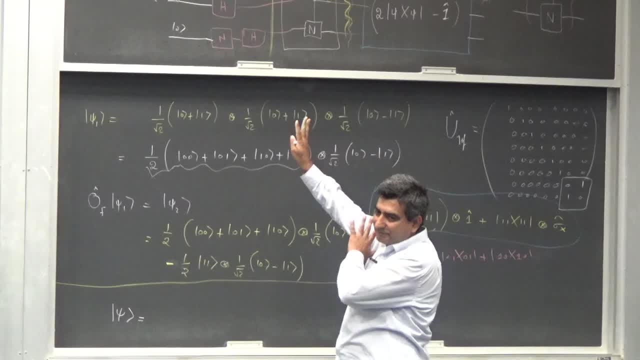 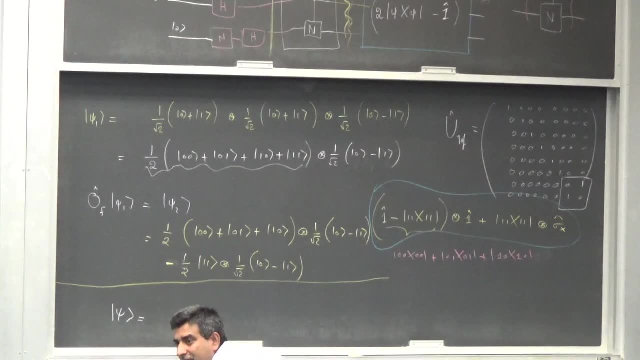 I'm just looking at the first two qubits. my psi is defined as an equal superposition of all the four basis states: 0, 0, plus 0, 1, plus 1, 0, plus 1, 1, over what should be the normalization factor here. 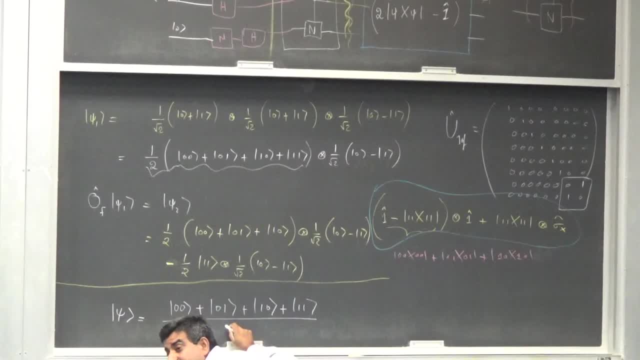 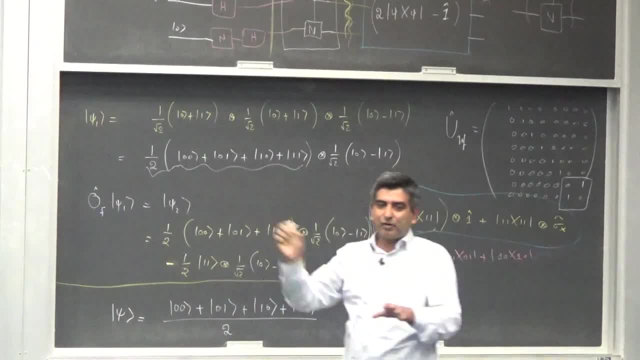 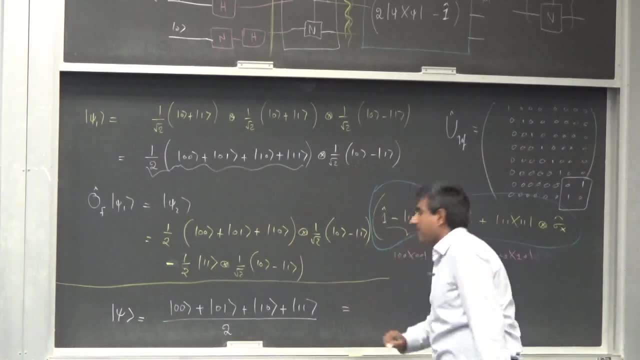 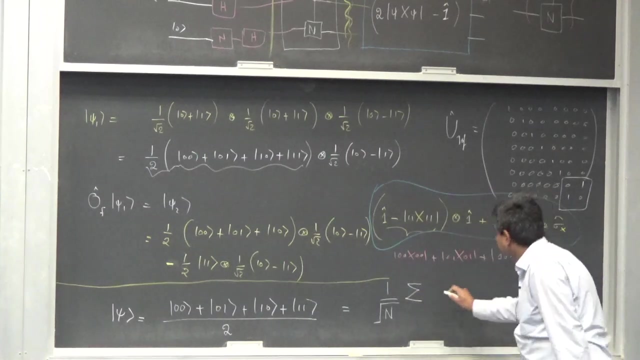 Under 2? Under 2? Under 2?? So this is an equal superposition of all the four basic states. In short hand, I could write this as: 1 over under root n, where n is 4, capital N is 4, sum over ket i, where i goes from 1 to capital N. 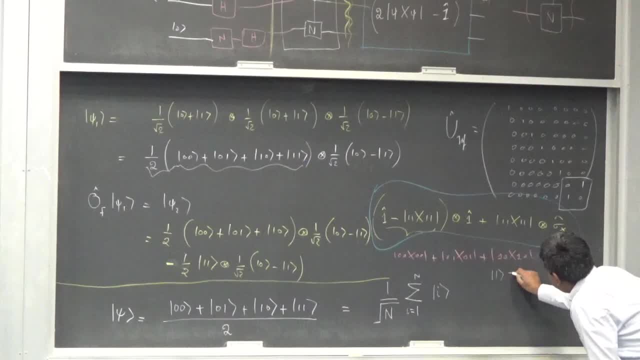 And ket 1 is defined as 0, 0.. Ket 2 is defined as 0, 1.. Ket 3 is defined as ket 1, 0.. Ket 4 is defined as ket 1, 1.. 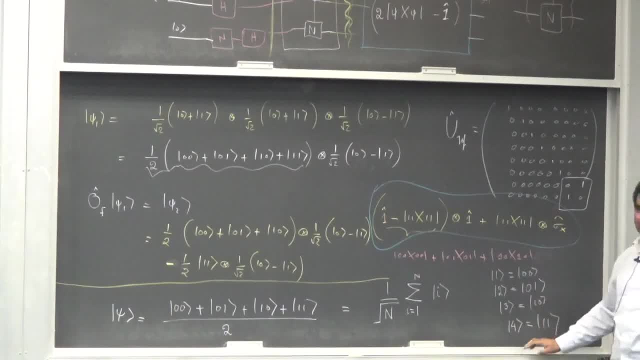 So I am just giving integer labels to these four basic states. Now let us see what is the action. So this is the action. So this is the action. So this operator now acts just on the first two qubits. 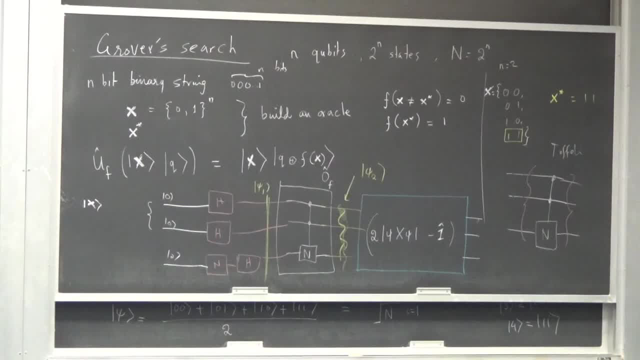 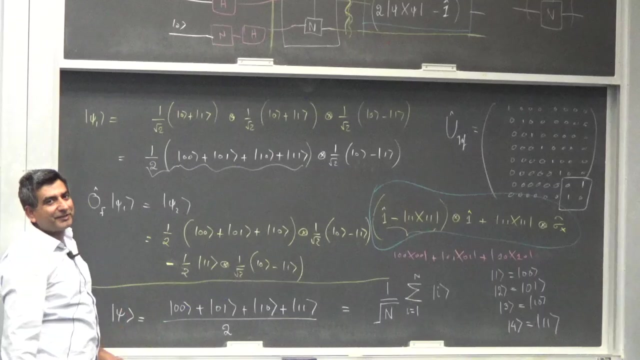 I do not care about the answery qubit any longer, So it just acts on the first two qubits. Now what does this operator do? This looks like a strange kind of operator. Let us see what is the action. 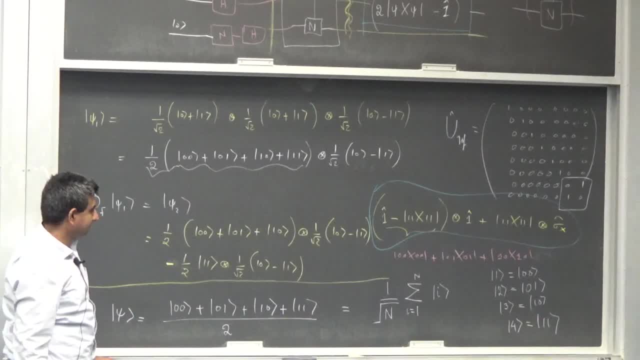 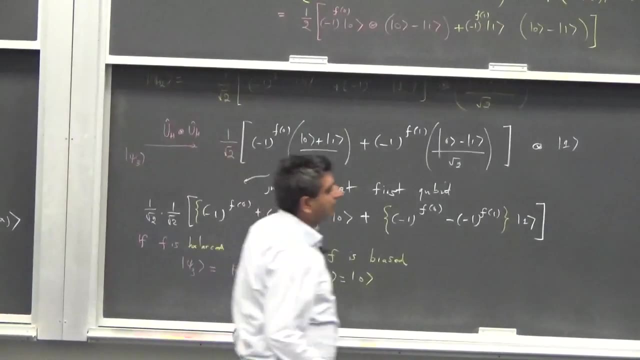 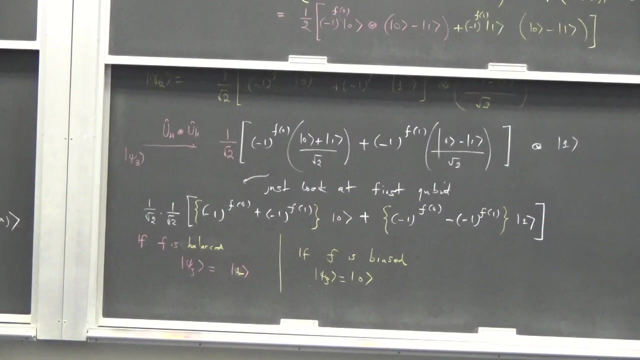 What is the action of this operator? I am defining an operator. I am defining this operator. This is some psi. What is this psi? That is how I define this psi. This is not psi 1, psi 2.. It is just something. 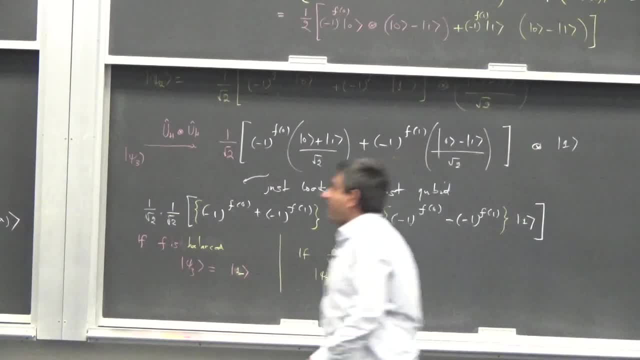 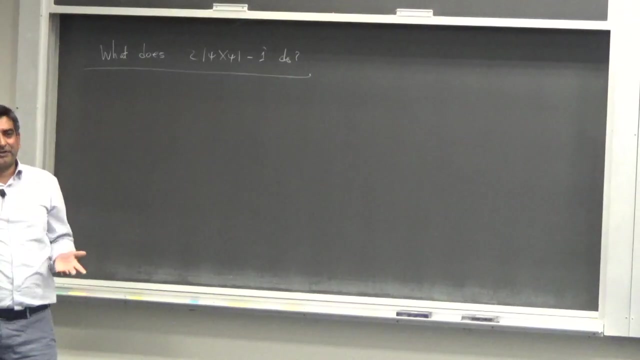 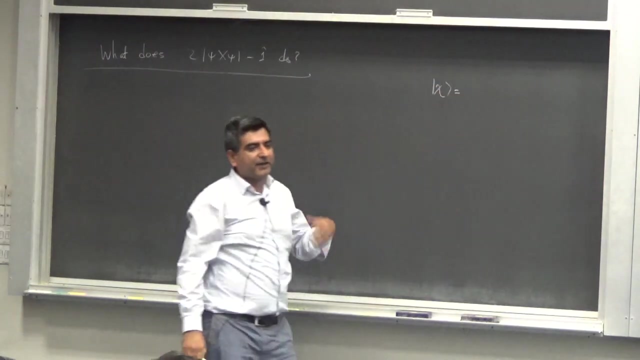 side good point. so what does to get side drops? I, minus identity, do. so let's see what is the action of this operator on an arbitrary input state. let's see what this function does. so if I take an arbitrary input state guy, how can I define an arbitrary? 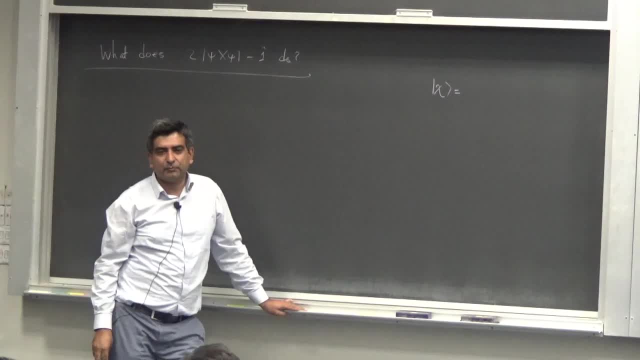 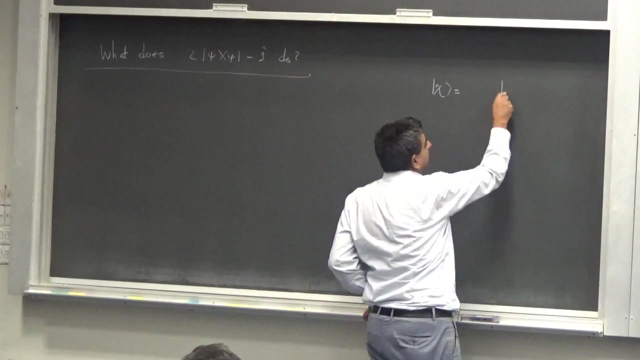 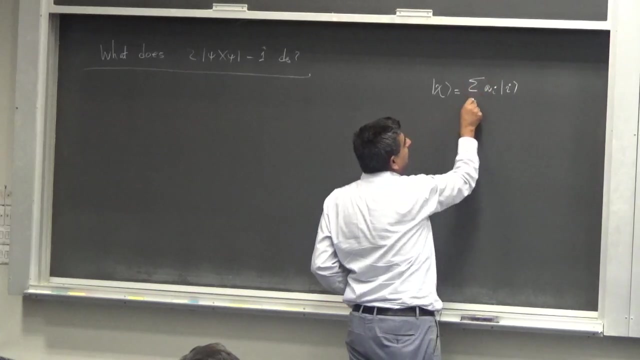 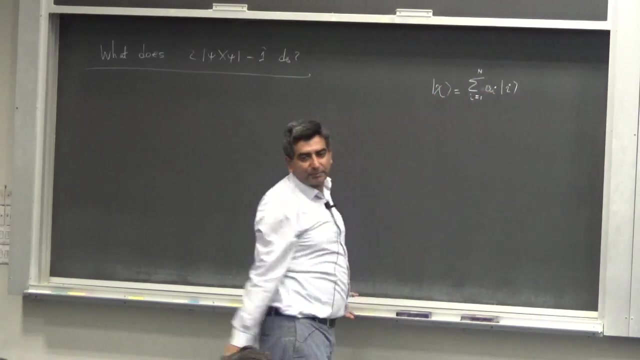 input state that what's the general form of guy? so it's, and it's small, n qubits now. so it will be: sum of all. the head is with some amplitude right, you know, aizer complex numbers, correct? that's an Martino state. now let's see. 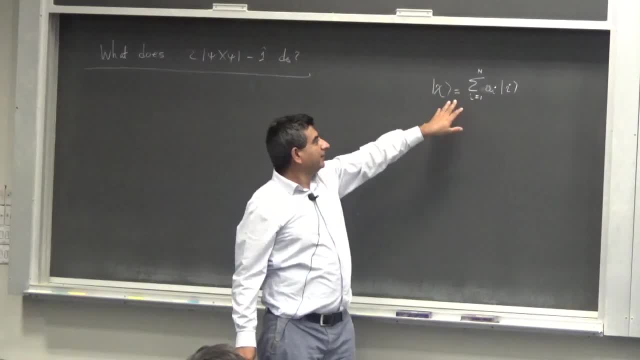 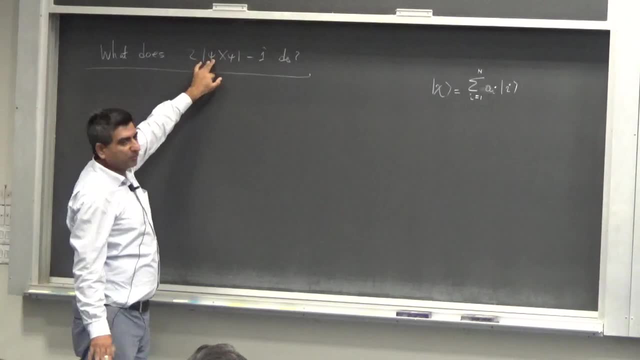 what is the impact of this operator on this page? now, this is the state, it's in cat form, it's a superposition. all Sherman, the bias is all the gab presents. let me recommend now in allлу船 of cat. so it is a state. is this an operator? yes, because it's an outer product, a cat, the. 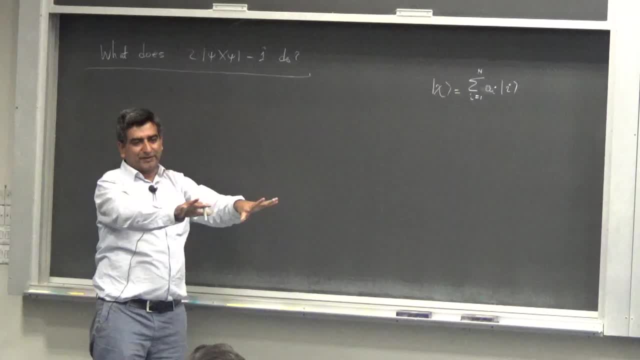 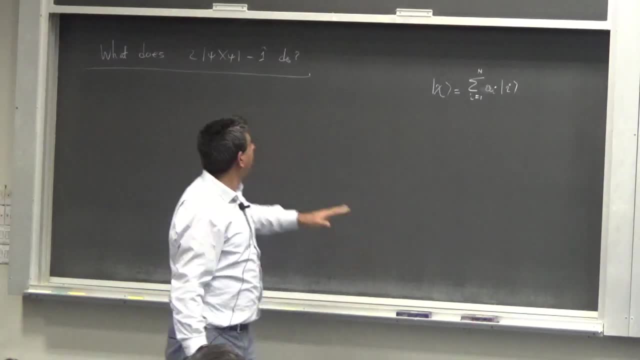 bra, so it is an operator. the identity, of course, is an operator, so this operator is now acting on some arbitrary input state. so we're just going to find out what the action is of this operator on an arbitrary input state and then we'll come back to the Grover algorithm. 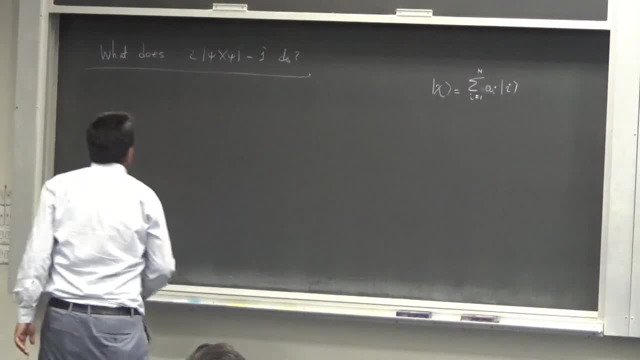 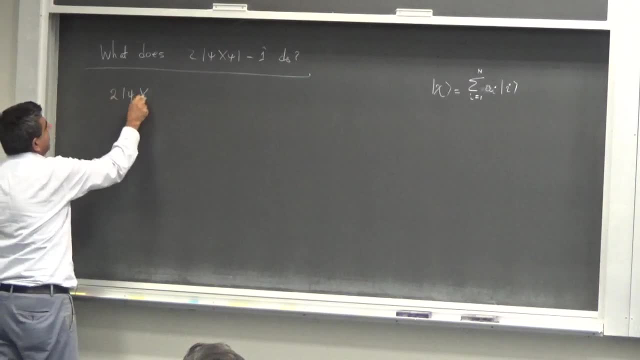 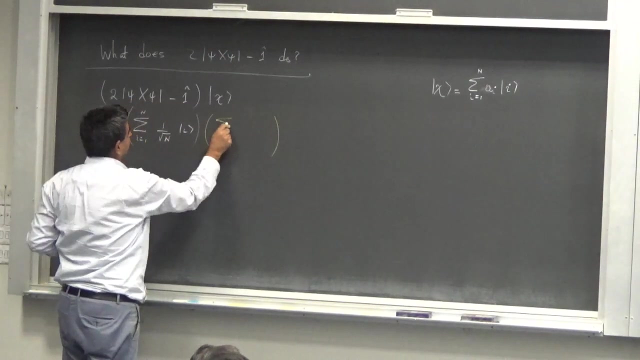 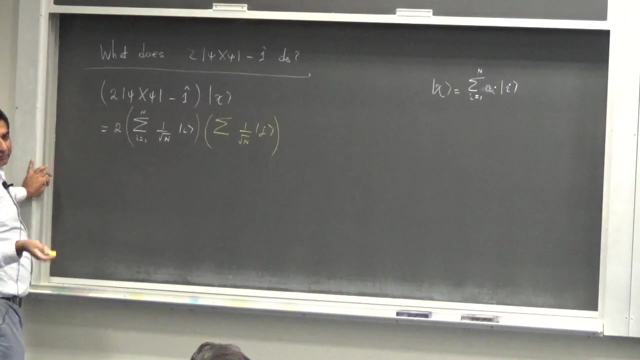 all right. so if I just look at the operator acting on guy, so this guy is given by 1 over and root n get I. now the corresponding bra is given by 1 over and root n. I just use a different label now: J instead of I use J. I can't use I here. I have to use a different index here. this is: 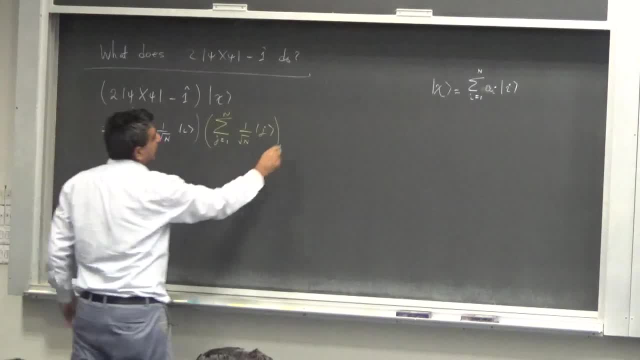 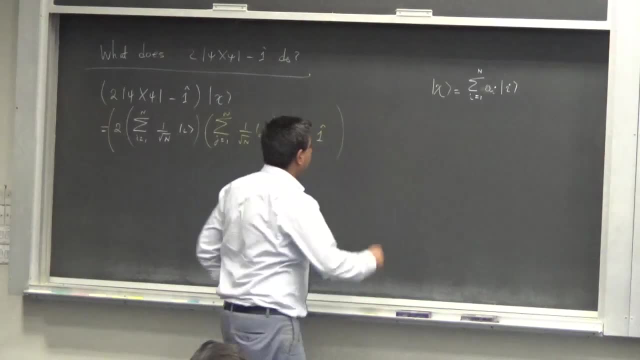 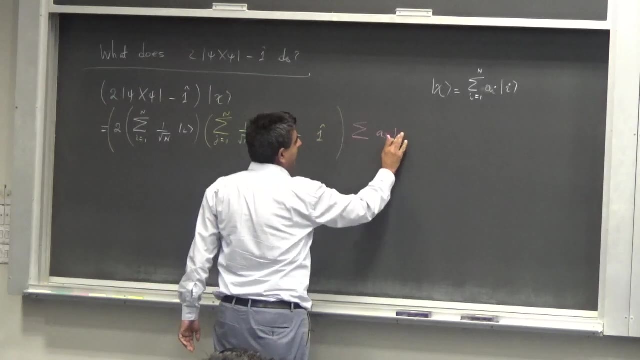 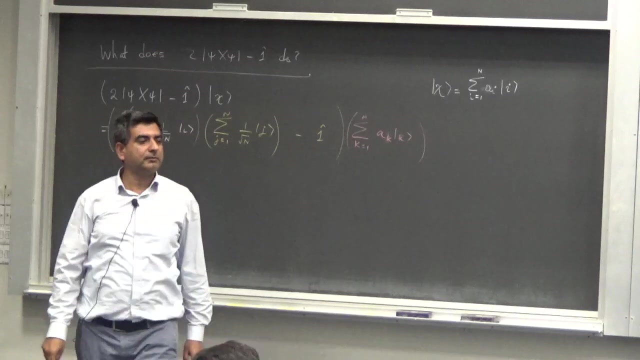 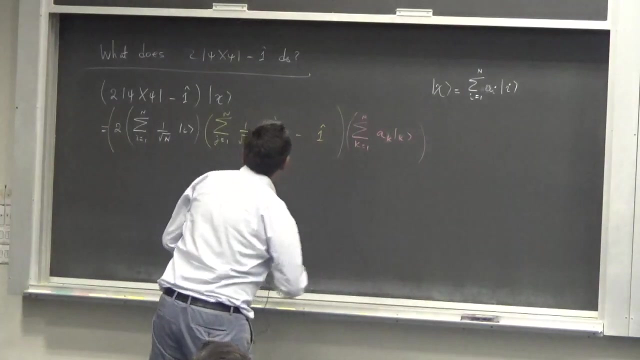 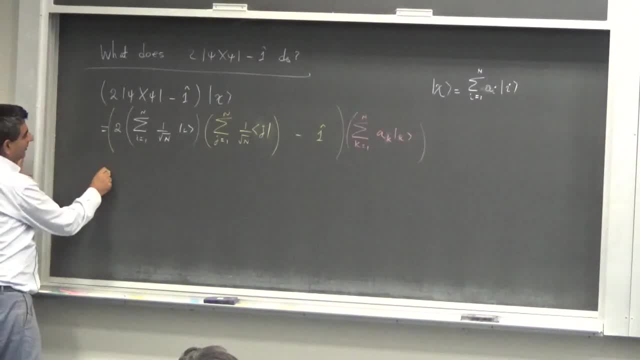 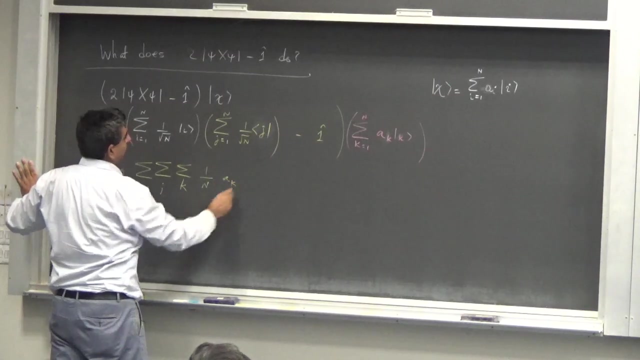 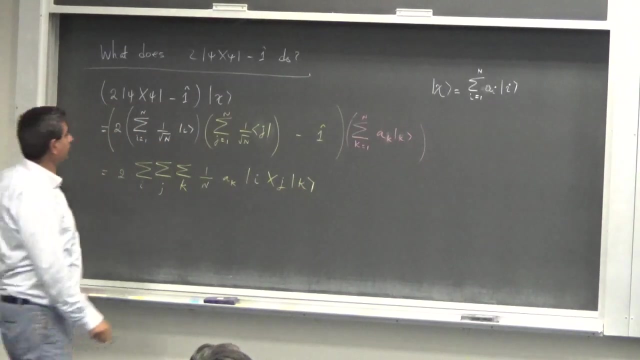 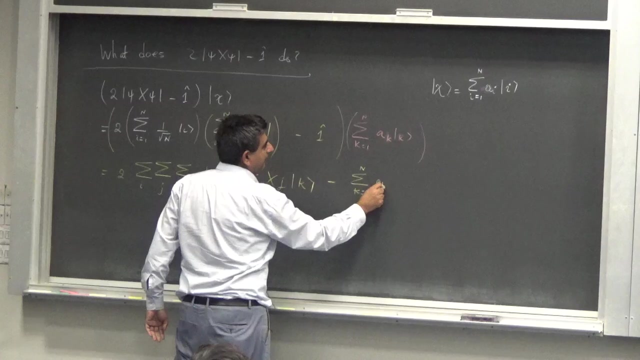 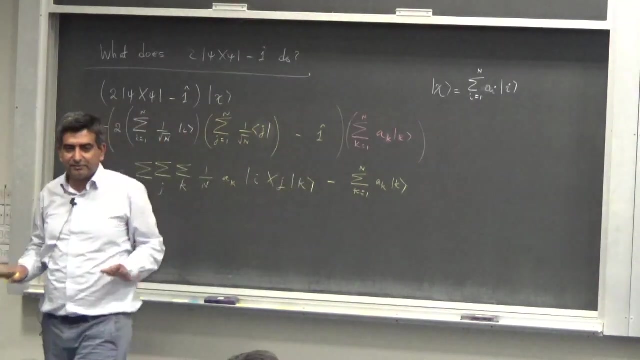 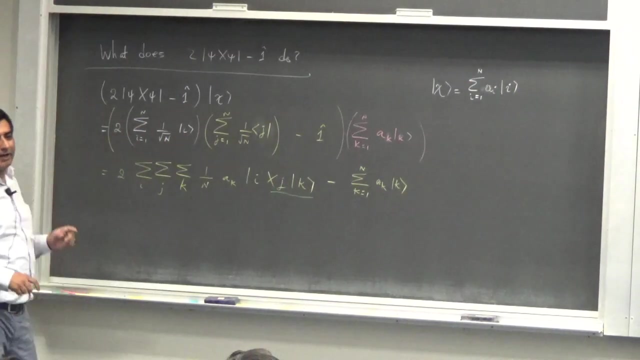 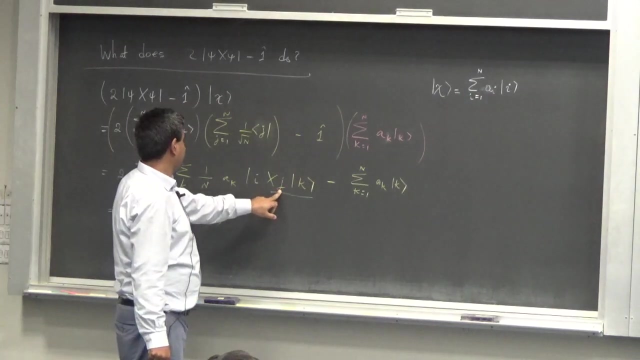 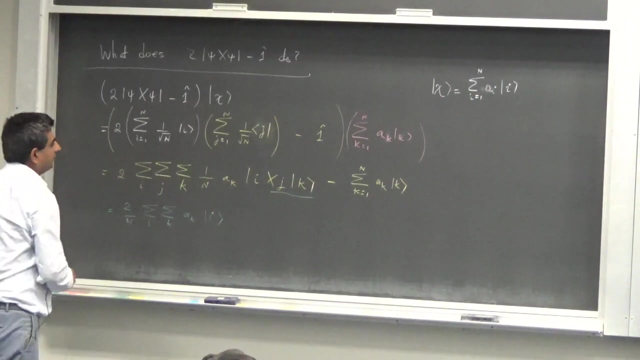 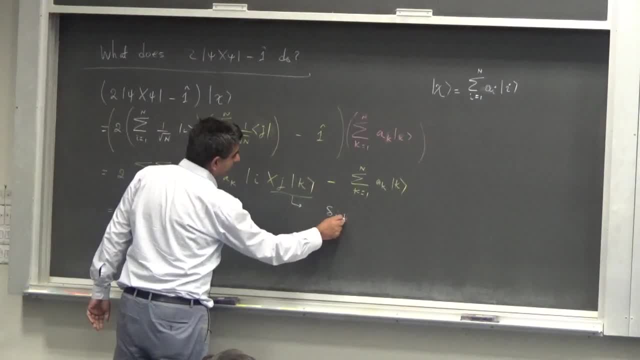 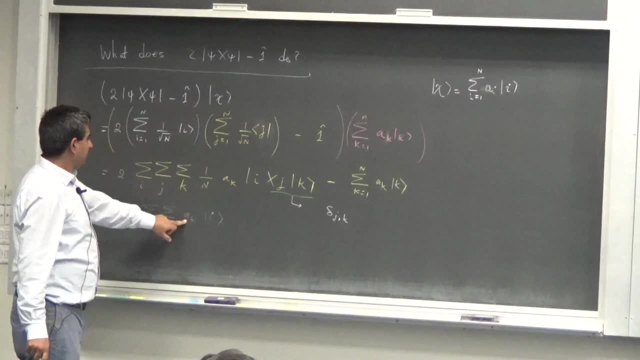 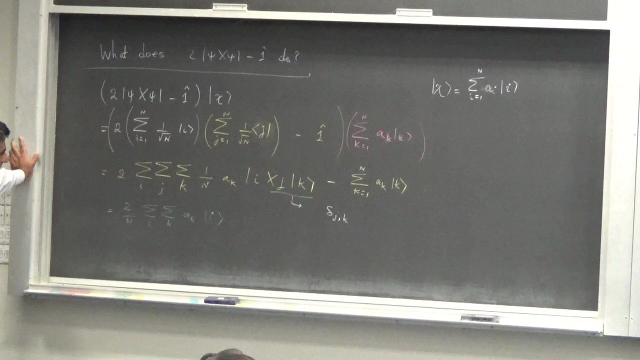 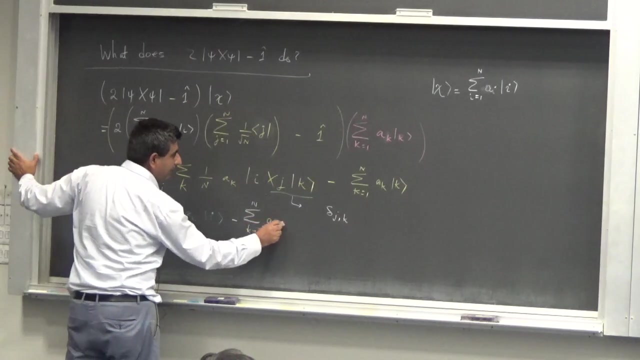 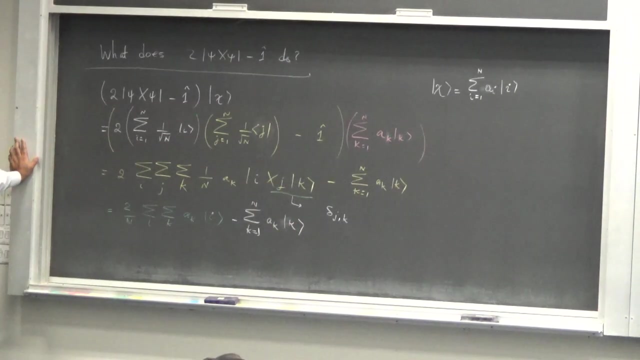 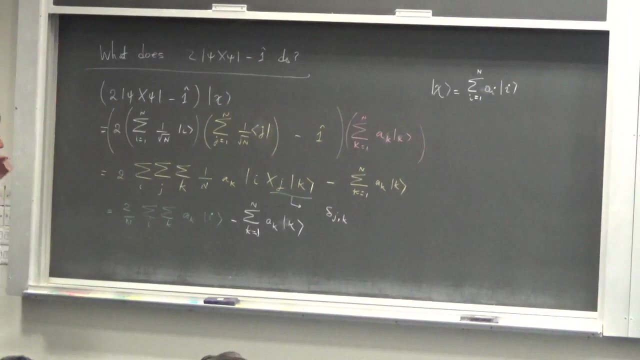 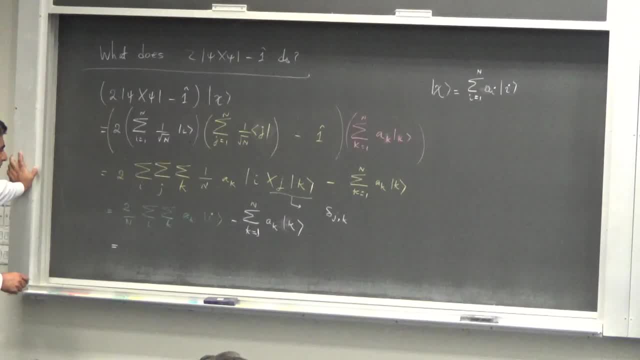 this is 2 over n k k over j. Full. Here we prove that 2 over n k k over j is like this. So here this shape. here is 4 over n k k over j. Check this Here: this is 3 over. 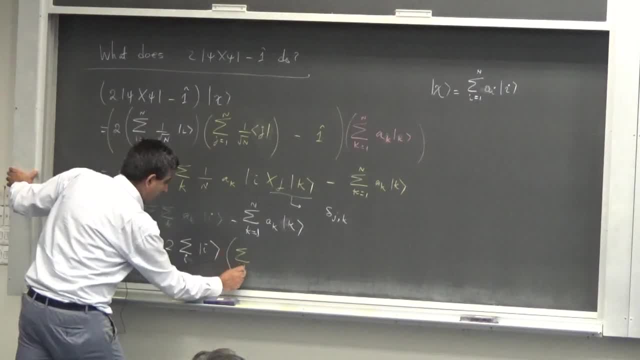 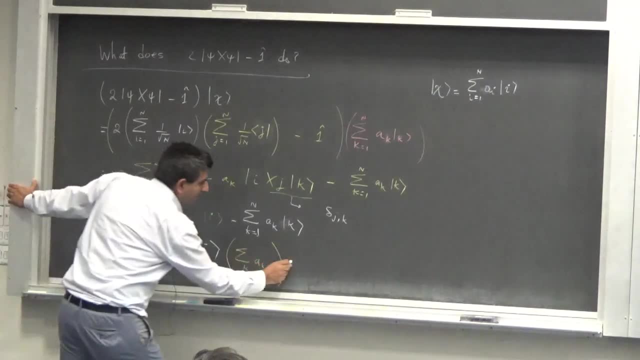 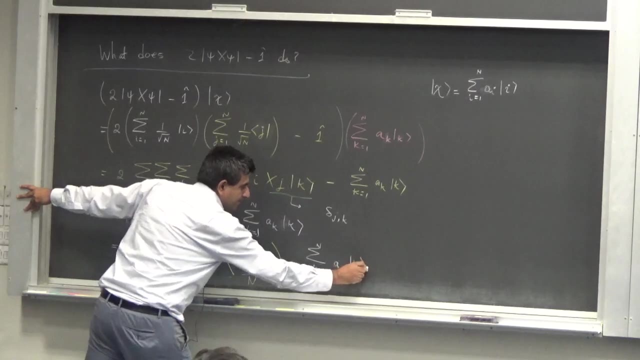 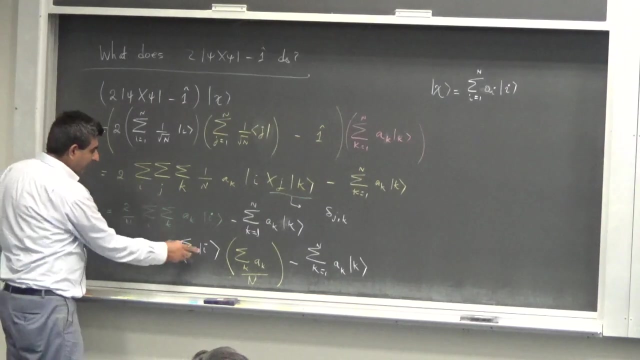 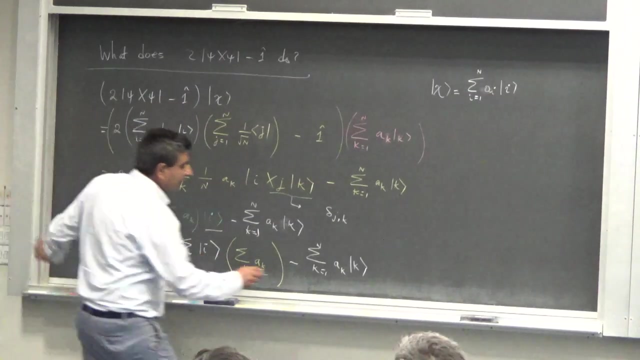 n. k got it, so this is. so I am just connecting this ket with this summation. this is independent, this has no Iota and it can just can be pulled out. Alright, so am I missing a factor of root n? so I can also write this as the formula: 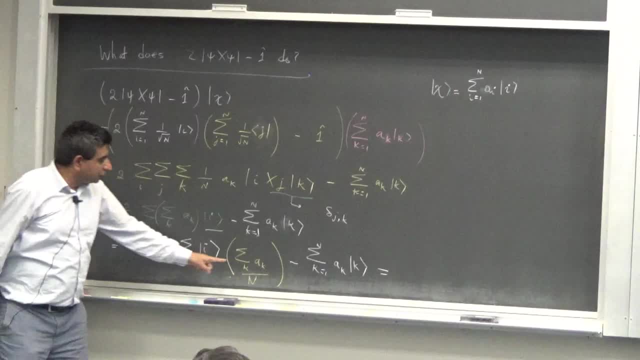 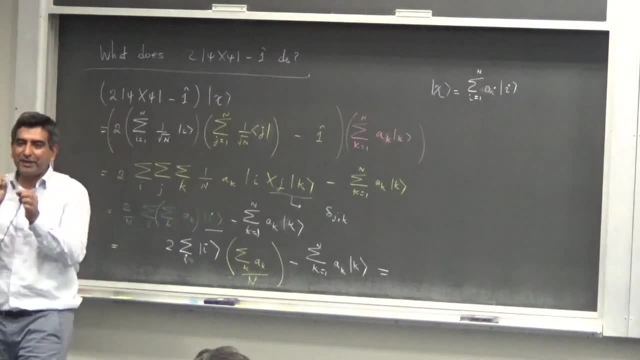 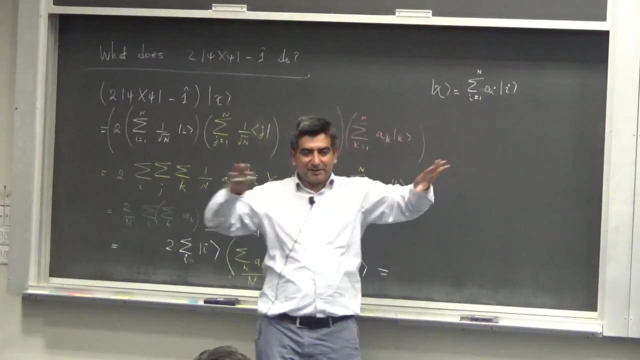 So can you imagine what this thing is? This is the number of MYT. is a number, a k, it's a coefficient, it's a probability amplitude, a k of a particular state, this state here, any arbitrary input state, and this is the sum of all those probability. 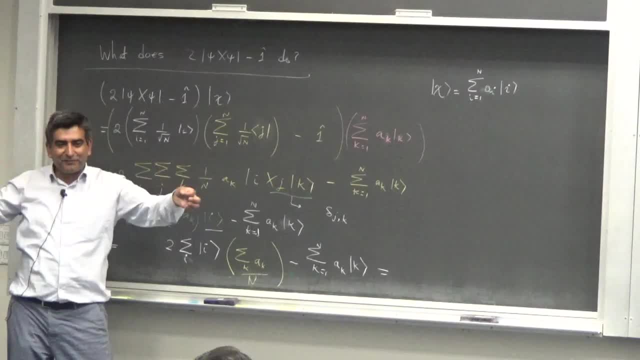 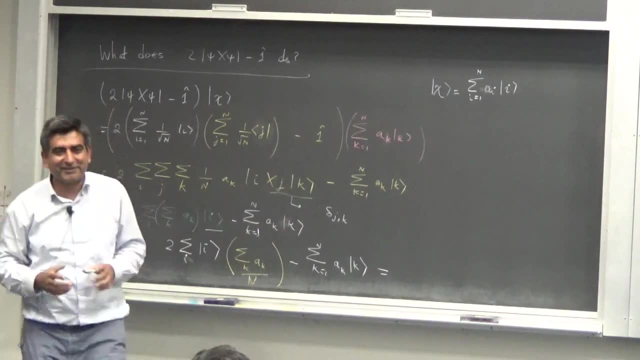 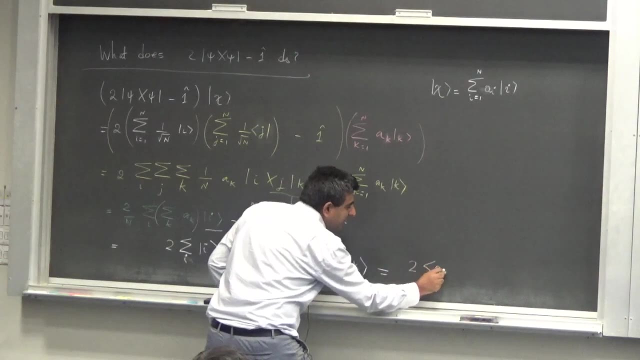 amplitudes and then you divide by the number of states. So what does this look like? This looks like a mean amplitude, this is a mean amplitude, So this thing becomes 2 times the mean amplitude. let's denote that mean amplitude by expectation value of a. a is. 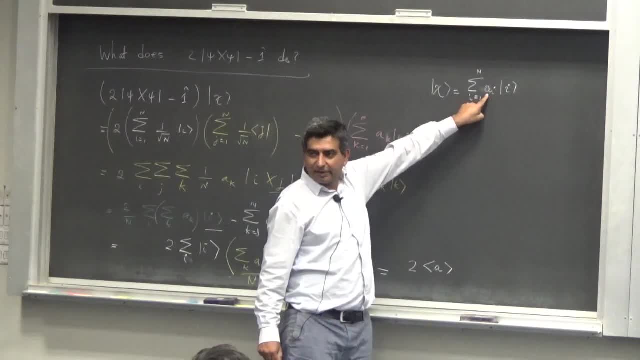 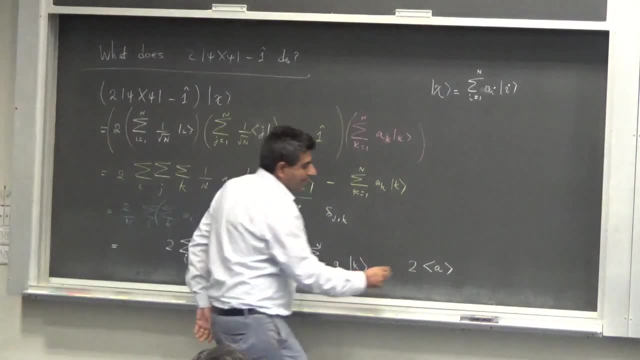 just a complex coefficient over here, right Now. this is a number, a pure number, and of course I also have this sum of all the i's, of all the i's right. So this is the number of the i's. 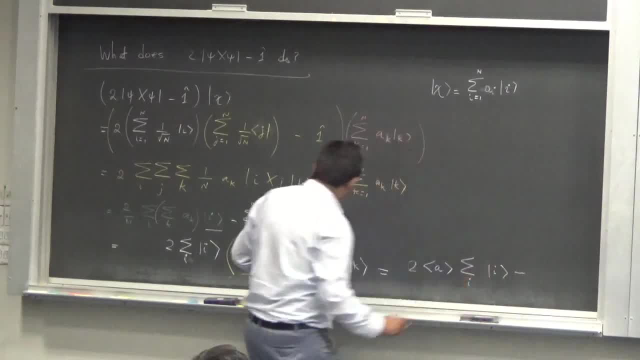 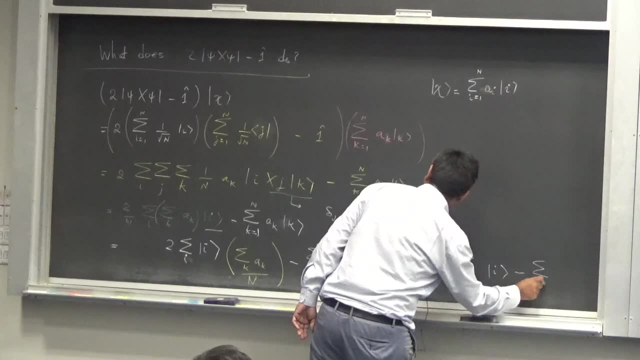 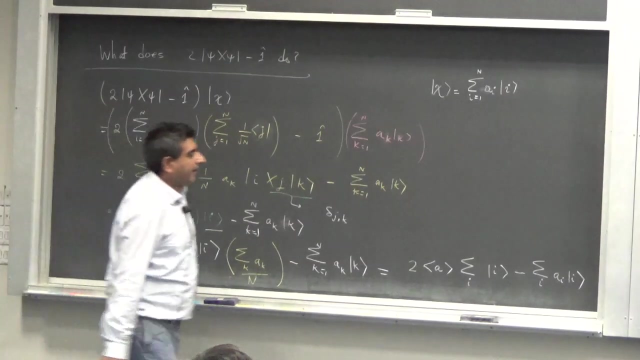 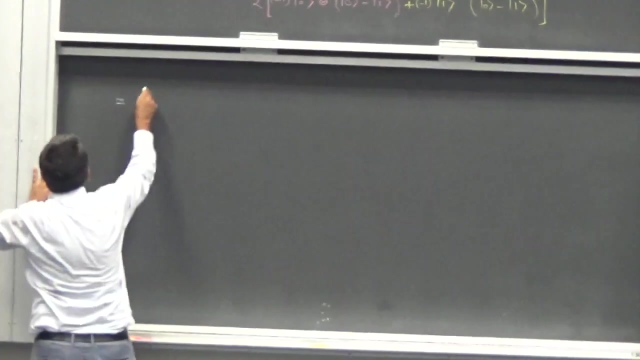 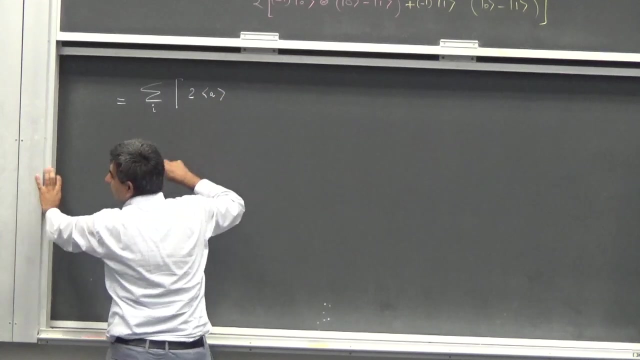 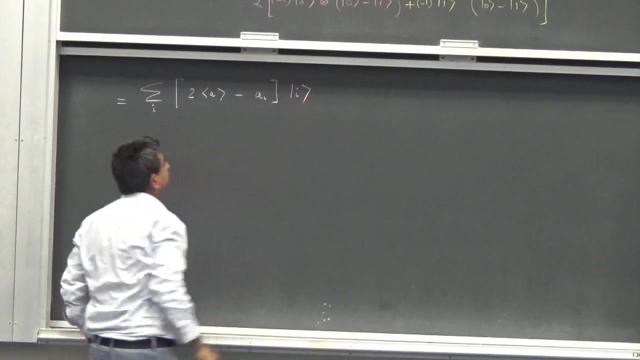 the basis states minus. now I can replace this index K with I, doesn't matter, so I can put this as I a, I get a I, and this eventually becomes sum of over I of 2 a minus a I. So what is the impact of this operator? this strange looking? 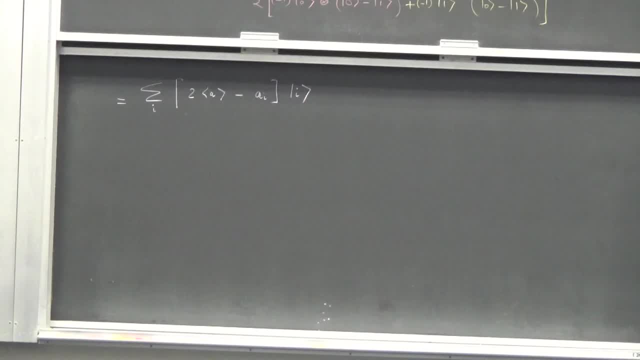 operator two times an outer product, acting on its arbitrary input state. what does this operator do? So what does this operator do? So what does this operator do? Just look at the output there. what does it do? the input was this: this was the input here. 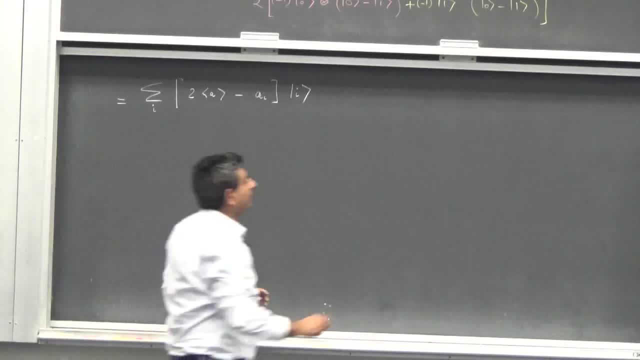 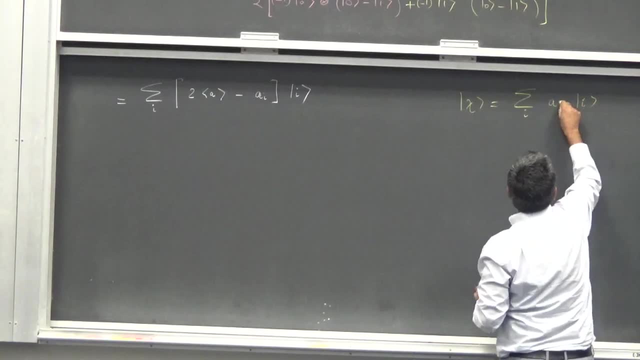 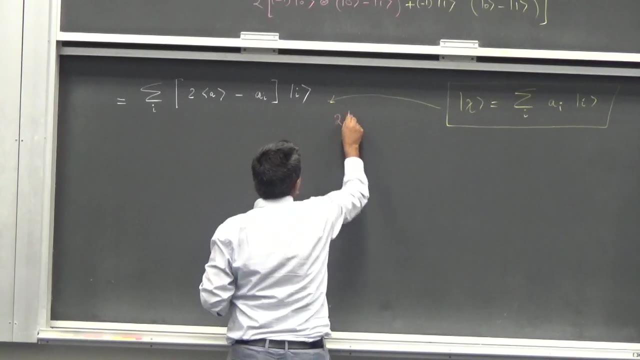 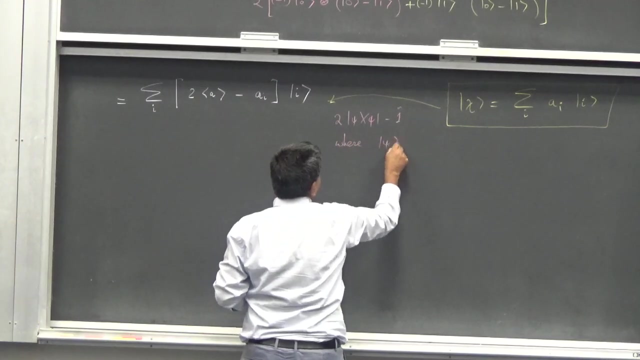 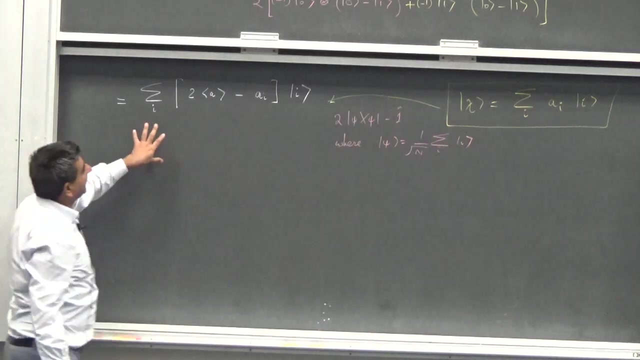 let me rewrite that input over here. ket I is sum over I of a I complex amplitudes basis state, ket I. now what the action of an operator to ket? psi, bra, psi minus identity, where psi is an equal superposition of all the states. what this does is that it just 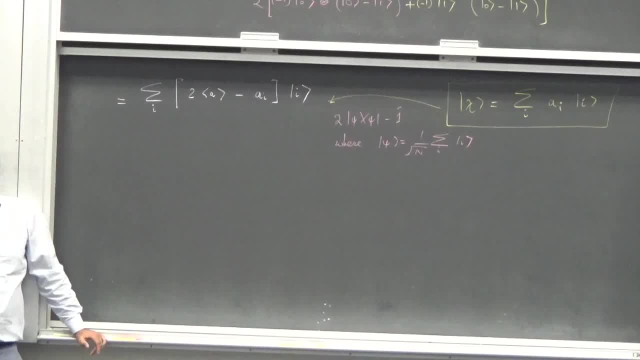 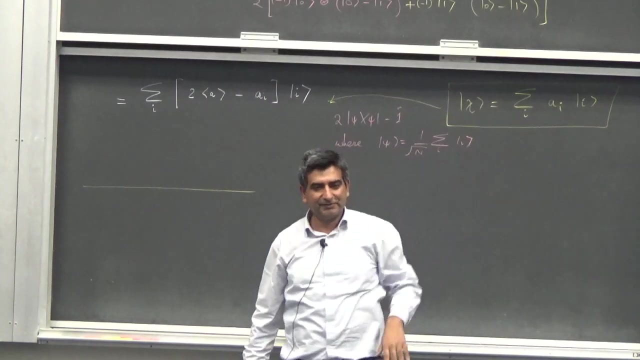 changes the complex coefficients. and how does it change the complex coefficients? Something really, really, really clever and strange. So if suppose- let's look at this graphically- you Suppose my input state were an equal superposition of all states, So all of these were one half. So I am looking at two qubits. Each one of this is one half. So I start off with. 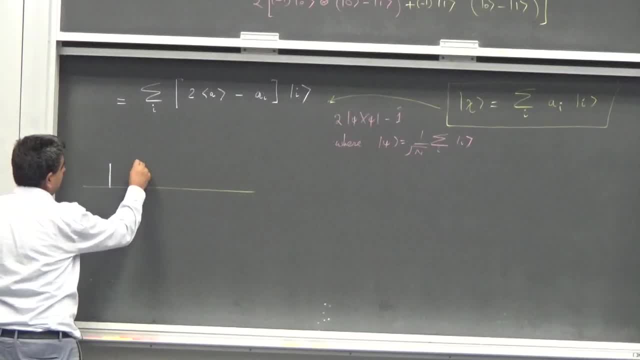 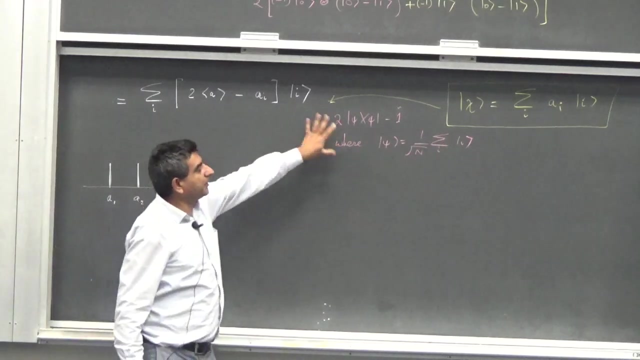 A1, A2, A3, A4.. So this is A1, A2, A3, A4.. Now, after this operation, a new state is formed. That new state, of course it can be written. 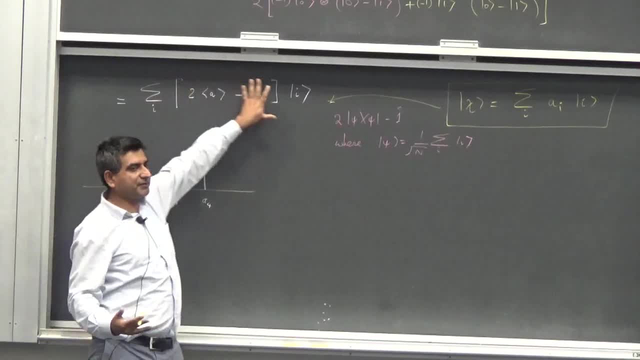 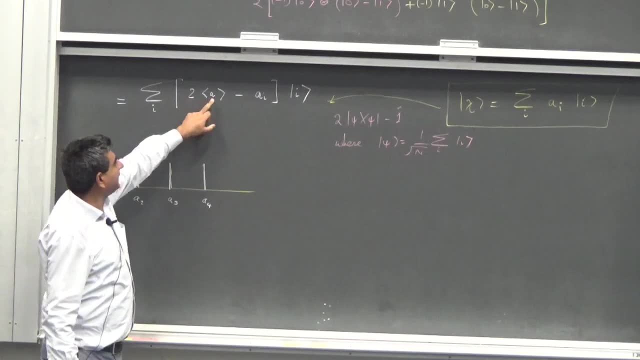 down in the same way. So this is A1, A2, A3, A4.. So this is A1, A2, A3, A4. So this is A1, A2, A3, A4. So this is A 2, A3, A3, A4. So this is A1, A3, A4. 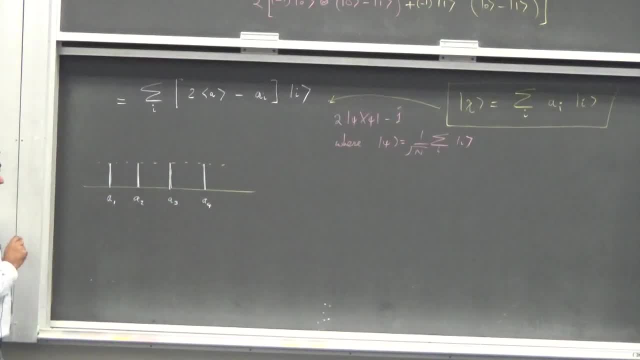 So this one is A: 2.. And this is A: 2.. So these are all states and B, Boo, B, D, C, D, O and C. The farthest state I am writing down is a 3 divided by number ofаб COME UP. 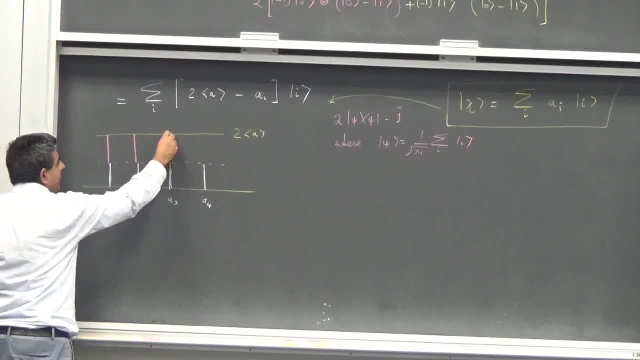 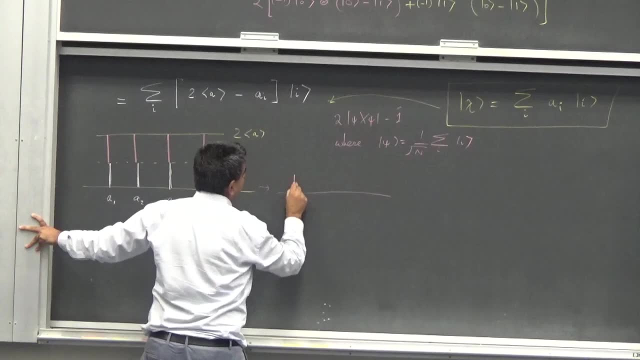 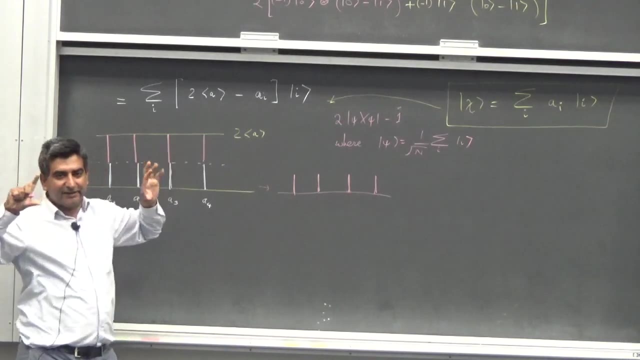 B 2, B A. So this is one half hot state I am writing down. insert these numbers in fraction. I get this. So I get back the same kind of distribution. it is of a different height. each height is now equal to 2 times the mean minus a. i for duciously, it is the. 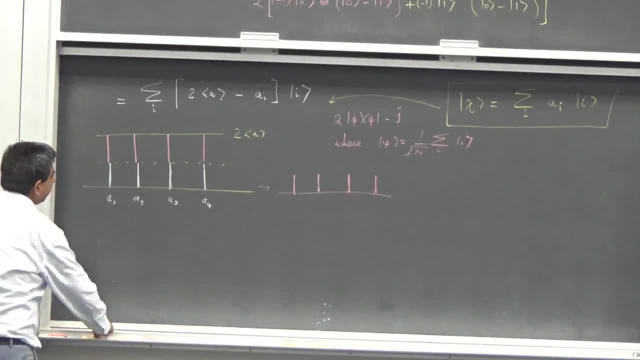 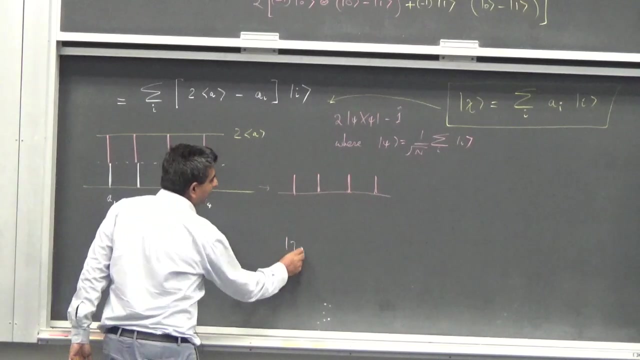 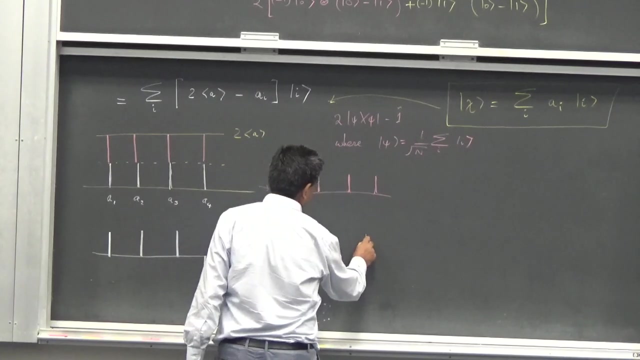 same in this particular example. but what if my input state is slightly different? what if my input state looked like this: if one of the amplitudes were negative? suppose my input state were this: say my chi were some: say, say, say, say, say, say 1. 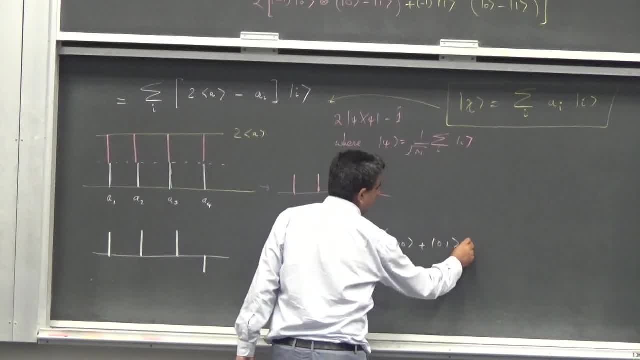 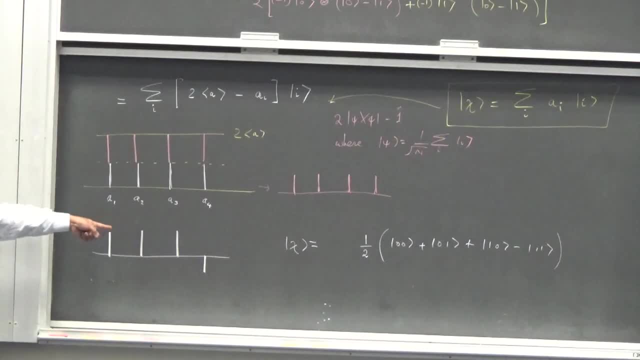 say 3, say 3 i. this is what my input state. so there is a legitimate state normalize. but now the four amplitudes, a 1, a 2, a 3 and a 4, look like this: one of them is negative suppose. 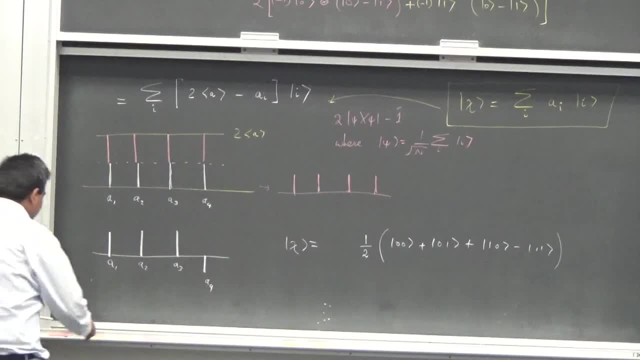 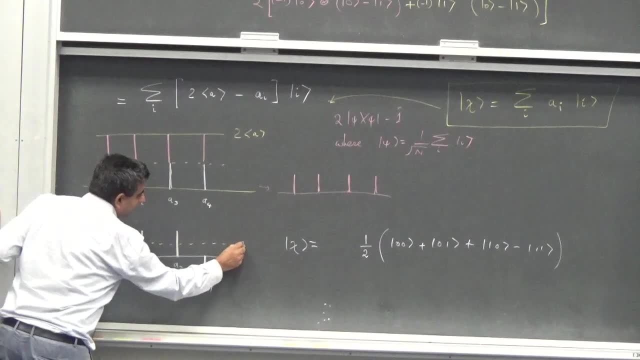 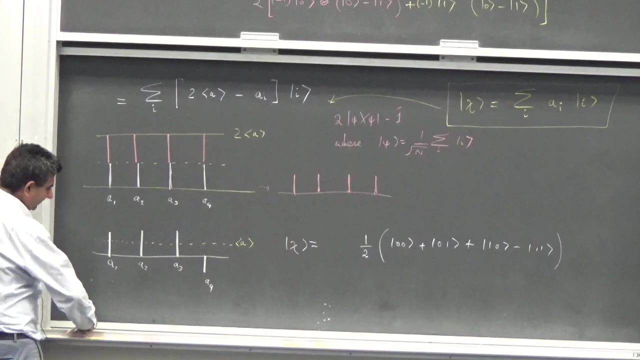 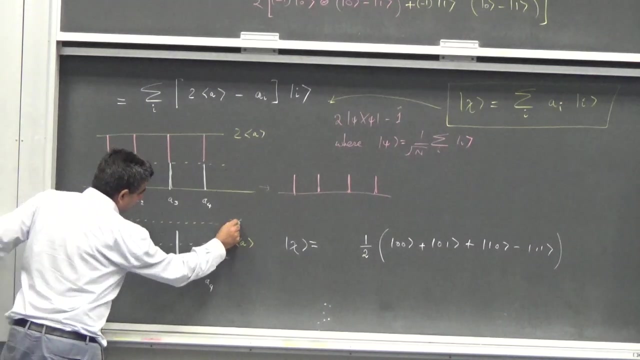 one of my input states is negative here, So of Now the average of these states will be somewhere here right, somewhere here. this will be average of these four numbers. I take the double of this. I get somewhere here 2 times this. 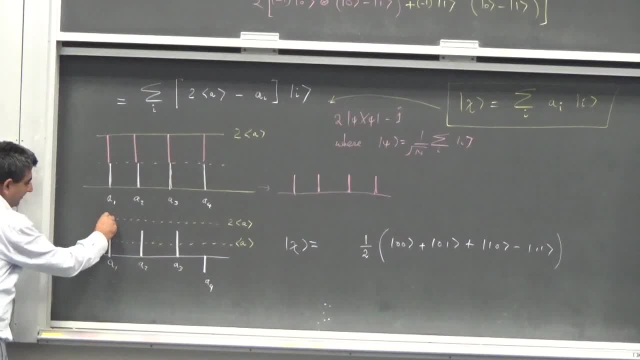 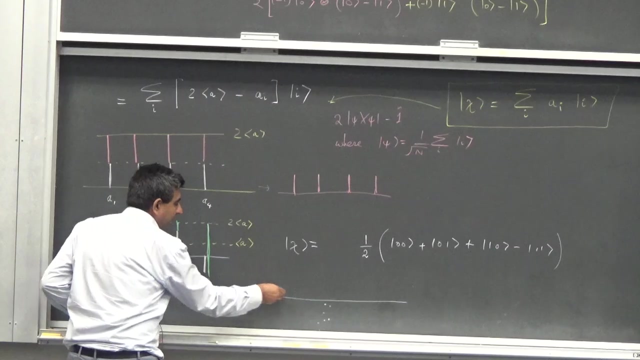 Now I do a subtraction, so I get this height, I get this height, get this height and I get, say, this height. So now the new state that has been created has the four amplitudes redistributed, three of them smaller And the fourth one we will use. 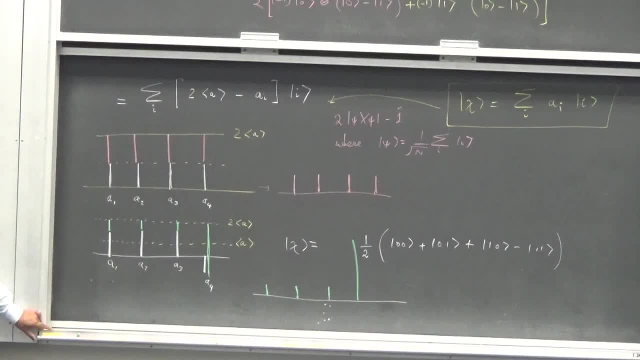 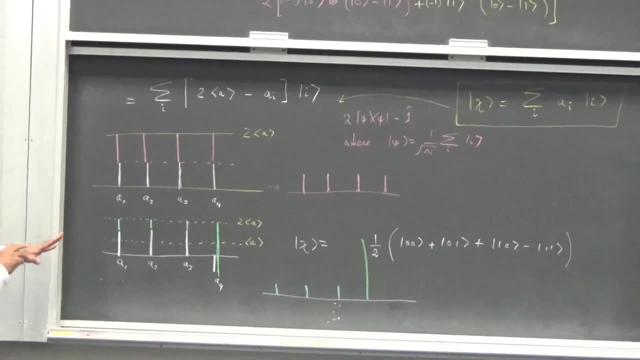 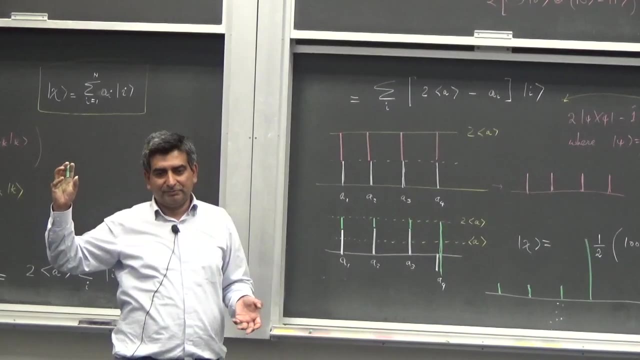 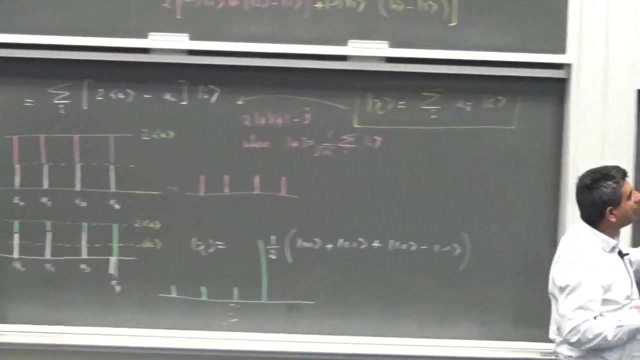 Okay, And the fifth one is going to be large. So if one of the amplitudes is of a different sign, then this operator that we have in the Grover's algorithm is going to amplify that response. So now, what we would like to do in the next class is to build on from here and see how. 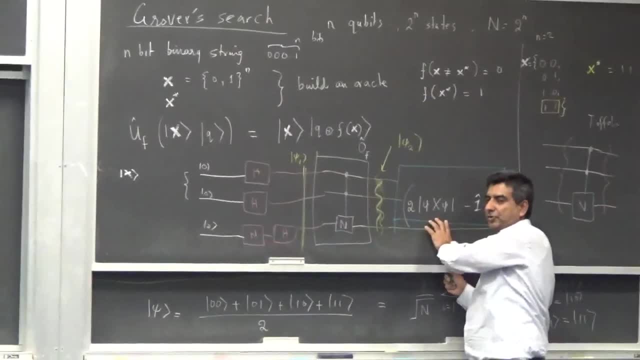 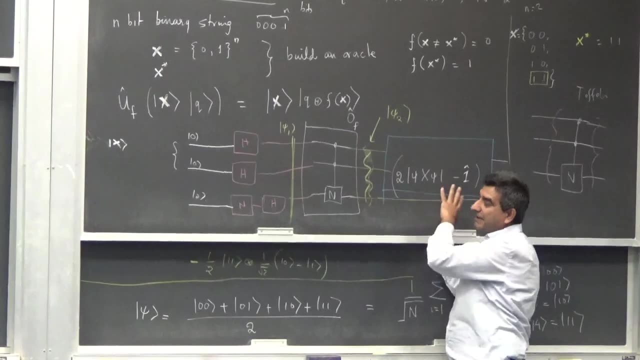 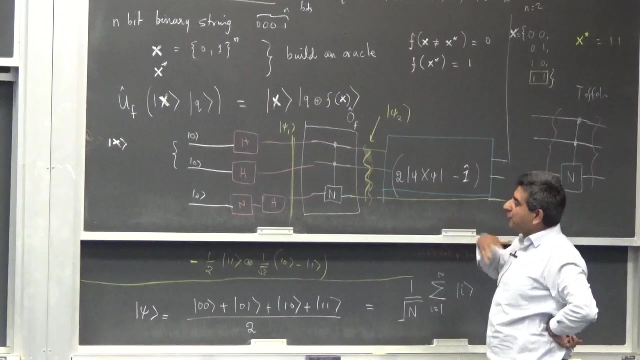 the combination of this oracle and this operator. Both of them together are called a Grover diffusion operator. How would they achieve this amplification If this were to amplify our? so what we want to do is we want to amplify our desired search solution. 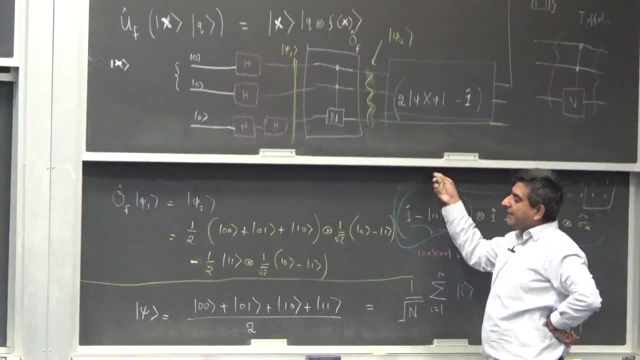 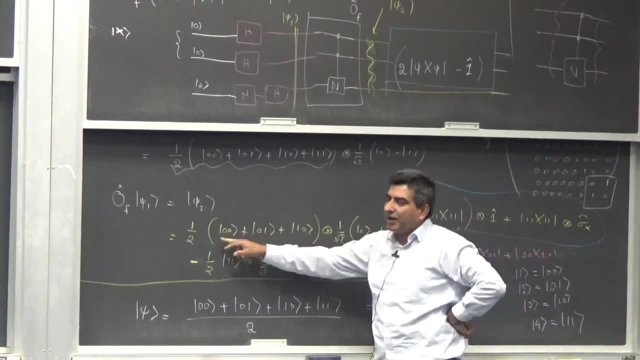 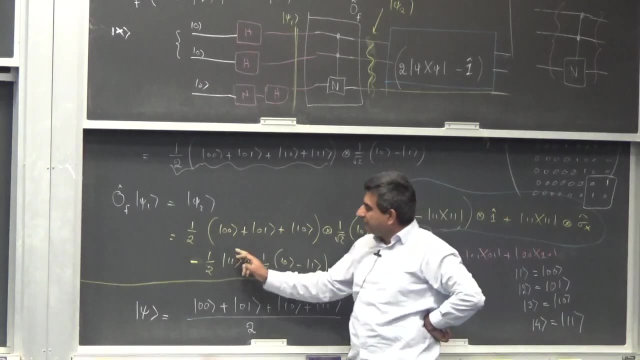 If that desired search solution accrues a negative sign, which it really does. over here you see all of these states which are not our solution. They appear, They appear with a positive sign- positive, positive, positive. But here the solution that we're looking for has accrued or acquired a negative sign minus. 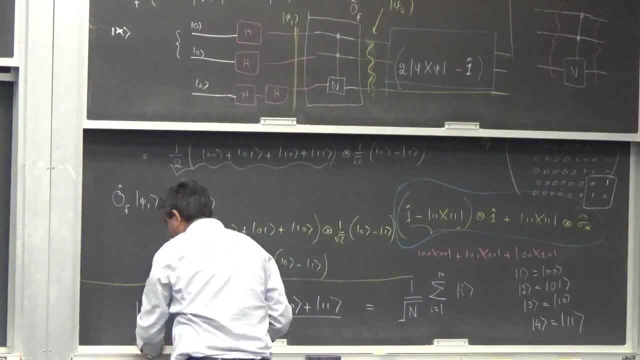 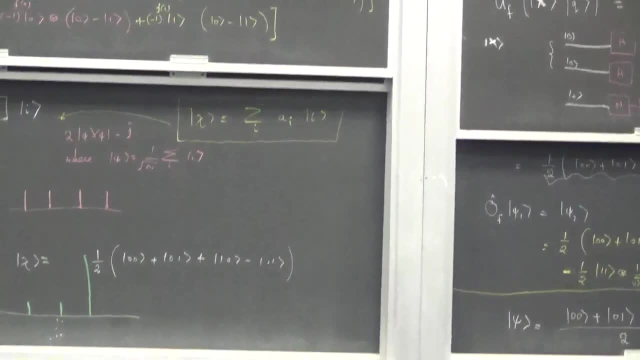 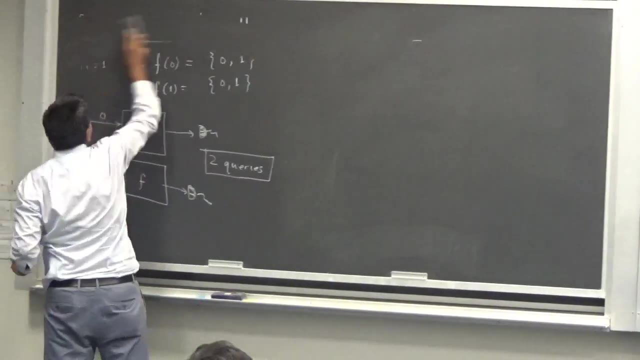 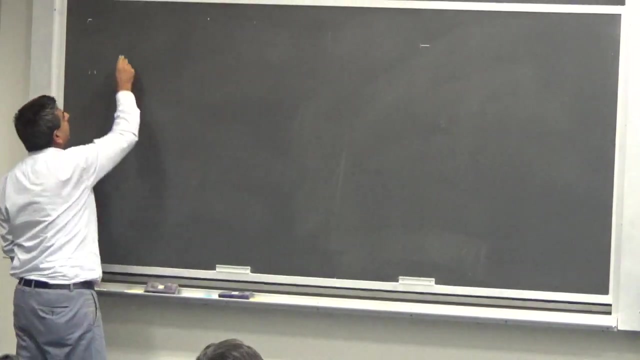 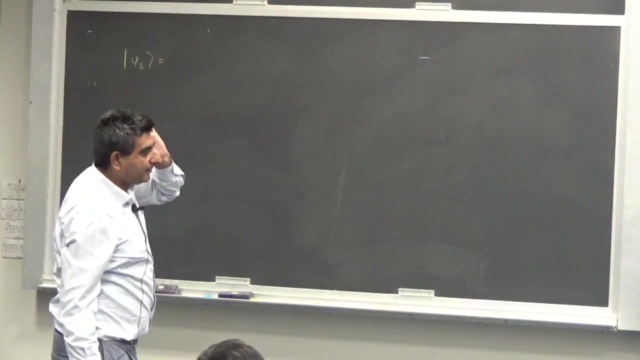 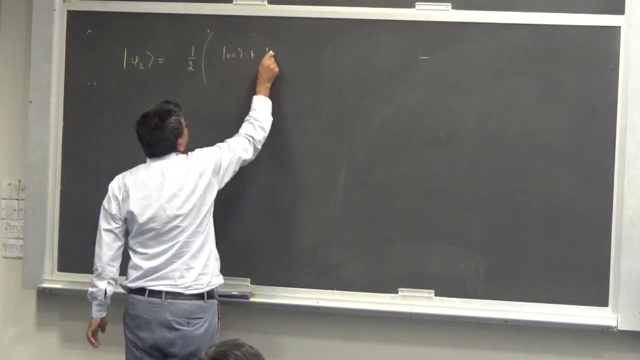 one. So if I were to look at this state side two again, let me finish off this argument. In fact we're almost done. After the oracle operator. my state side two is really one half zero, zero plus zero, one plus one, zero minus. this is really really important here. 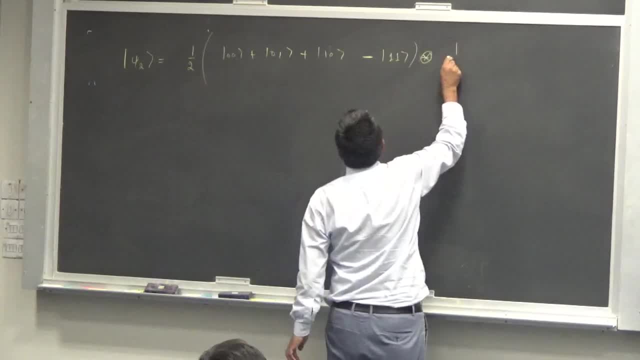 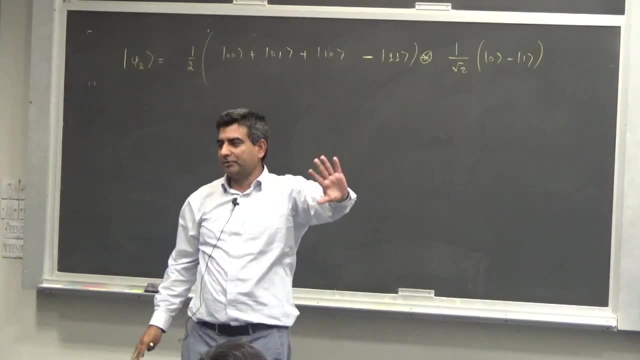 One over and root two One over and root two One over and root three One over and root three One over and root four One over and root five One over and root six One over and root seven. third qubit: the answer to the qubit. I don't care about the third qubit any longer, But now after the 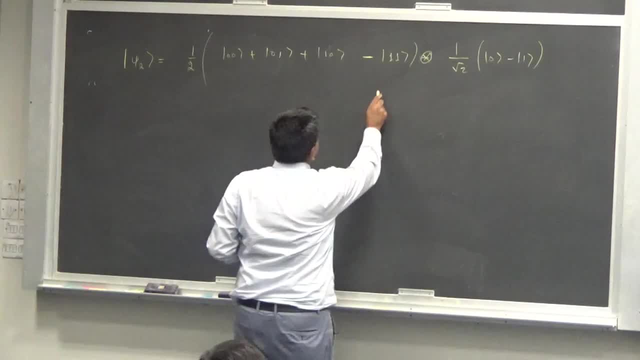 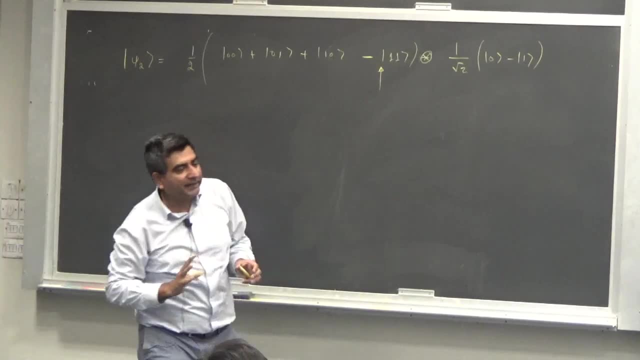 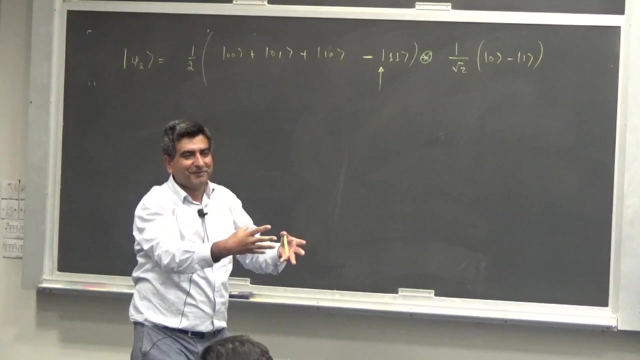 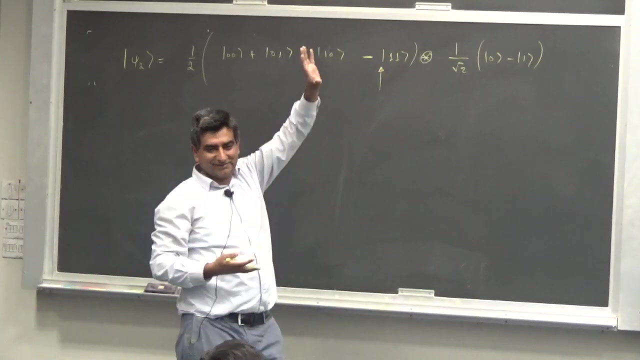 oracle operator, my desired solution has picked up a negative sign, And if this were to be followed by that amplification operator, the end result is expected to be one in which this probability corresponding to this state is enhanced and the amplitude corresponding to these three states is. 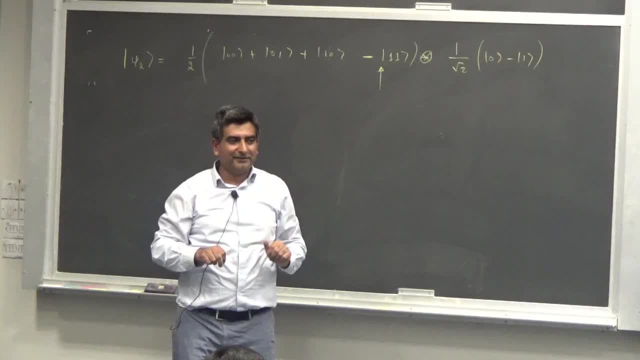 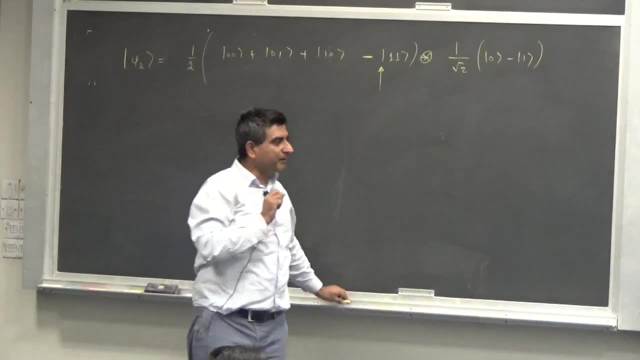 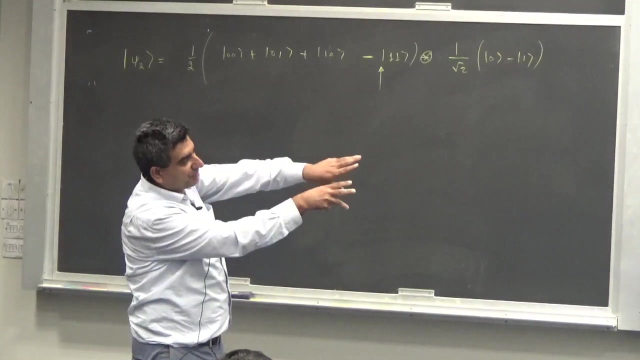 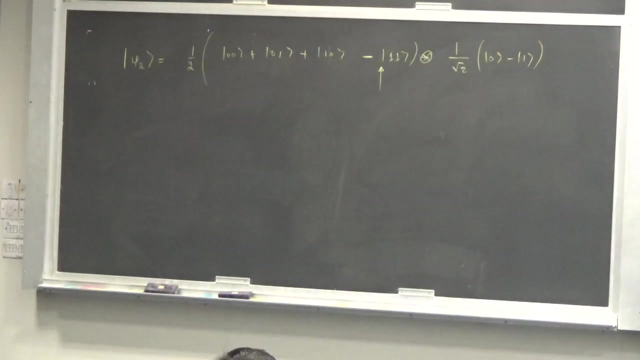 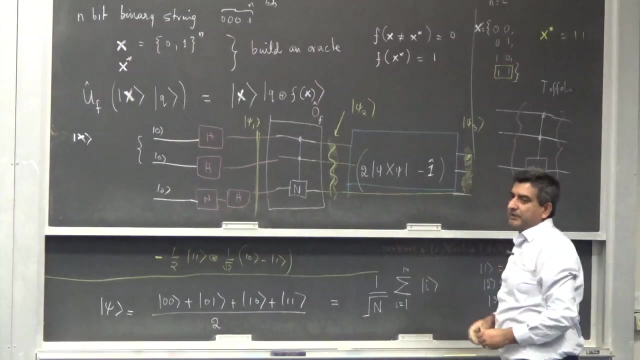 diminished, So my output state will be brimming with the desired solution. So, before we meet on wetness, what I would like you to do is apply the Grover operator, the amplification operator, sorry- onto this input state And tell me what the state would be at this location, slightly, Now that you know what the action of the 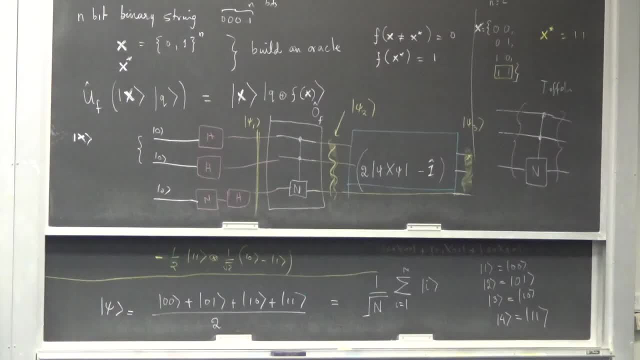 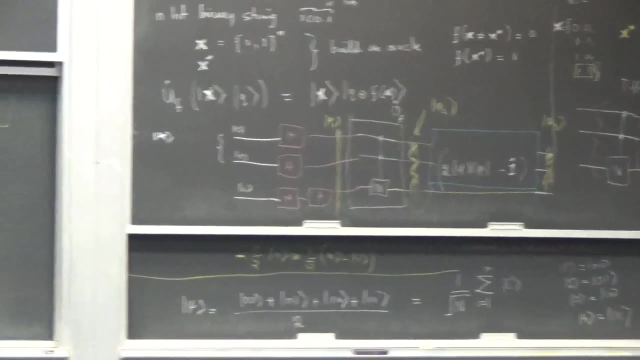 amplification operator looks like. So I would like you to precisely determine the probability amplitudes In the next lecture. we would like to start off with that. So I will look at the notebooks and see if you are able to find out the action of that amplification operator. So the solution is: 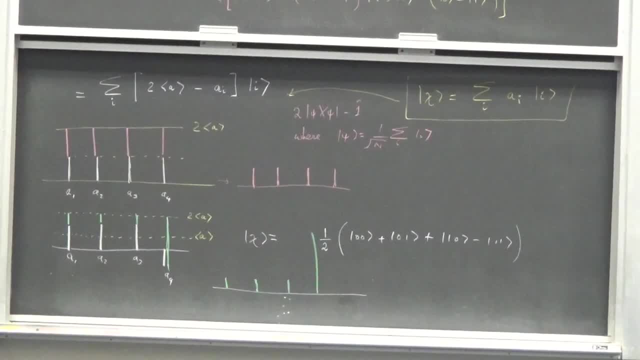 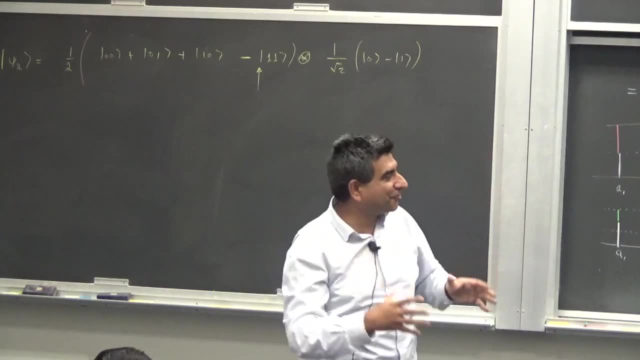 verified in its response And then we can detect it. So in the next lecture we would like to look at this from a geometrical perspective. I would like you to write the unitry operators for this. I would like you to write down what the quantum circuit for that amplification operator will look like. We already